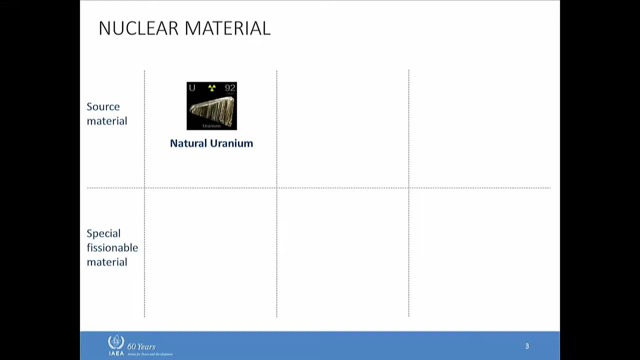 a certain stage in the nuclear fuel cycle where it's a suitable form and composition, it's subject to safeguards. So this obviously is naturally occurring. but if I take that and I put it through a process, let's say I have to do something else to it. we'll get into this, we'll have to convert it to UF6 or something. 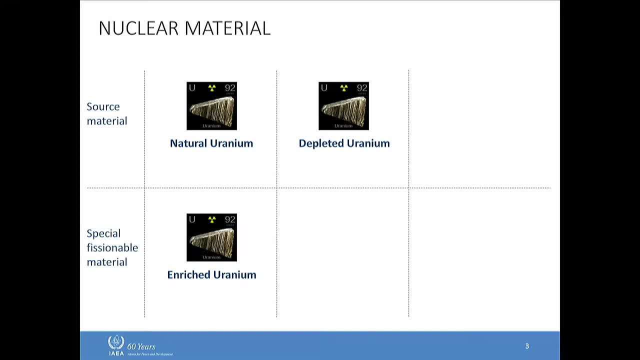 in order to enrich it. But essentially I can produce high-enriched uranium and the tails from that is depleted uranium. Are these both nuclear materials? They are, and, as you can see, one is what we call source material, the other is a special. 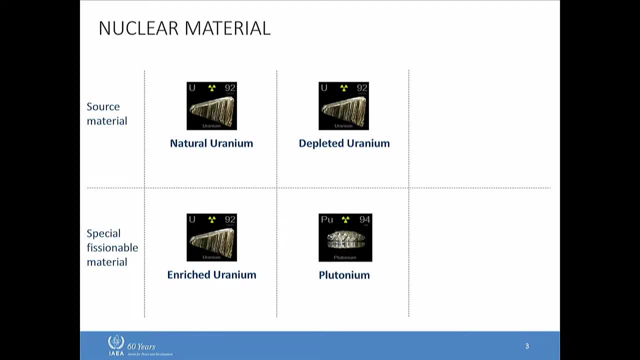 fissionable material, and we'll go into that in a second. I can also put this in a reactor, which we talked about this morning. a research reactor would be one possible source and I can irradiate the natural uranium for the depleted. 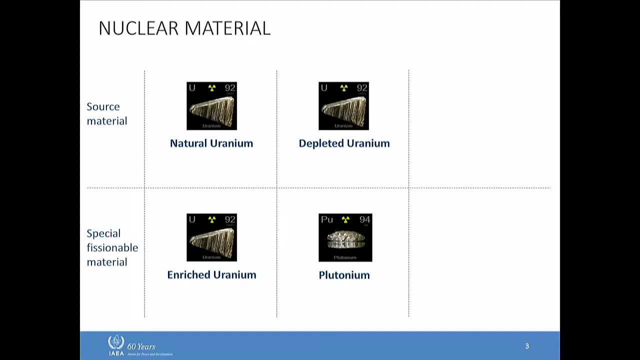 So I can irradiate the natural uranium and convert the U238 isotope to plutonium. primarily, PU239 is the isotope of concern. And then there's also one other fuel cycle, Yeah, yeah, exactly So the thorium cycle not very common. 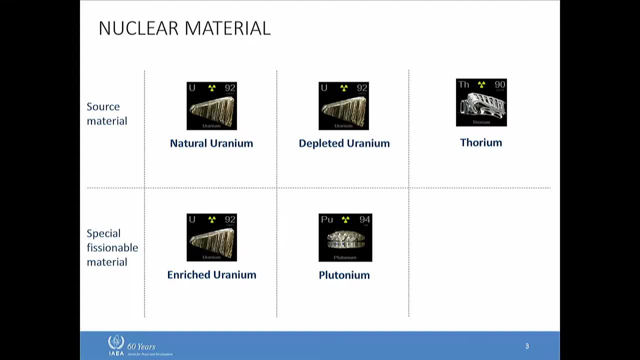 India has a pretty advanced program, has for years, but as far as the civilian fuel cycle, it's under safeguards, it's not widespread And you can produce similar to irradiating and separating. you can produce uranium-233.. So I just want to highlight that the materials up here, what we call source material, that's. 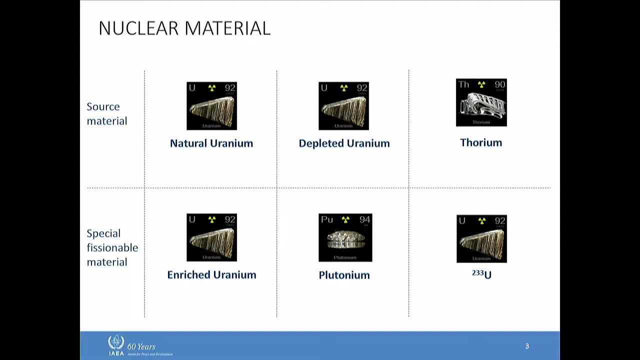 fertile material. Can you make a bomb out of that? Not directly, so we refer to it as indirect use of nuclear material. You have to do something to it, add what we call strategic value and turn it into special fissionable material. We'll go into that in detail, But 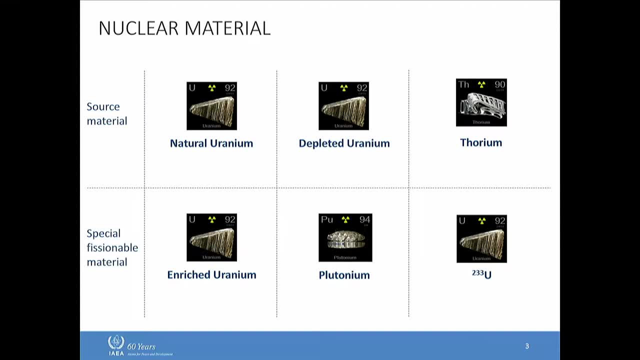 down here we have special fissionable material. You can make a bomb out of this directly if you have the right amounts. So there's a term we call significant quantity And this essentially is how much nuclear material you need in order to make a nuclear explosive device, Or it can't be ruled out. So I just 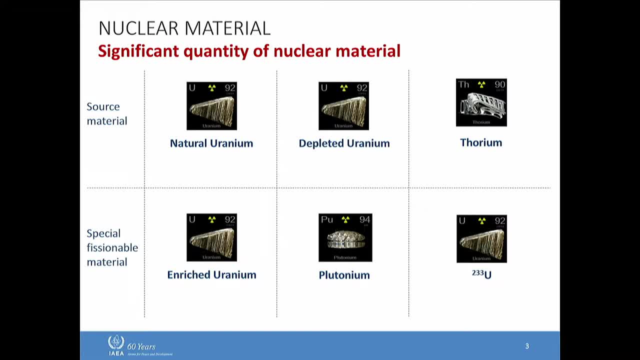 want to highlight. these would be good numbers to know. You can see, for the source material. we're talking tons of it. So naturally uranium we need 10 tons of naturally uranium. Depleted uranium- 20 tons. So if anyone's familiar with UF-6 cylinders, you basically need two large depleted uranium. 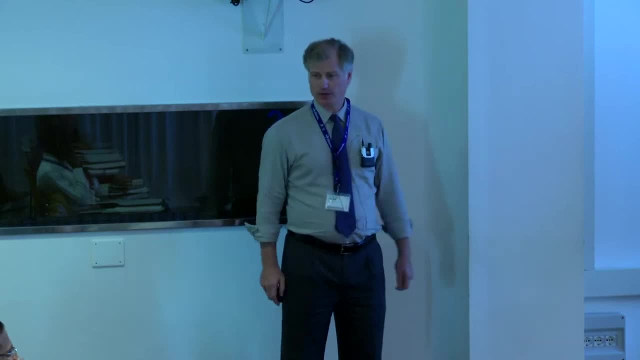 So you can see for the source material, we're talking tons of it. So naturally uranium, we need 10 tons of naturally uranium Depleted uranium- 20 tons. So if You would need two large depleted uranium UF6 cylinders to get 20 tons, 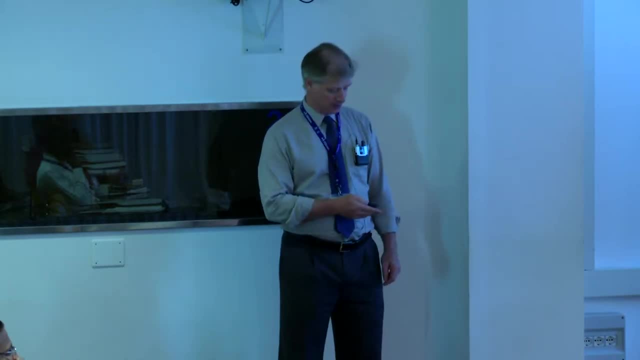 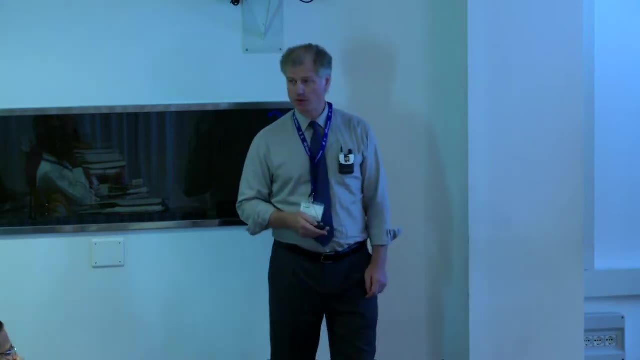 Thorium is also 20 tons. So lots of nuclear material would be required- Again ton amounts. And then for the special fissionable material, the SQs are much lower. So, as you can see, for plutonium it's only 8 kilograms. 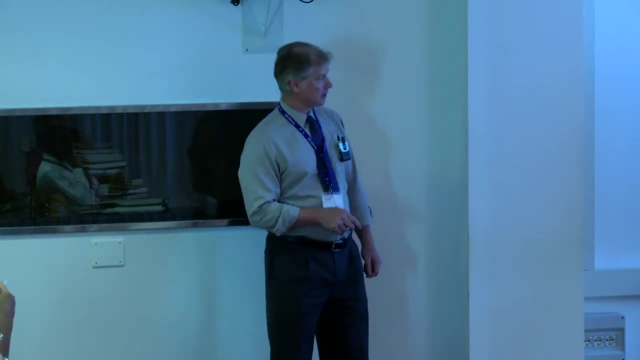 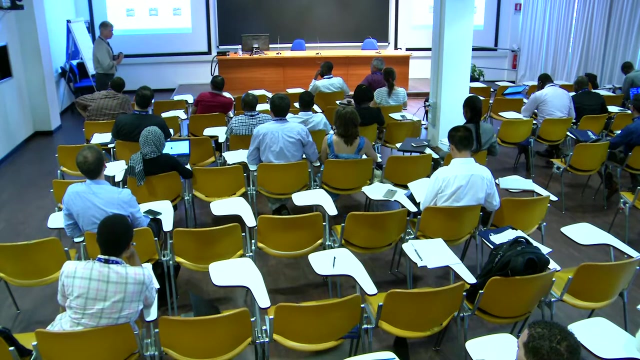 So a much lower amount. Uranium-233 is the same. I have to clarify here, and we talked about it this morning: Once uranium goes above 0.71, when you take it out of the ground- 0.71, you put it through an enrichment process: 0.72,, 0.8,, 0.9,, 1,, 2, 3.. 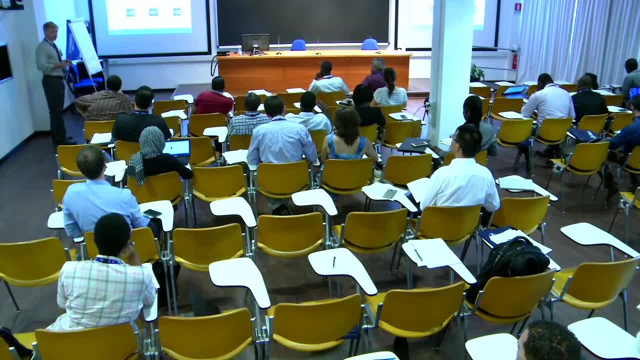 Now we call it low-enriched uranium, Usually for reactors. as you probably know, they stop at about 3% or 4% For fuel for power reactors. for research reactors they may go a little higher, maybe up to around 19% now. 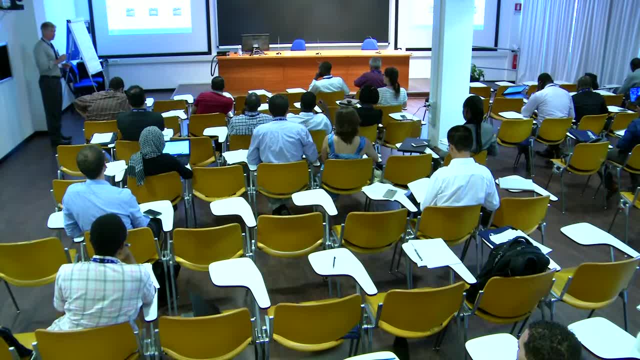 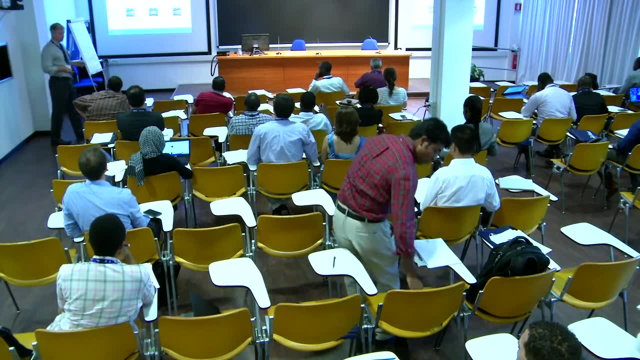 There are some research reactors that still operate on high-enriched uranium And HEU is. when you go above this 20%, It's just somewhat arbitrary and it's spelled out in the statutes of the IEA. So 21% Okay. Can you make a bomb out of HEU? Probably not At 30%, 40%, 50% probably getting. if you have a sophisticated country and they have some know-how, maybe probably be a pretty large bomb, But 60%, 70%, 80% when you get those percents of U-235 isotopes. 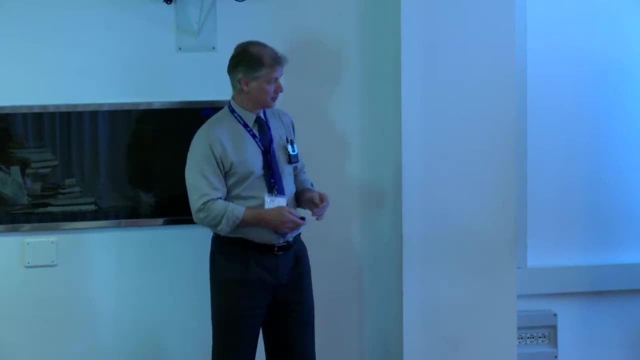 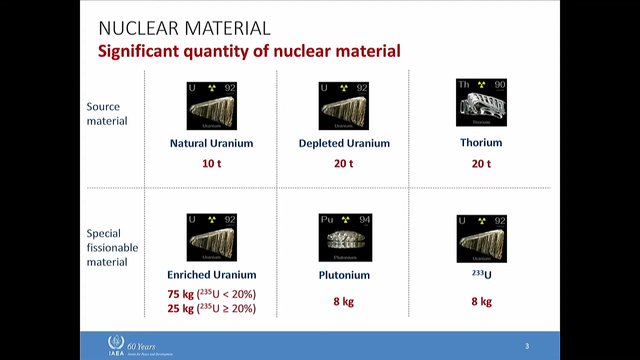 especially in the 90%, 92%, 93% range. it's getting much smaller And you can see the significant quantity drops down drastically down to about 25 kgs. Not that much material really. So from a safeguard standpoint, 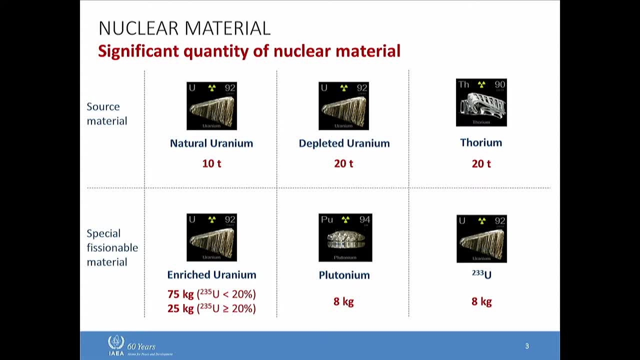 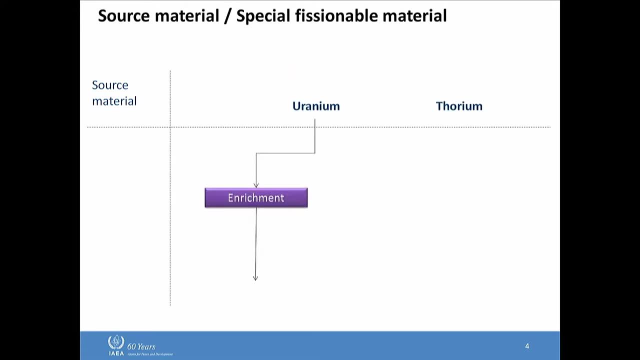 these are the numbers we're concerned about. We sample and we verify against these numbers. Now, just to highlight, it's not just about the nuclear material, There's also processes. So we safeguard the nuclear material. We also safeguard the facilities where these nuclear materials are located. 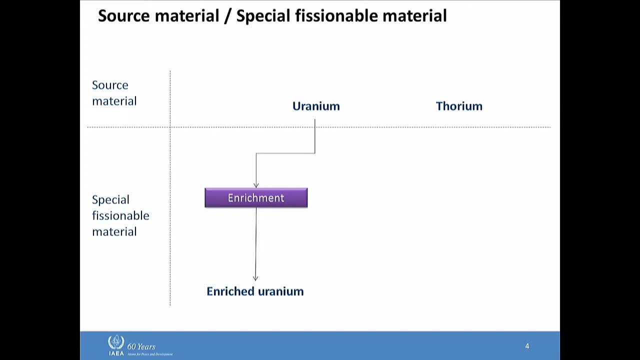 So, as I mentioned for uranium, if you enrich it you can make high-enriched uranium. So enrichment is a very sensitive stage of the nuclear fuel cycle. Likewise for uranium and thorium: you can use it in a radiation path, put it in a reactor. 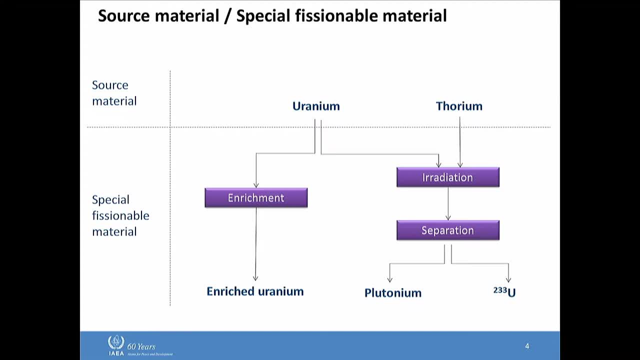 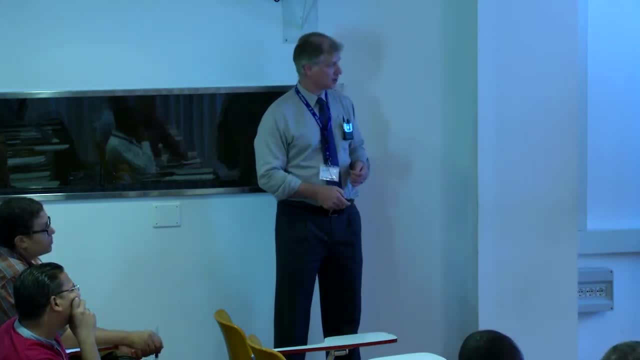 And then you need to separate it because it still has fission products, actinides, other things you have to remove from it in order to have plutonium and uranium-233.. And I should highlight that ultimately, you need these in a metallic form. 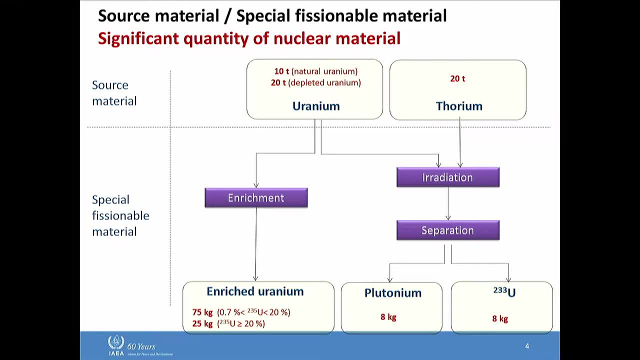 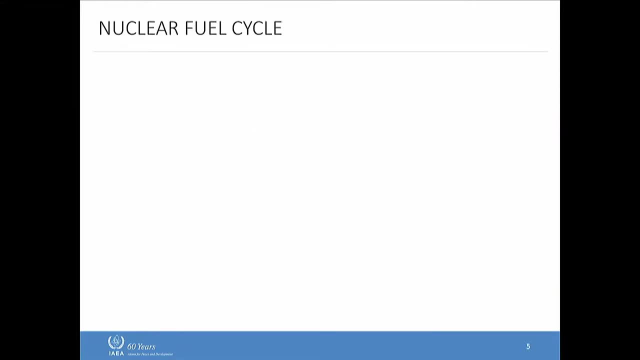 And just as a reminder, those are the significant quantities, And just keep that. maybe, if you're a test, keep this number here for plutonium, 8 kgs- in mind. So real quick, let's go over the nuclear fuel cycle. 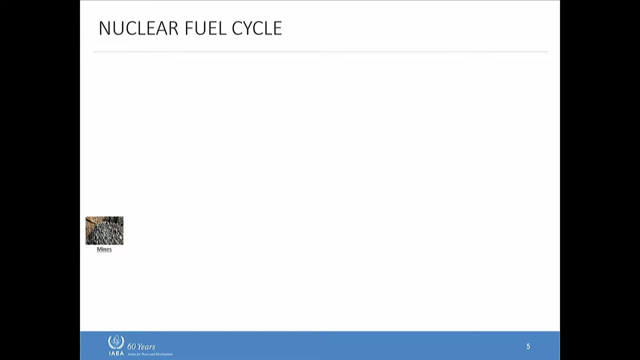 I think you had this earlier in the week. But uranium comes out of the ground. could also come from other sources. Could come from phosphates, could be a byproduct of gold mining, copper mining. There's some research into extracting uranium from seawater. 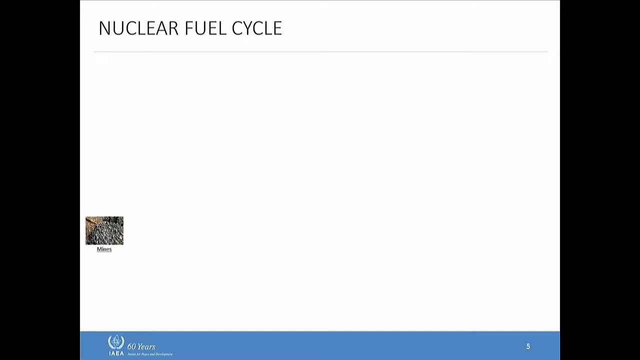 Not very viable commercially, but it's theoretically possible and practically possible. So it's been done. Once it comes out of the mine, usually it goes to a milling and a concentration plant. It's still not under safeguards. Let's assume this is uranium here. 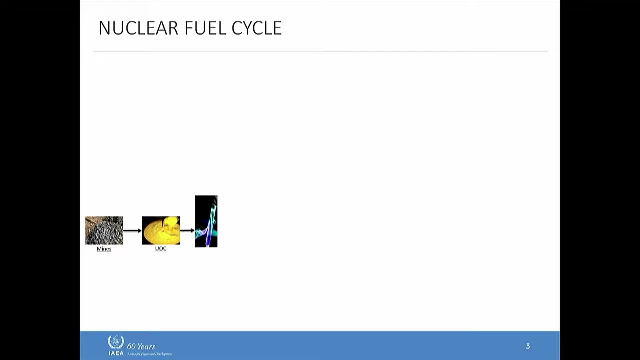 It still wouldn't be under safeguards yet. But once it goes to the next step, conversion, it usually has to undergo some kind of chemical conversion process for the nuclear fuel cycle, So let's say UO2, in order to be used as fuel. 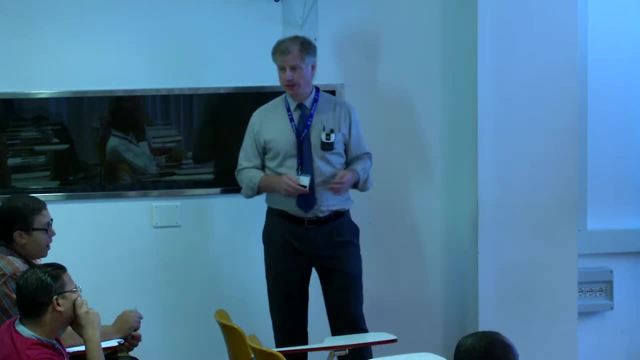 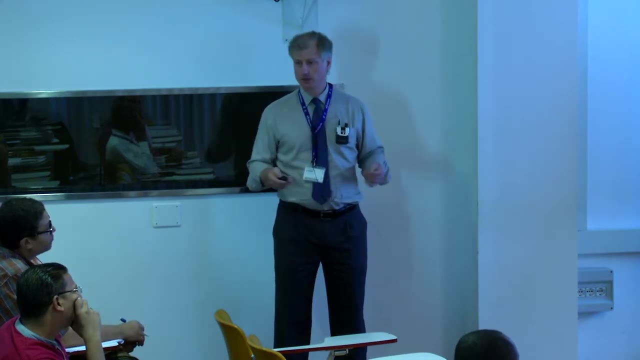 It could also be uranium metal, It could be some exotic uranium carbide if it's going to a research reactor fuel, Or maybe a UF6 compound if it's going to be used in enrichment to be enriched And then it'll be further converted to UO2, typically for fuel. 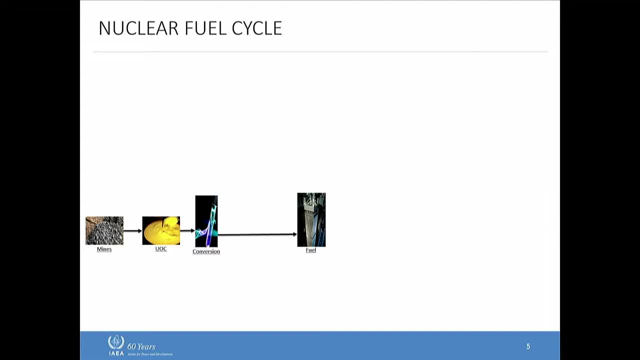 But at this point- this is generally. this is where safeguards will start. When I talk about safeguards, I mean detailed nuclear accounts where the state is obligated to report information and the agency inspectors will verify that information. After conversion, it could go directly into fuel. 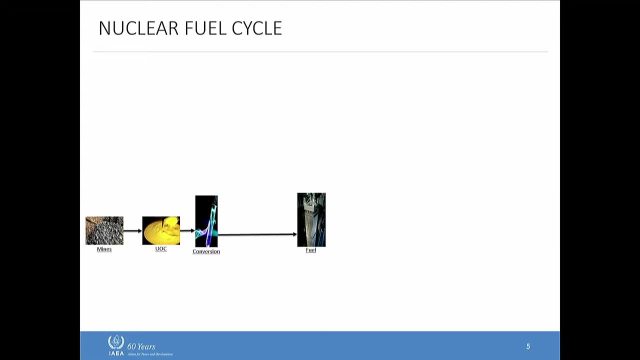 This is a little bit misleading. This wouldn't be an LWR type assembly. But if it's not enriched and it's just naturally uranium based, it could be converted into, let's say, an on-load reactor bundle or a candy type cycle. 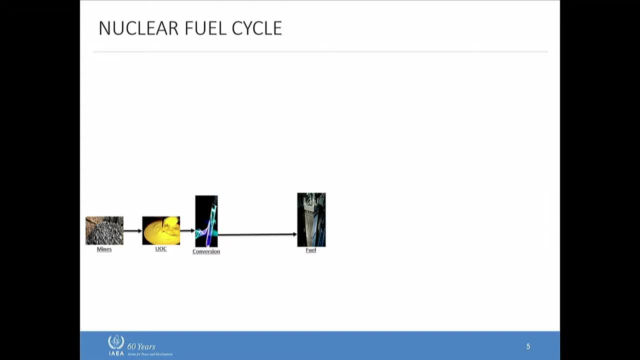 Or Magnox would also work. But if they want to use it in an LWR type reactor, they'd have to first enrich it. So it'd have to go through an enrichment process, some sort of enrichment services, and then they could bring it back and make fuel out of it and fabricate fuel. 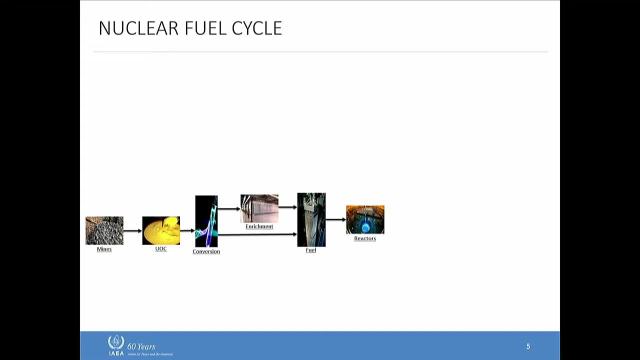 Eventually, though, this would go in a reactor, And this reactor, as I mentioned, like the enrichment plant, is a sensitive part of the nuclear fuel cycle. because what did this reactor? what does this reactor do when we make electricity Or medical isotope? if it's a research reactor, 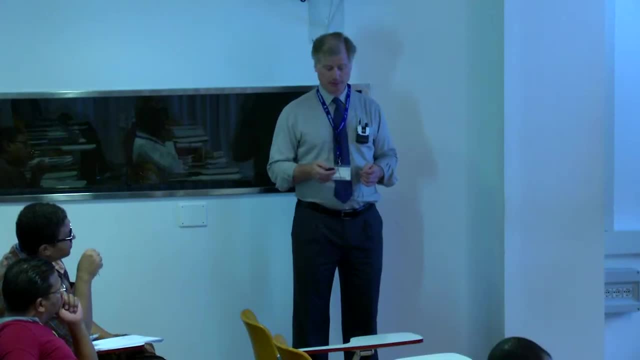 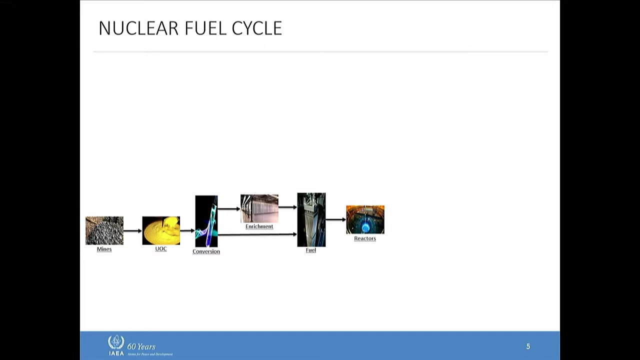 It converted that uranium- U238, into plutonium. So this added strategic value from a safeguard standpoint. We're still concerned with fuel fabrication, with LEU fuel, But putting it through the reactor created plutonium inside that assembly So it's more sensitive from a safeguard standpoint. 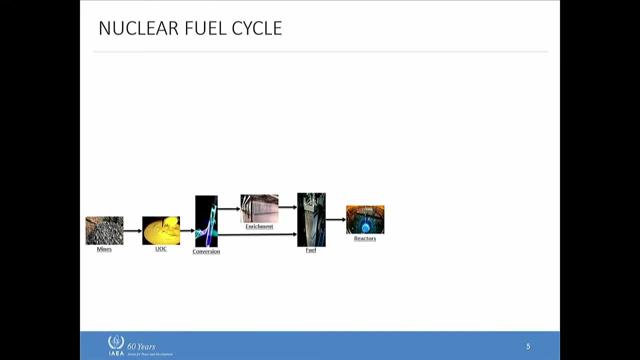 The good news is it's heavily irradiated, So it's got fission products with it, actinides with it, So it's not easy to get to. So in that sense we call it self-protecting. It usually has to go into a pond or cool for a few years. 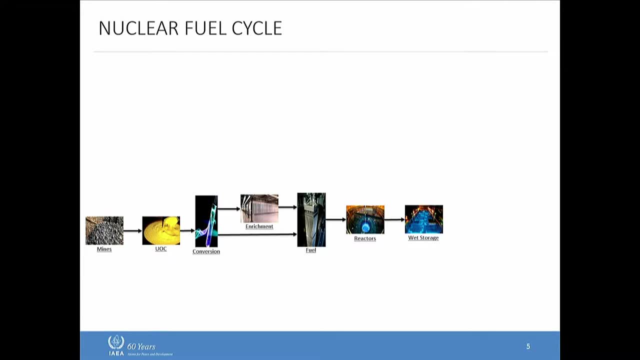 Depending on the burn up and the radiation history. Typically it's for power plants in there for three cycles, So three years about, And then it goes into wet storage. It's cooled in a spent fuel pond for three, four, five years. 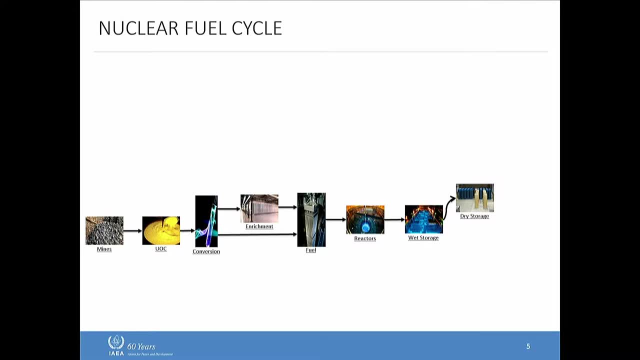 Sometimes longer. Usually it's determined by capacity. Once they fill up the pool, they've got to do something because they can't discharge any more fuel into the pond. It's that capacity So usually transferred to what's called dry storage and large casks. So you still need this heavy shielding, Even after it's cooled 10 or 15 or 20 years. you still need it. Even after it's cooled 10 or 15 or 20 years, you still need this heavy shielding. Even after it's cooled 10 or 15 or 20 years, you still need this heavy shielding. Even after it's cooled 10 or 15 or 20 years, it's still highly radioactive And that's a benefit from a safeguards perspective. The other option is a country could go a reprocessing route. Not many countries do this. Some of the advanced nuclear fuel cycle states, like France and Russia, do this. 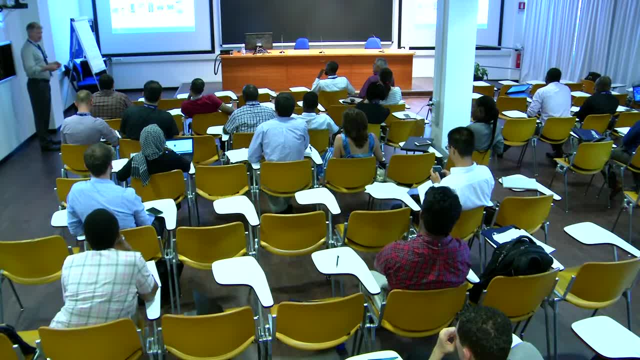 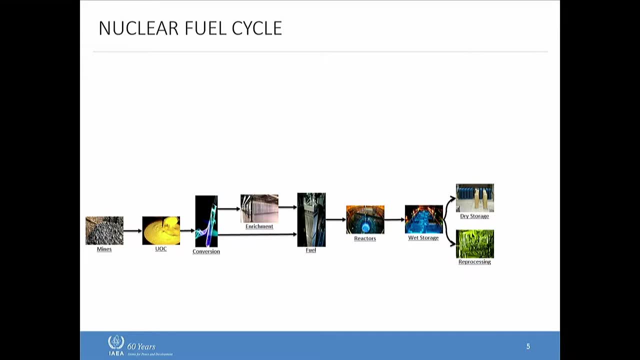 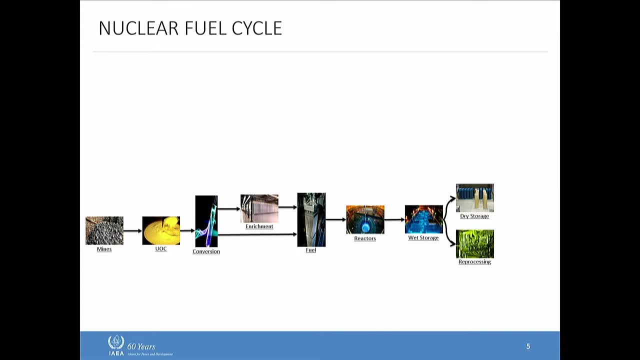 which is still useful. Most of the uranium isn't even consumed, So it's sort of a waste if it stays in the fuel. If you extract it it becomes an asset again. But it also took away those fission products. So this material went from being what we call irradiated direct-use material to unirradiated. 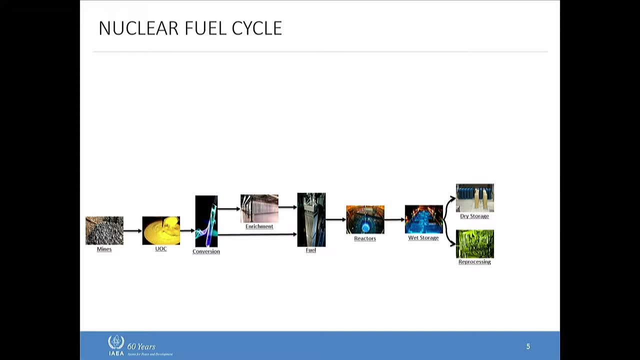 direct-use material, Very attractive from a safeguards perspective, And sometimes a country might do this. Japan does it for mixed oxide fuels. So they'll mix the uranium they recover, Or they can mix the depleted uranium, mix it with plutonium and they'll make a MOX fuel. 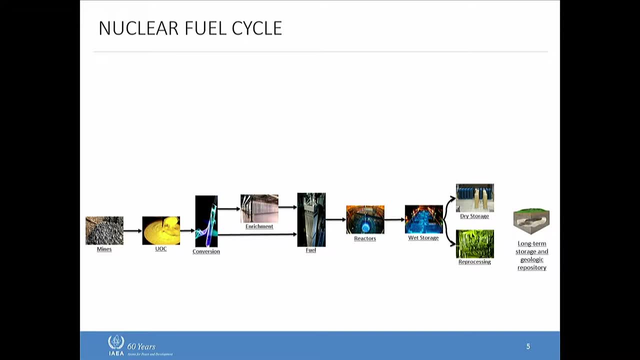 The other option in a couple countries looking into this is a long-term repository, So Finland. I don't know if they'll come online, but maybe in the next decade or so they're looking at a repository. They've been doing it for a while and testing. 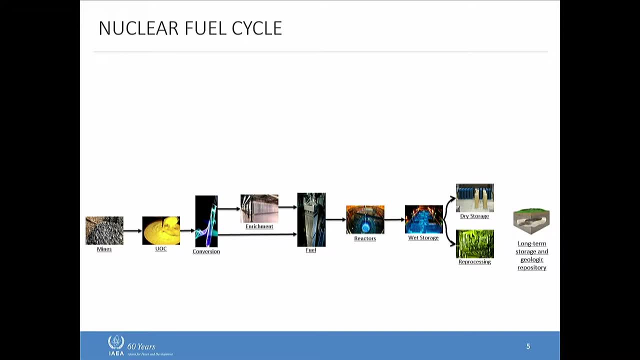 Sweden also has an underground facility that they're testing, So maybe ultimately they'll put their spent fuel into a repository. That's sort of an advantage from a safeguards perspective because it's below ground, very far down, As long as the repository is irretrievable. 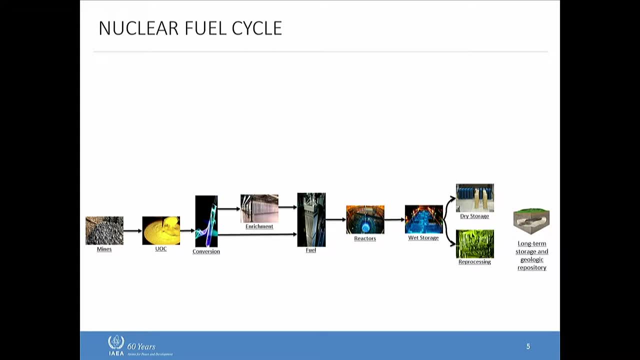 But you'd still probably need some safeguards measures on that repository once it's operational. And just to highlight: to have a fuel cycle like this- and this is pretty extensive- This would reflect something like Germany 15,, 20 years ago. Germany's a bit in decline now. 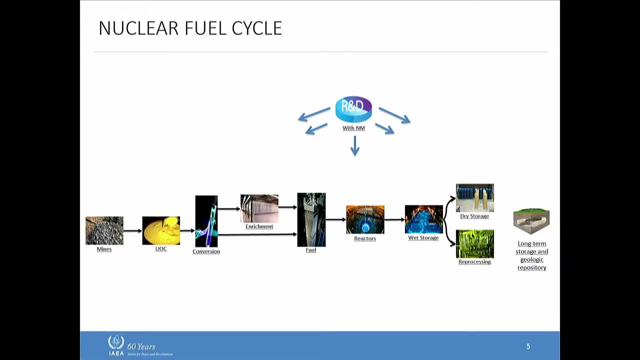 Japan, maybe South Korea. You need some R&D associated with that And you can have research and development without nuclear material You can. also, you'll need some kind of manufacturing base. So if you're going to have your own reactors or export reactors, 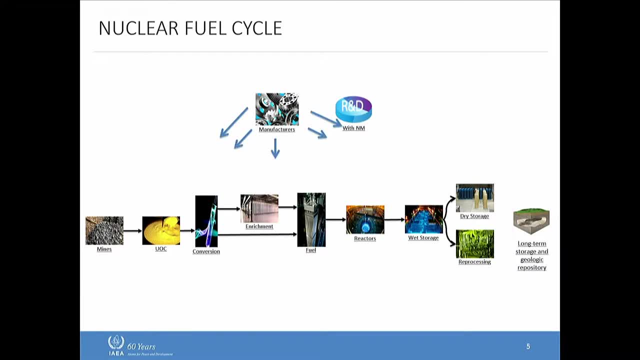 you've got to know how to make control drive mechanisms, reactor coolant pumps. This is important from a safeguards standpoint because it tells a lot about the capability of the state And I'll get into that in detail later. And the other thing- and this is a little bit worrisome from a safeguard standpoint- 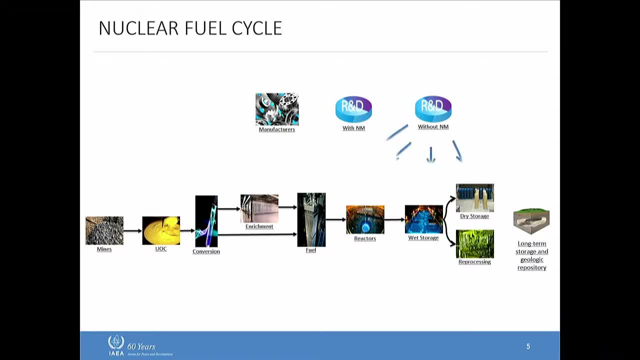 is, you can have R&D without nuclear material They don't have. the state is not obligated to tell us if they're doing research with centrifuges, with hot cells, as long as they don't introduce nuclear material. The minute a gram of nuclear material enters the picture, that's a facility with nuclear 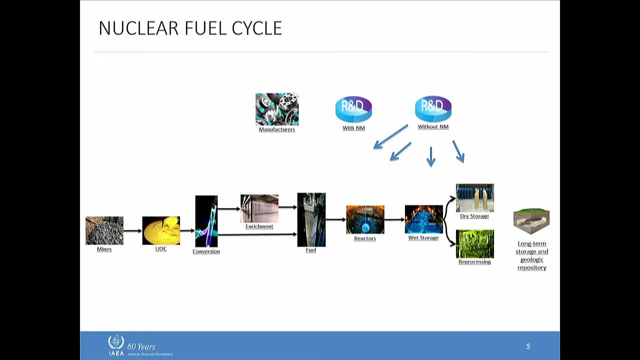 material in it and they have to report that. But if they're just, they're not. if there's no nuclear material in the facility they could test, let's say it's a if they're testing with centrifuges, a small pilot plant. 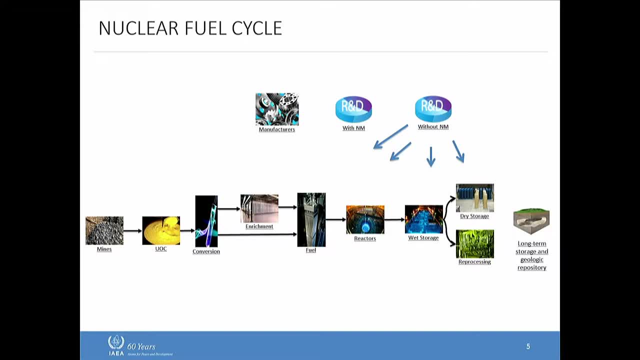 they could use a surrogate gas instead of UF6. And most states will have what we call a location outside facility. This tends to be like a small, like a hospital or a university, where they might have reagents. a lot of times it's depleted uranium or natural uranium for shielding of radioisotopes things. 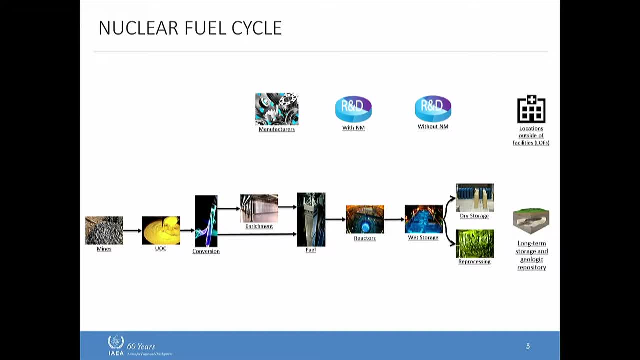 like that. It might be a plutonium source, but in gram levels and they're allowed to have that And usually it's in. we don't call it a facility, we call it location outside of a facility. We refer to it as lofts. 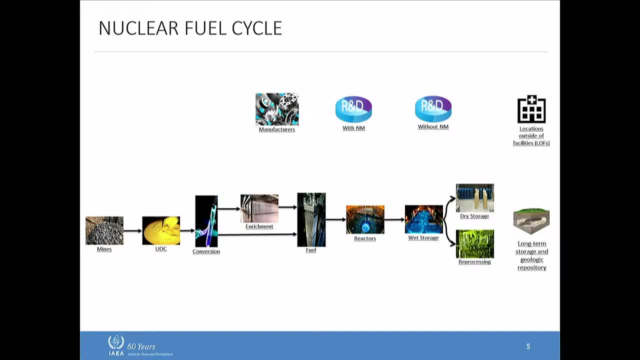 So this is a pretty. I have to admit this is a pretty extensive nuclear fuel cycle. But just to show you what's under safeguards, what they're again obligated to report and we have the right to verify under a comprehensive 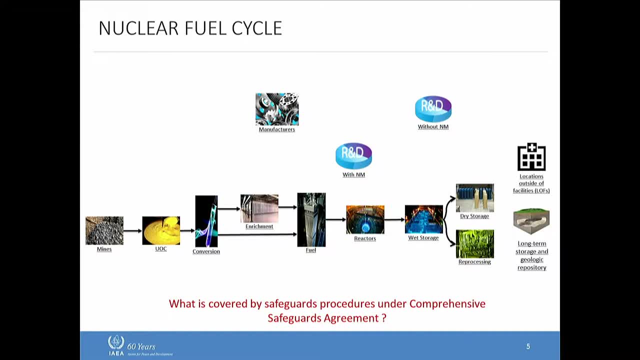 safeguards agreement and I think you'll hear more about this tomorrow. Usually the legal aspects is covered before this, so there's something called a INSERC 153.. INSERC's just a bureaucratic name for a document at the IEA, but there's a 150,, 151,, 152, 153. 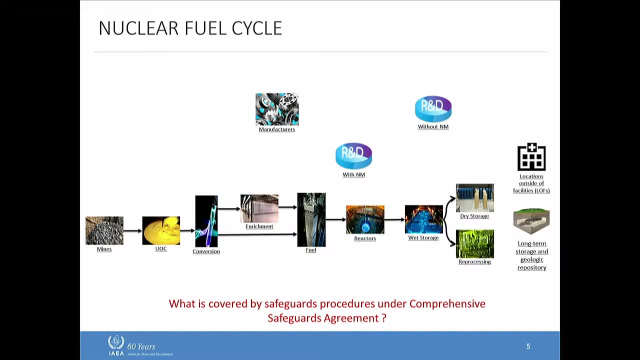 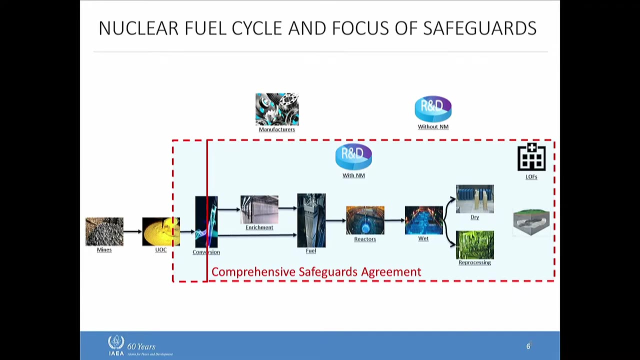 was the next number and that referred to comprehensive safeguards agreements And the lawyer from safeguards will talk about this in detail tomorrow. But under a comprehensive safeguards agreement, this is what is under safeguards. I mentioned that the starting point is here, Depending on the purity and how much purification equipment they have. 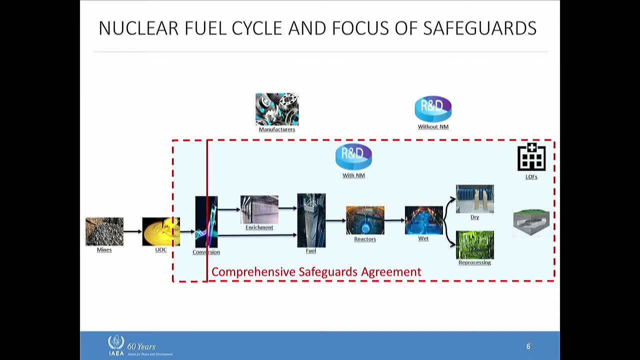 at the concentration plant. it might start earlier, But generally you can see that manufacturing is outside. I mentioned about the R&D without nuclear material. If it involves nuclear material, it's got to be in a facility or a loft. It's got to be under safeguards. 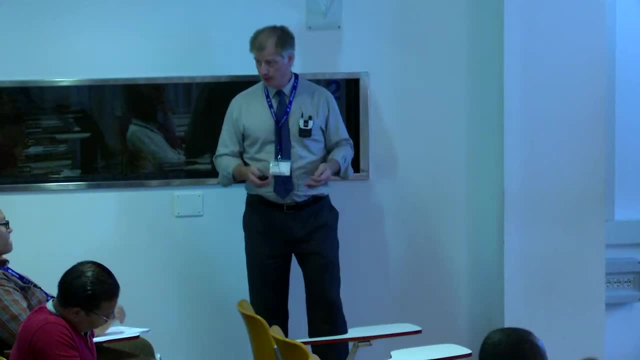 But, as you can see, the comprehensive safeguards agreement which was part of the NPT, which came out in the mid-'70s- I'm sorry, the early-'70s- the NPT and then these CSA agreements started coming out in the mid-'70s. 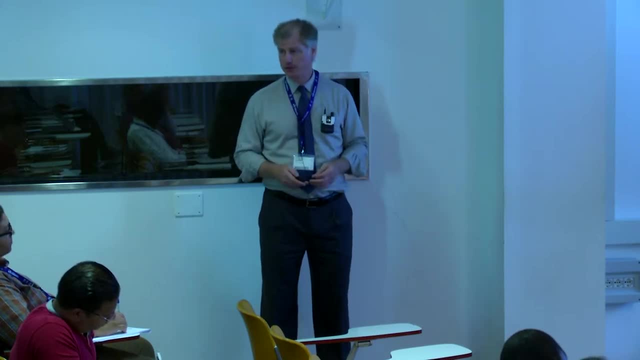 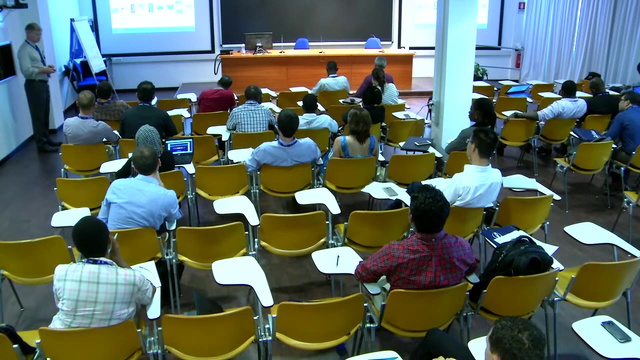 wasn't so comprehensive because it didn't cover everything. This was found to be a weakness in the early-'90s- actually late-'80s, early-'90s- with case studies like Iraq and later with Libya and other countries. So after that, in the mid-'90s, the agency came up with what they referred to as the 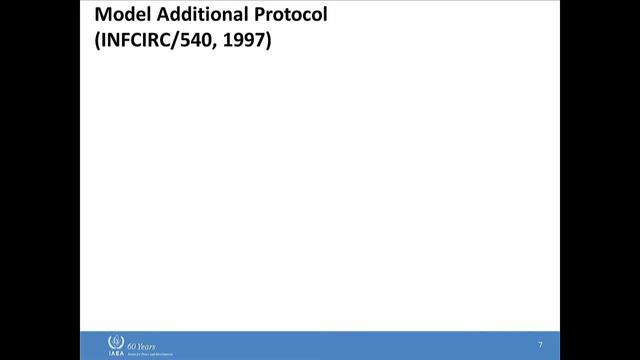 additional protocol. The number for this was INSIRC 540. And under 540, it basically gave the agency increased information and increased access. So the main features are: we got access. We got access to mining, not in a detailed nuclear material accountancy way. 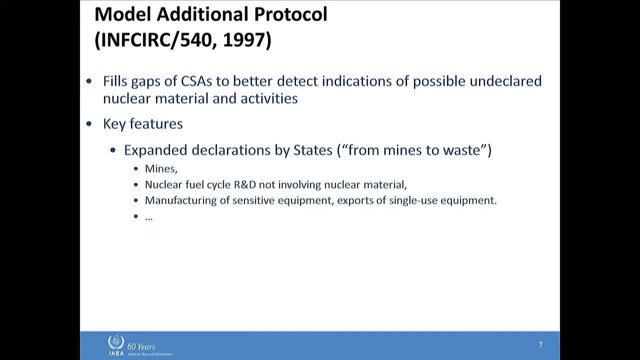 but in general production levels at the mine. So we have information about a state's mining capability. Before they didn't have to tell us about mining. Now they'd have to tell us that they're actively producing uranium. Mentioned the nuclear fuel cycle, R&D not involving nuclear material. 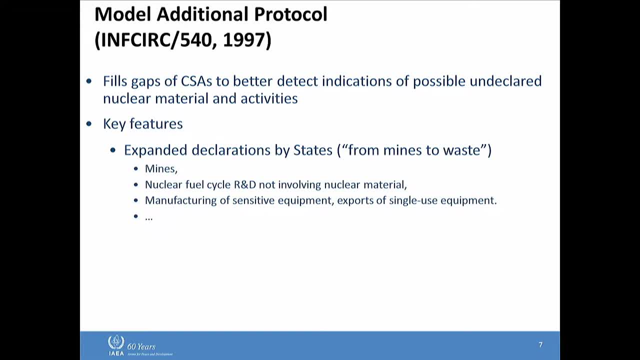 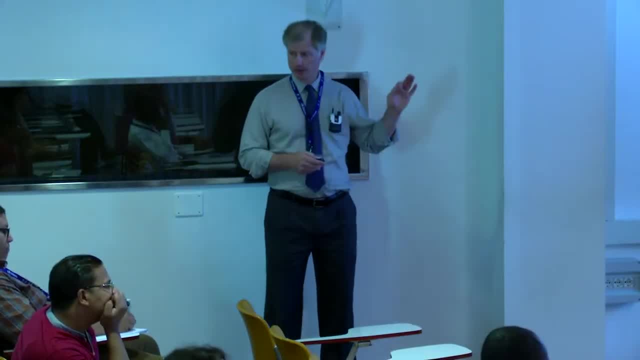 They have to declare that and tell us about it. And also if they're manufacturing sensitive equipment- So if they're manufacturing hot cells or rotors for gas centrifuges, that has to be- the agency has to be notified of that- What we call additional protocol declarations- even if there's no nuclear material involved. 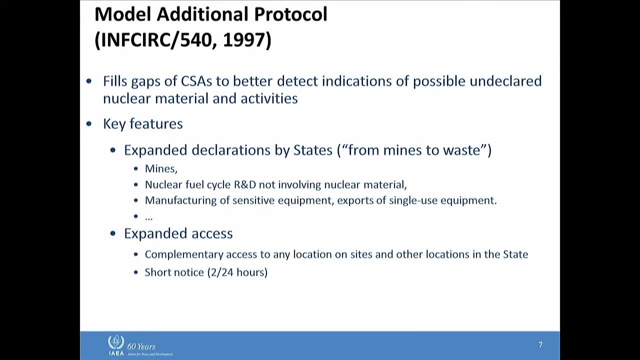 And there's other things like 10-year plans. They have to tell us their- basically their- forecast of where their fuel cycle is going in the next 10 years. It also gave us increased access, So we have short notice Depends on the type of what we call complementary access. 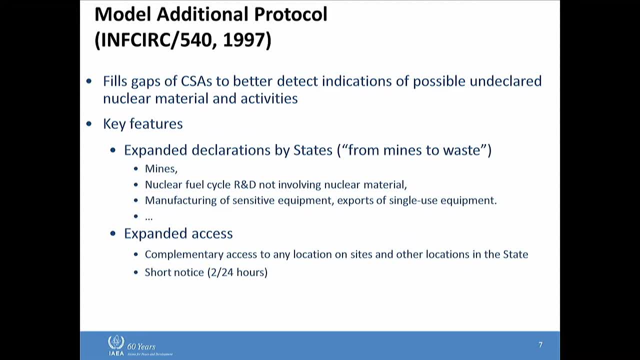 So it's not technically inspection but it helps the agency go to places that other than facilities, because we have access to facilities. That's where we normally verify nuclear material. But now we're checking There might be undeclared locations. We have information that possibly there's undeclared nuclear material activities. 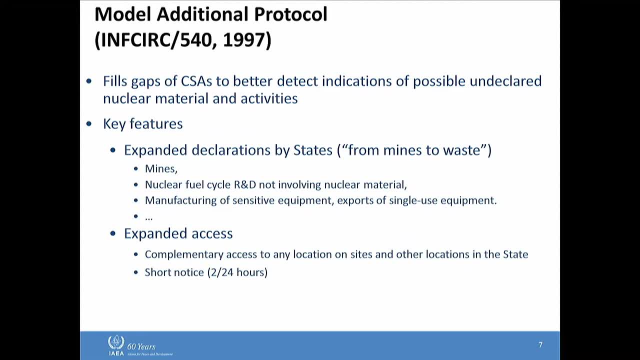 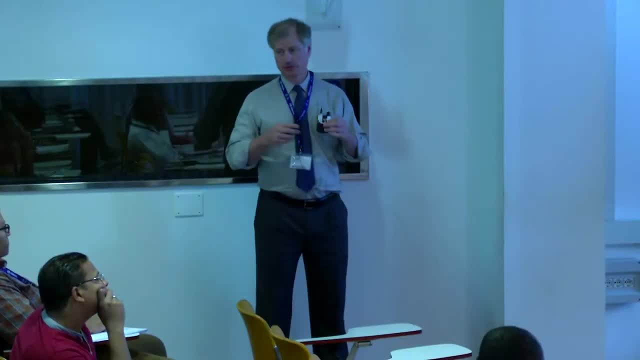 Or at least there's an inconsistency. We're trying to resolve it. We might go to that site And a complementary access allows us to go there legally, Because there's no facility. Inspections are for facilities. Complementary access is for locations where there are no facilities. 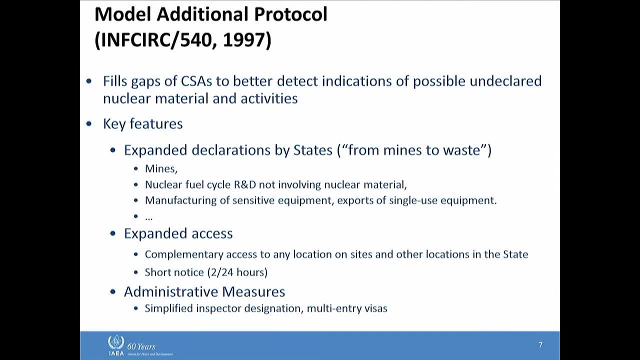 And again I mentioned the short notice. It also gave us some administrative measures because usually when we go to a state as an inspector, you have to get a visa from the state typically. Well, if you have to get a visa, you're tipping the state. 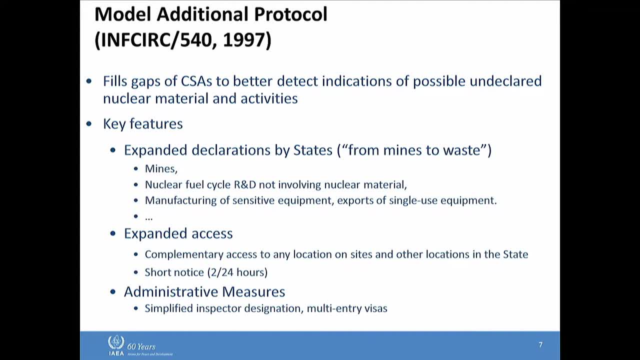 Often you're going to be going to the state, So under the additional protocol states are required to issue multiple entry visas. So usually it's good for a year, So you don't have to keep requesting a visa to go to the state. 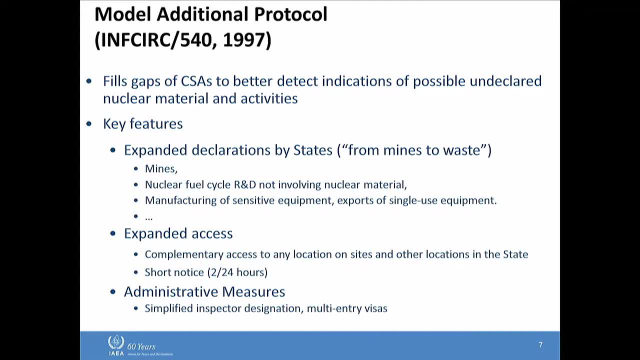 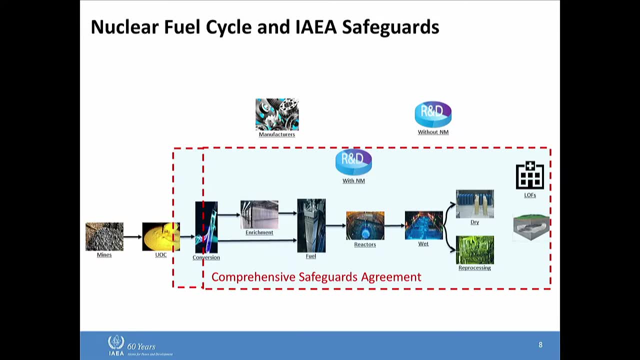 So that also streamlines the whole administrative process. It makes the complementary access more effective. So that was the original comprehensive safeguards agreement under 153.. Under 540, what we call the additional protocol, that increased information, it increased access. You can see it's more all-encompassing of the entire nuclear fuel cycle. 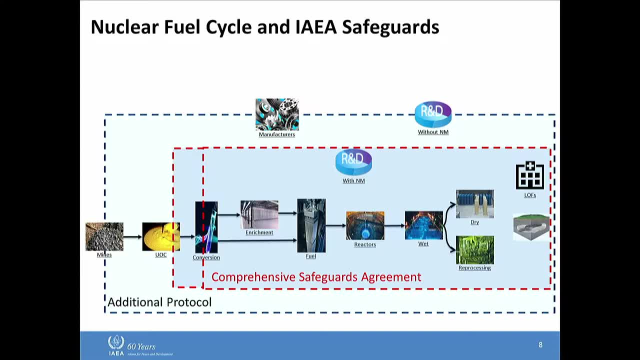 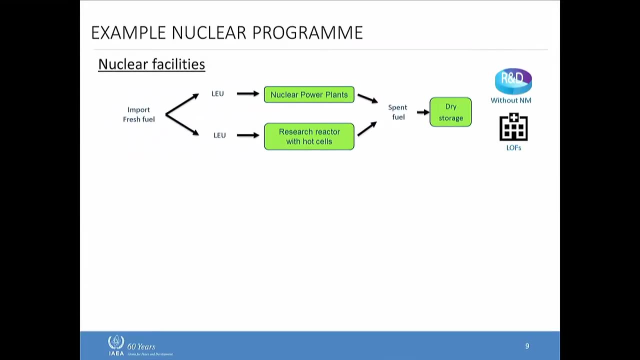 This is important- I'll get into this later- because now we have a more comprehensive understanding of the nuclear fuel cycle, the capabilities the state has and the potential those capabilities can offer the state in terms of if they decided to proliferate. So I want to go over and introduce a quick nuclear fuel cycle. 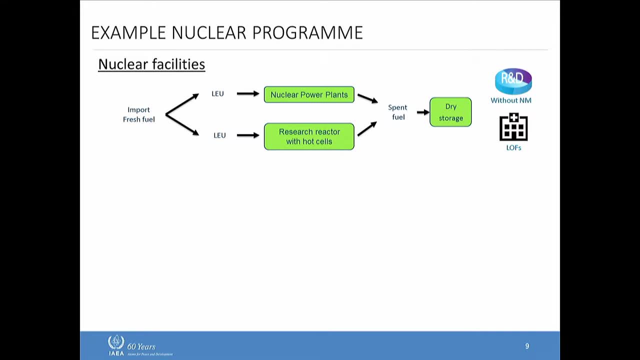 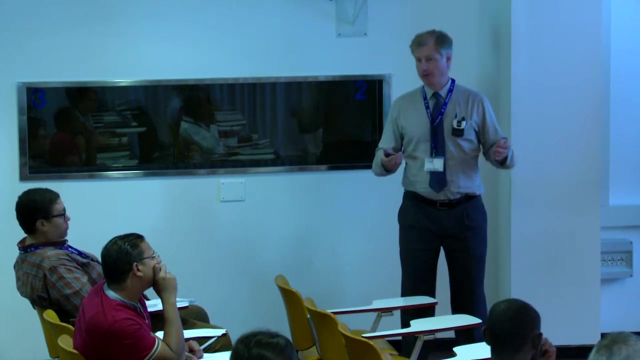 This is a fairly common one. Yes, yes, When you put it along the line, it's along the border And you can see the. And what they're obligated to report is the production of uranium in ton quantities, So they don't have to say how much ore they produced, but how much uranium was produced. 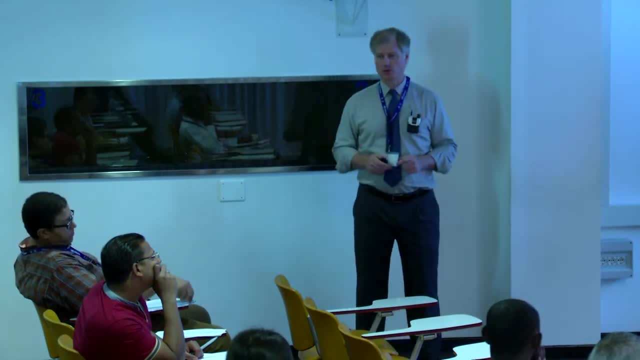 from that mine. Or it could be if it's a copper mine and they're concentrating uranium as a byproduct. you have to tell us about that uranium production. Basically, it's not just a mine. It could be from states, it could be from seawater. 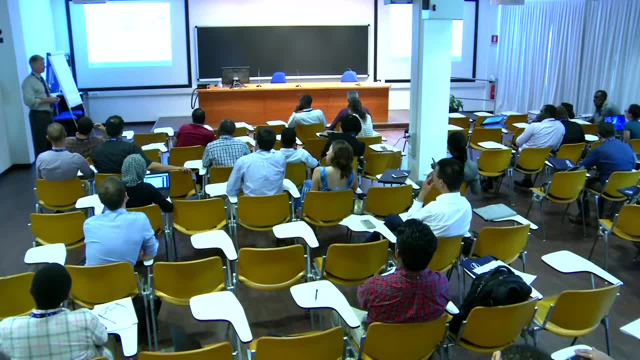 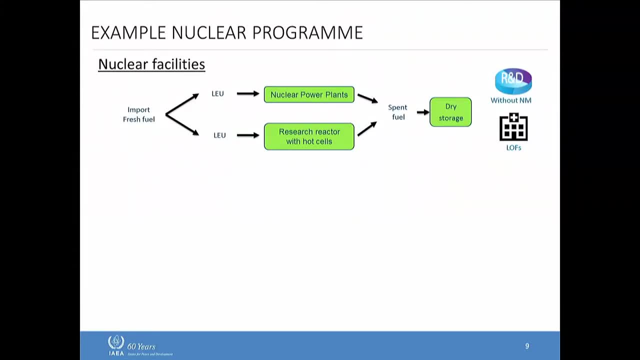 But the most common ones now are mining or byproducts of mining. So here's an example of nuclear fuel cycle. Let's say, just for illustration, this state imports its fresh fuel. Part of it is LWR-type fuel. It goes to their power plants to make electricity. 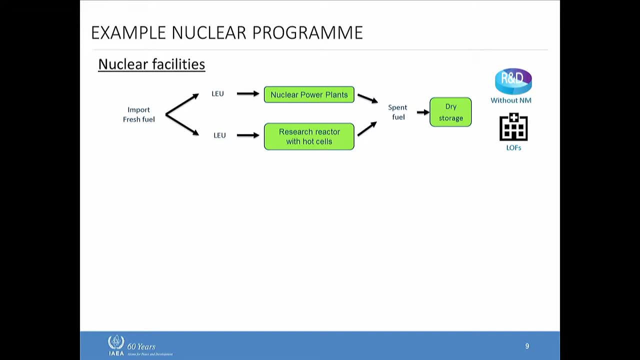 The other part is, let's say, MTR-type fuel plates And it goes to a research reactor that has hot cells. You heard about that, We talked about that earlier today And we'll say they're making medical isotopes. I think it looks like molybdenum-99 technetium-type operation. 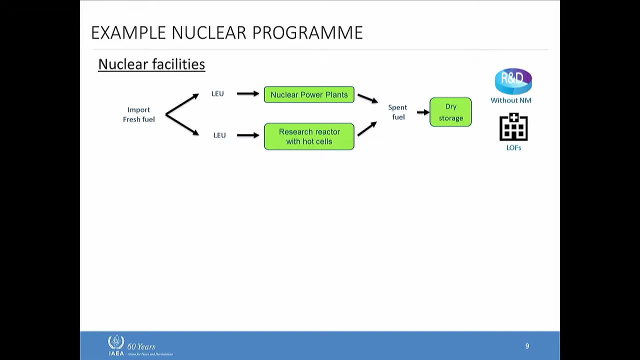 And maybe they do some training too. Once it's spent, it's been in a reactor for a few years or it's discharged from the research reactor, it goes to some sort of cooling, not as long or not as intense in a research. 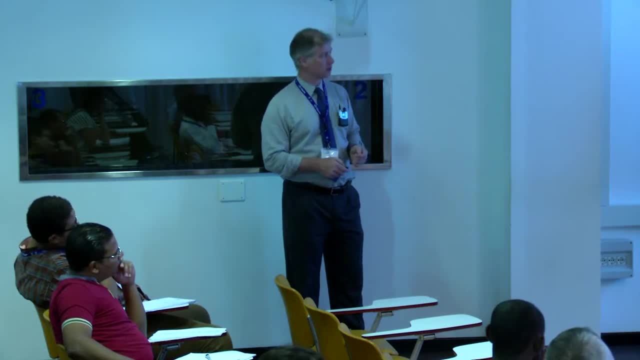 reactor, But for power plants they'd have to cool it And eventually, as I mentioned, they'll transfer it to dry storage. And let's say the state has some, let's say, a nuclear power plant, It's going to have to cool it. 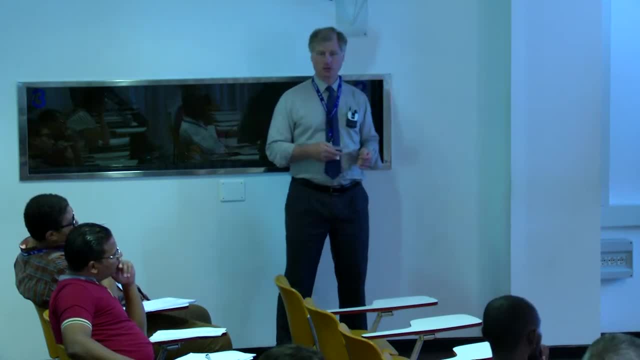 It's going to have to do some research without nuclear material- R&D related to the fuel cycle without a nuclear material- And they have a law. This is a pretty typical. I can think of a lot of states with this size nuclear fuel cycle. 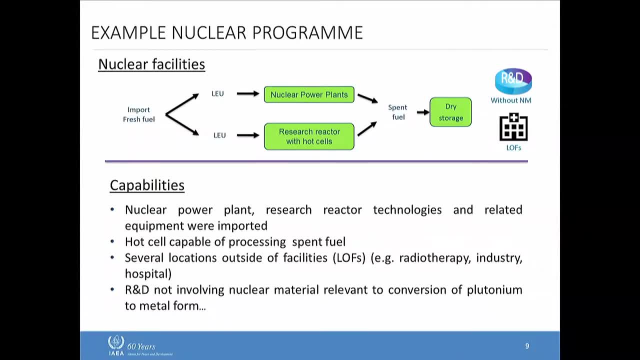 It's a medium-sized nuclear fuel cycle. So again, we want to understand the capabilities so we can assess those capabilities in terms of any proliferation risk, And I'll get into this as acquisition path analysis. So we'd highlight that from our understanding of the state. 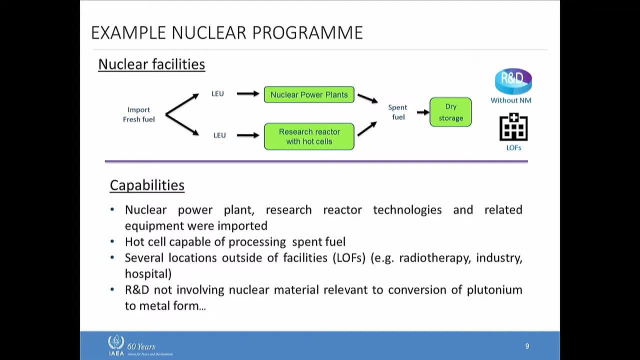 They have power plants, They have research reactor technology, And it was all imported. And that's kind of important Because they have a law. They have a law Because they've imported this know-how. They're a technology user, not a holder. 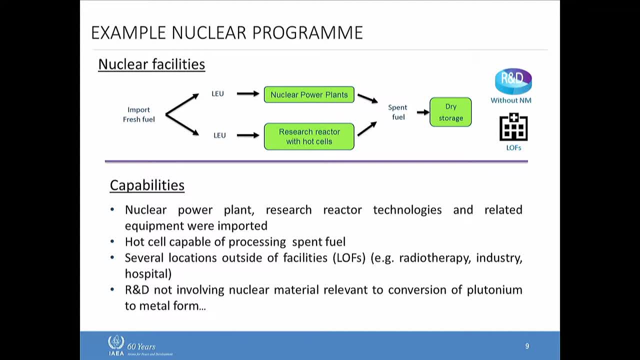 So they're receiving this technology, not supplying it. So it tells me something about their capabilities to replicate it if they wanted to. They have hot cells capable of processing spent fuel. Well, that tells me. these hot cells have got to be pretty large if they're going to take. 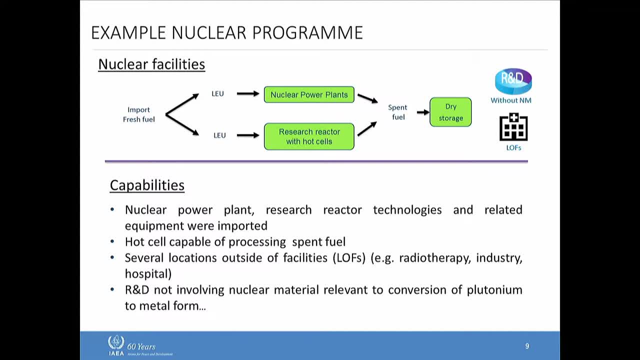 an LWR fuel assembly, But they could. I've seen some that are pretty long. Usually it's for pins post-radiation examination to test the pins, But they could have that So. So I'd like to remind that they have large hot cells. 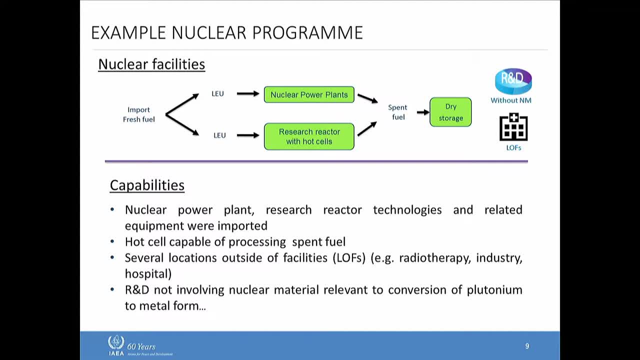 And they have some lofts, which is typical, And they have some R&D involving nuclear material relevant to the conversion of plutonium to metal form Sounds a little suspicious. Now, is the state allowed to do this? They can. They just have to declare it. 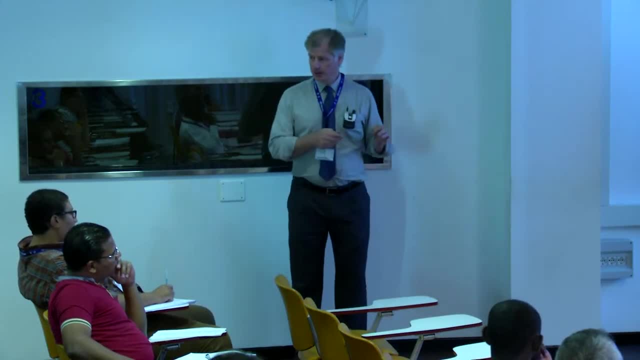 So the state has declared it. We understand it. The group at the agency that would look into this we call the state evaluation group. The country officer might be a little bit concerned about that, But it's OK, The state does it. We might want to follow through on it just to learn the extent of what's going on with. 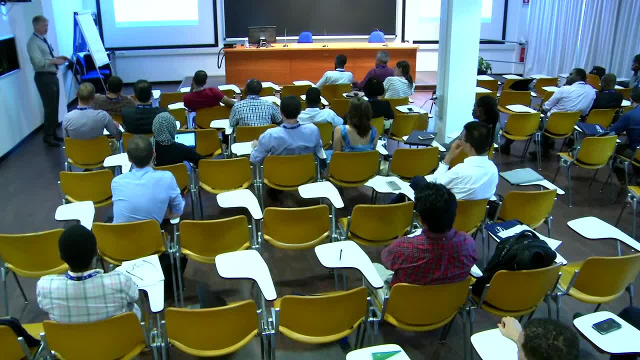 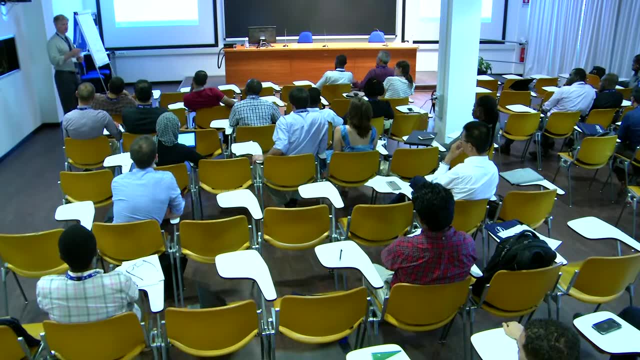 this R&D down here. It doesn't seem coherent with the nuclear fuel cycle. But I don't know, Maybe in their 10-year plan they have a future. Someone mentioned earlier, I think, fast-breeder reactors, or maybe they have some research reactor on the horizon that may use a PU-type fuel. 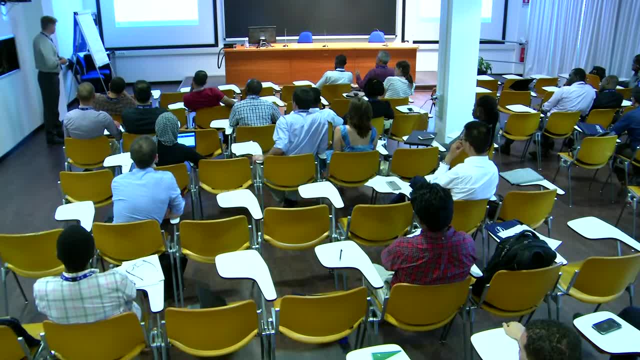 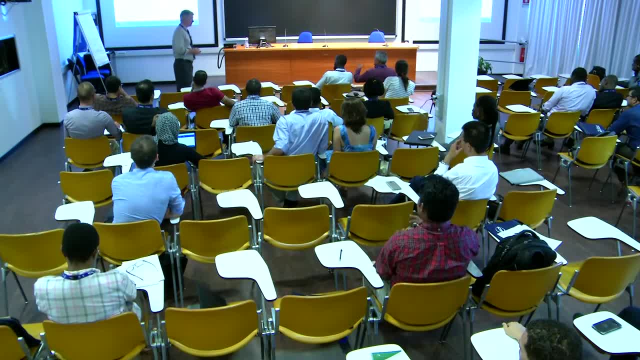 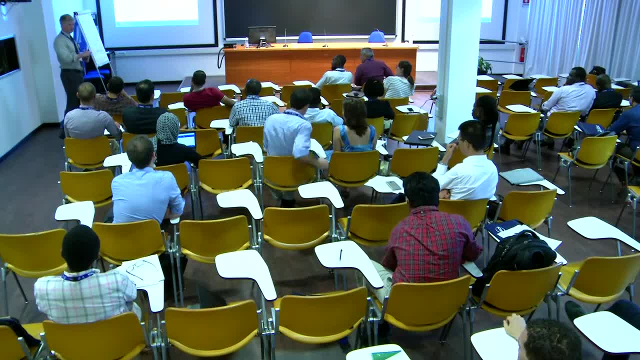 I'll get to that. So right now, this is just a peaceful fuel cycle that has to be safeguarded. All this is allowed. Is that what you're asking? what the safeguard aspect are. OK, I'll get into that and the measures we take. 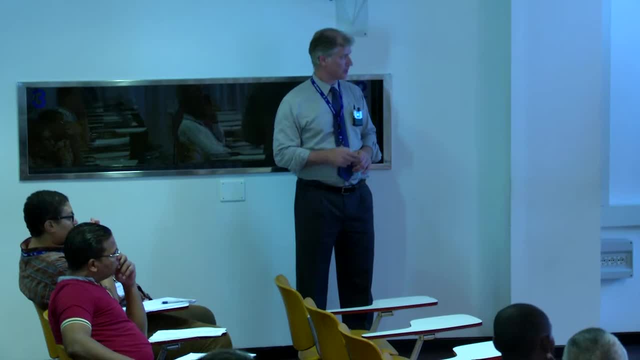 Just using this example so you can see a typical fuel cycle. This is very important. We have to know our legal basis, So we'll assume we have a comprehensive safeguards agreement and additional protocol enforce. You'll learn more about these tomorrow So you have full information, full access about this state. 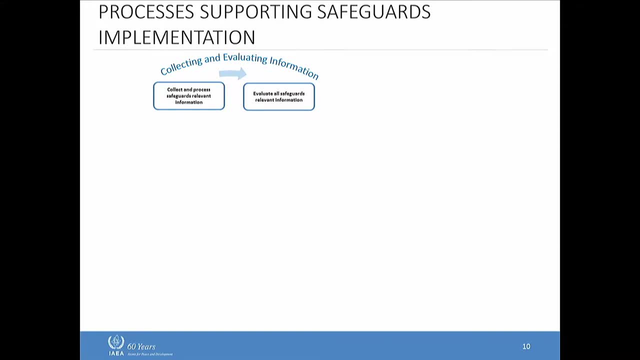 So I just want to back up a little bit. So we have four basic core processes at the IEA and the Safeguards Department. First we have what we call collecting and evaluating information. We call this state evaluation. We're always constantly looking at information that's coming in. 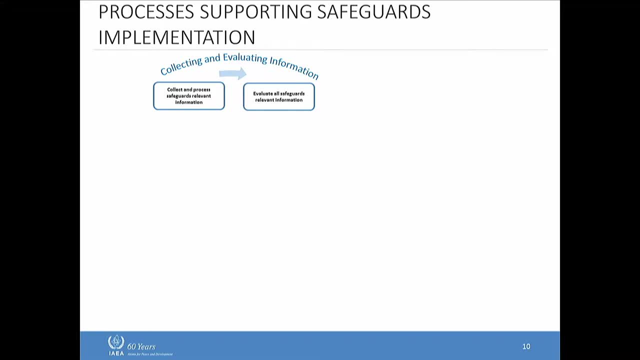 and doing what we call consistency analysis to make sure everything's adding up, If there's something we expect, and then we observe something and we make sure it makes sense. After that, once we have this solid understanding of the state, we get into what we call action path analysis. 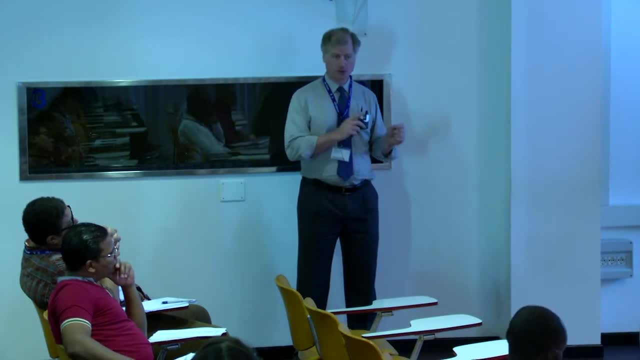 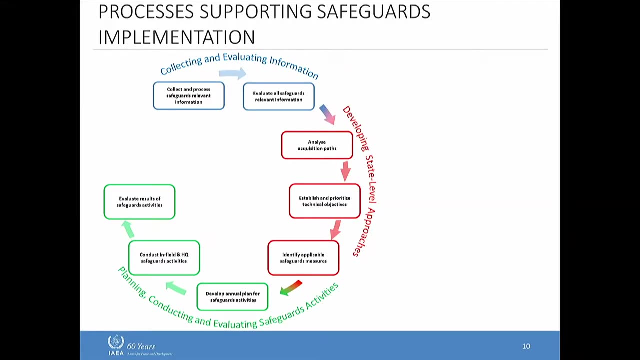 and we develop state-level approaches. This is where we identify the measures to cover those that cover the field cycle And then we actually conduct activities in the field. Inspectors will go on the field, Analysts at headquarters will simulate and synthesize information. 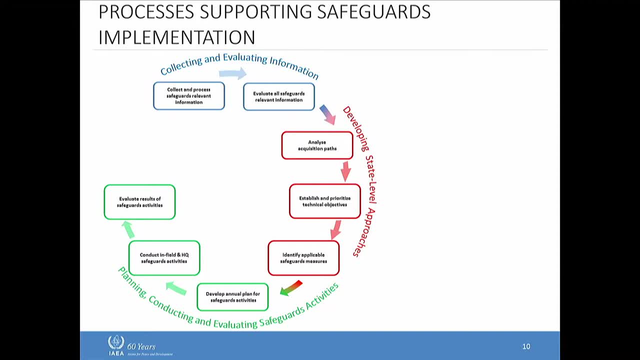 and analyze information And we'll look at the results of that And finally, we'll draw conclusions based on that, And there could be issues that arise or inconsistencies. We have to resolve those. So there's always a little bit of a framework. 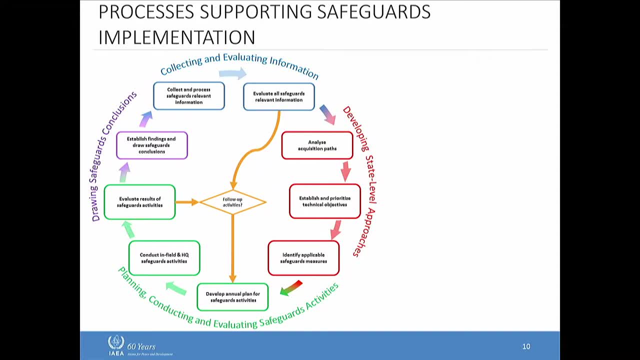 of feedback We call this. if it's minor, it's generally inconsistency. If it gets a little more serious, we refer to it as a safeguards anomaly. It has to be resolved, Otherwise it could impair the conclusion for the state. 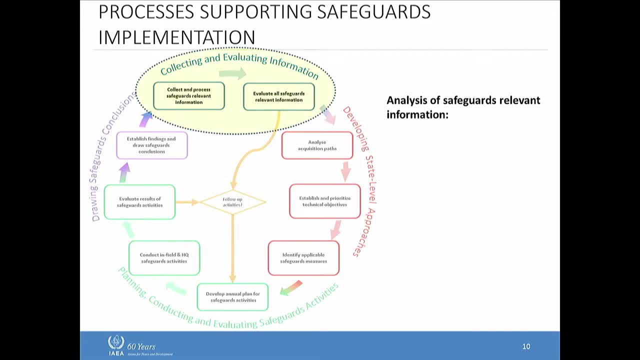 the final safeguards conclusion. So let's focus on this top part where we collect and evaluate information. Again, it's to get a firm understanding of the state, so we can do rock-solid consistency analysis, So we consolidate all relevant information We'll get into the various sources. 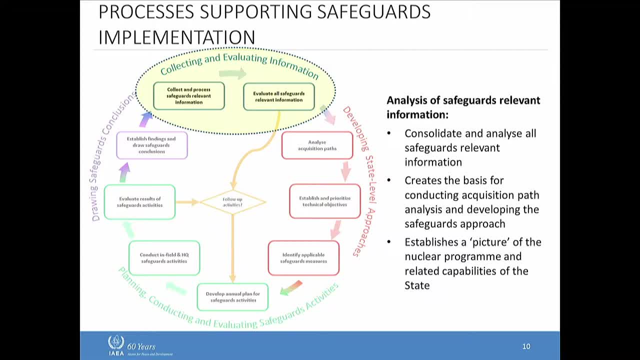 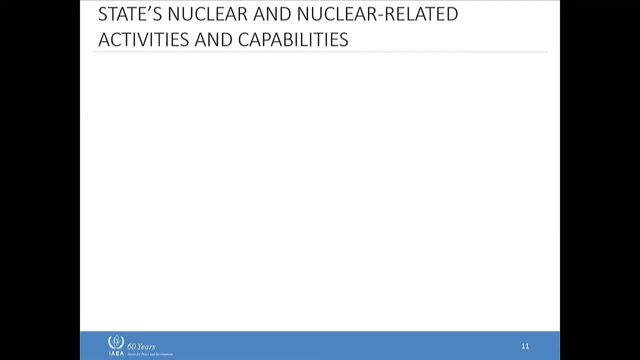 This helps to form the basis so we can do an informed acquisition path analysis- because we have to make technical judgments in that analysis- and establishes a profile or a picture of the state's nuclear fuel cycle. So there's the state and there's the IEA. 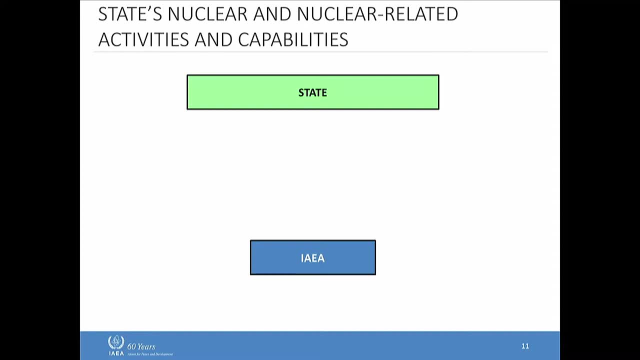 IEA is always blue. I'm not sure why. So there's information that comes in from the state that they're obligated to provide and supply to the agency, And I'll go into the various reports they have to submit. But I just want to highlight: is this information the truth? 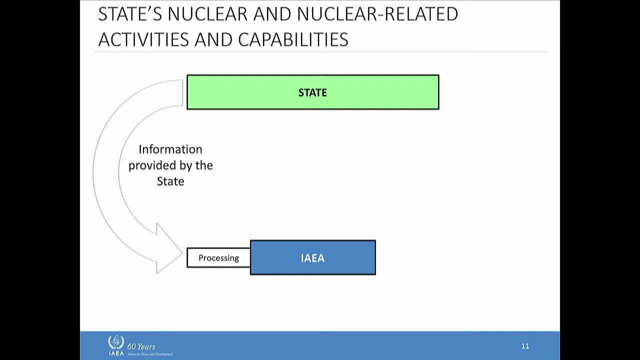 Is it the whole truth? Well, I hope so. I hope the state is honest and they're declaring all their activities and all their new material. But if they have a clandestine program, they're probably not going to tell us about it. 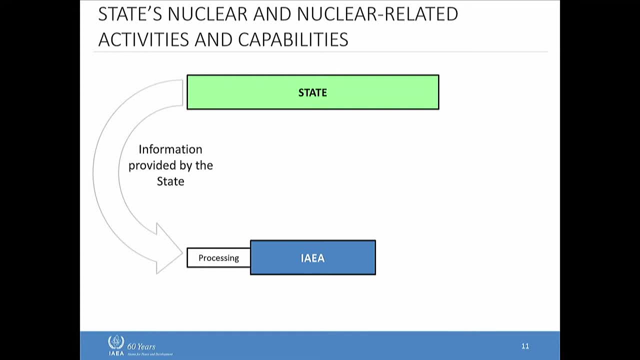 So we just have to take it with a grain of salt. Thank you, the state, for providing lots of information, But we also have to check that information. So the IEA conducts its own activities. They take measurements, We have containment surveillance. 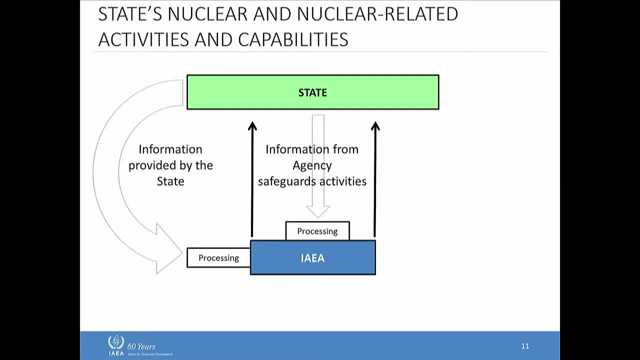 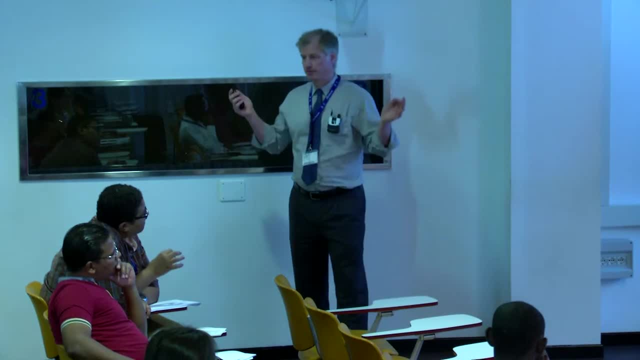 I'll go into all this in detail And that information comes back and we check it against what the state has told us. So the example state that I gave you the imported fresh fuel. let's say they import 40 assemblies for their power plant. 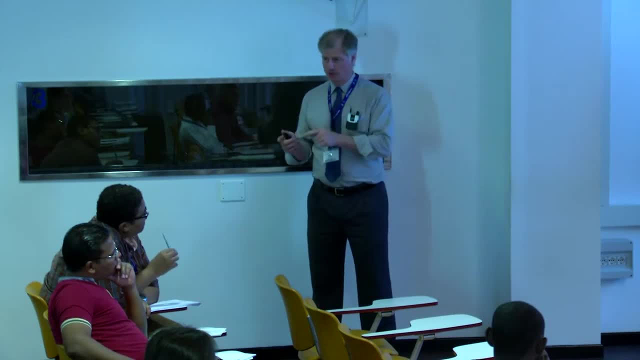 to refuel Unit 1,, let's say, The state that exported those told the agency we sent 40 assemblies. The state that received it is obligated to tell us they received 40. But we would know 40 new assemblies are in this country. 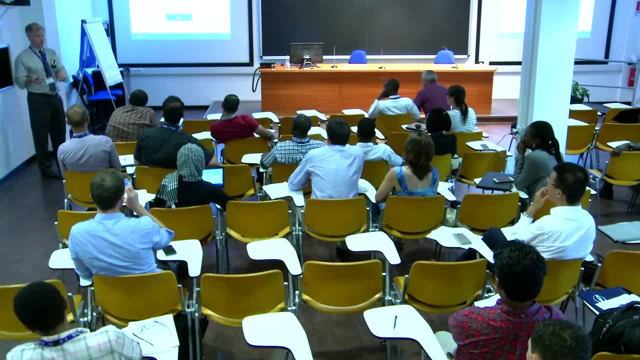 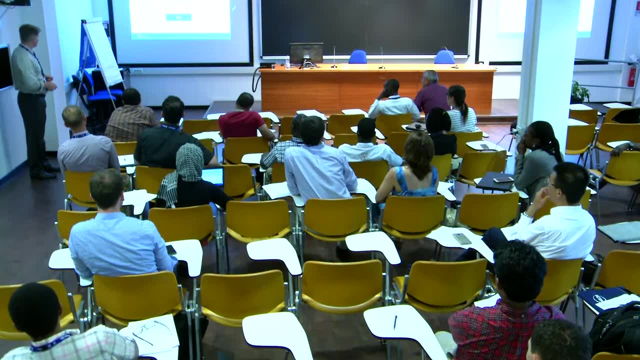 So next time we go to an inspection to that facility, we know there should be 40 new fresh fuel assemblies and we can verify those, So we're always corroborating and comparing this information that we receive. Hopefully this is the truth. 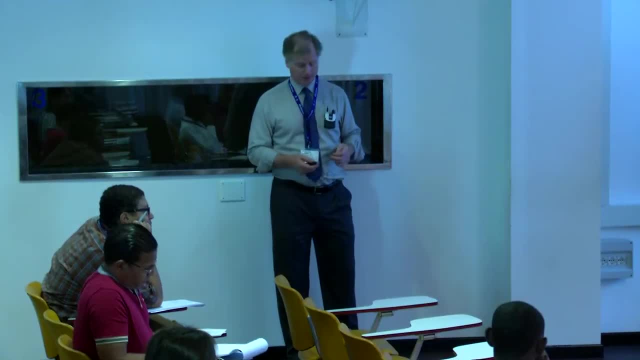 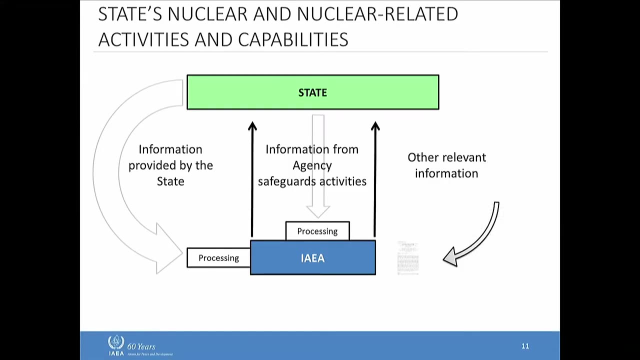 Our instruments are calibrated, The inspectors are trained well in order to compare it to this information. And there's another source- I'll just refer to this as sort of other- or the public domain. There's information that's in open sources. It could be in trade journals, newspapers. 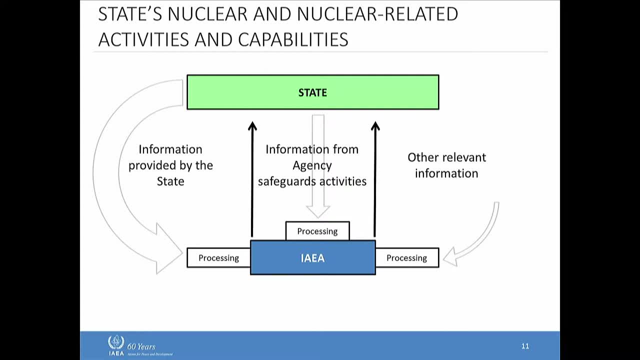 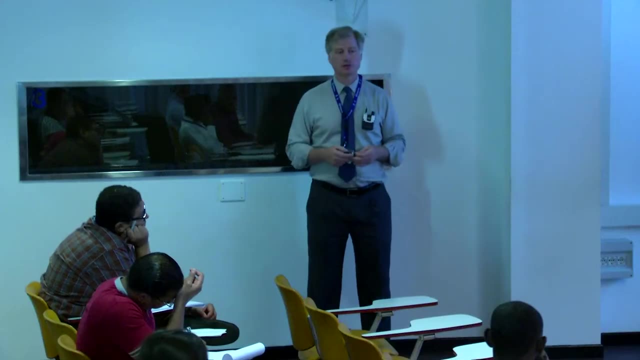 Yeah, And I'll get into it. But what I mean here is this is things like physical inventory listings, inventory change reports, detailed reports for the nuclear material in their state at their facilities. That's also the additional protocol declaration. So if they're doing mining, it's a report related to their mining production. 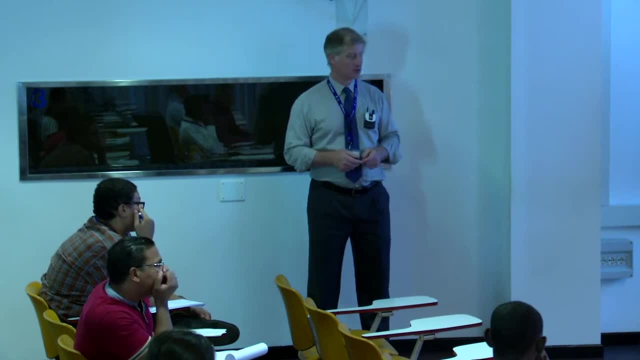 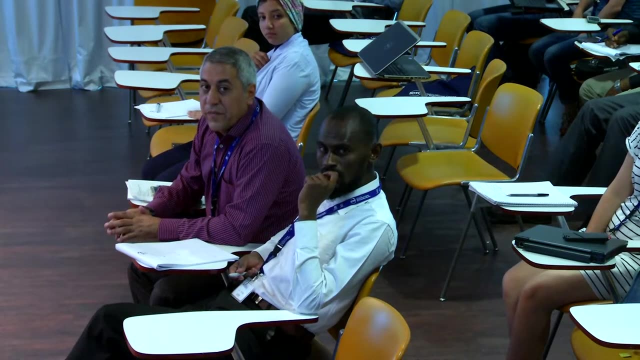 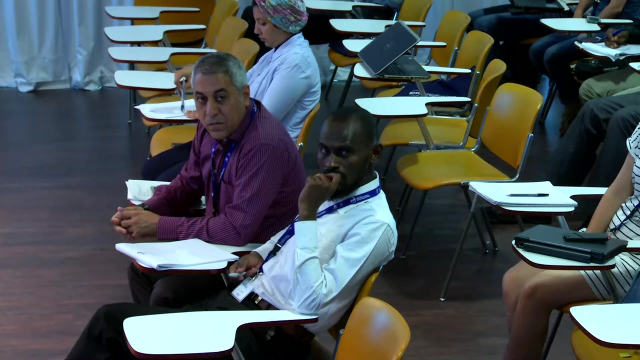 articles that they prepare related to their mining production. So that's safeguards- information provided by the state. Yeah, it's just safeguards And this whole thing is on safeguards- relevant information If they tell us things like: well, we're going to improve the health physics department. 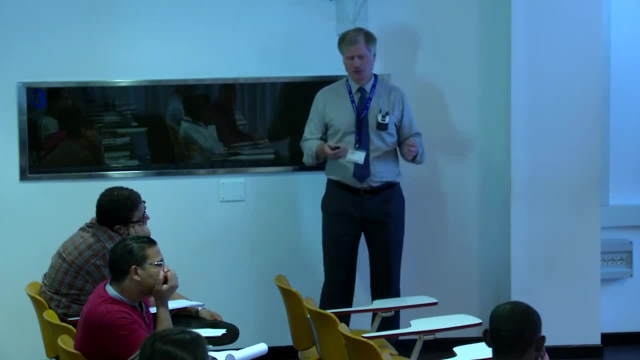 at one of the facilities. it's interesting information. OK, it's needed. It's important to have trained health physics staff, But it may not be entirely safeguards relevant, So it may be less of a concern for us. We're just aware of it. 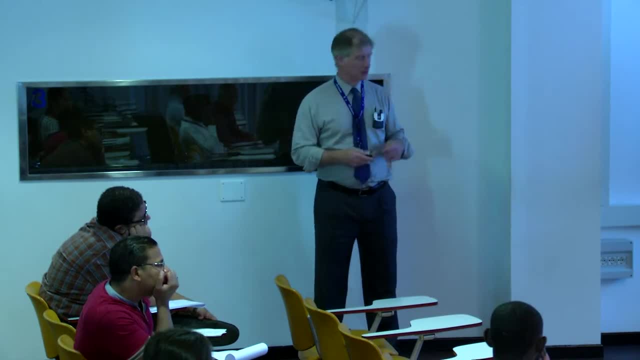 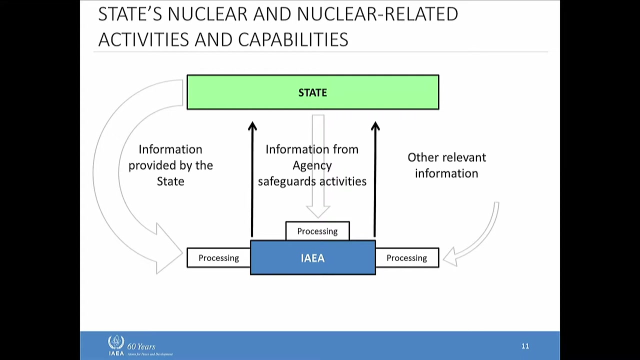 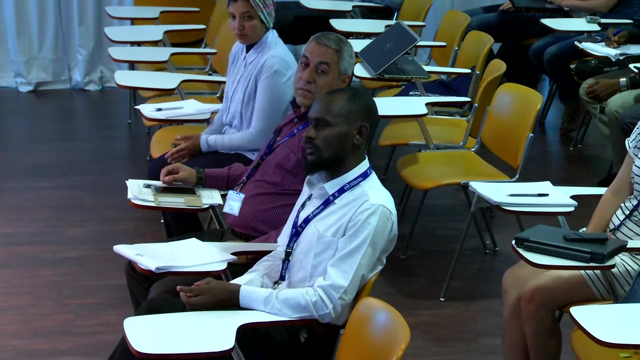 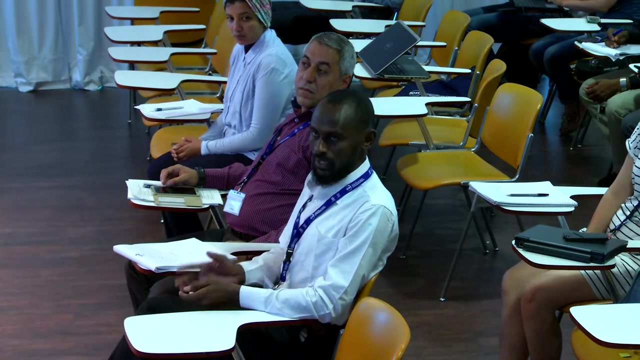 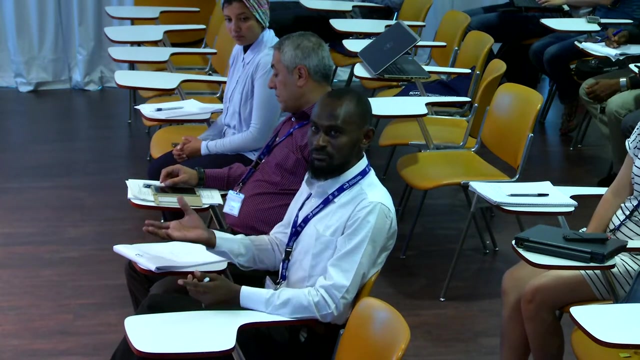 No, you read about it, but it may not influence anything. So I'm talking mainly about safeguards, relevant information that might impact the conclusions for the state. So I think that, yeah, Yeah, the state, yeah, State's responsible. Ultimately, the state is responsible. 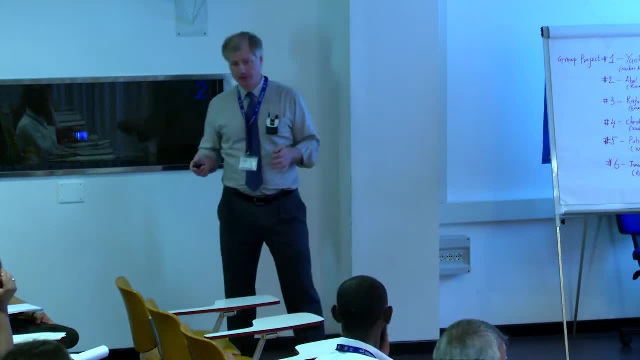 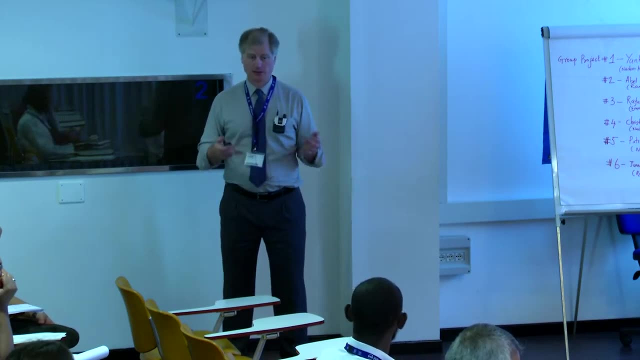 I think you mean like the operator is operating a plant. Some places, some states, have more authority or autonomy than other places, But in the end- and their legal agreement will require this- the state is responsible for the new material on their territory and their jurisdiction, under their control. 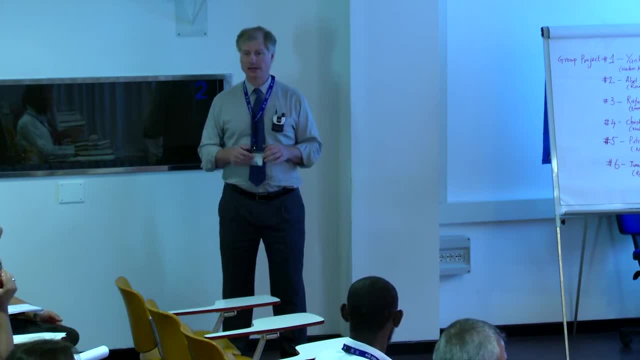 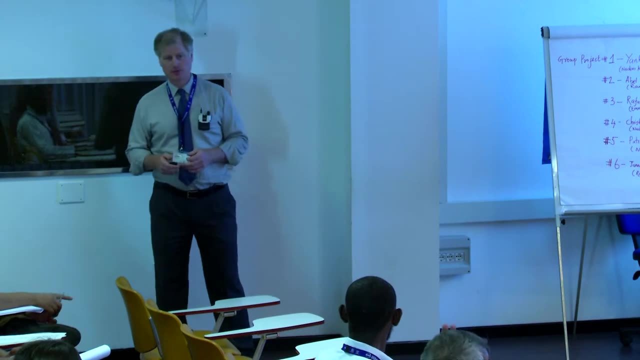 I forget the exact legal wording, but they're still responsible. Some states have a stronger- you know- legal authority, A stronger national inspectorate or national program national authority. We refer to it as an SSAC State System for Accounting and Control. 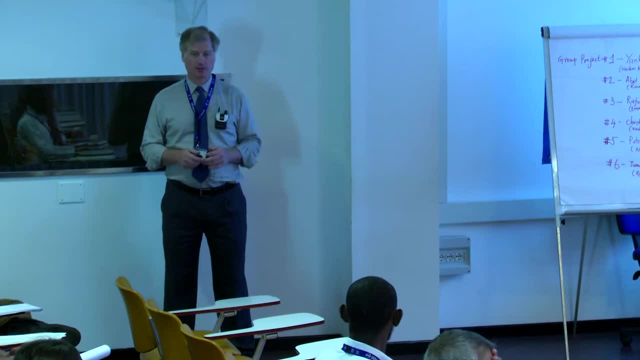 Some are stronger than others. Actually, some may not have one, It might just be a point of contact, But their fuel cycle may be very small. But if they have a reactor and they have facilities, they have to have a governing body that regulates that. 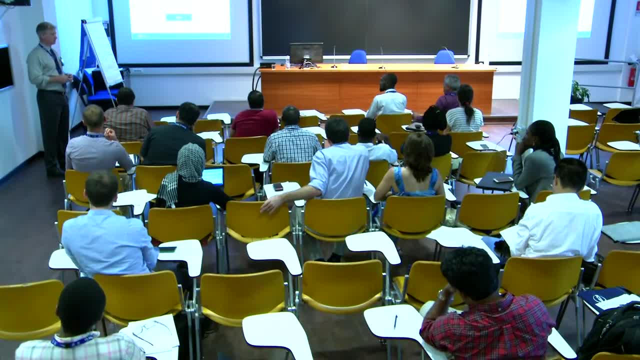 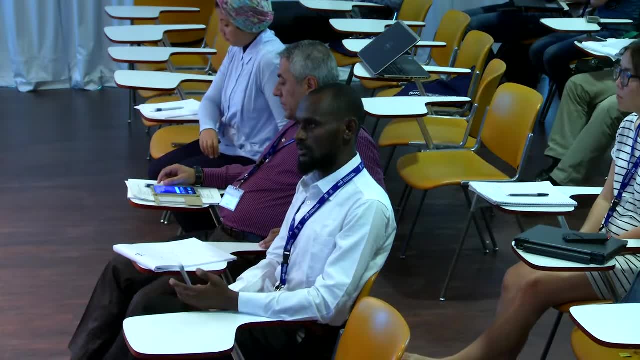 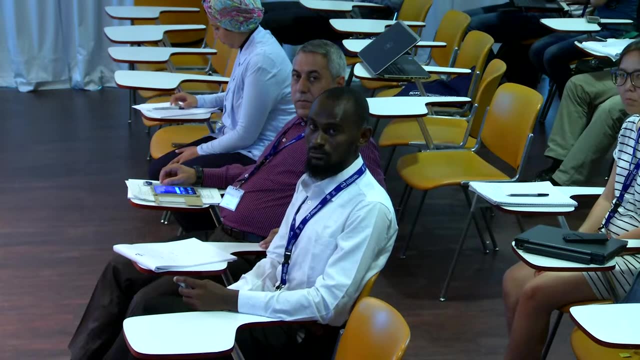 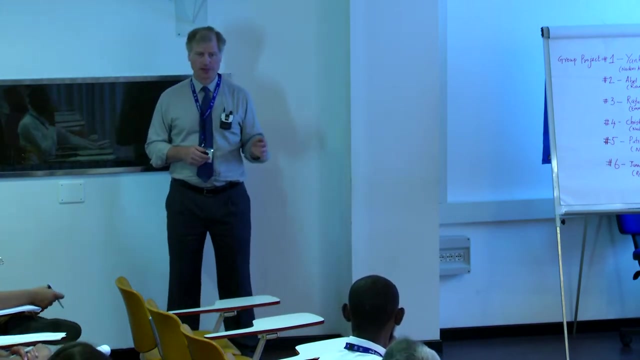 The things we heard about today: security, safety and for safeguards- Is that what you meant? Or Well, the nuclear material. they're obligated to tell the agency about it, down to gram levels for plutonium, For natural uranium and depleted uranium. it's kilogram levels. 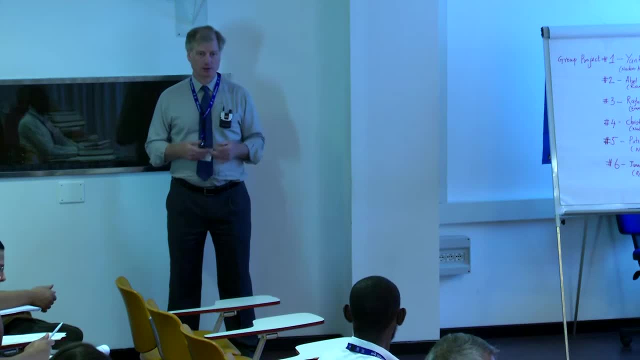 They have to tell us about it. They have to tell us where it is and the purpose. It's in a facility, It's in what we call a material balance area so we can account for it. It's a bit bureaucratic. It's a bit bureaucratic administratively, but we have to have that in order to 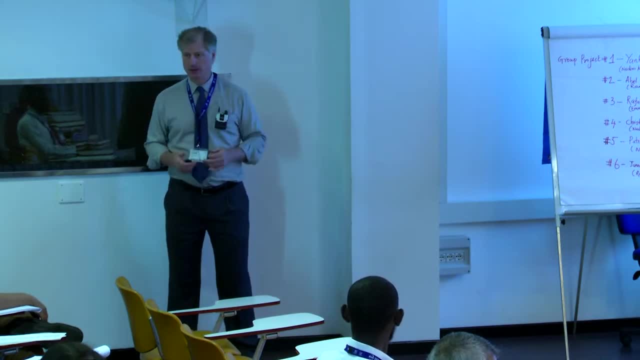 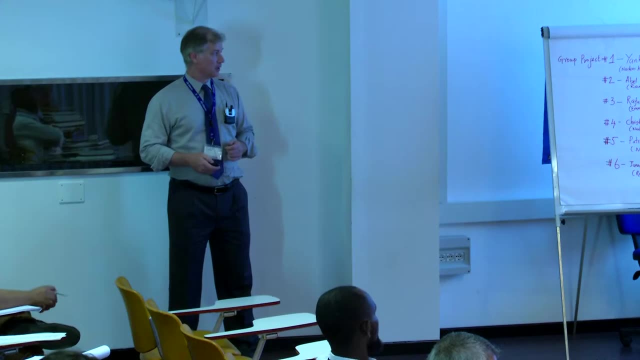 because nuclear material may come in and out of that material balance area at that facility, We always have to be able to, at any moment, know how much nuclear material is in that facility. So this information is again synthesized and sifted through by analysts. 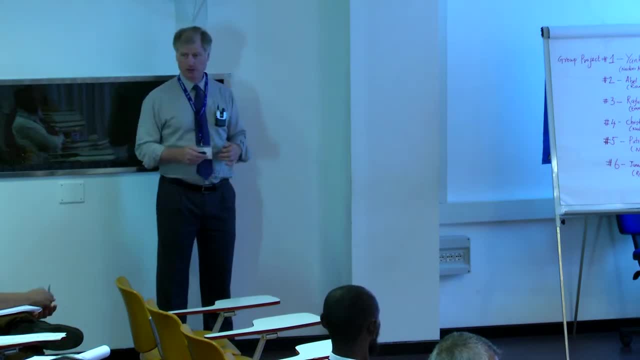 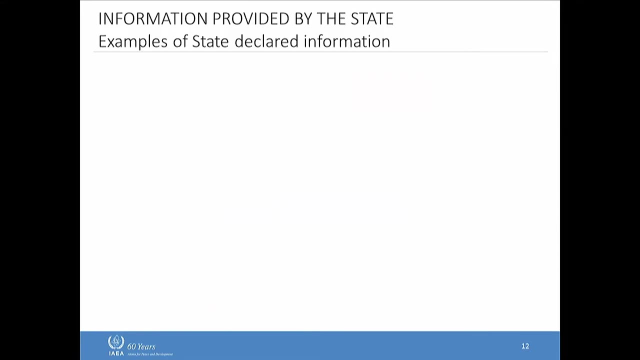 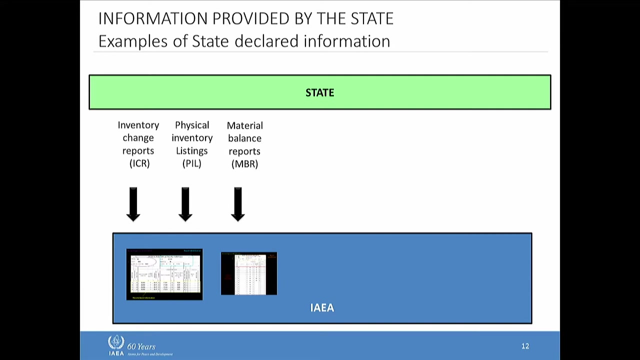 Again, the state evaluation group would look at it. It's put into what we call very secure servers digested, so there's a firm understanding of the state. Let's go over some examples of declared information by the state. I mentioned some of these already. 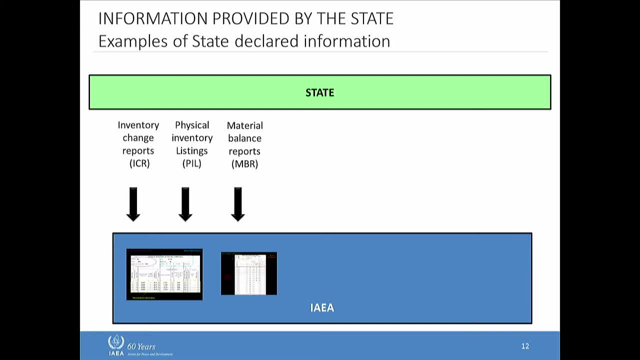 From a nuclear material accountancy standpoint. we have physical inventory listings. This is a list of how much material is in the facility, usually by item and weight. Any change to that inventory they have to submit an inventory change report, typically at the end of the month. 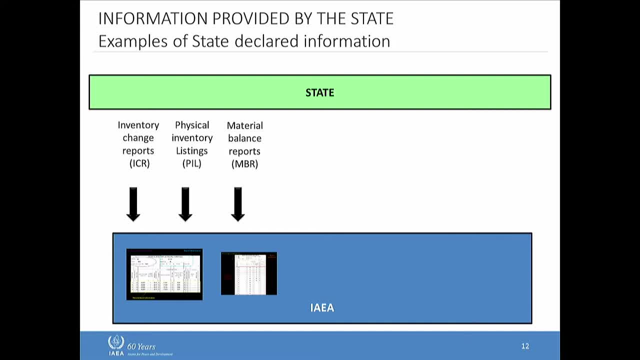 of when the inventory change occurred, so they know how much is going up. It could also be going down. It could be going down if they ship material out of their facility. It could be traveling through the nuclear fuel cycle in the country and we're just keeping an eye on it where it is in the facility. 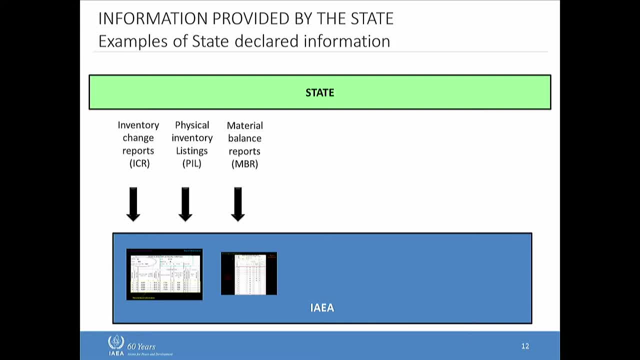 or it could be going out of the country. But again, at any one time we should know how much nuclear material is in the country or in a facility And a material balance report which is sort of an end-of-year. There's this material balance evaluation. that's done, but we need a material balance report. 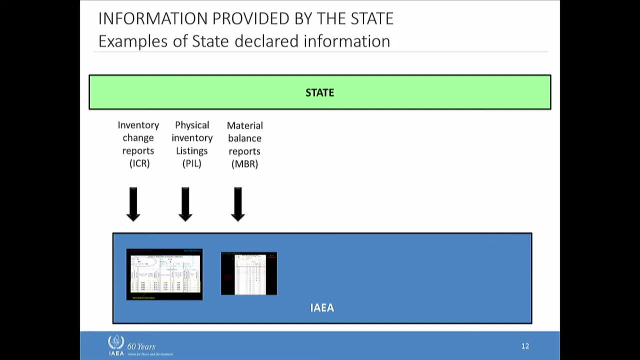 which tells us the initial inventory, any increases in inventory, any decreases, and then a verification inventory is done to confirm the closing of the inventory and close out the material balance evaluation. That's the report submitted. associated with that We also get design information, so it's not just about nuclear material. 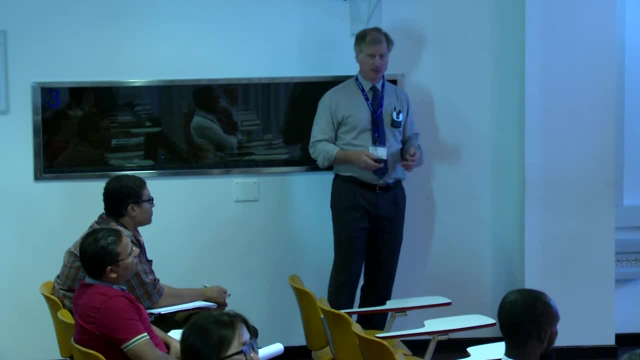 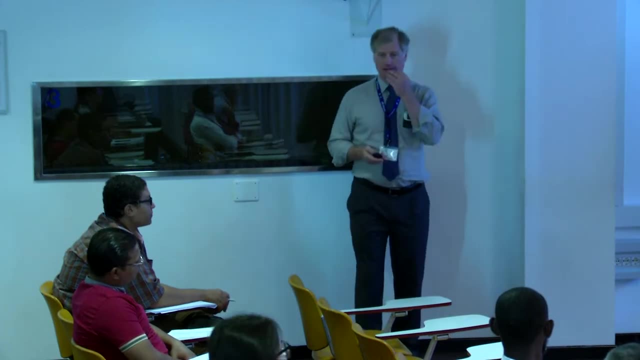 It's also how the facility is designed. It's not detailed design information, but it's safeguards. you know, relevant information, the rating of the research reactor. I think this morning someone mentioned- I'm not sure, I guess- Jordan is building a research reactor. 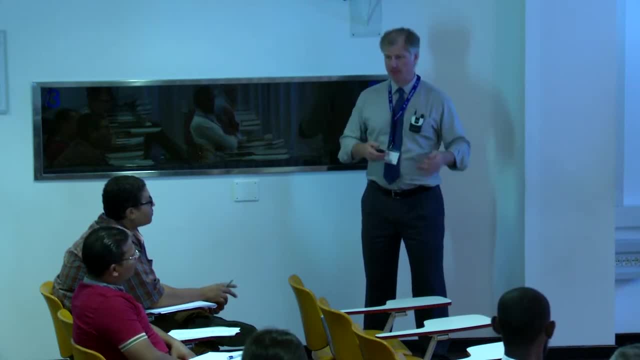 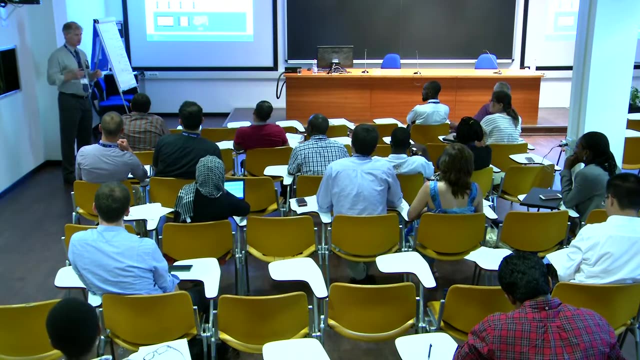 Now, from a safeguards standpoint, if it's 1,000 kilowatts, okay, they could. from a safeguards perspective, I tend to stay up nights I'm thinking about things, so I'm probably a little bit suspicious. but anyone that has a research reactor in any country, I would say 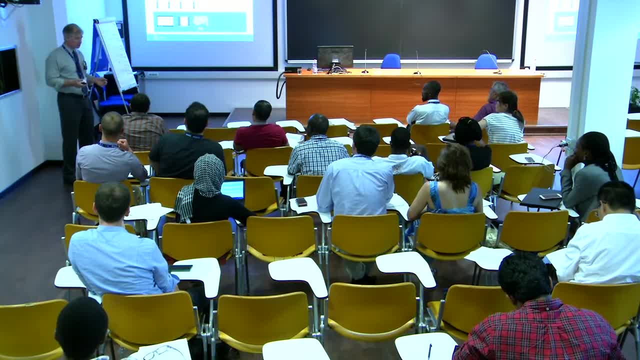 well, if they've got a 1,000-kilowatt reactor, they probably can't do too much with it in terms of misusing that reactor to produce plutonium- Maybe at an R&D level, but that would be it. If it's 5 megawatts, 10 megawatts- Now they're starting to produce some plutonium. I wouldn't call it appreciable quantities in a short time, but over several years they could produce SQs And if it gets up to 25,, 30, or 40,, 50 megawatt type reactors. 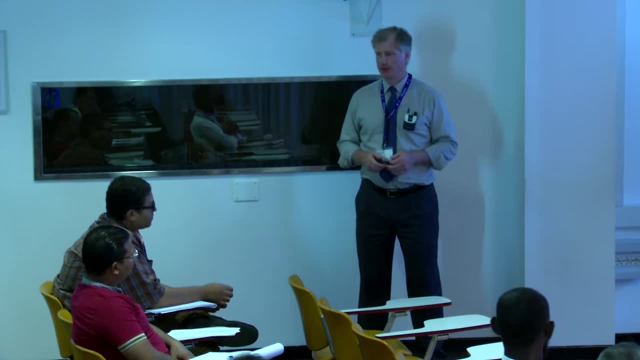 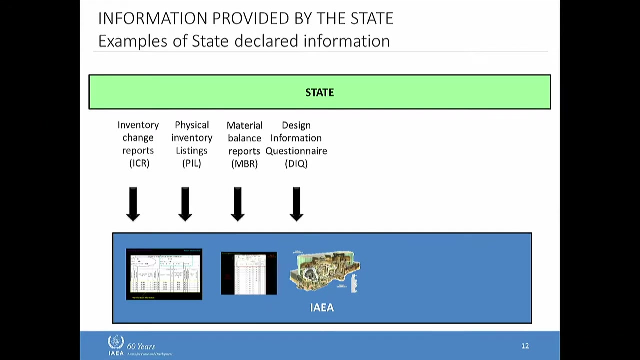 now they can produce enough plutonium Half a year a year for weapons usable in the material. So then in safeguards you might be more alerted to that reactor and that might get more attention from a design review standpoint. So we get this design information from the state. 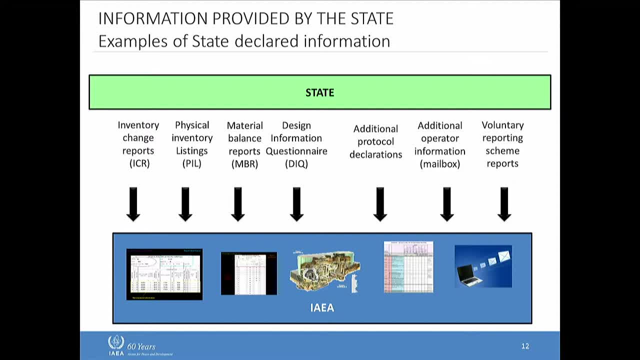 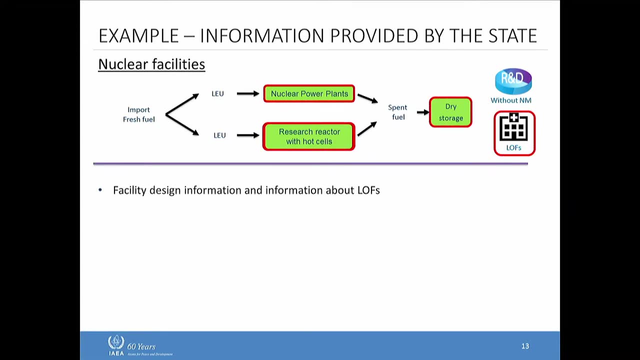 We also get these additional protocols. I was referring to increased information on various parts of the nuclear fuel cycle. These are basically gaps that were missing originally in this original 153 agreement. So just to show some examples, you see the red blinking parts. 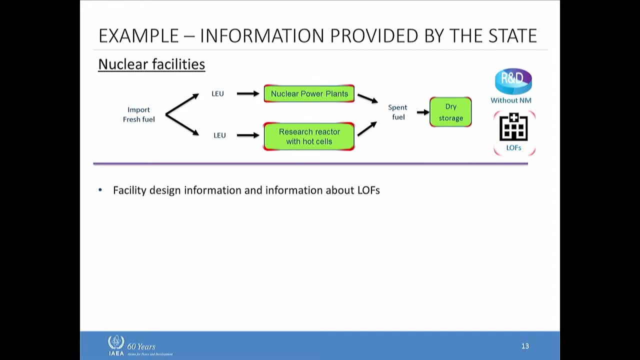 Those are facilities, so the state is obligated to tell us and give us design information about those facilities. The earlier we get it, the better. Someone mentioned safeguards by design. Ideally- and the agency is trying to push this- we're trying to make the architects and engineers and designers of nuclear power plants. 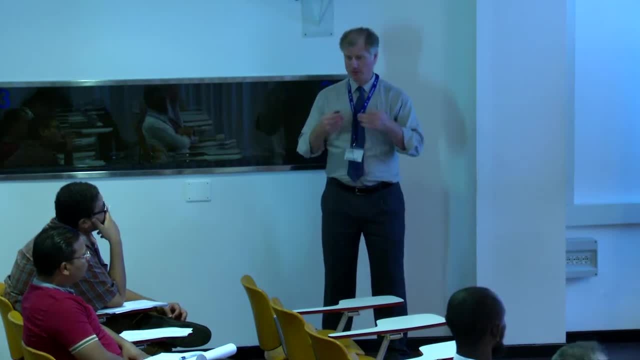 familiar with safeguards so they can what we call design safeguards in early on. Later on we can always come when they're constructing and commissioning the facility and we can put cameras and apply seals and things like that. but it's kind of late in the game to do anything innovative. 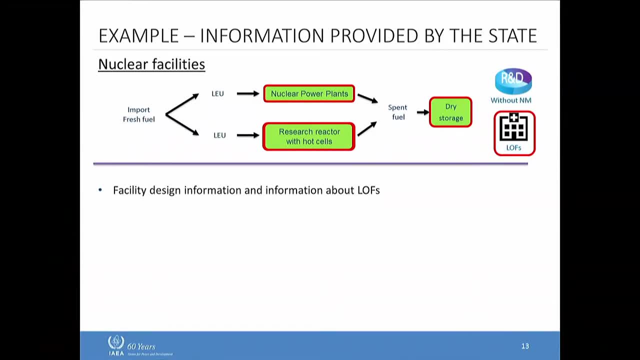 So they'll probably just get a traditional suite of safeguards and measures. We get material balance reports, physical inventory listings that I talked about, ICRs, notifications of imports and exports. We have a good handle on the nuclear material. On the additional protocol side of it, we get things like the description of R&D. 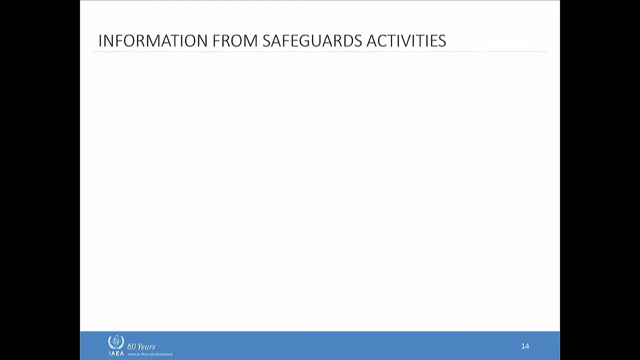 not involving nuclear material: 10-year plans, things like that. Now these are some examples of information from safeguards activities. So these are things that the agency does- inspectors or analysts- So we would go verify nuclear material and we'd have results from that nuclear material accountancy. 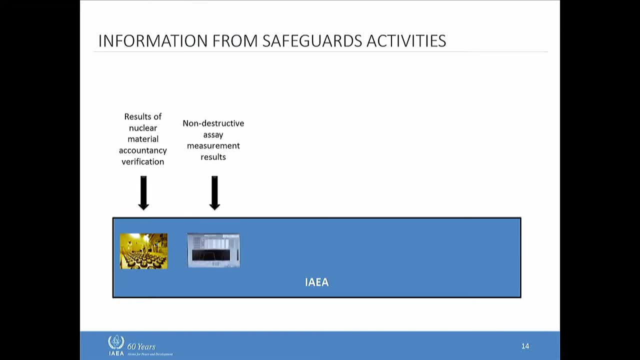 We call it book auditing. We would also kick the tires. We would also take measurements with instruments to determine the uranium content or the plutonium content of a certain material. We could actually, if it's more for bulk handling facilities where there's powders and things like that, pellets. 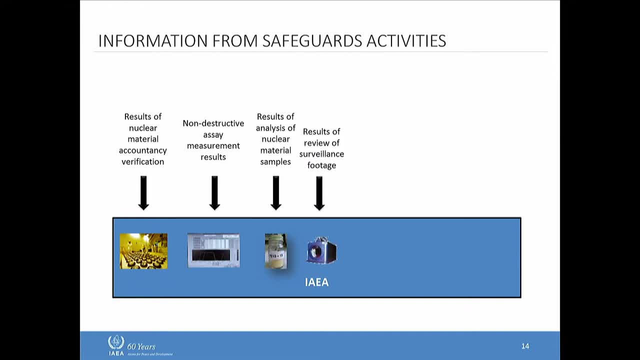 we can take destructive analysis samples In terms of continuity of knowledge. if we verify some nuclear material, we can put a camera on it- let's say over a core, over a spent fuel pond- or we can apply seals, let's say on a reactor core. 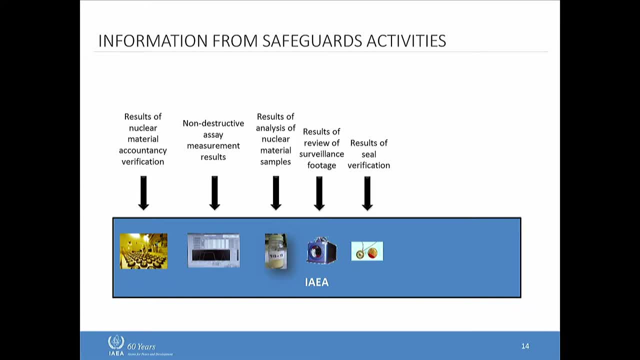 So we don't have to come back and verify the entire core. We can just verify the seal. If the seal is okay, we can say, okay, that's the same content that's in that core. Now, if the seal is tampered with or broken, 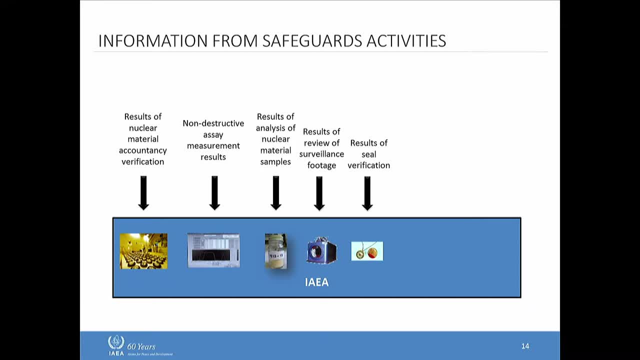 then we'd have to give up. That's an issue, probably an anomaly we'd have to resolve. And again, that design information that's submitted by the state. we do what we call design information verification. They're technically, legally, they're not inspections. 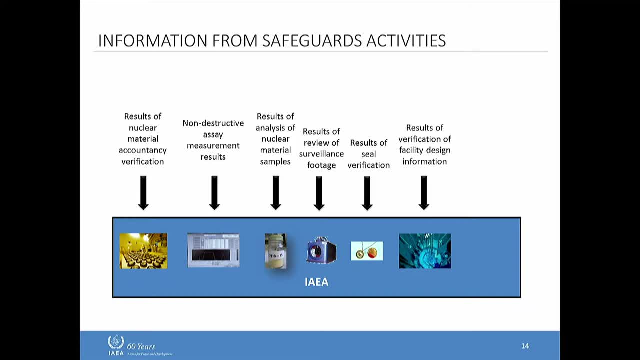 They're visits for design information purposes, but we go and basically confirm that the facility is operated, is built as it's designed and operated as designed, And also we could do things like environmental sampling. Typically, this is done along with the, with the complimentary accesses. 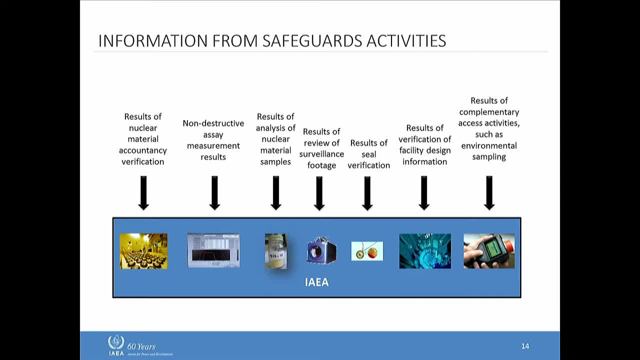 So basically three types of access: Inspections, design, information, verifications, BIDs and complimentary access. There's a fourth one, technical visit. It usually has to do with testing and installing equipment. But generally those are the four types of legal access. 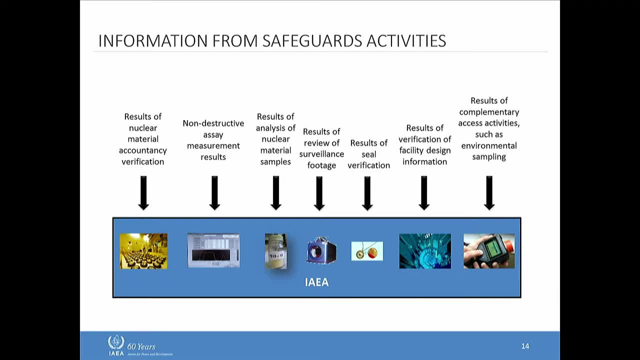 that the inspectors will enter the state in. I should mention there's one more. It's hardly ever used. It's called a special inspection under 153, but it requires very serious conditions to warrant and approve the Board of Governors and things like that. 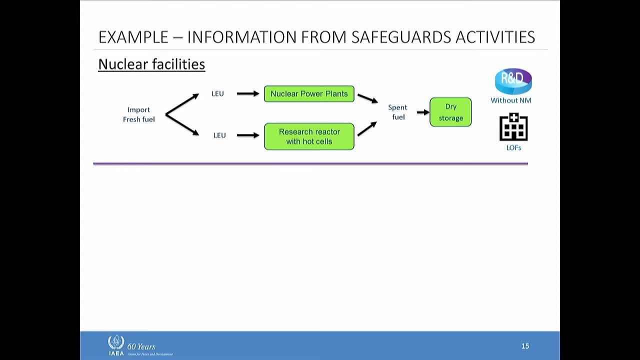 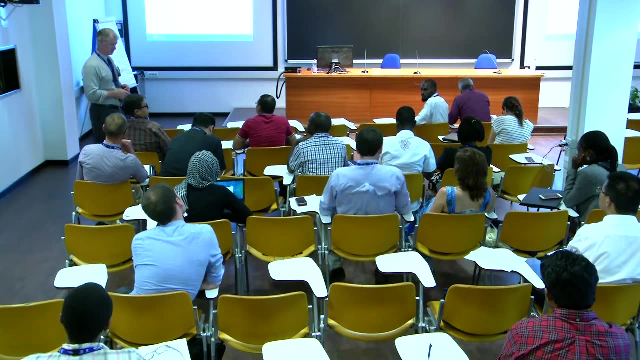 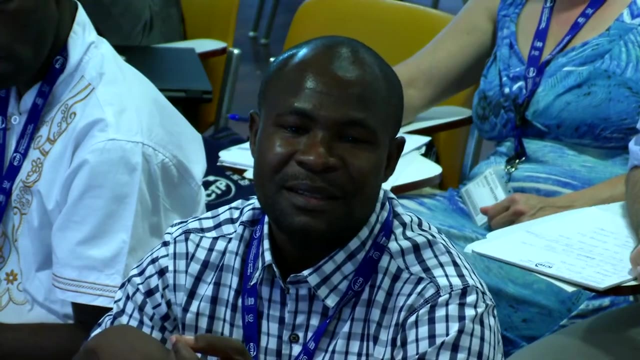 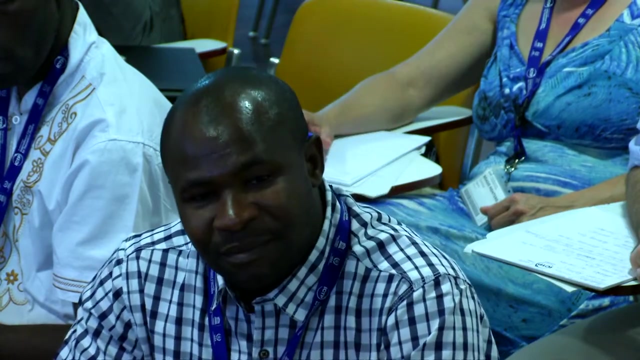 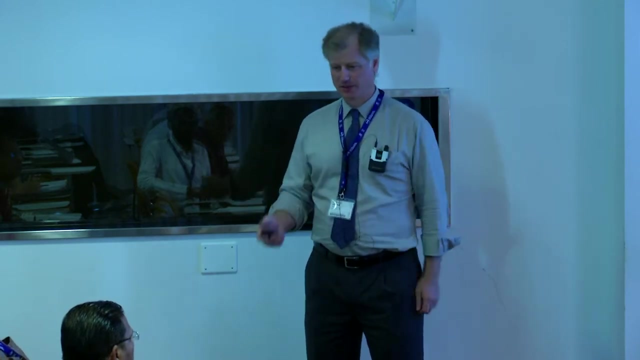 So some examples of oh sorry, go ahead. Could be. my initial thinking when I was inspecting was I trust my instruments And I should have a rough idea If I'm measuring, you know, let's say, a fuel rod scanner. 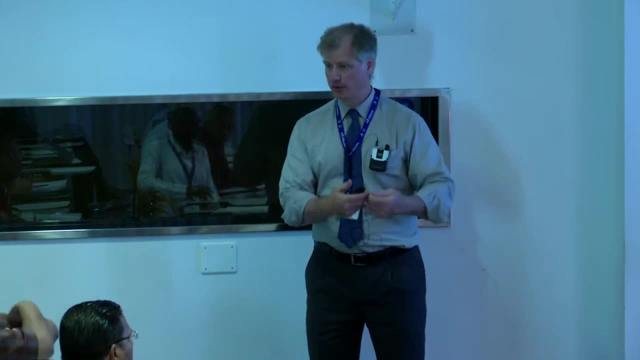 or something. I'm measuring a fuel rod and it's declared that it has 4.2% as the enrichment level of the LEU pellets inside the fuel rod and I get 4.21111 or something I might be satisfied. 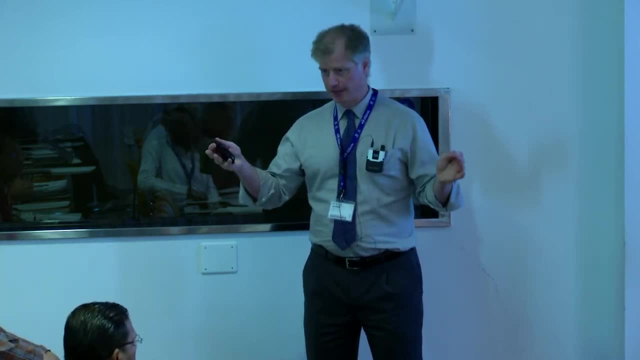 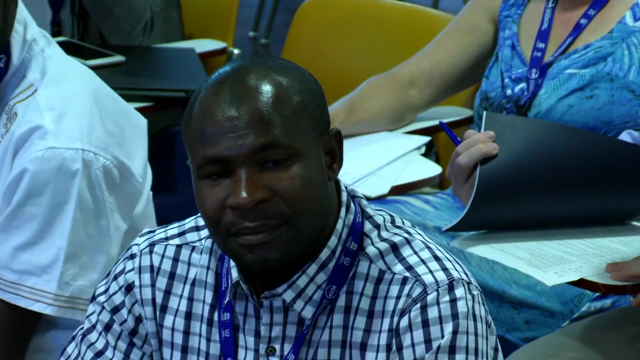 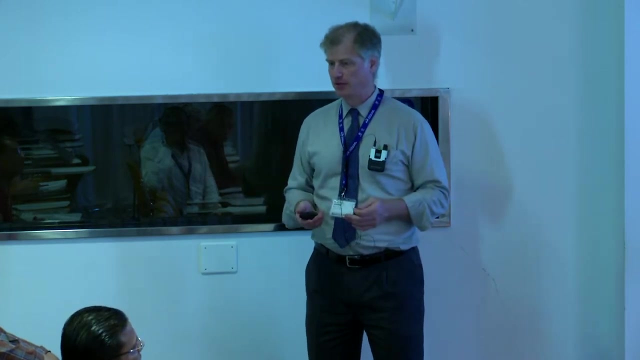 We actually have a threshold statistical windows. it has to be within so many relative standard deviations, But if it's wildly outside that it could be an outlier. Now, if it turns out to be .71,, like natural, I would say this is a bit strange. 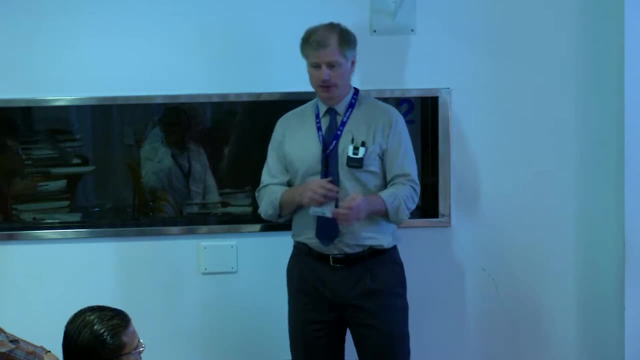 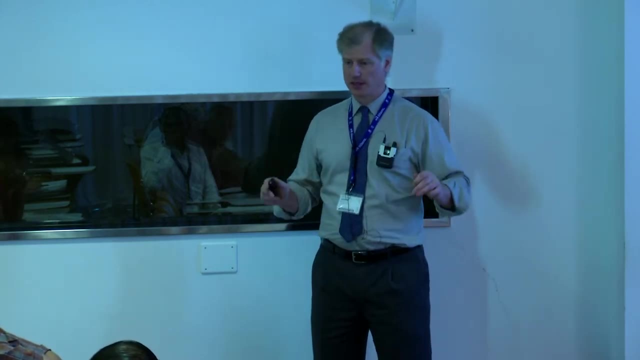 and we would have to resolve that. It could be an instrument problem. Maybe it's calibrated to natural and the inspector didn't set it up properly or something, So they could back off, restart the instrument, check everything. Generally we have standards that we check it against. 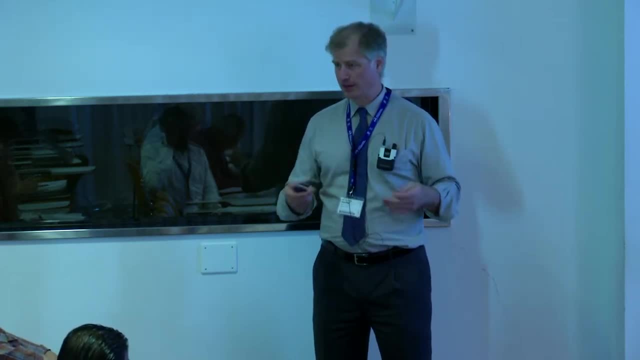 before we do the measurement. So that would be a problem. We would hopefully correct that or make sure the instrument's working fine. But if it turns out it's natural and a re-measurement says natural, we'd probably check some other ones. 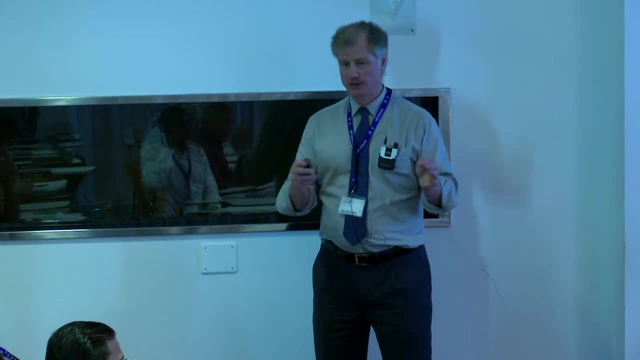 check some other fuel rods around that just to try and resolve it. It could be an instrument problem. It could be a training problem. It could also be it's not as declared. I've seen that Sometimes they take a measurement and I'll say this is not correct. 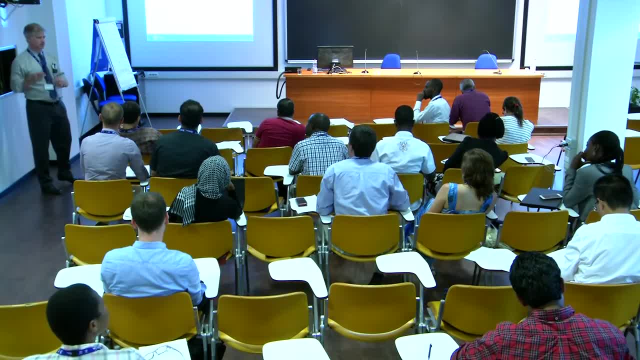 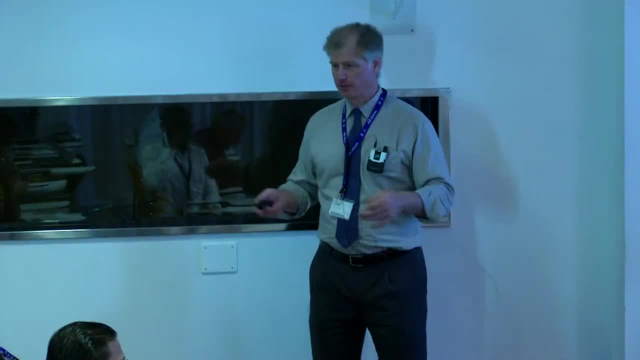 and I realize, ah, we gave you the wrong item, This is the item over here, So we go get the right item. So sometimes we're kind of- I call that QA-ing the inventory of the operator to show we obviously provide the right data. 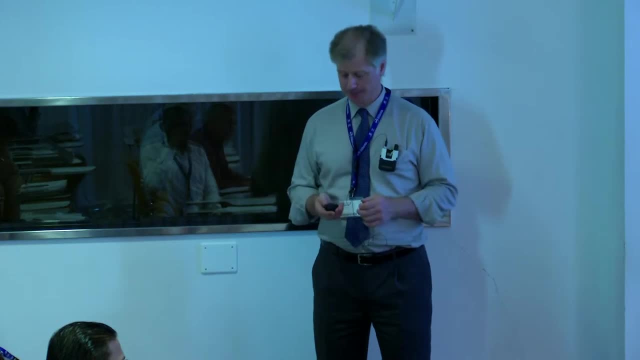 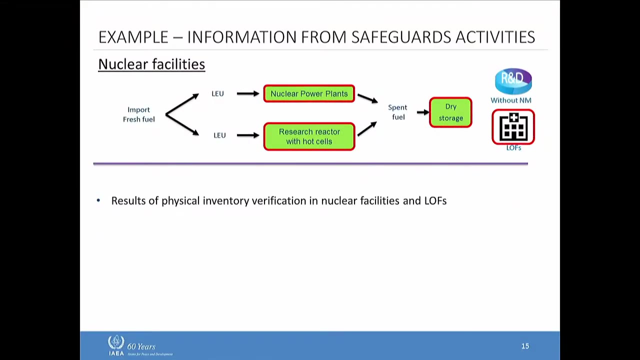 but things happen in the paperwork world and things like that, So it could be an honest mistake. So this is information from safeguards activities. So things we do are physical inventory verification at those sites that are blinking, results of design information verification and results of complimentary access. 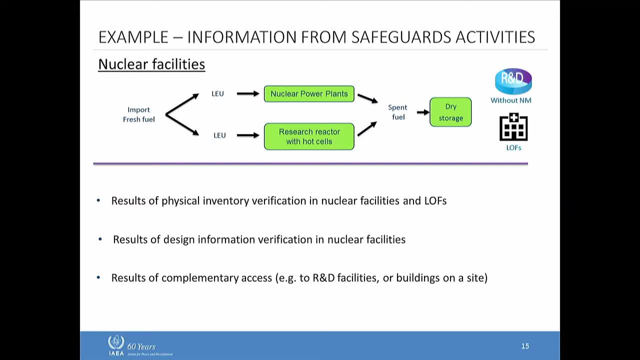 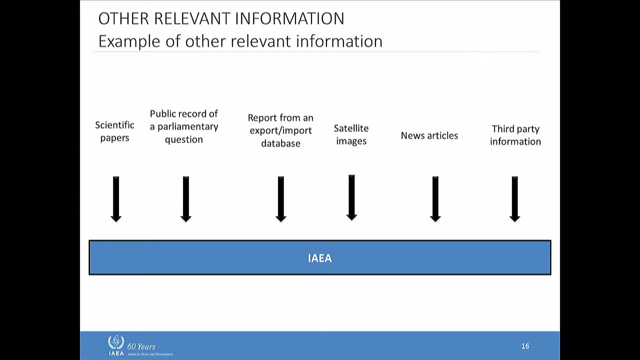 So again we're getting information back. We're comparing that against information supplied by the state And some examples of other information. again I talked about it. It could be just open source in the trade journal technical paper in the news. 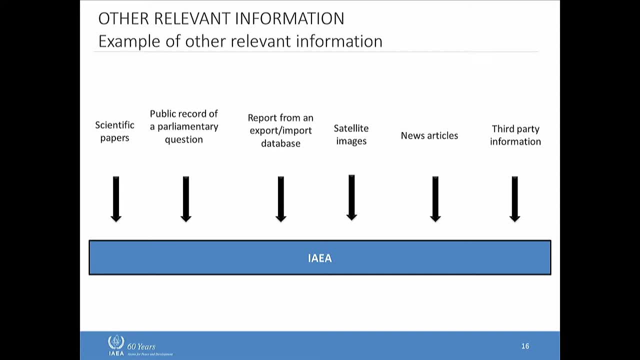 You've got to be careful here, because sometimes there's a lot of bogus information out there, Sometimes an author. if they're not familiar with the nuclear fuel cycle, the terminology might be off, The article might be accurate but it's not so precise. 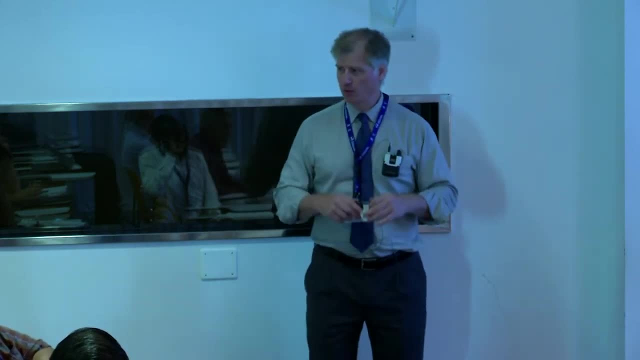 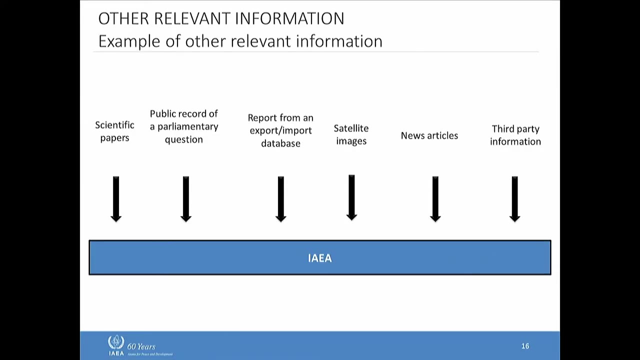 It might be a nugget in there of truth, but you've got to go to the wording because the wording might be incorrect in the terminology. Other satellite images: a lot of commercial satellite imaging providers. now, Again, I talked about these articles. 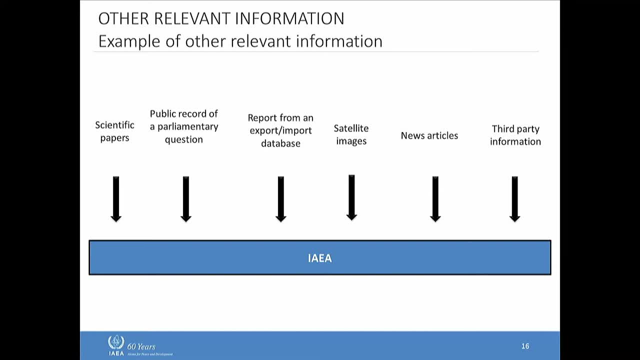 I've probably mentioned this briefly. Third-party information is information that's provided by another state, usually in regard to a third state. So they have a concern about another state that they've gained from their own information gathering processes and they've informed the agency about that. 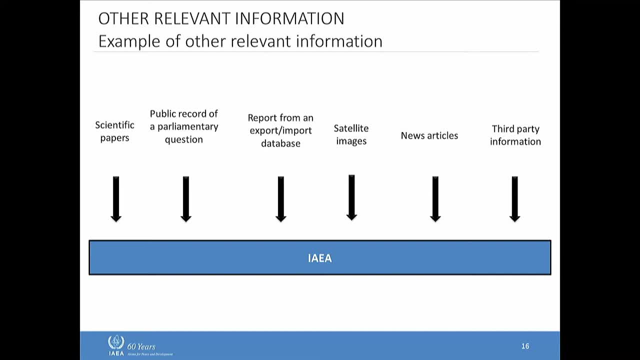 Now we have to be careful here, because that information has to be corroborated. We can't look the other way, but it might be something we need to follow up on. If we just can't assume the state is guilty, we have to corroborate that information and confirm it. 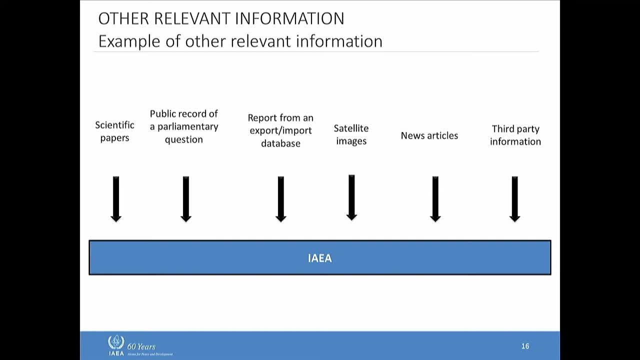 And I should emphasize this- is a very small amount of information that comes into the agency. Most of the information is declarations provided by the operator. There's a lot of literature, accounts, information that they've got to submit And this is growing as more people. in the last 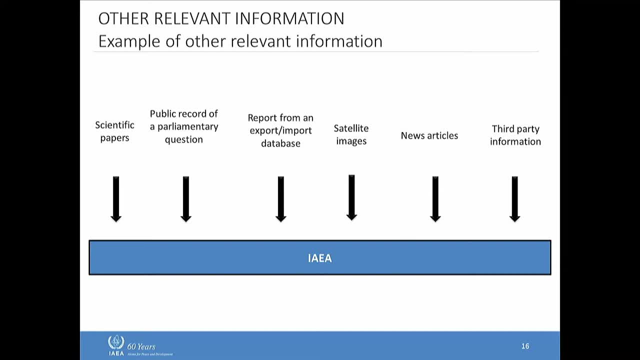 probably the last 10, 15 years- are publishing. There's a lot more people writing about non-perforations. There's a lot more articles out there than there was probably 20 years ago. Obviously, digital technology and desktop publishing. 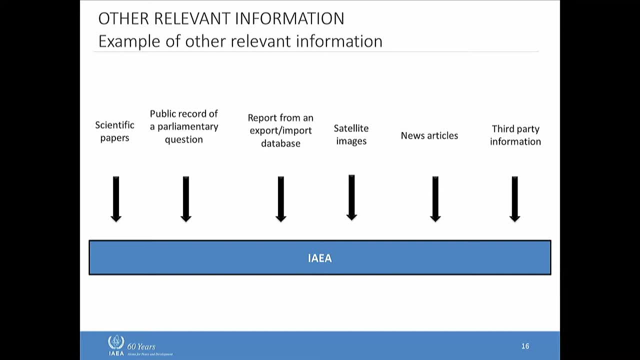 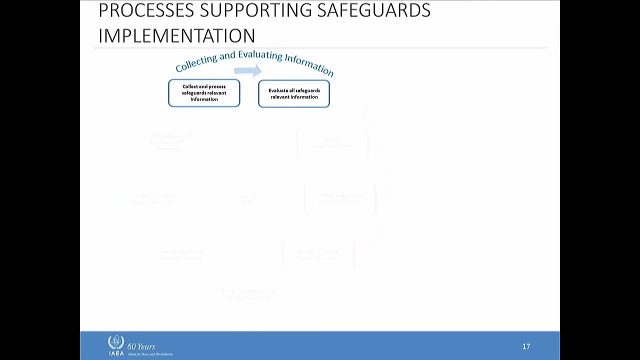 email, iPhones. everything else has to happen, So you get a lot more of this called big data. So we're talking about this part of the safeguards process in terms of the wheel. So this basically established an understanding, a detailed knowledge and understanding. 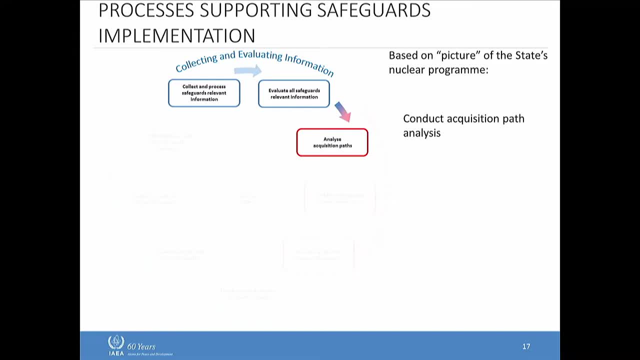 of the state's nuclear fuel cycle, And this will help us now to do what we call acquisition path analysis. Out of that we'll identify the paths that the state could use to acquire weapons usable material. We have to cover those paths and we establish 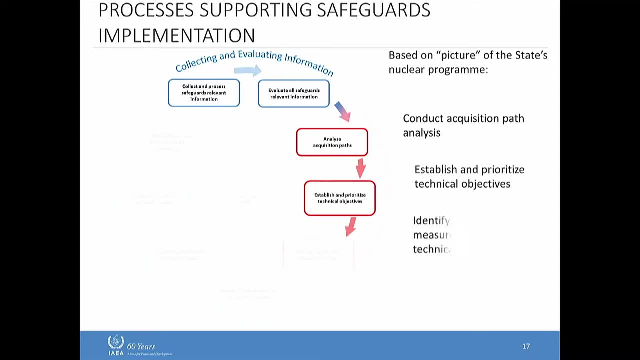 what we call objectives or technical objectives. to do that that we have to meet, We identify measures, and I mentioned some of them. We'll go into more of those At this point in the wheel. we develop what we call state-level safeguards approach. 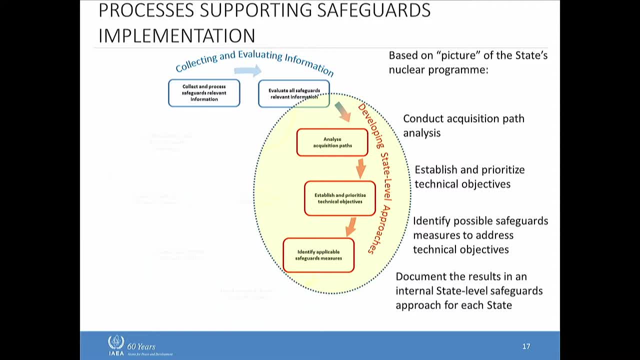 This is essentially the game plan for how we're going to safeguard the state, Still academic, still sort of a headquarters exercise. We're just thinking about how we're going to do this and documenting a plan. So if we return to our fuel cycle again, 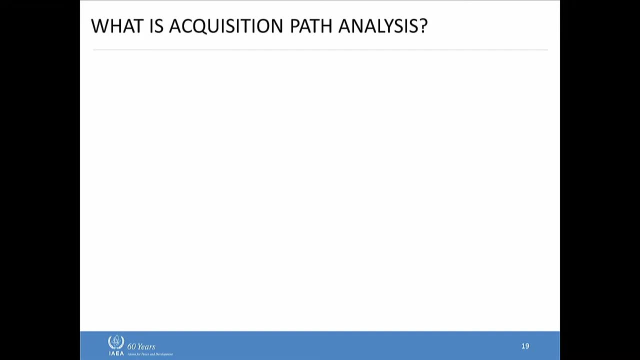 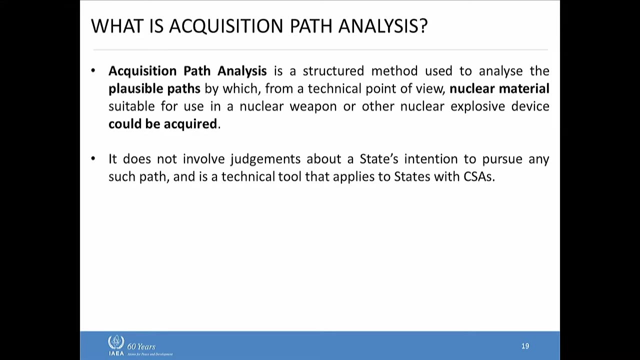 the example fuel cycle. So what is an acquisition path analysis? This is basically a structured analytical method, a technique or a tool we use by the state evaluation group to assess how the state might acquire what we refer to as weapons- usable material that could be useful. 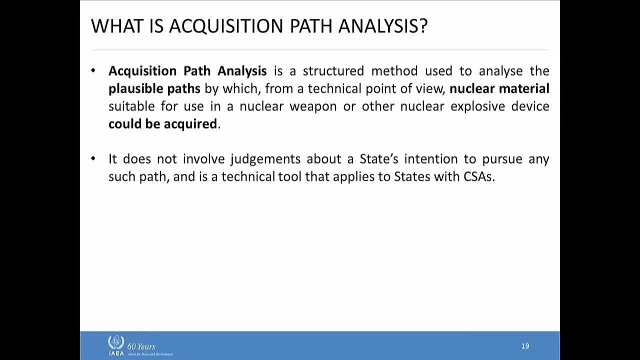 on a nuclear explosive device. I want to highlight it doesn't mean we assume the state is going to do this. It's a hypothetical assumption for the purpose of analysis. We make this assumption for all states. So if the state decided to pursue a nuclear weapons program, 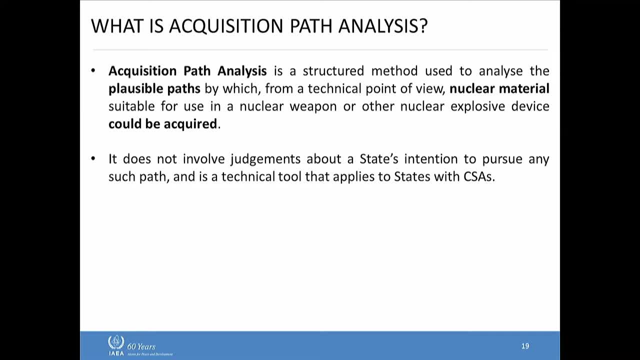 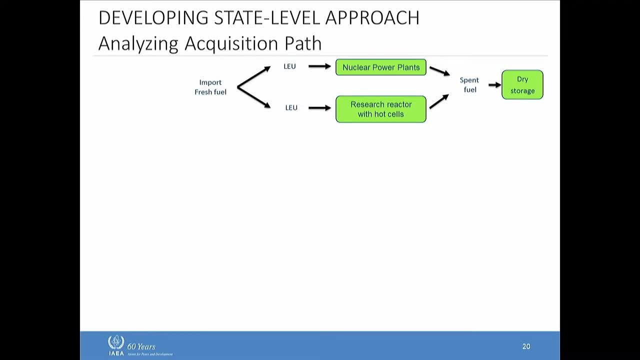 how might they go about acquiring the weapons usable material to make that happen? So let's look at our example. If I ask you to look at this peaceful fuel cycle and you're doing acquisition path analysis and we usually tell the analyst to kind of switch, 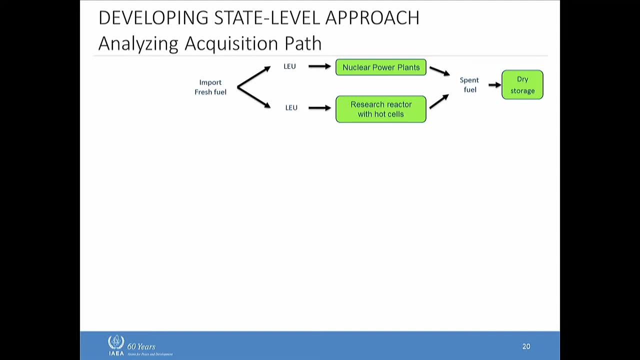 their thinking a little bit and adopt what we call a red team outlook and look at a little bit from the state, from a state that's again hypothetically proliferating. if they decided to do this, how would they go about it for this nuclear fuel cycle? 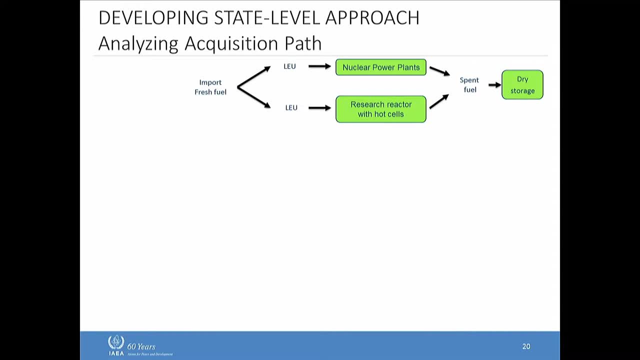 Remember I mentioned earlier, there's three types of nuclear, three types of nuclear bombs with three types of materials. What were those three materials Might be good for the test: High enriched uranium, plutonium and then less obscure uranium-233,. 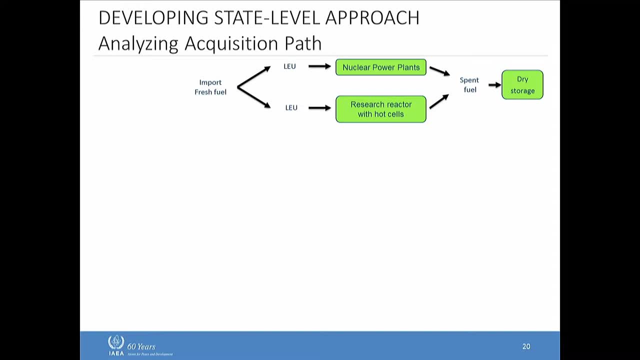 a little more obscure uranium-233.. So if I looked at this fuel cycle I didn't tell you anything about thorium. So they probably you know they could irradiate. They'd have to have some knowledge about that and separation, but that wouldn't indicate any thorium. 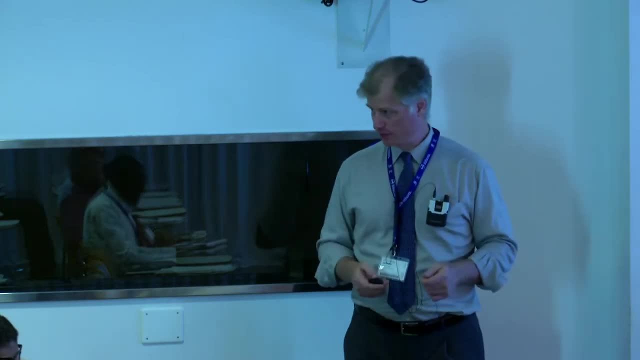 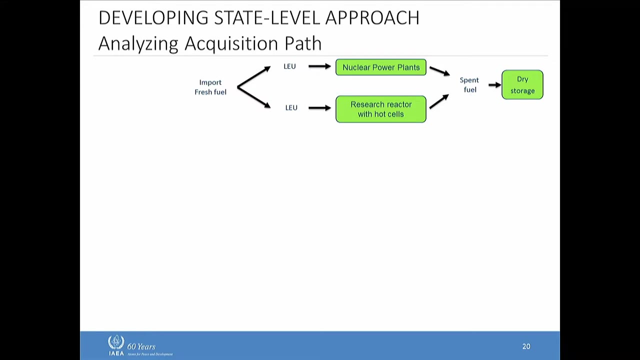 in this fuel cycle, So that may not be a main consideration. Might assess for it and then rule it out. They have LEU. They don't have any uranium on it. They don't have any mining or anything like that, but they do have this uranium inside their fuel assemblies. 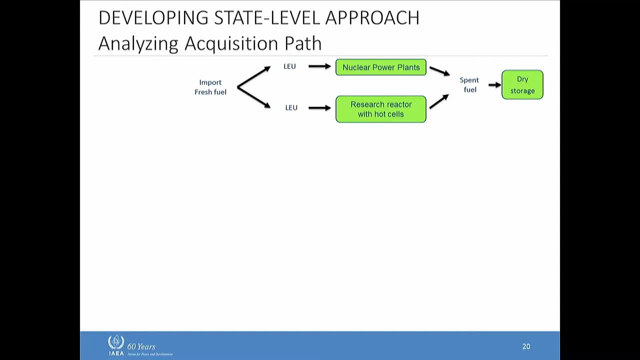 They could not put them in a reactor. They could divert the assemblies, break the assemblies, take out the pellets in some process. That material's very, you know, it's not highly, it's not radioactive. You could approach it in a hood. 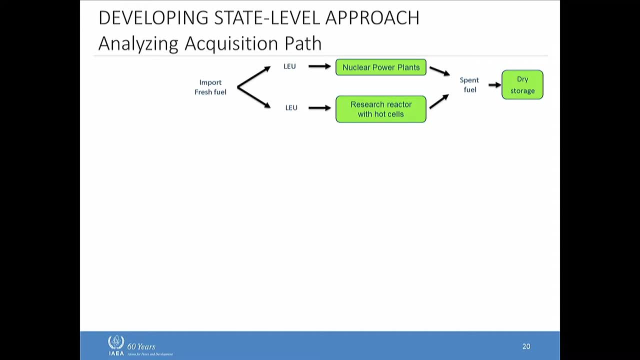 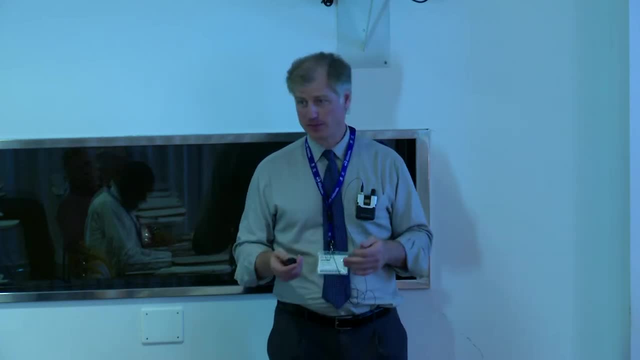 glove box type environment. But they'd have to do a lot more to it. They gotta break it down, They gotta crush it, They gotta dissolve it, They gotta convert it into UF6. They have to have burn enrichment. So there's a lot of capability. 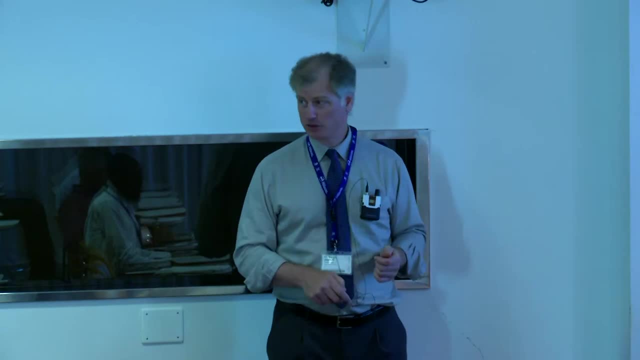 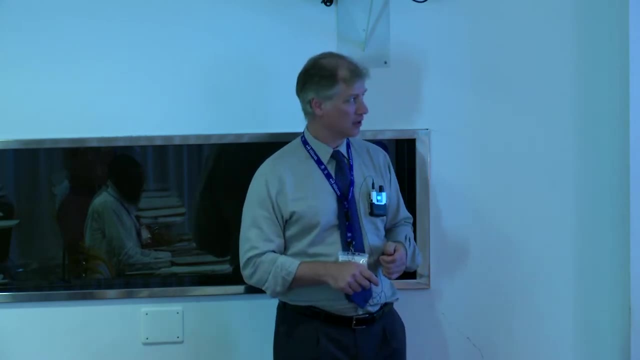 this state doesn't have in order to make that LEU turn into an HEU weapon. So the SEG would assess for this and say that would take a long time for the state to accomplish. We don't ignore it, We just put less emphasis on this LEU. 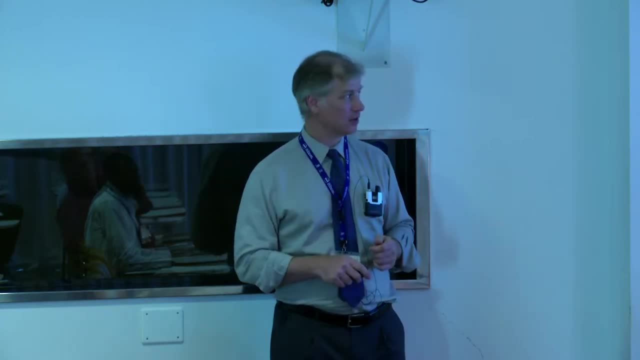 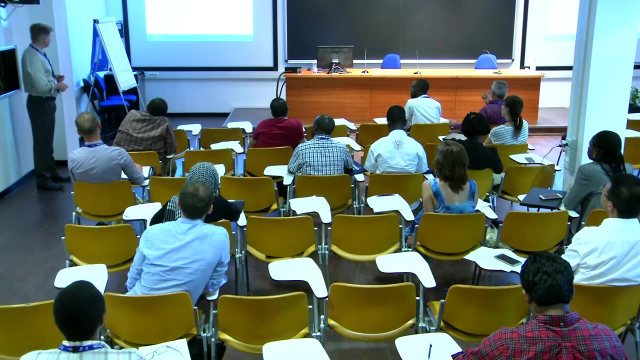 because we're recognizing for this state's capabilities that hopefully you understand very well. it would take them a long time to turn that into an HEU weapons use material, HEU for a bomb, But this state they have plutonium in their spent fuel. 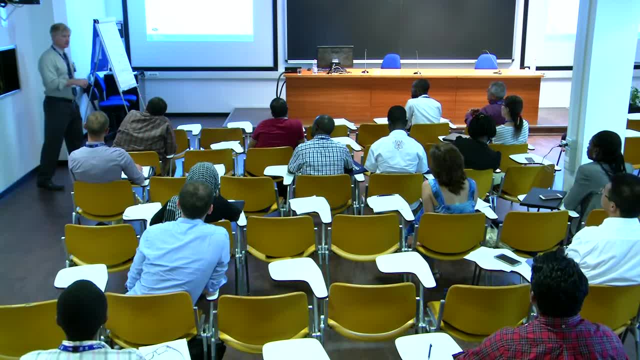 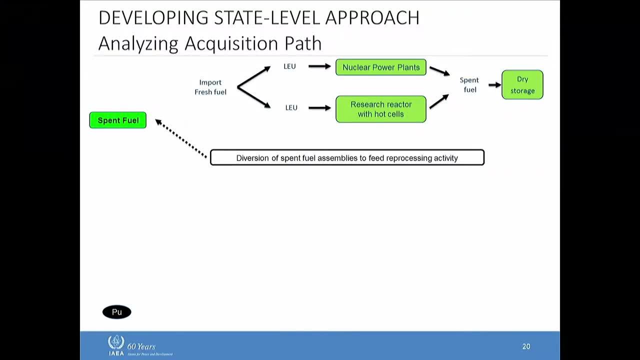 So let's see if we analyze for that begin with that end point. Let's say the state wants to aim for plutonium. Okay, the first thing they'd have to do is they have the spent fuel. they have to divert the spent fuel. 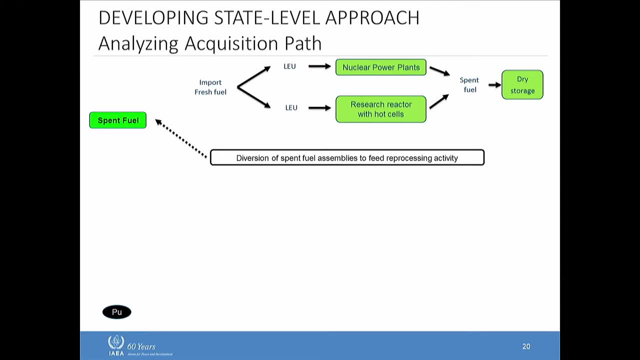 So they gotta take it out of the dry storage, or take it out of the spent fuel pond, or when it's discharged from the core, they've gotta take it out, Although there they'd still have to set it to cool for some time. So that would be the first step in this acquisition path. 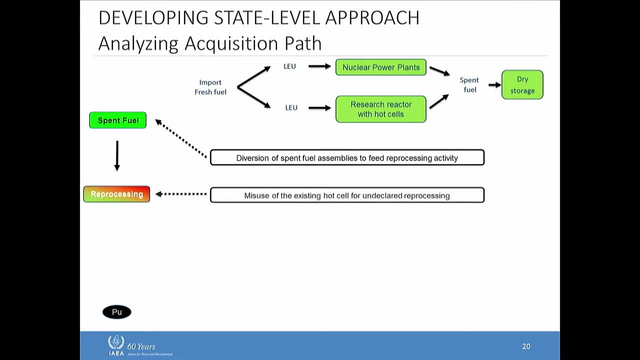 is a diversion step. Next, that spent fuel is no good, with all those fission products and actinides and what I mentioned earlier about it. It's highly radioactive, self-protecting good from a safeguard standpoint, because any processing of that material 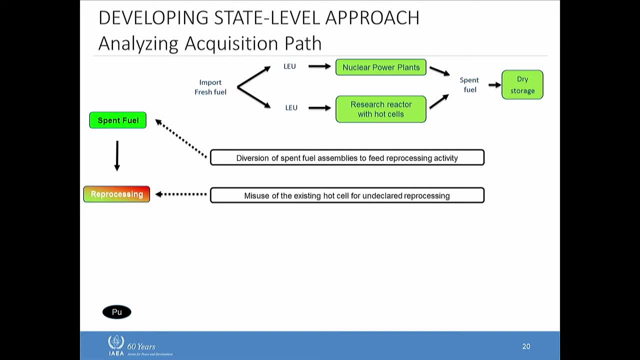 that's spent fuel requires shielded casks, hot cells- I used to work at large canyons that did this- But you need remote manipulators, leaded windows, things like that So sophisticated, But we did notice that they, as we said, for this. 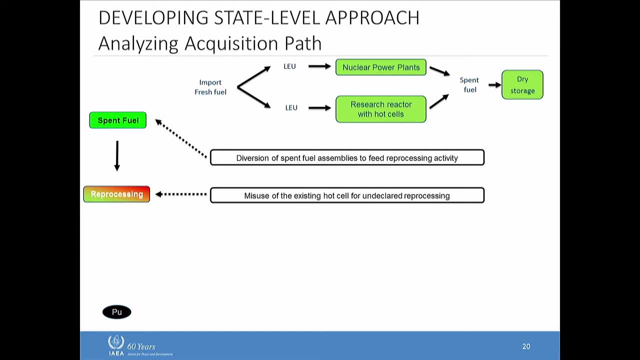 that they had hot cells. in this state They could actually process fuel assemblies, Definitely the research reactor fuel, maybe the power fuel. And we call that a misuse step. They misuse an existing declared facility. So they've diverted declared material, They've misused. 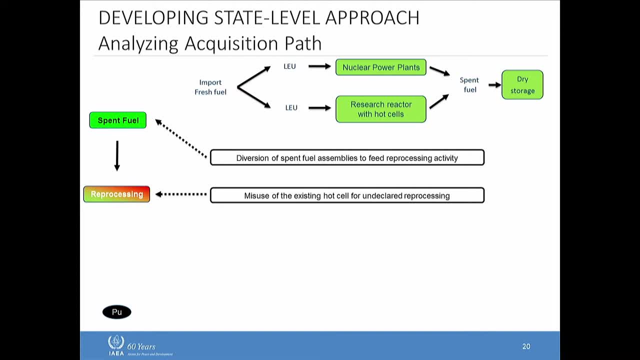 Again, this is just hypothetical. We're just speculating from an analytical standpoint. But even out of this it'd probably need one more step in its conversion, because usually reprocessing you get either plutonium nitrate or plutonium oxide, But once you've removed the fission, 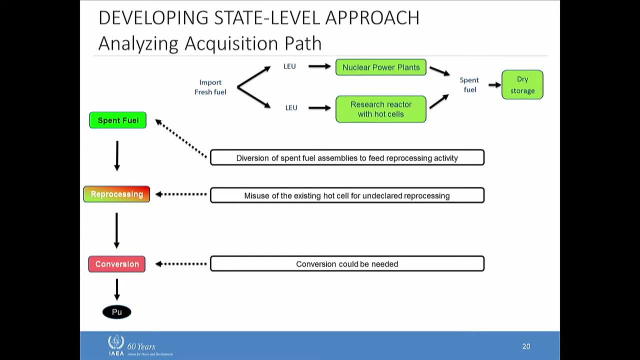 the fission products and the aconites there's not a lot of, then you don't need all this shielding and all these things. I was talking about shielded casks. Now it can go back into a generally a glove box type operation. 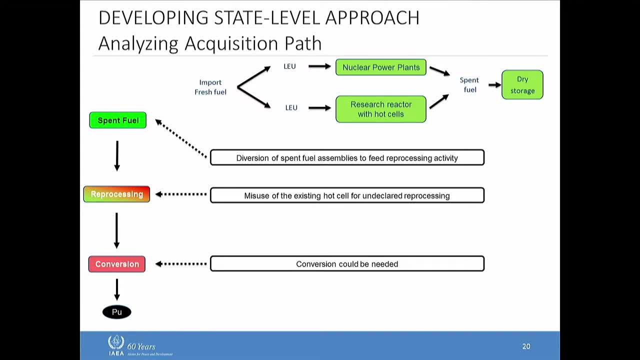 I used to work in a facility that did this. It doesn't have to be very large. The facility I worked in was pretty large because it had high throughput. It's also say it was in a nuclear weapon state, so it was permitted legally. 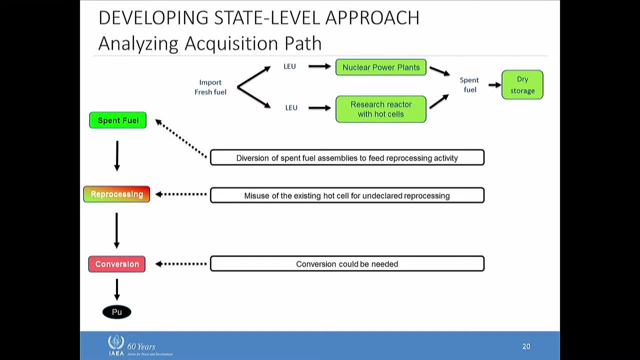 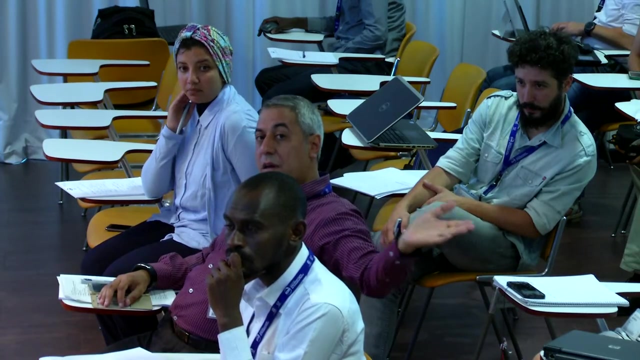 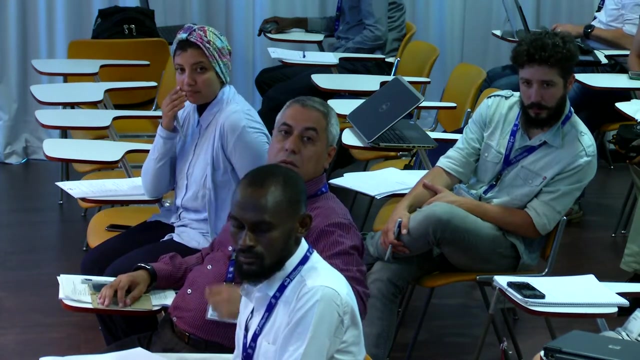 But it's not a big operation. We've identified a technically plausible path for this state to acquire weapons usable in the material plutonium. that consists of three steps: Diversion, misuse and an undeclared step. Yeah Well, generally we're just analyzing. 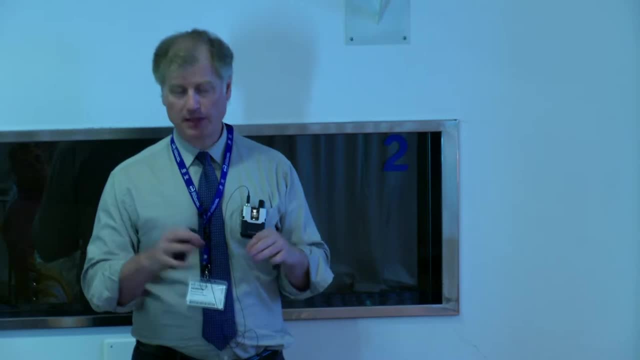 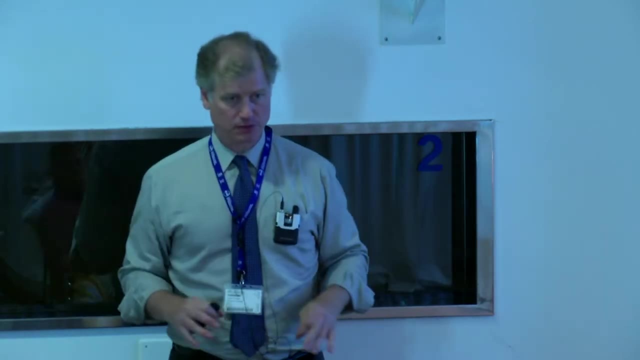 at a state level We don't really. I mean if they're getting material from another state, we'd say yes, that material was declared to us, it was exported, it was imported. it's all part of the peaceful nuclear fuel cycle. 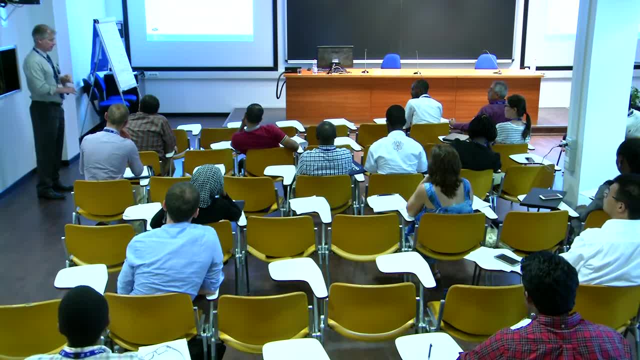 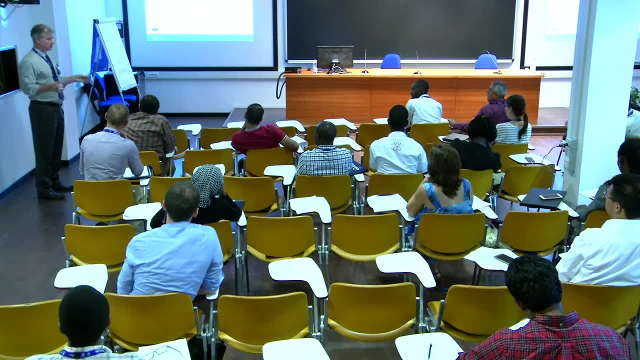 We recognize that it's now not in this state. it's in this state But there may not be any. I'm not sure if you meant this. there may not be any collusion going on And generally in X-ray path analysis we don't consider a collusion. 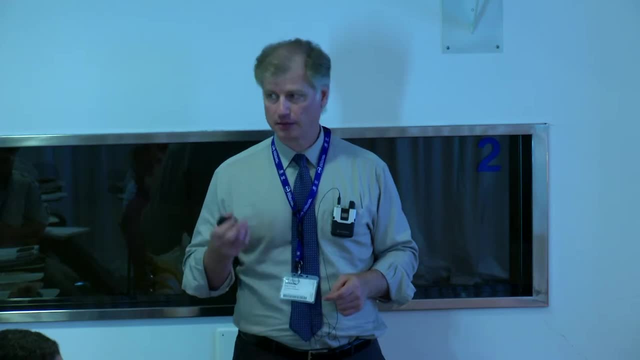 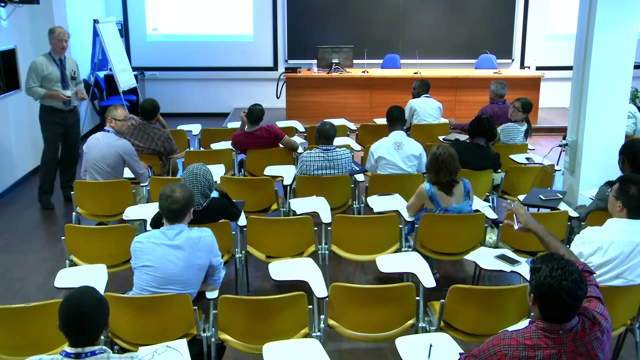 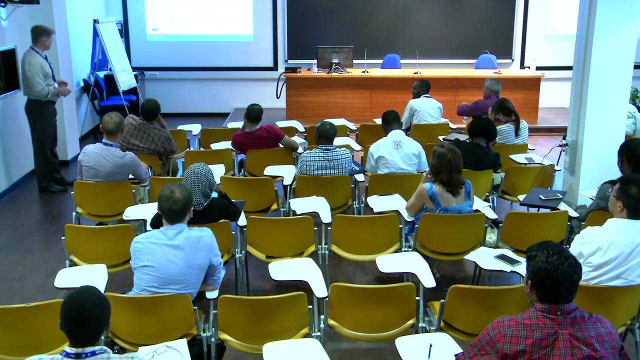 unless you have information to counter it. But generally it's just about a single state's nuclear fuel cycle capabilities- Again a hypothetical analytical technique. So here we hypothetically said that they have a as part of the illustration, they have a research reactor. 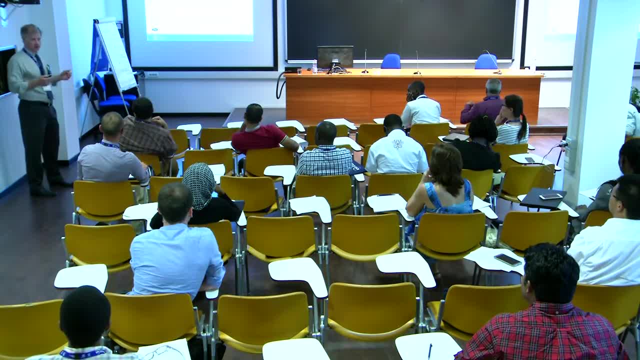 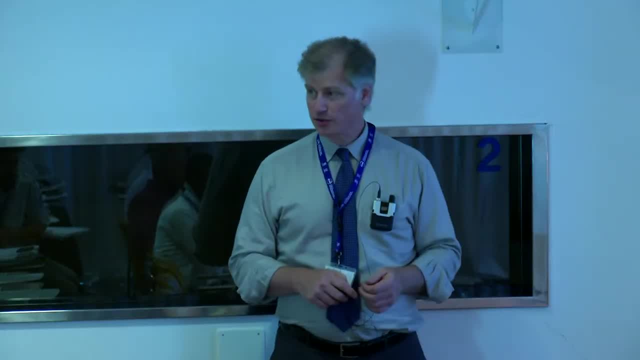 with hot cells associated with it. Let's say, usually they're making medical isotopes. I think that's what we postulate, that's what they do just for the sake of this exercise. So they're basically shifting this research reactor and the hot cells from a 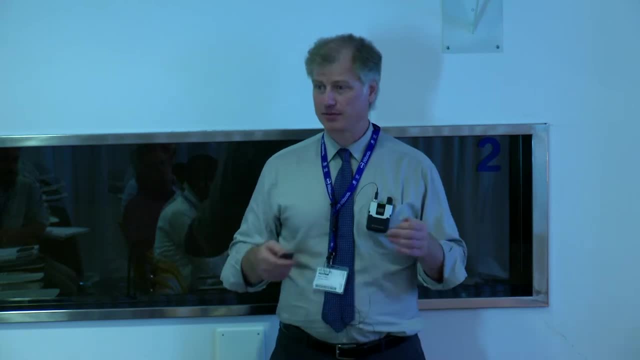 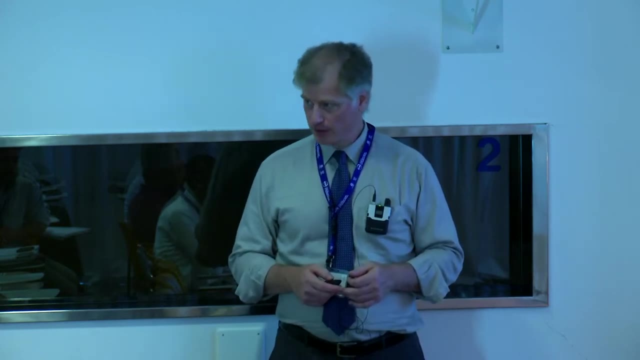 let's just say molybdenum technetium mode of operation might have to do some redesigning because they have to have some pretty smart people on the neutron management side of it. they have to have enough, but if it's enough, 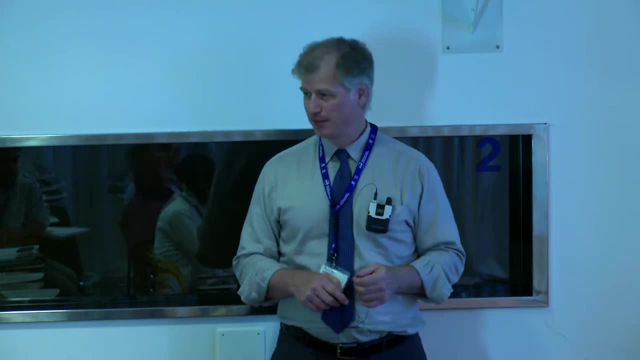 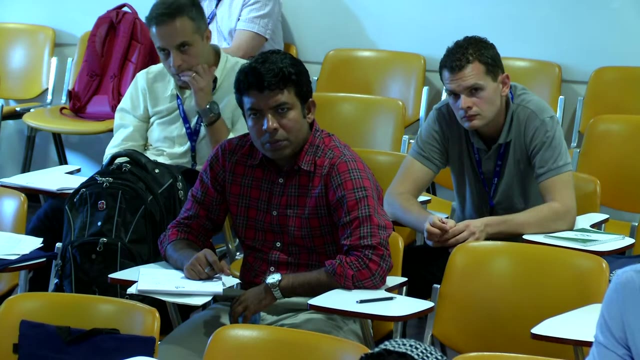 or if they upgrade it and they upgrade the cooling. if they need to do that, they can misuse this. They basically go from a medical isotope production mode to a plutonium production mode and they shouldn't be doing that. Their declaration and their design. 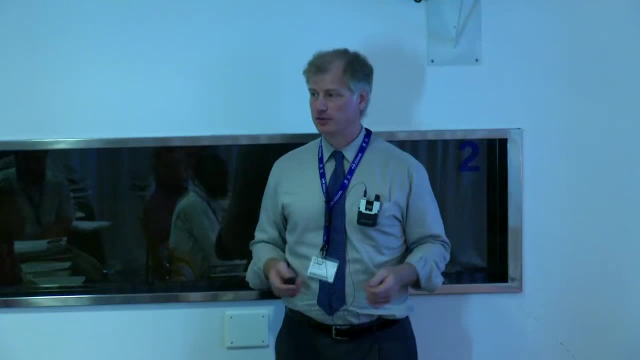 was for medical isotope production. they shouldn't be producing plutonium. That's not what their declared stated purpose of that reactor is. That's what we mean by misuse of the facility. So it's undeclared production. They don't tell us about this plutonium they're producing. 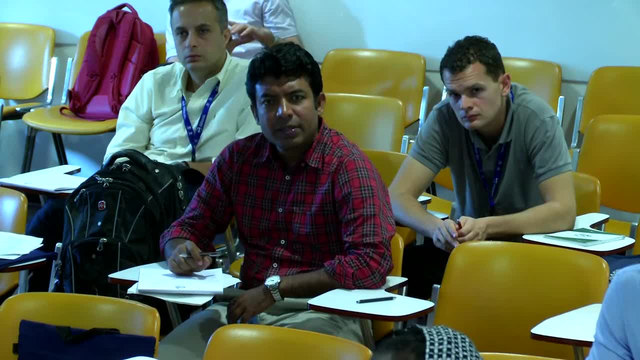 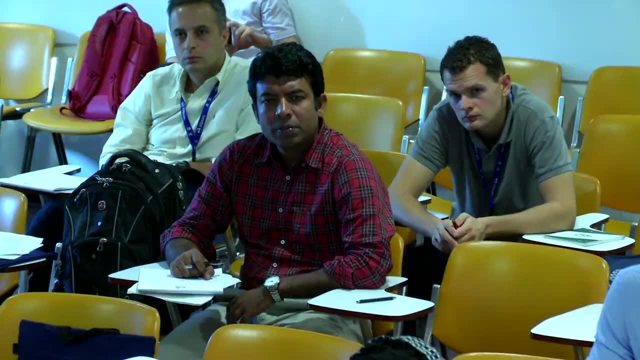 and they should. They're obligated to No, no, no, It's not authorized. This is an example that they've diverted the spent fuel and now they have to reprocess it to separate out the plutonium inside it, So they've got to chop it up. disassemble it. It's a messy process. It requires a lot of shielding, a lot of expertise. They have to have acids and chemicals that are going to dissolve the material inside that. Usually they cut it up into something called hulls, but they'll dissolve the fuel mix out of it. 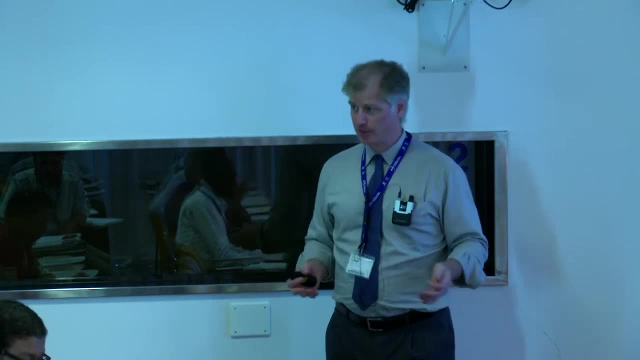 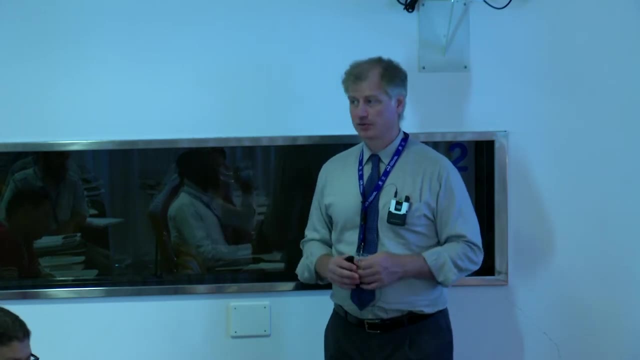 along with all these fission products. You have to send it usually through solvent extraction processes, So they'll need processes to deal with that, for solvent extraction Mixer, settlers or pulse columns, things like that. So there's a lot of- in addition to a lot of- chemistry know-how. 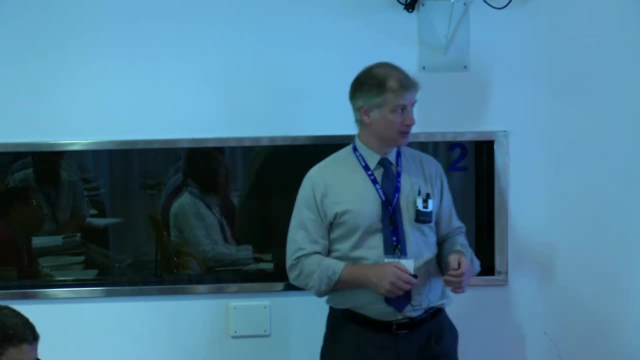 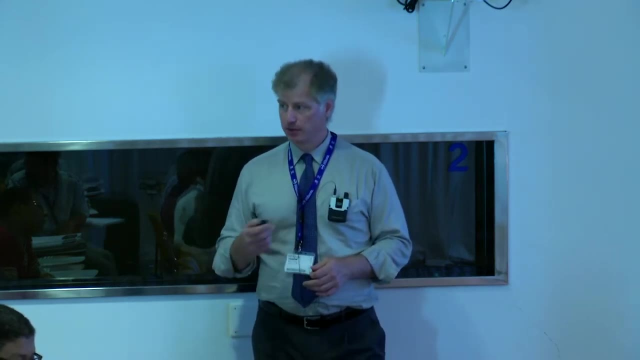 there's a lot of plant know-how they have to have. I should say that doesn't have to be massive. So I mentioned earlier Japan has reprocessing. They have a huge plant, Hikasho, for covering their plutonium uranium from their large. spent fuel inventory. But that's on the order of, I think, 800 tons a year. You don't need 800 tons, You need like a hundredth of that size. You just need a much smaller scale footprint reprocessing facility. 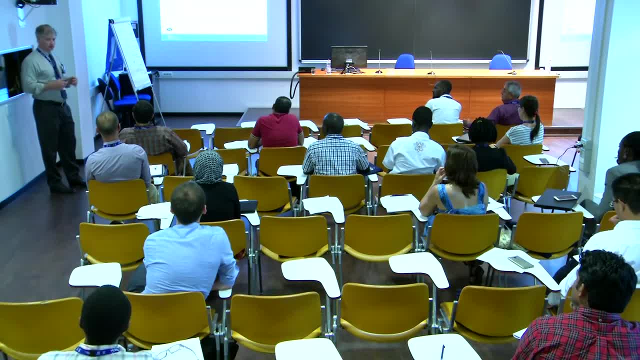 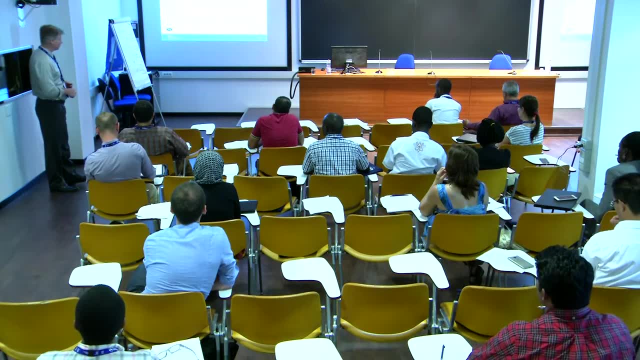 It could be on the order of a hot cell, But you would need some shielding and heavy duty remote manipulators and that type of equipment for reprocessing. For the initial step, This part here Down here- less shielding, less remote operation. 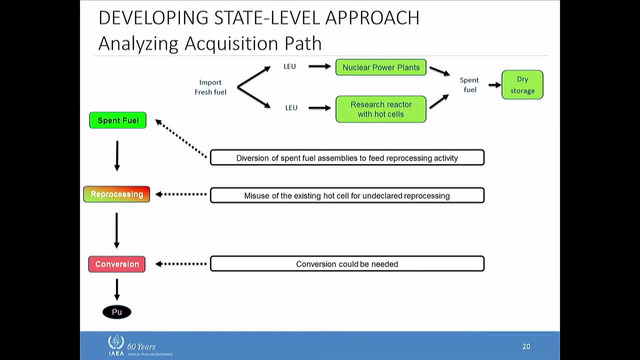 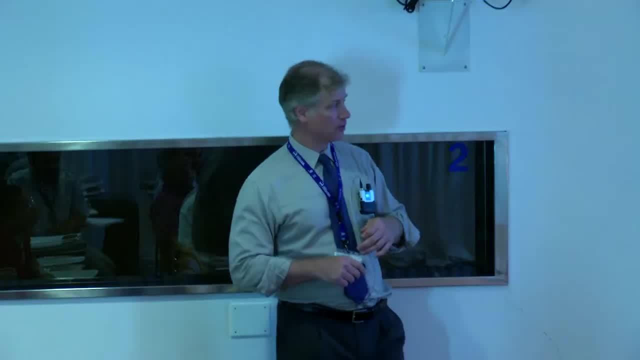 Here you would. So just to highlight, that's a diversion step, Because they shouldn't be doing it. And then this is a facility they should tell us about if they're introducing new material. They don't even tell us about it. We're just postulating this might be happening. 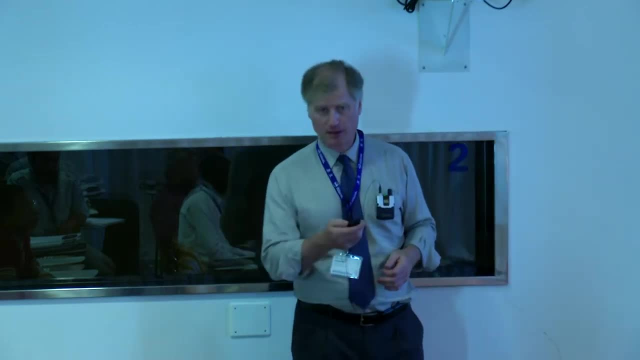 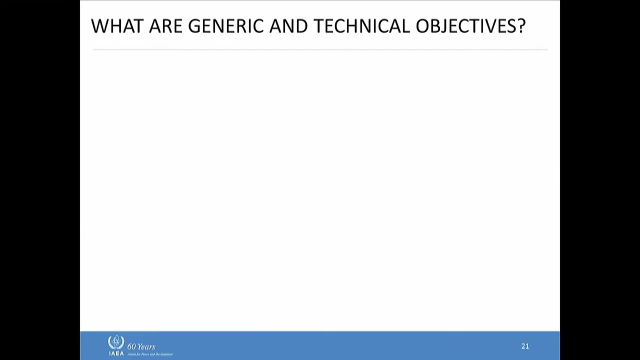 because we have to say how can they complete this path, because that gets into how we're going to cover the path And I'll move on to show you how we do that. So we have what we call generic and technical objectives. Generic, as it sounds, is just generic. 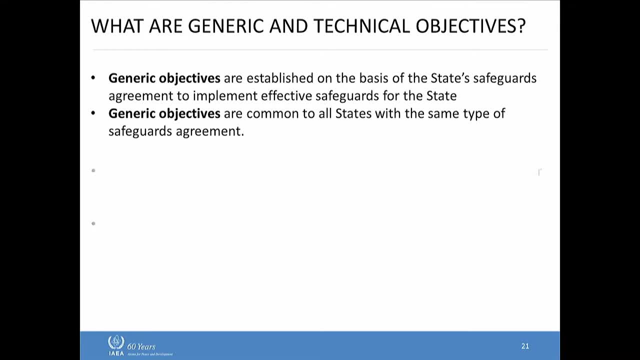 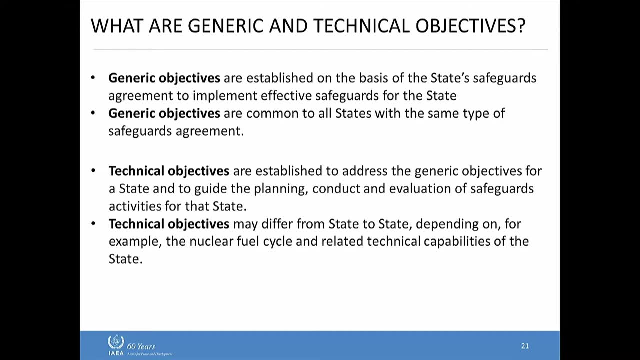 We're looking for diversion and misuse and undeclared new material and activities, But we have to turn these into specific what we call tailored or customized technical objectives to cover that step. And they're more specific And this is what that safeguards evaluation group that SAG or the operations has to meet. 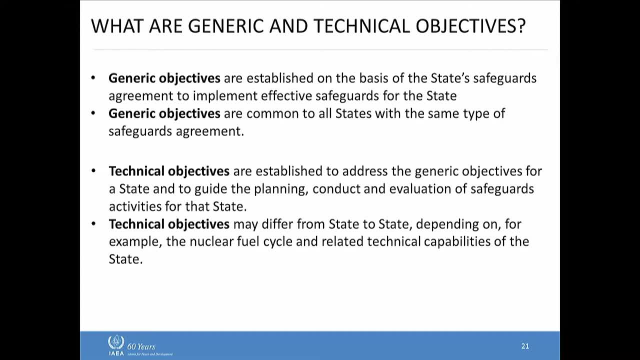 We have to meet these TOs to make sure that we have assured ourselves that our activities conducted were adequate, to make sure that these postulated acquisition paths are not occurring. So we inspect the nuclear material. It hasn't been diverted, It's there. 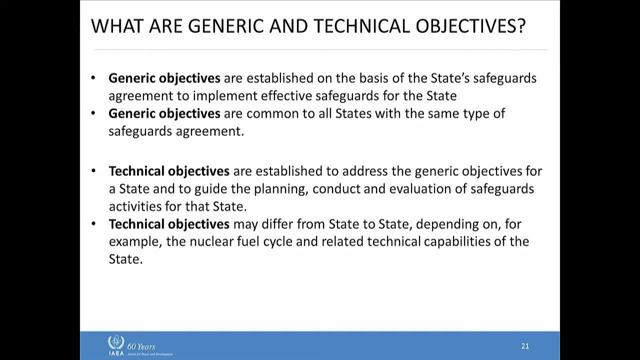 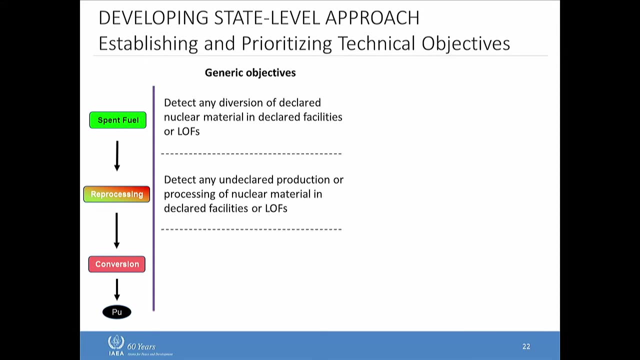 So that path is probably not occurring. So, basically, TOs help us to plan and guide how we're going to conduct our activities, allocate resources, things like that. So, if I go back to this example, we have generic objectives And I just mentioned them. 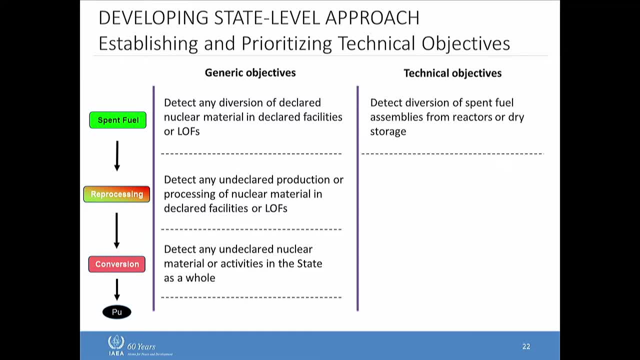 And we turn those into technical objectives A little more specific: Detect diversion of spent fuel assemblies from the reactors or the dry storage. Detect undeclared reprocessing in the research reactor, hot cell. Detect undeclared conversion to PV metal in the state. So those are technical objectives. 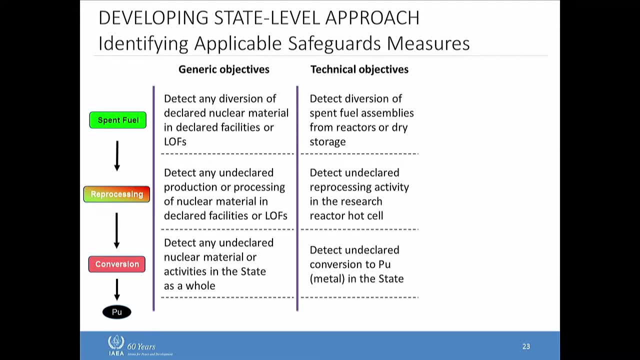 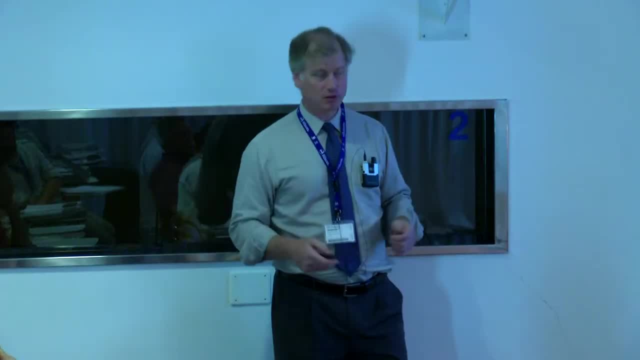 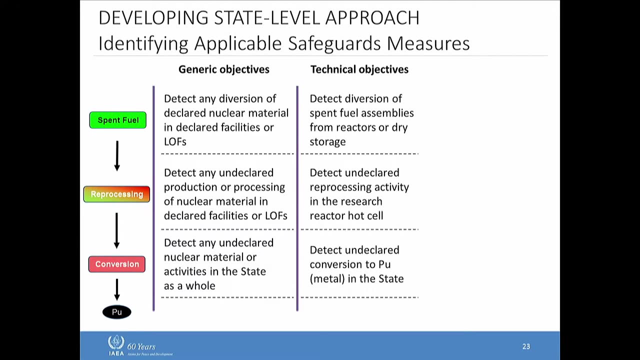 And we have assured ourselves that these are not occurring. So we just speculate that they might, but we conduct activities that will help us confirm that that is not the case. Just as a general question, do you think to cover this pathway, is it more important to meet? 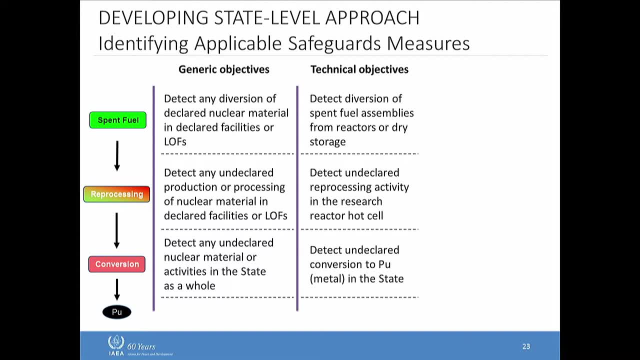 the first TO on diversion, the second TO on misuse or the third TO that's related to a totally undeclared clandestine facility. Well, this would have to go before a committee. actually, I think a lot of industry officers would have to sell their approach. 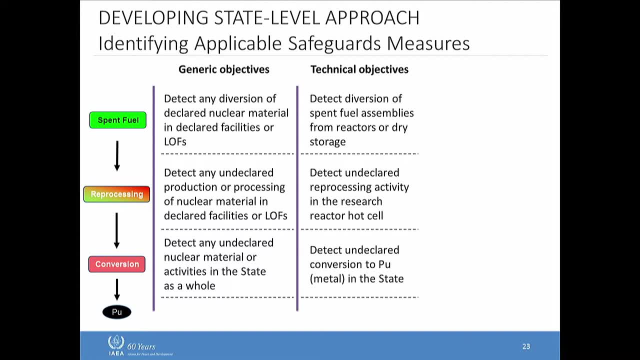 to the committee. So to me it would make sense if they put a lot of emphasis here on the spent fuel, some emphasis on the reprocessing step and some, but not too much, on the conversion step. I mean theoretically, if I could cover this conversion step. 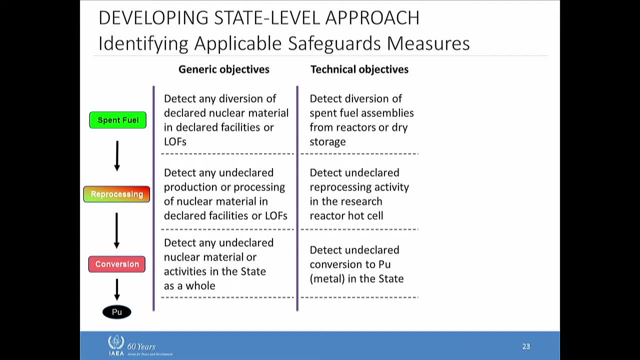 and say this did not happen. I don't have to do anything at these two steps. If this step doesn't happen, the measures here are not so good. We don't have an address, We don't have a location. It's probably not going on. 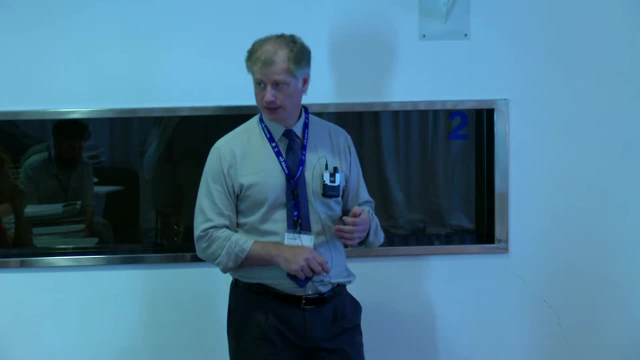 shouldn't be going on. hopefully isn't going on, And if it is it'll be very difficult to find, So we would focus more at the locations where we have an address. We know where this research reactor is. It's under safeguards. 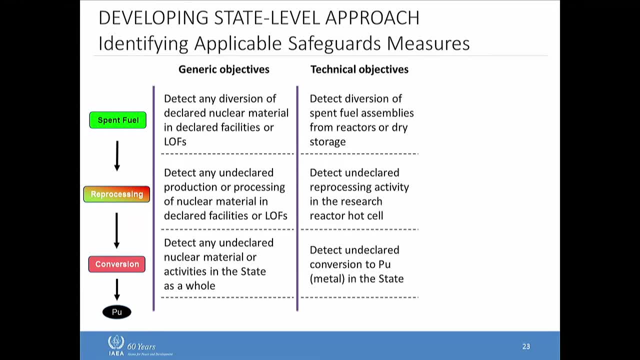 We would just go there to make sure it's still being used to make medical isotopes and not being converted to PU production type mode And the spent fuel. We could check the spent fuel so we would put the lion's share of the emphasis on that spent fuel. 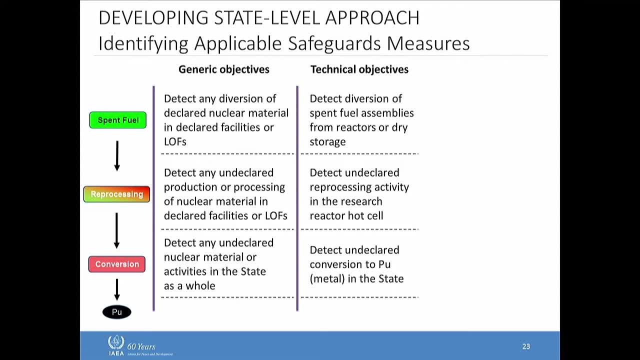 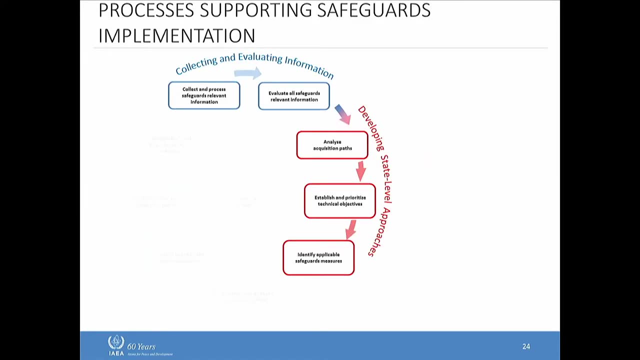 That would be the highest priority technical objective. We would also check the reprocessing facility and less emphasis on the conversion facility. These are just some examples of safeguards measures. I'll go into those in detail. So now we've done this part of our wheel. 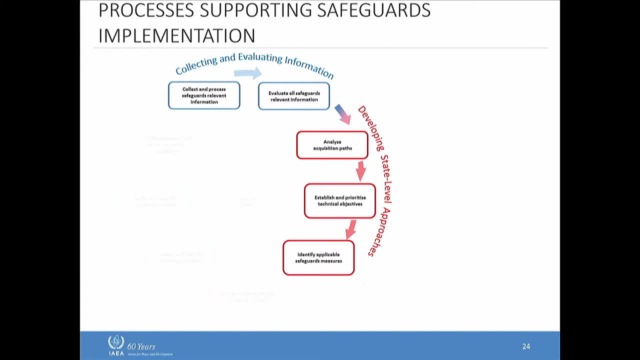 where we've got our approach. Again, as I mentioned, this is fairly dynamic at this point. We've done all this analytical work at headquarters, but now an inspector's actually got to go in the field and got to kick the tires. So we develop what we call an annual implementation plan. 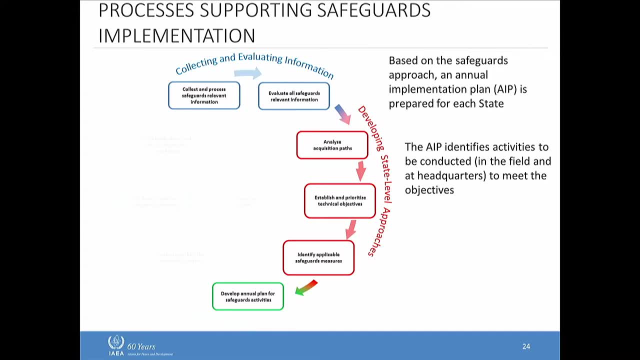 And this will help identify what activities we're going to conduct, which facilities we're going to go to, how often we're going to go to those facilities. Sometimes it gets into random selection probabilities of facilities And then, after we conduct those activities, 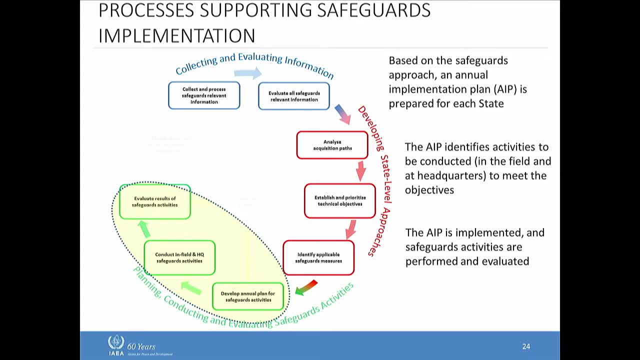 inspectors will come back and I think I mentioned earlier we have those results. They verified the new material, did the book audit, check records, things like that, and came back And if everything's consistent, that's fine. That's an acceptable inspection. 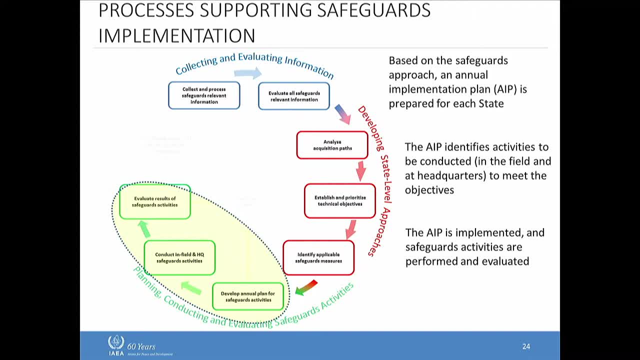 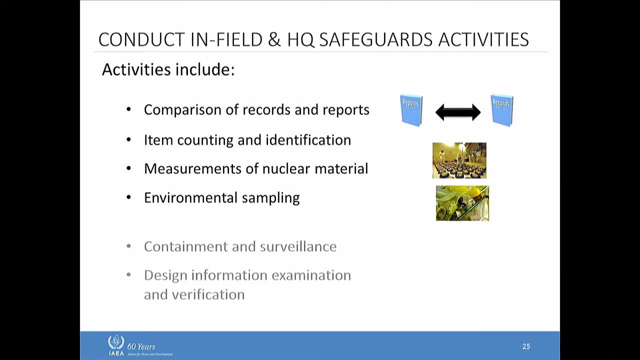 But if there's any issues, they'd have to follow up on it. So this is what we refer to as this whole conducting and evaluating activities. So let's go back to that a little bit, And these are just some common activities that we do during inspections. 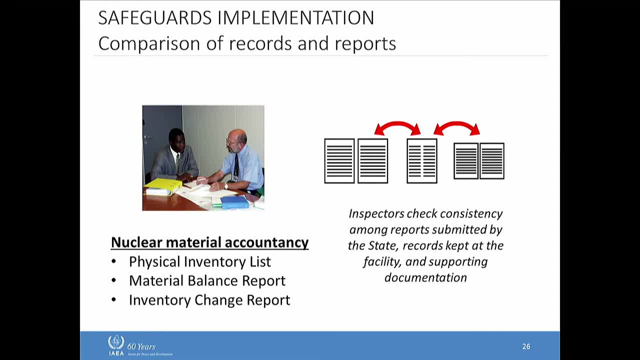 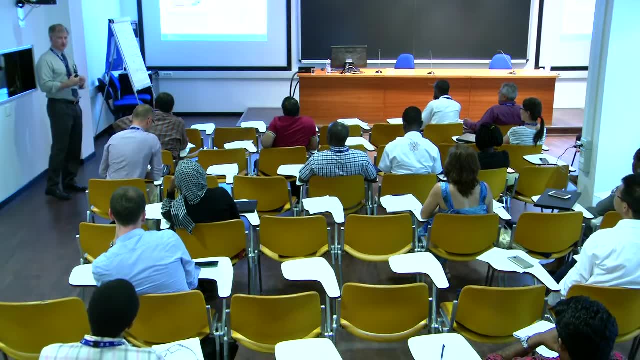 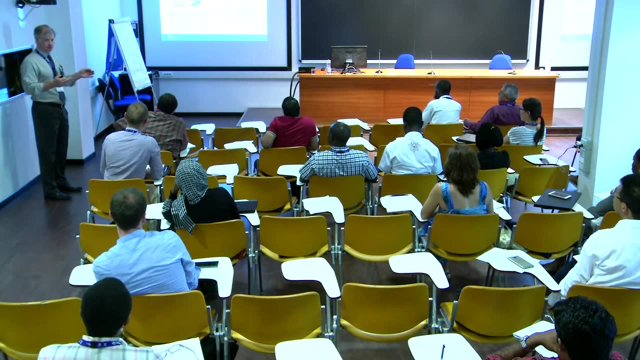 So I'll go through these one by one. We compare records and reports. So I talked about that. the state is obligated to submit a report, let's say a physical inventory listing or an inventory change report. When we go to the facility we'll actually check the books. 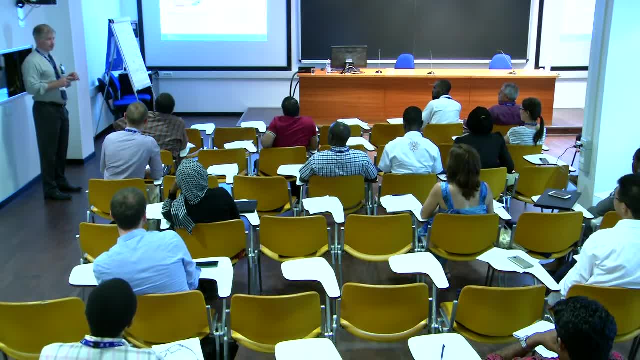 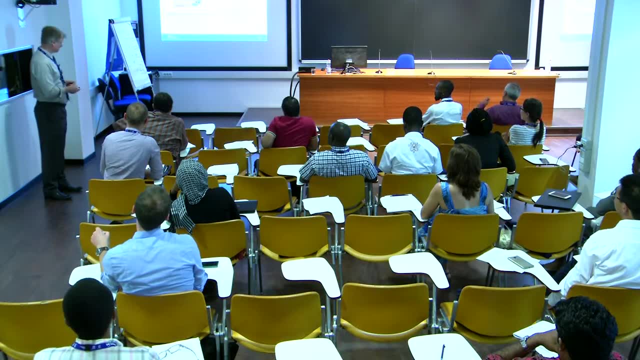 Oh, they could be smart and they could cook the books and they could be consistent with the paperwork they submit. everything could add up. But if there's paperwork involving a separate state, that gets a little bit harder to cook the books. 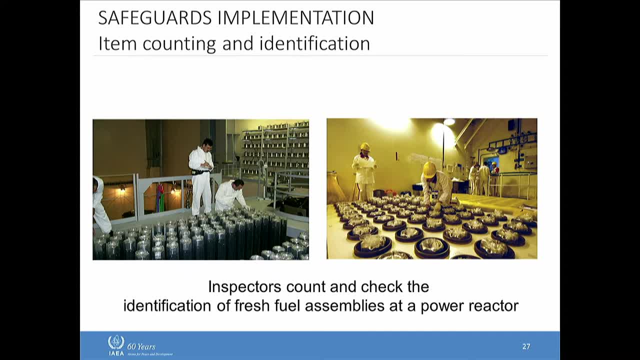 But we do a little bit of what we call book auditing. We actually verify the nuclear materials. So here you can see some inspectors. This is a fresh fuel storage area, So it looks like they're doing what we call item counting, so physically counting how many assemblies. 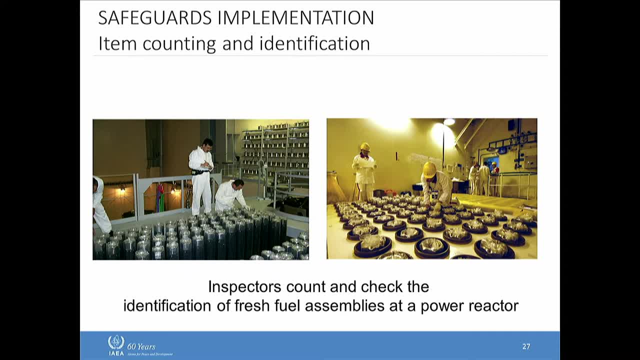 checking serial numbers, because they may have serial numbers that were provided by the manufacturer that might be in a different country, so they can corroborate that information. And then we also, in addition to just item counting, we can also assay and take measurements. 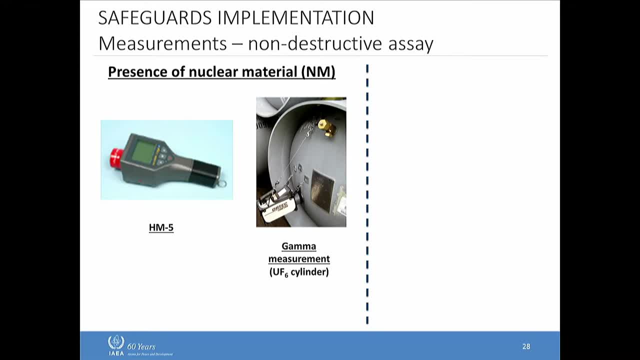 of the material. So here are some instruments. It's a common one. We use HM5, handheld portable. This is one for measuring UF6 cylinders, And these can get more precise and more accurate. This is a very gross method. we call it. 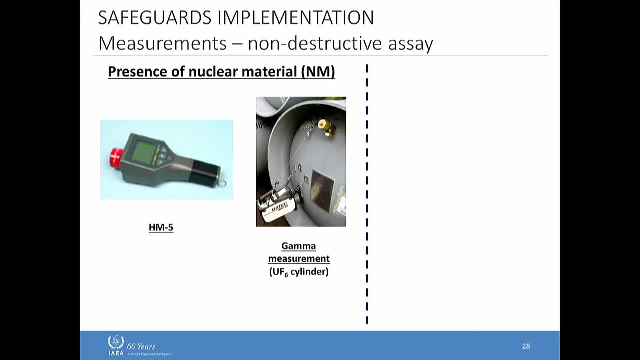 Is there nuclear material in the drum, in the cylinder or not? And then we can get into what we call partial-type methods a little more precise, a little more accurate. We can start to get isotopics, We can start to get rough quantities of nuclear material. 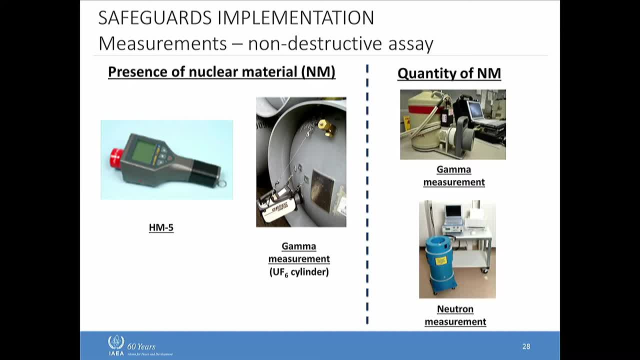 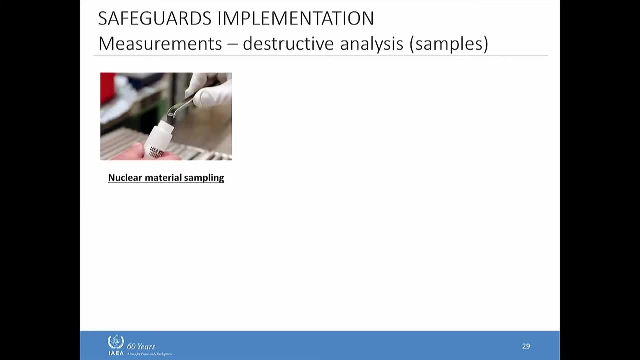 Sometimes the standard deviation's a little wide, but still we can get rough a partial defect test- we call it statistically- And then even further. I don't want to go into too much detail on this, but we can actually get destructive analysis. 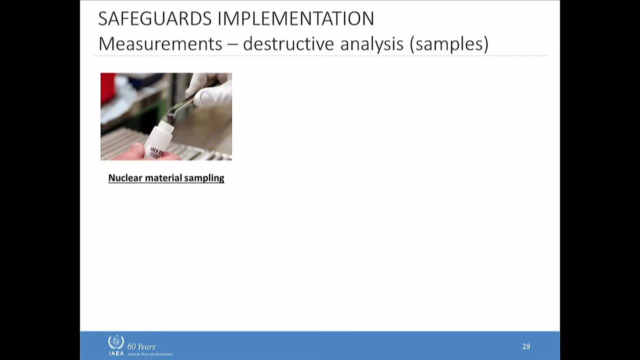 This is the most precise: If we analyze a pellet, tell exactly what that pellet was, or a sophisticated laboratory and a network of labs that do this for the IEA. And again, we can do isotopics for uranium, for plutonium. 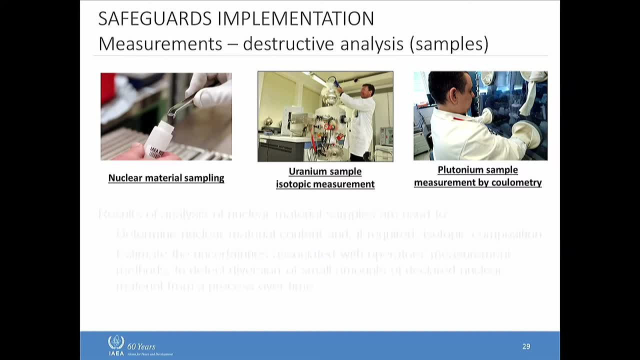 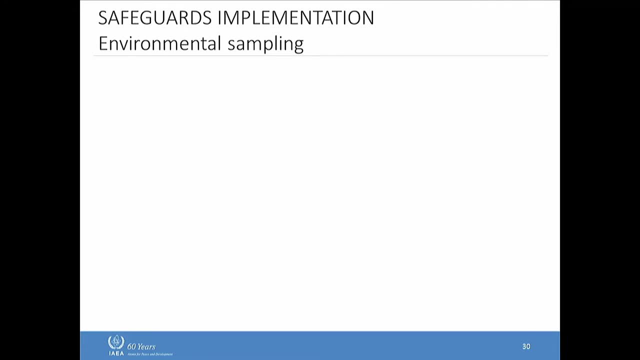 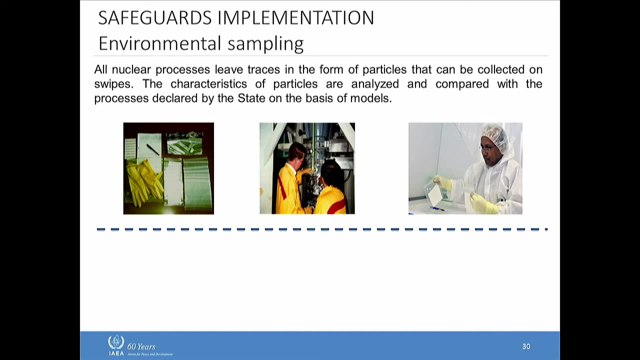 and the state would have to declare these isotopics and then we can confirm it. Environmental science sampling is another powerful tool we have. So this is basically a swipe, like a small square cotton swipe, and it usually comes in what we call a kit. 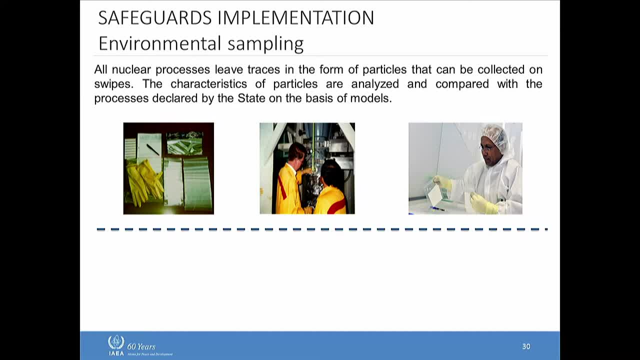 We usually have six, could be more. So go around and you'll swipe at strategic locations. So if I thought that undeclared nuclear activities may have occurred here and the state had sanitized the area and tried to clean it up and decommission everything and remove the equipment, 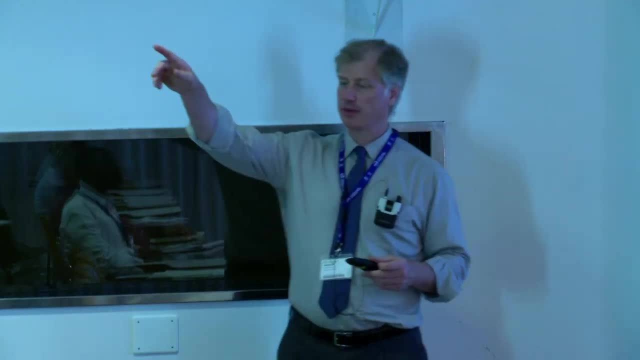 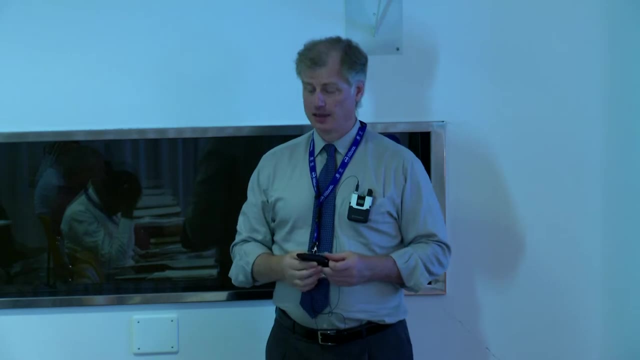 I probably wouldn't swipe the floor. I would probably take a smear of maybe the ventilation duct or inside the grill for the ventilation duct. The area is that it's very difficult If I thought that that might have happened. This is a very sophisticated 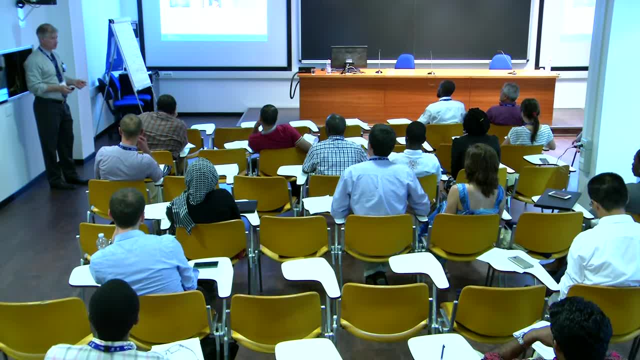 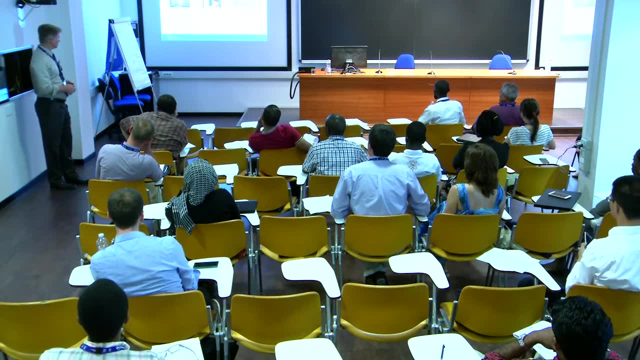 powerful tool because the state, if they do have something to conceal, they can sanitize and they can paint. but usually most nuclear processes leave a trace And this is a very sophisticated, very sensitive tool. Sometimes you can get false alarms, you can get cross-contamination, things like that. 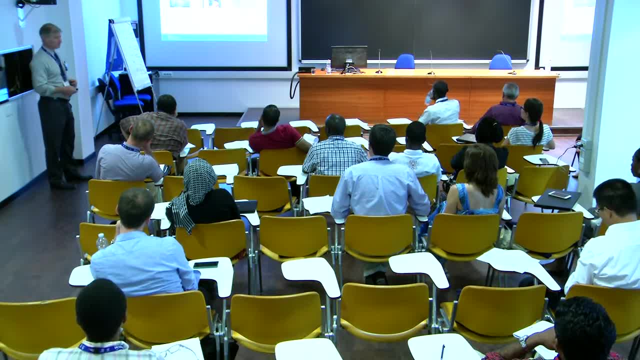 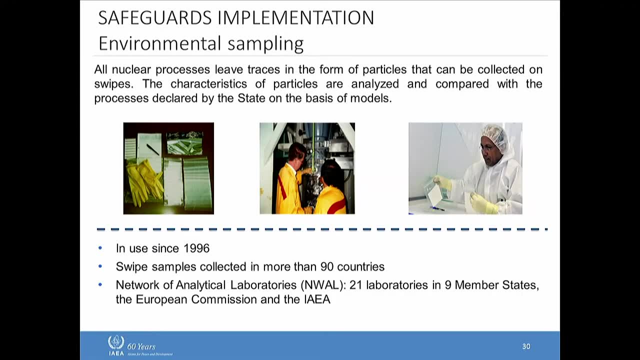 But it's a powerful tool for us in terms of detecting undeclared activities And actually it's been going on for a while. It's just sort of new Over 20 years ago. now it's pretty commonplace. We take swipes in all parts. 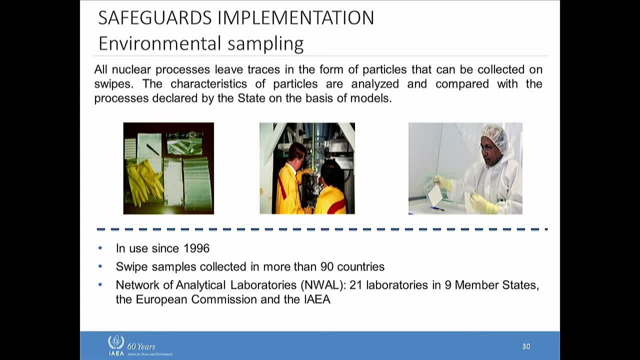 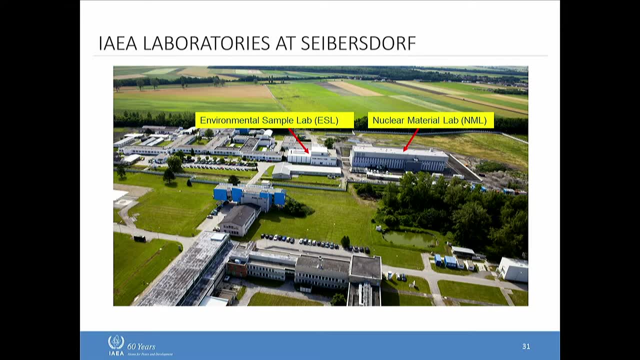 So it's sort of a standard part of agency practices. now Here's two of the laboratories we have at what we call SAIL, the Cybersdorf Analytical Laboratory. It's just south of Vienna And we have a material, a DA lab for destructive analysis. 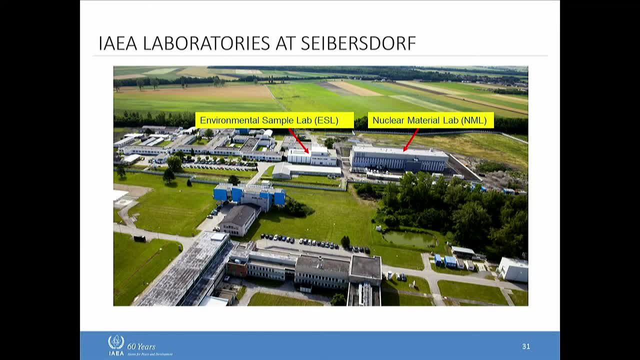 and also a swipe lab for the ES analysis, But we can also farm it out. We have a network of analytical laboratories that help out in several countries And generally for the ES. if it's not urgent, some of this is pretty slow actually. 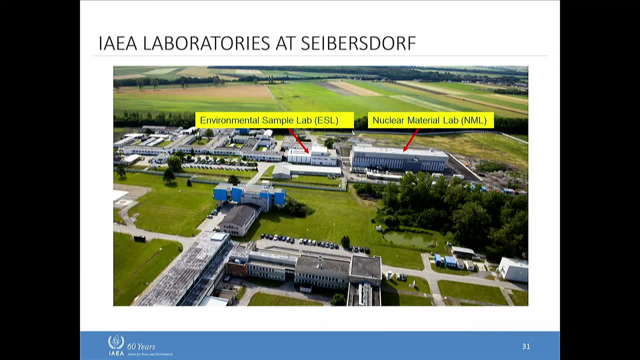 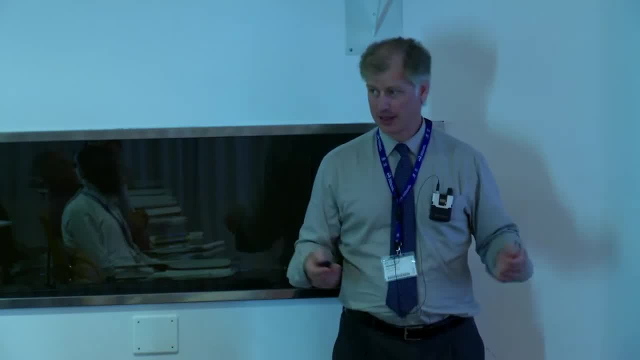 It could take several months for the results to come back, for it to be analyzed and evaluated. It's long and drawn out. Same thing for DA. samples can last sometimes months, But if it's urgent as opposed to routine, then it can happen in the order of weeks. 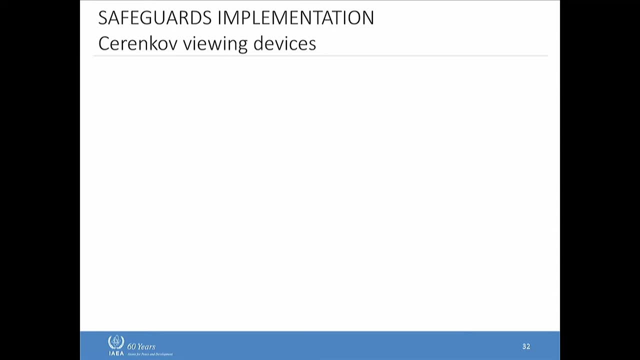 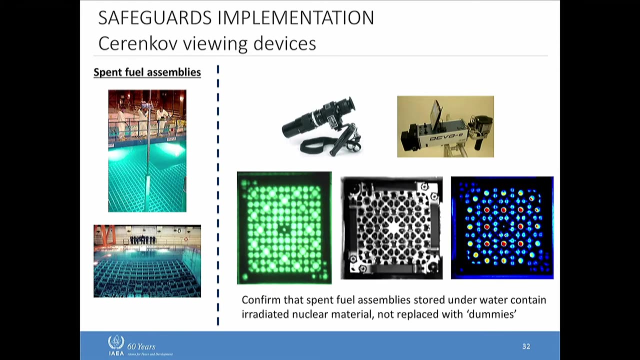 or a few weeks. We have other devices. I mentioned this fictitious fuel cycle we're talking about had spent fuel, So we have devices that can measure what's known as Cherenkov radiation that's given off by spent fuel Generally- if some of you have been at spent fuel ponds- when a reactor discharges, this is visible to the naked eye at first, Right away, for a few weeks, maybe in a few months. Then it tends to decay away For the frustrated discharge. you can see it, But after months or years. 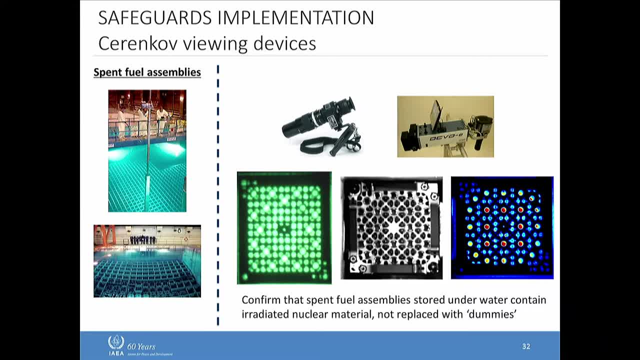 you're not going to see that anymore, but this instrument can pick it up. It can still pick up this Cherenkov radiation for years afterwards, Decades in some cases, if it's high burn-up fuel. So that's a tool. we have to verify spent fuel in a pond. 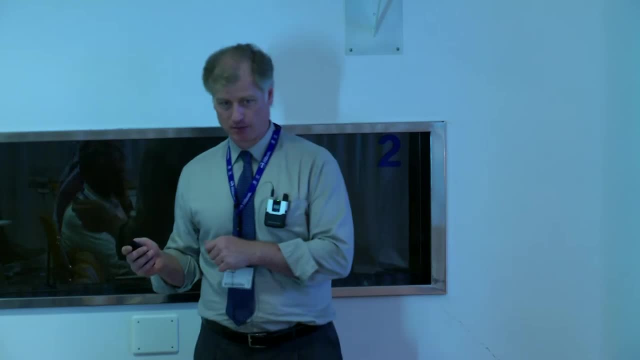 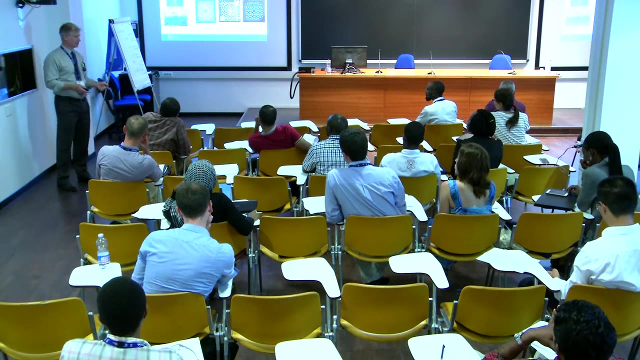 That fuel is indeed spent fuel, Because if they take an assembly out as part of that diversion step, well, they're not going to just leave it blank, because they'll probably say: well, you had 500 assemblies last time over here and now you have 480. 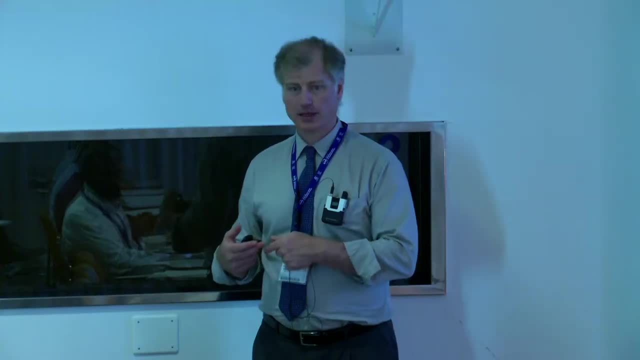 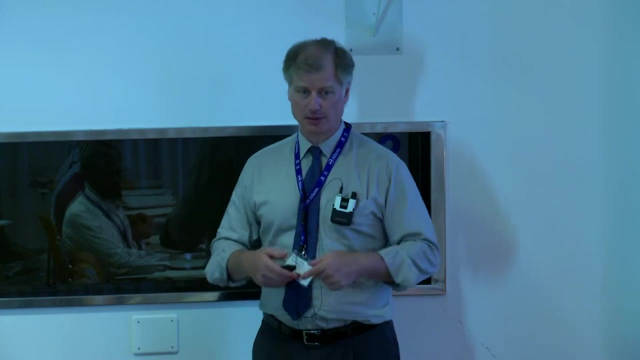 So if they did divert 20 assemblies as best they can, fabricate 20 dummies that look like those spent fuel assemblies, They probably won't have the same signature as the earlier ones that had plutonium and cesium and spent fuel and fission product fragments. 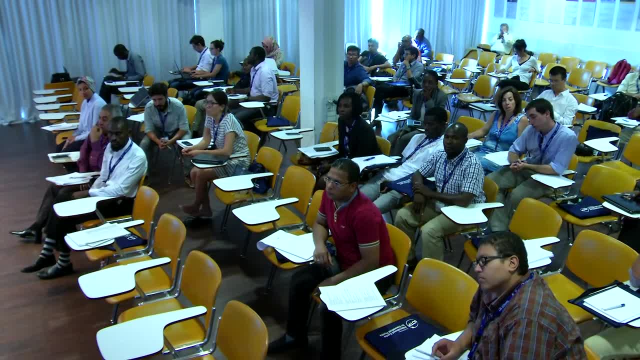 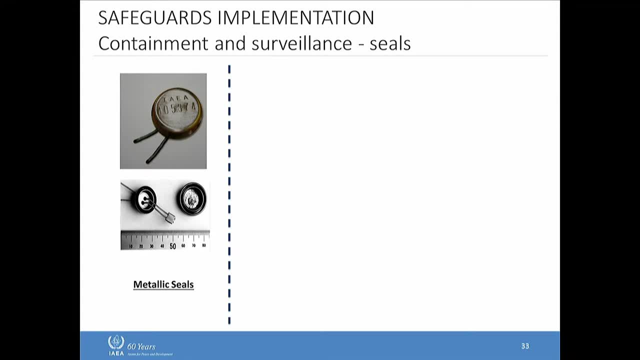 things like that that are giving off a certain gamma spectrum which we can detect with instruments. I talked about seals. We can apply seals. This is a fairly standard what we call a metal seal: Very simple, very reliable. We also have what we call in situ seals. 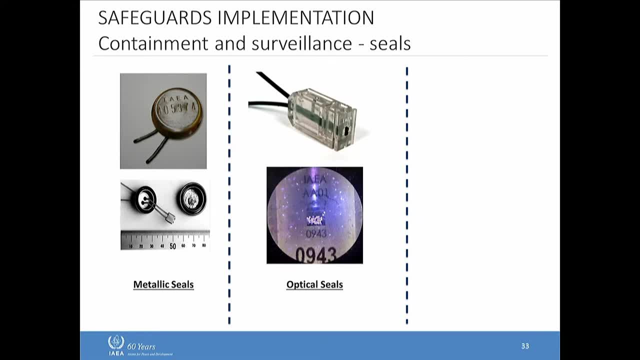 where you can verify them in place. This is what we call a cobra seal, And for this one I would have to detach this and bring it back to Vienna to have the inside of this seal checked and verified. This one I can do in the field. 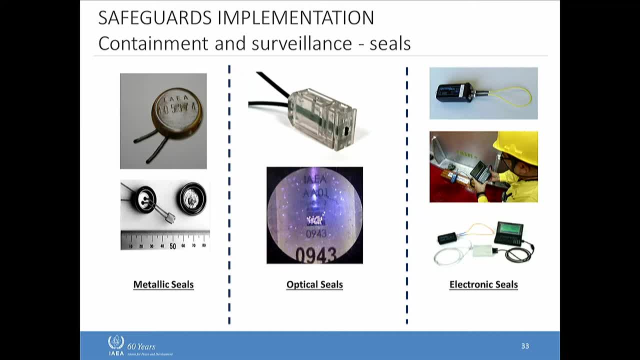 and this last one- electronic seal- can also be done in the field. So if someone opened one of these wires or cut this wire and you go to verify that seal, it would say there's some event, You can close it, But that's all saved in the seal. 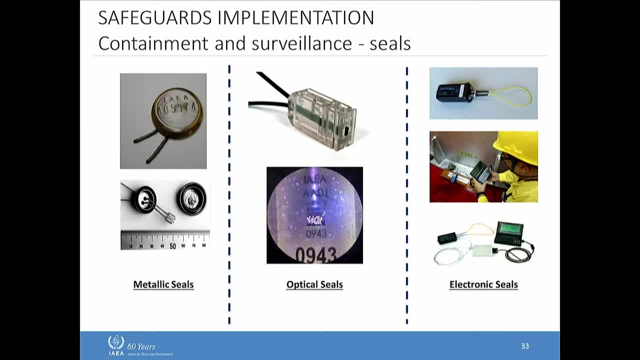 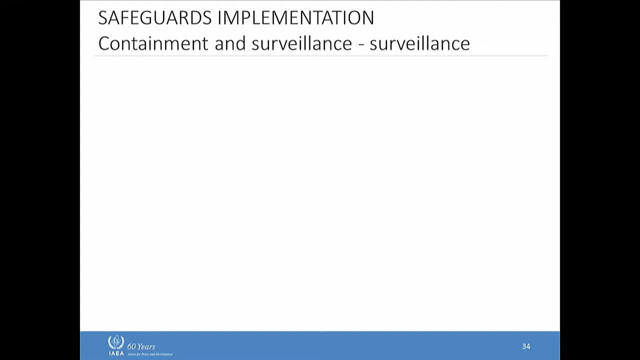 any kind of event like that. So you'd say, well, there was no inspector here who opened this seal, So again you'd have an issue or an inconsistency you'd have to resolve. We also have, we use quite a bit of surveillance. 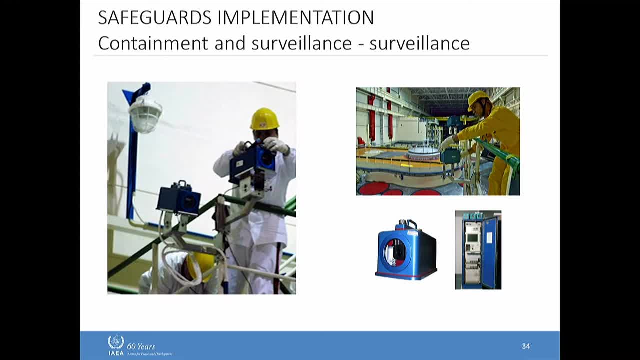 so cameras. So it's also the main purpose is to maintain continuity of knowledge. So they close up the core, they refuel and we may not go back there until the next refueling. So it could be 12 months, 15 months, 18 months. 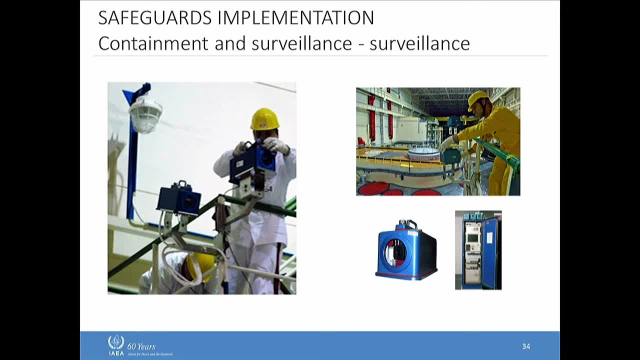 So we can install cameras overlooking the pond. They have a certain picture-taking interval, so they're not video cameras, but they can have short intervals And then we can come back later and it's saved on a storage media. We can take the media out, use software to review it. 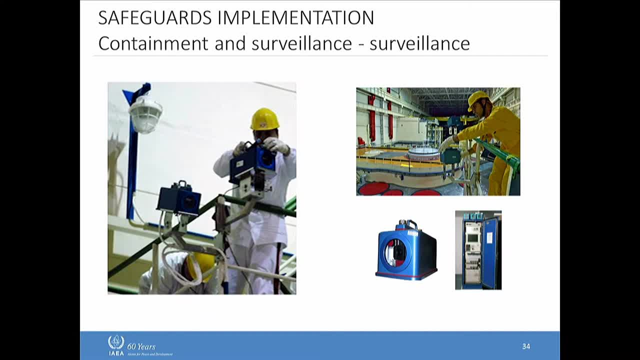 and see if it was an uneventful closed-core period. if nothing happened, We don't expect much Now. during a refueling period, there's a lot of activity as components are removed, but during a closed-core period you don't expect that much activity. 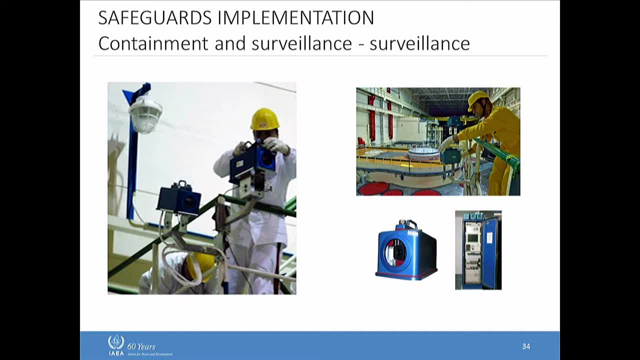 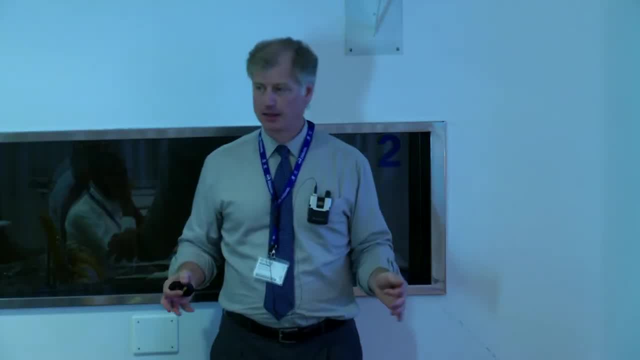 So anyway, just another way to maintain continuity of knowledge. And if something unusual, if there was a cask that came in and a cask that came out and that's on surveillance and the operator in the state told us nothing about it, that would be an issue. 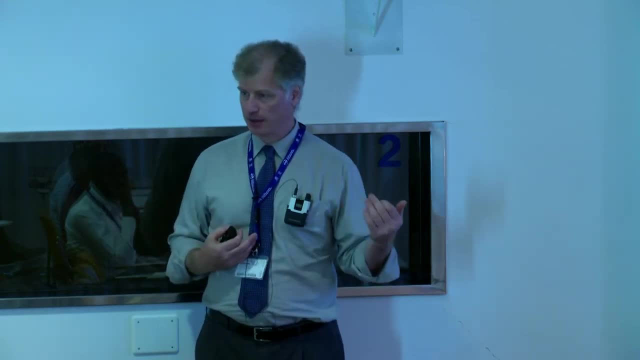 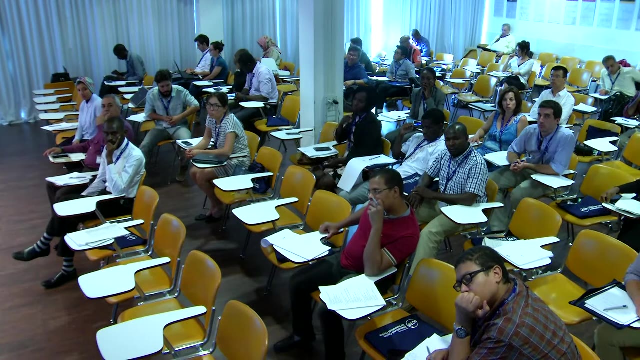 That would be an inconsistency. We saw a cask come out on our camera. he didn't tell us about it. it's an anomaly, we'd have to resolve it. So we'd have to go verify that pond again. Even if it was accidental, they put a cask in. 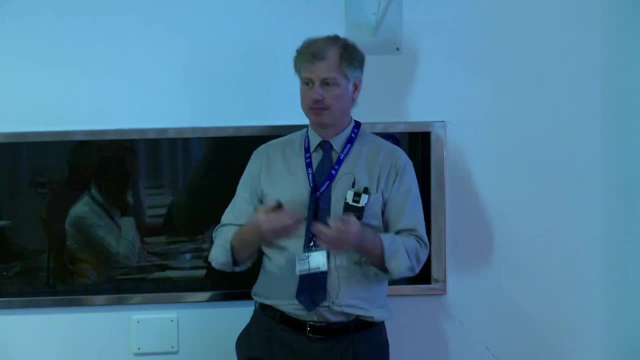 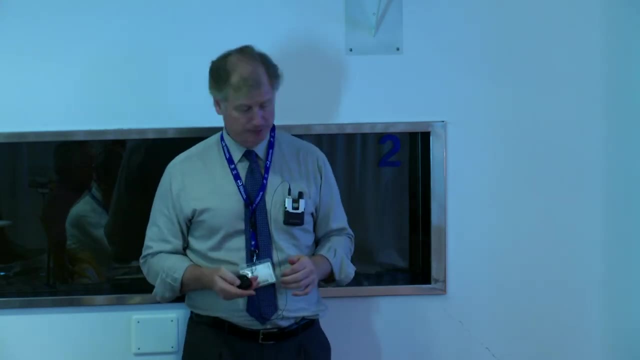 and for some reason, training or something we didn't get- to verify that that cask was empty when it came out, Because these cameras can see the top of the pond but they can't see underneath the water. I talked about design information verification. 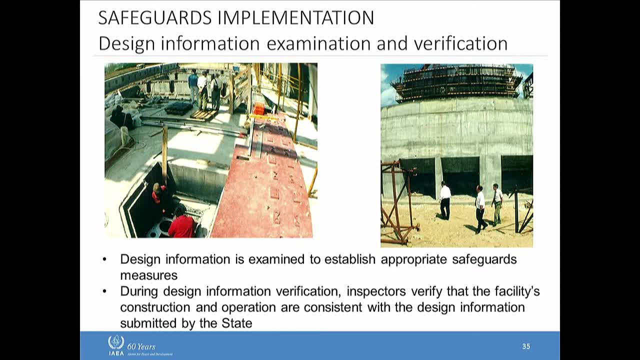 We can actually go through all phases of the life cycle. so when they're under construction, commissioning, that's the best time to go actually to crawl around, because nothing's hot yet You can get a pretty good understanding of how the facility is designed to operate. 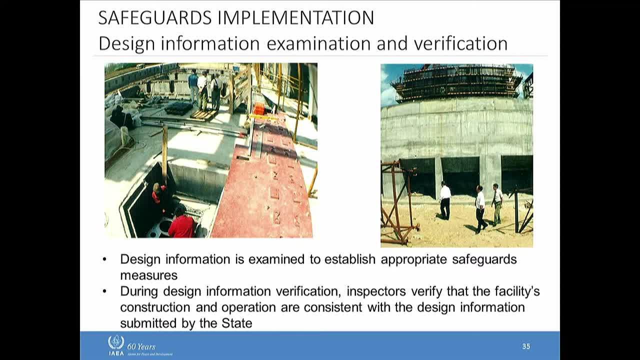 So we're just confirming that, even all the way through to decommissioning, We're validating our safeguards approach. Where are we going to put these cameras? Are we going to seal the core? Are we going to seal the equipment hatch? Things like that. 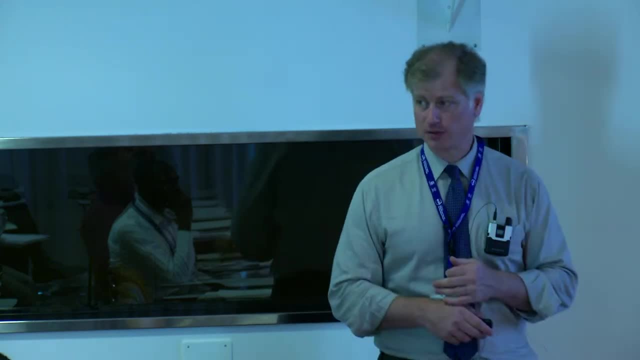 As I mentioned earlier, if we can do this earlier in the process, if there's a new design, if you're talking earlier about the Generation 4 designs, if some of these new fangled fancy reactors came out like fast breeder reactors. 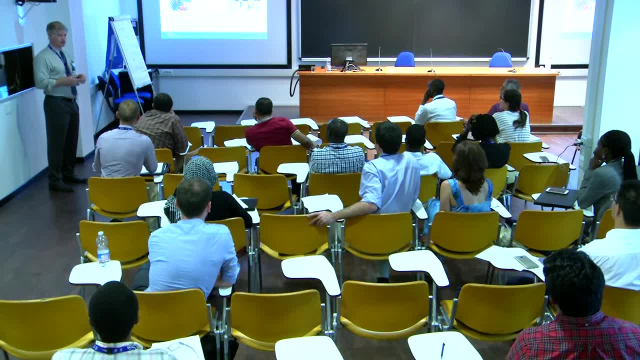 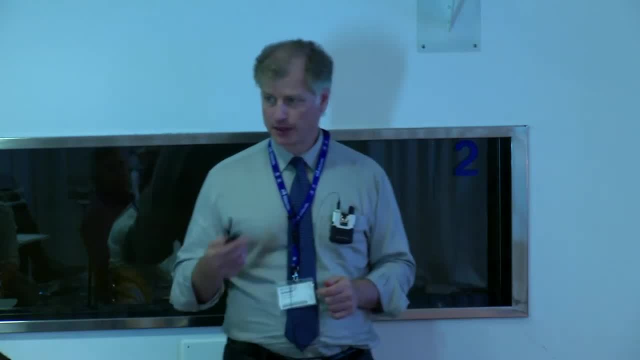 actually there's one in Japan, Manju, but other than that there's not too many, but they're very complicated to safeguard. So the earlier we can get involved in that process, the more optimal the safeguards measures are on the road when it finally becomes. 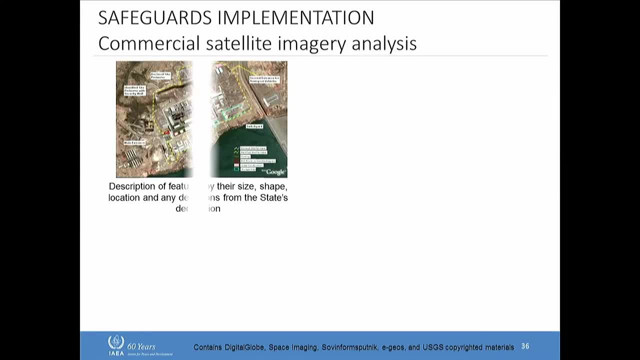 you know, under construction. when it's under construction I talked about commercial satellite imagery- Oftentimes we'll get a declaration from the state, of sort of a sketch of what their site looks like. site declaration of buildings. Well, satellite imagery- the analysts can actually overlay that. 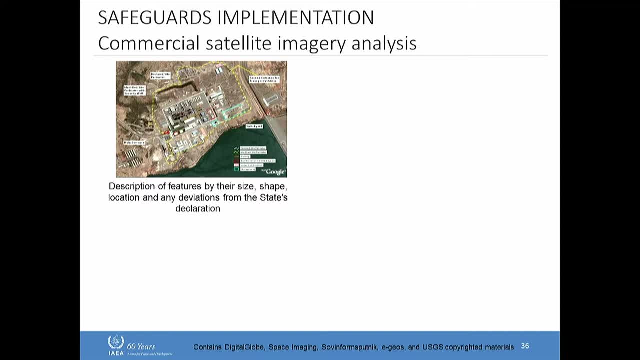 onto the actual imagery. I think you see this on your iPhone now some of the GPS technology, But they can see if there's a really quickly it'll tell them that there's a building that's not identified. It's not a satellite declaration. 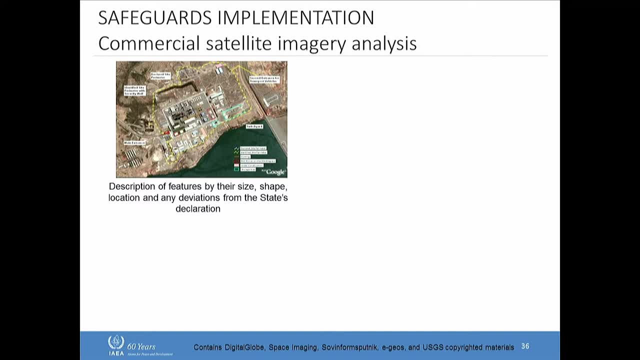 but it's the overhead imagery. Some sites can have hundreds of buildings, some small, some large. It can be a little bit misleading. I've been on CAs where I was told there was a building and I went to that area. 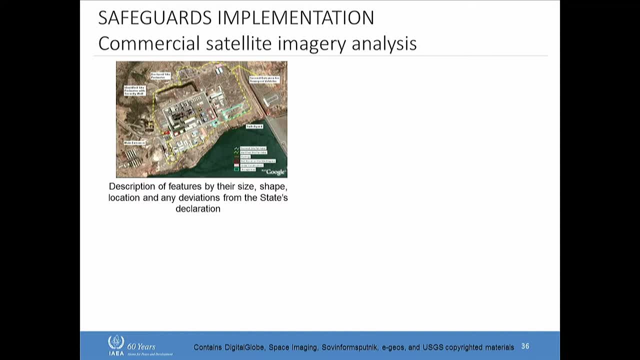 and I couldn't find the building and I finally realized it was basically a bicycle port that had a little roof on it like a tin roof on it. So at the ground truth level it wasn't a building at all. I was like: where is this building? 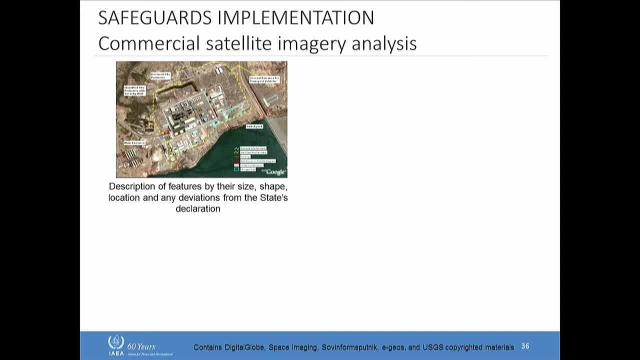 It was a bicycle or something. In that case it was nonsense. So most of these you can resolve pretty quickly. The other thing: satellite imagery can help you to look at change detection over time, if the facility's under construction or if they changed it. 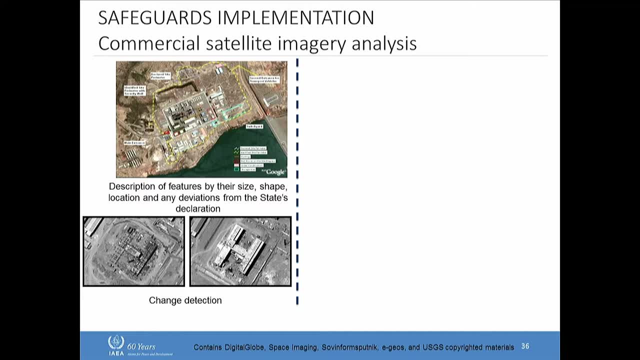 if they were trying to get rid of the facility or clean up the area. There's a case with Syria like that, with a probable reactor which was bombed but then it was sort of cleaned up and sanitized and buried basically. So you can augment it with other types of 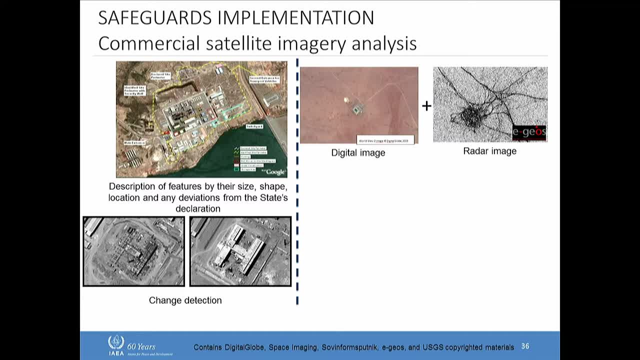 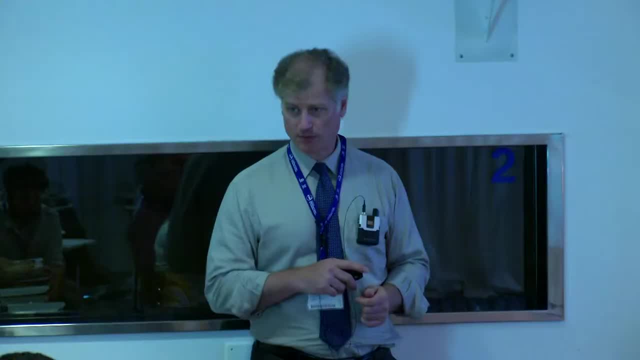 if it's a cloudy day or whatever, you can use radar and things like that from your satellites to also augment it. So this is very advanced. now There's also quite a few commercial satellite providers, So this is pretty exotic, definitely 30 years ago. 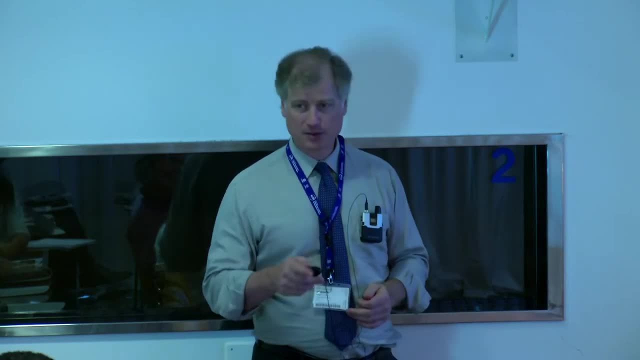 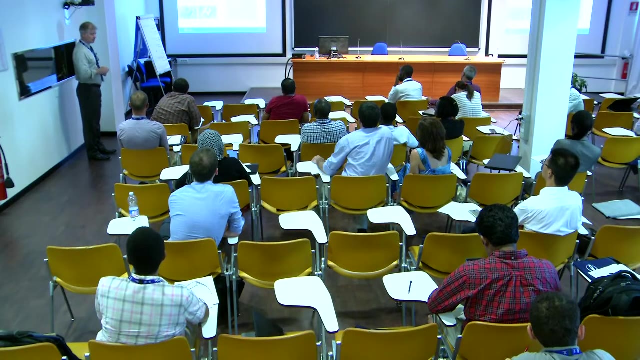 probably only a few states had the capability but now there's a lot more satellite imagery commercial providers. There may still be some restrictions from the states where those companies are operating from, but generally there's a lot more commercial satellite imagery down quite a bit. 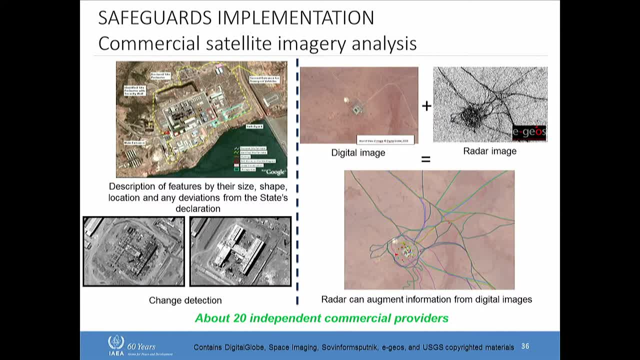 I just mention it because it's a very powerful tool. It's also a tool the state may not know that we're using. They may not know exactly when the satellite is going to be overhead, and some of them are taking pictures at angles. 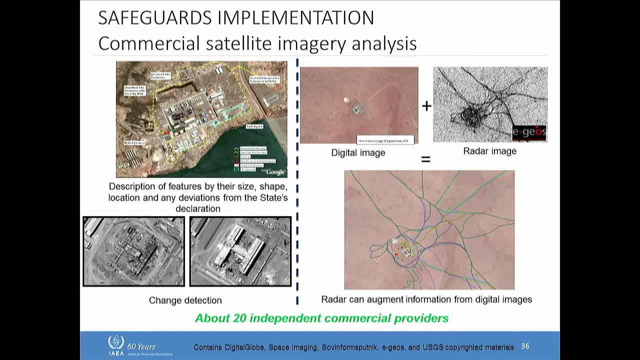 and my understanding is now it's so fast that it's almost like, in some cases, like a short video of the area they're trying to take pictures of. So overhead imagery very powerful tool and it may drive some potential proliferators underground. 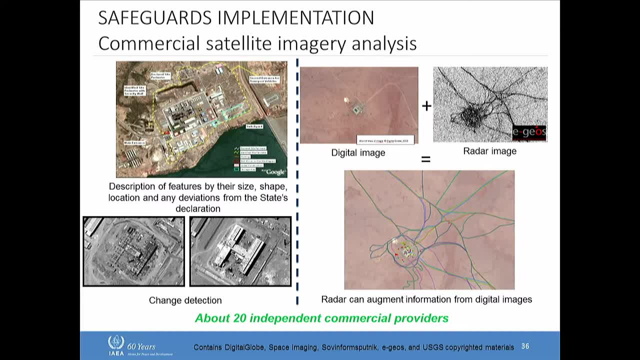 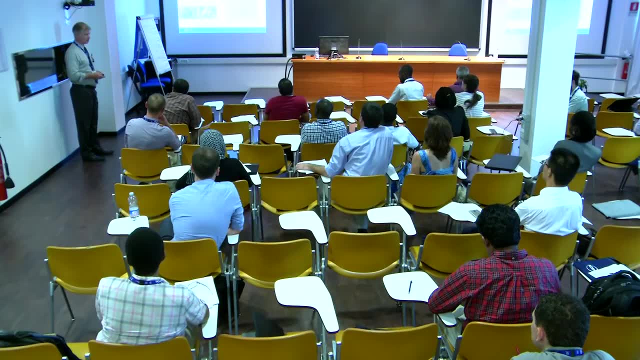 That's something that's noticeable on the surface, But that digging and stuff could also stir up an indication. But I should say you'd almost have to have some kind of location-specific information, unless you have a small army of people and analysts to do this. 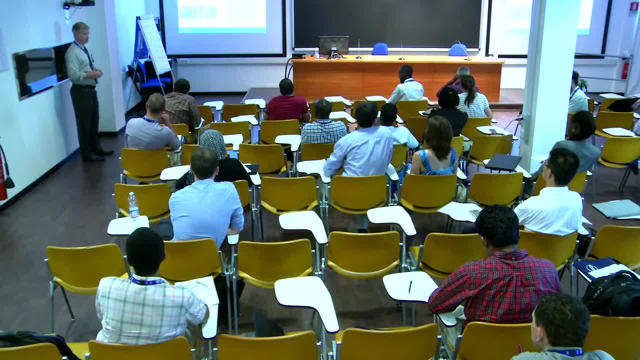 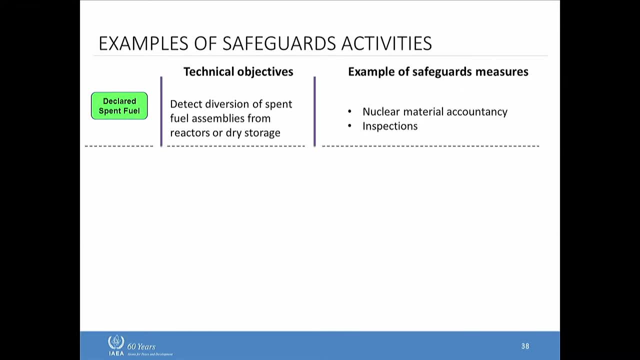 So the agency would probably need some tip or location-specific information in order to focus a commercial satellite imagery on a certain section of the country. So, returning to our path and our objectives and our measures, So for safeguards activities we've declared spent fuel. 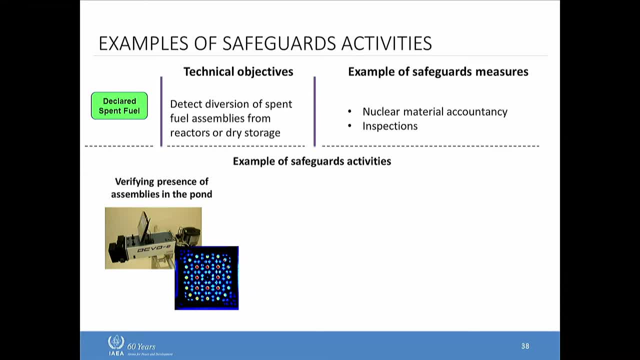 So I mentioned a bunch of these. We could do things like measure the spent fuel with an ICBD, this Turenkov fueling device. Make sure it's spent fuel, that it hasn't been diverted and replaced with dummies When a state transfers. 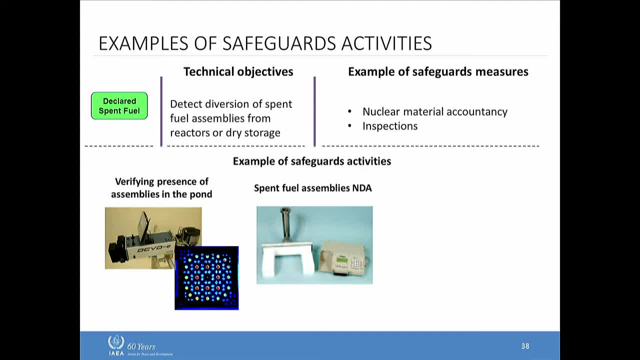 their spent fuel to dry storage. we usually verify it with a different instrument. This is a fork detector. They actually underwater. stick the assembly in there and this will measure the gamma-neutron counts and can determine roughly based on burn-up. 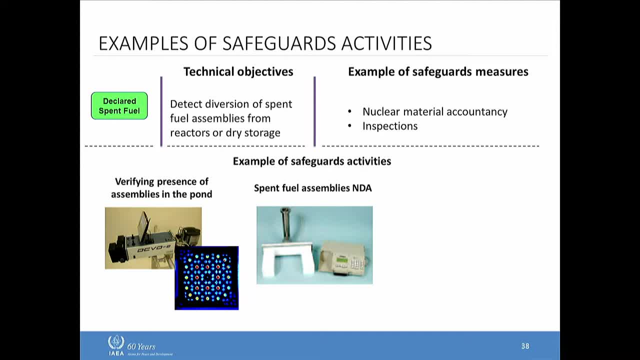 how old that assembly is. So that's spent fuel and almost not so precise, but roughly when it was discharged and cooling time, things like that. And then I talked about the seals and the surveillance. So that would be part of normal measures. 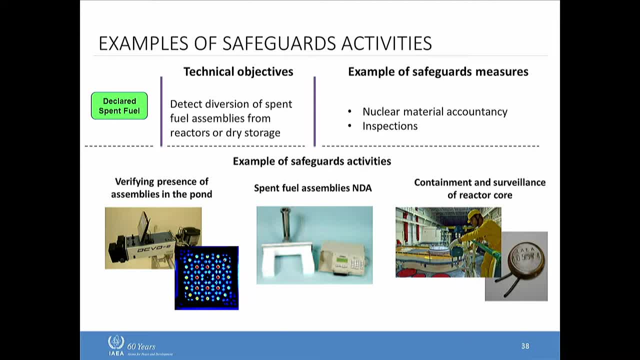 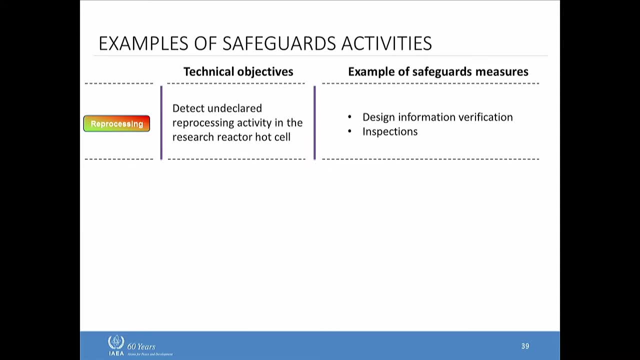 to cover this spent fuel step. So if these are coming back, fine, that spent fuel hasn't been diverted. we're happy from a safeguards perspective. The reprocessing step with the hot cell. So some measures and activities we could do. there would be things like: 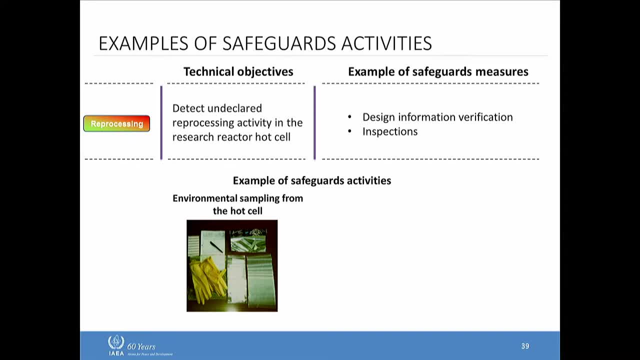 the environmental sample We could take a smear inside the hot cell. It's usually done with remote manipulators But usually a hot cell will have a certain signature in it And usually we've done a baseline so we're familiar with that signature. 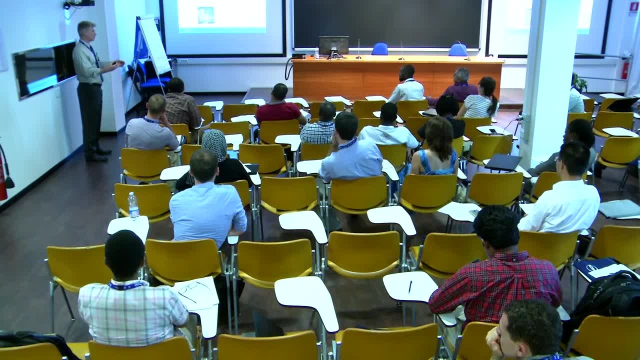 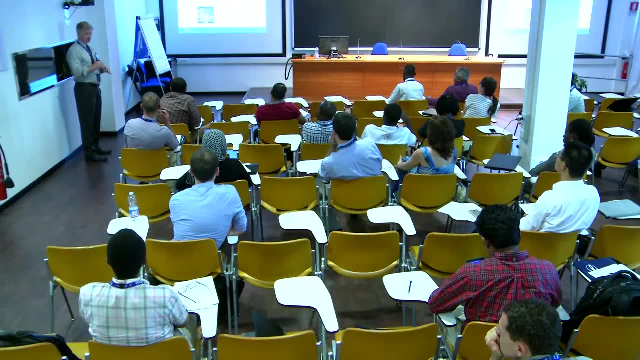 and it's in the agency's database. So this is a type of signature that you'll see in this hot cell. So if we take another hot cell a year later, two years, three years, five years later, we'll see an entirely different signature. 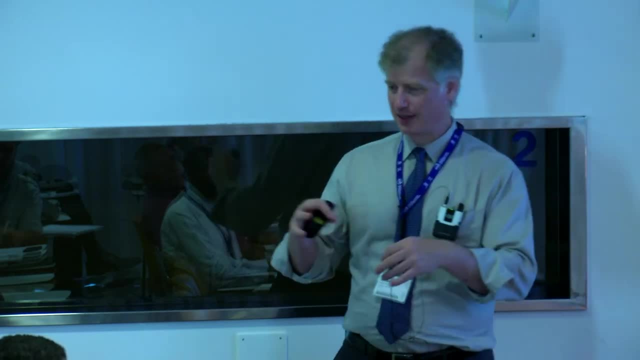 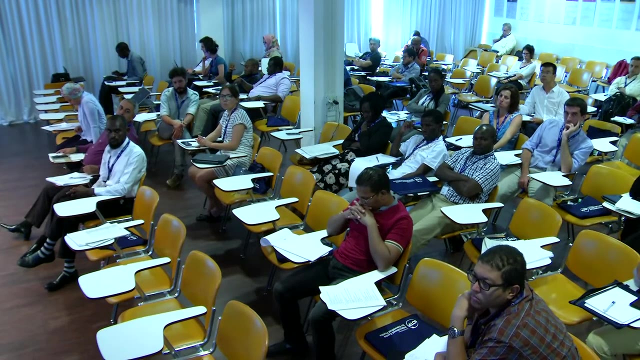 that maybe is indicating we're not really doing medical isotope production. Now we're getting hits and particles that are related to plutonium separation in this hot cell And we'd have to ask: why is that? So again, we'll come back from these laboratories. 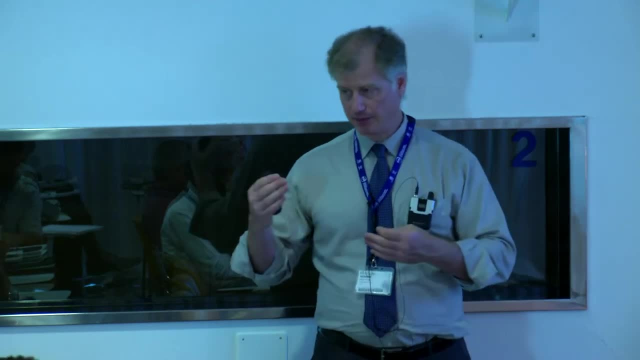 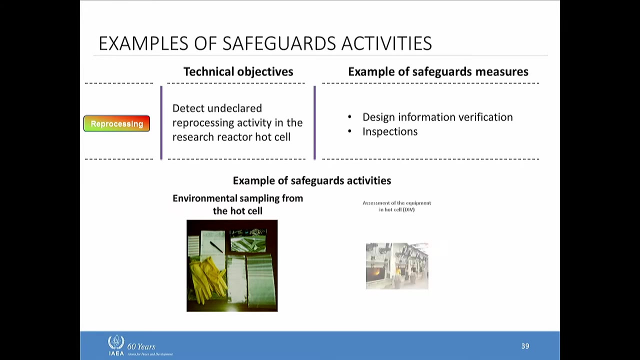 There's evaluation people to look at what's expected, and very detailed. It's a very powerful tool in this environmental sample. And the other thing we could check in this hot cell. we could just physically look inside the windows If we're familiar with the reactor. 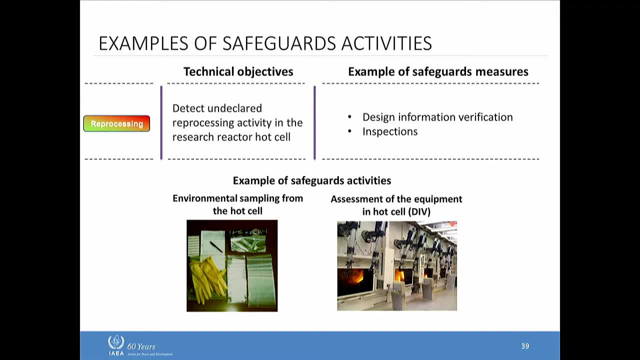 operation, let's say the research reactor. if we look in their hot cells we should see the same equipment: the glassware, labware chemicals that are used for the medical isotope production. It should be a relatively small-scale operation. 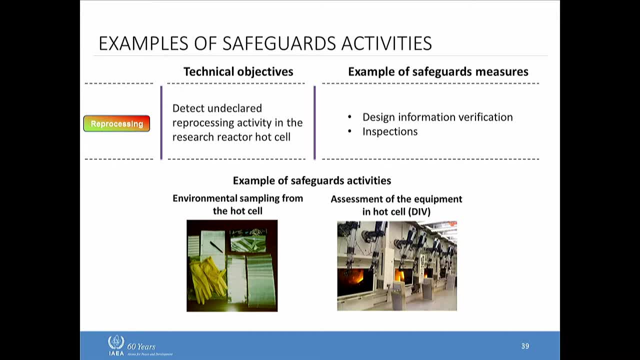 And if they go to plutonium production mode, I expect the equipment would change a little bit. It may not be large, I'm sure the unit operations would change, the chemicals would change. You have to kind of mask that, But something would change inside that hot cell. 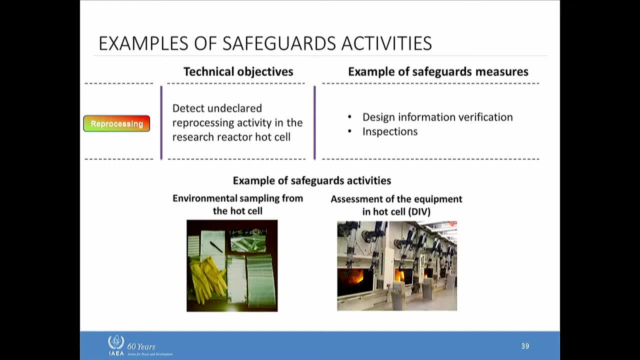 So you could even take a picture of normal and the inspector could come back a year or two later and say: okay, I see roughly the same layout inside that hot cell. It's not drastically different Because a lot of times inspectors can't be familiar. 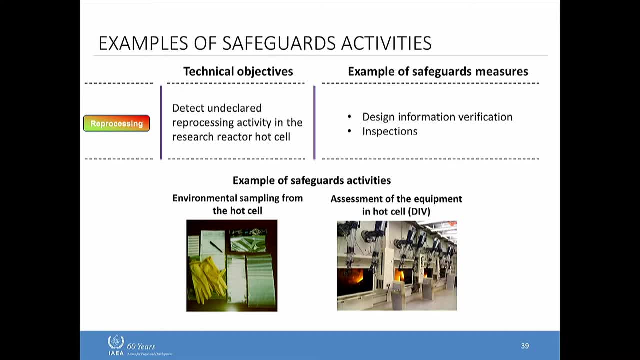 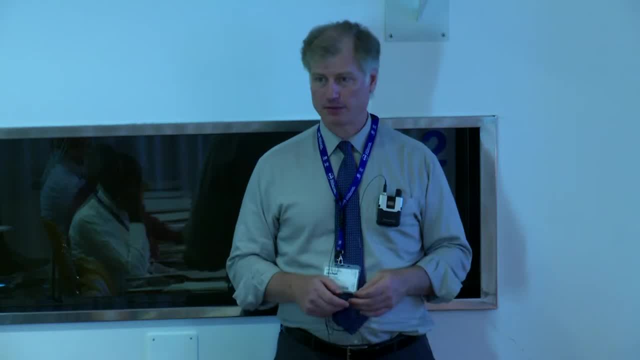 with every type of operation and they're going to different facilities all the time. So these would be two activities we could do to make sure this hot cell is not being misused- and hopefully it isn't- and we could conclude that the facility was operated as expected. 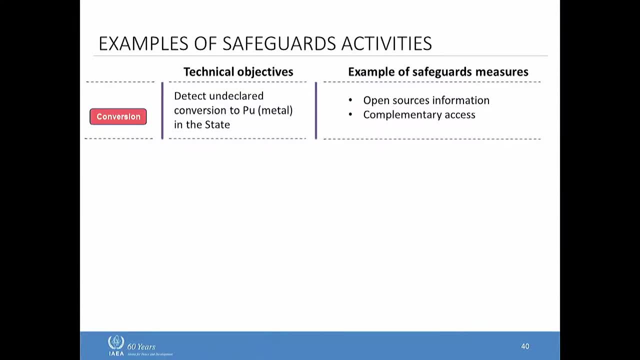 and, as designed For this conversion step, it's a little trickier because, as I mentioned earlier, it's probably not going on. we're not going to know where it's going on unless we have some location, specific information to indicate the location. 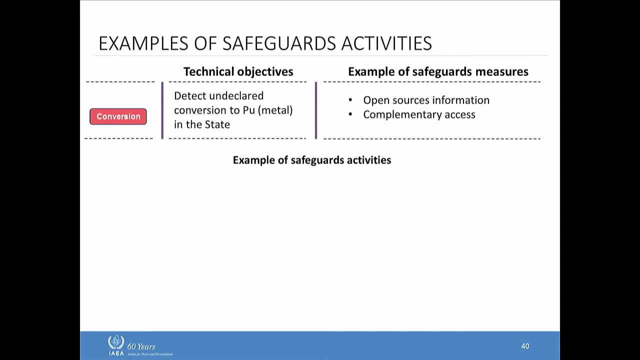 So here we rely more on what we call open source. That someone might write an article in a journal related to plutonium separation or metallurgy, and that's highly unlikely because the program would probably be very, very isolated. But in the event they did. 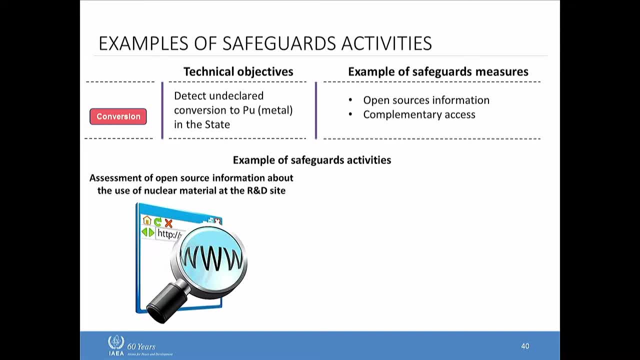 in a research mode, that might be an indication. So things like open source type information Generally, if you're seeing- I should say if you're seeing- a lot of open source, that would be that's one thing. but if all of a sudden that information was cut off, 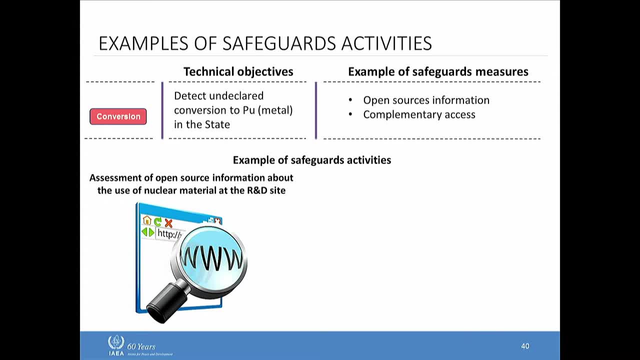 and dropped off or turns to zero, you'd say that might actually be suspicious. All of a sudden you had a lot of information in the research and then it just dried up all of a sudden And we could also do what I mentioned- that the complimentary access. 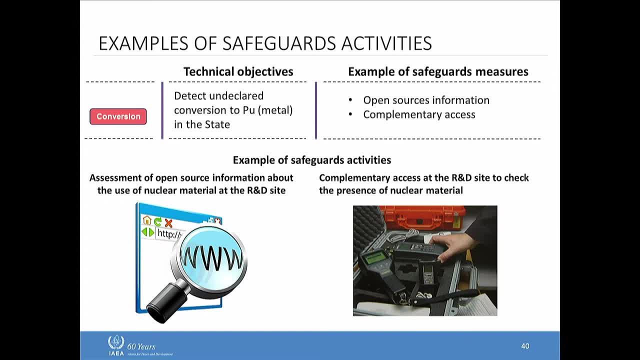 where we can check a site, we can bring instruments. There shouldn't be any nuclear material in this room. I could just go around and make sure that's the case, But again I'd have to have a location. I couldn't just scour the country. 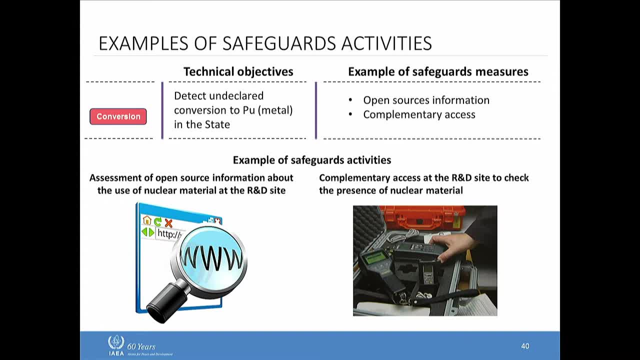 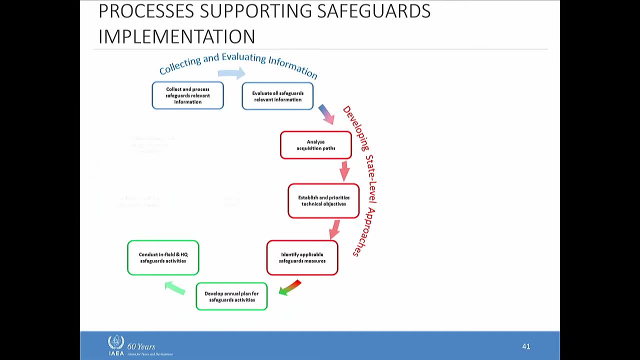 walking around aimlessly. I'd have to have some information on where to do the complimentary access, So we talked about these three sides of the wheel. Now we get up into this, information comes back, we evaluate it and we have to resolve any differences. 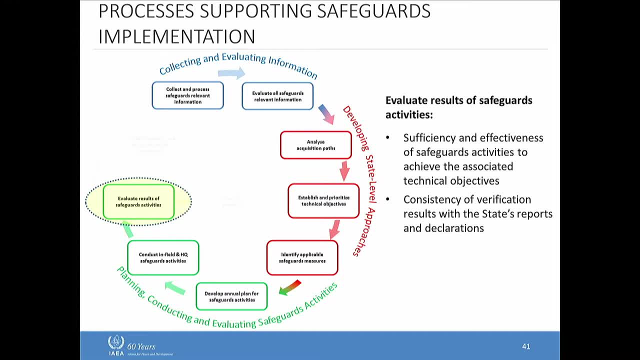 And we have what we call safeguards findings. And did our findings support our technical objectives? That part, on this side of the wheel, establishes technical objectives. Did we actually meet those technical objectives? Did we have any inconsistencies, any issues, any anomalies that have to be resolved? 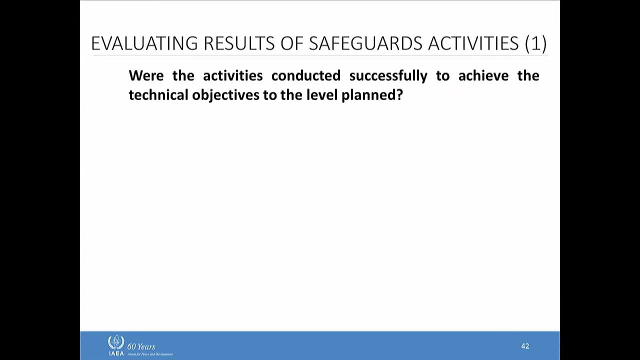 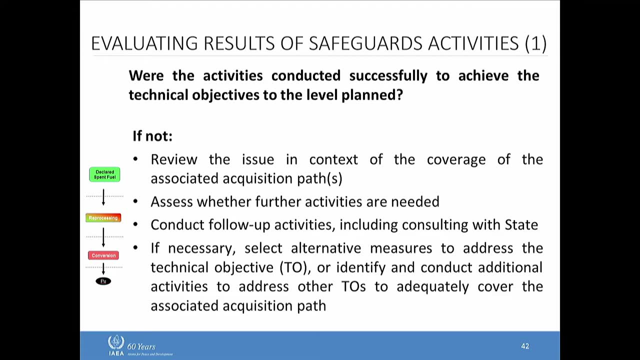 So we evaluate the safeguards activities. Did we meet our technical objectives? If we didn't, there might be a good reason. Maybe they had a safety mishap at the facility and we couldn't get access, let's say here at the hot cell. 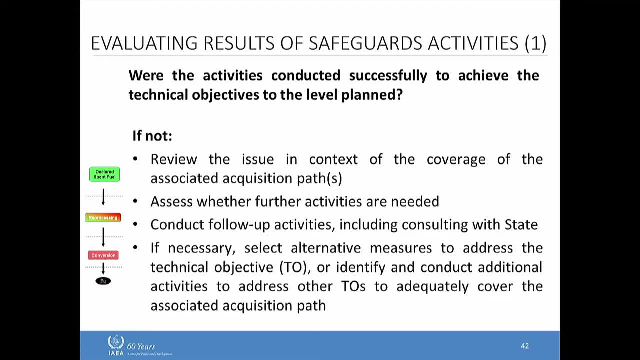 Well, it's a problem if we can't get access like we expected, but there could be a legitimate reason for that, A legitimate safety reason. So we could either wait and wait until the mishap is over and come back in a few months, or we could be more upstream. 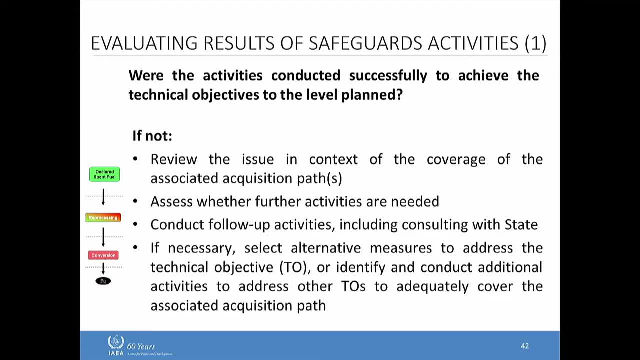 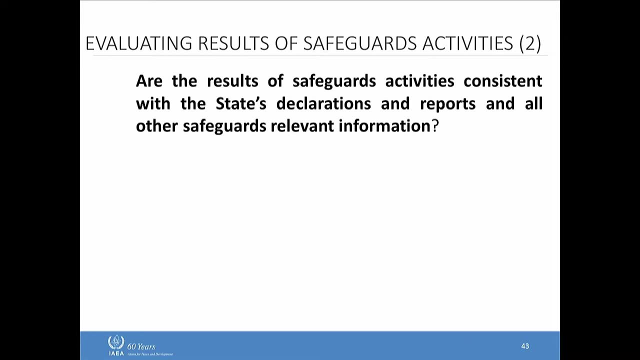 be more assured that this go visit the pond, the spent fuel pond, sooner than we had planned on it, So we could change our plan in the event something comes up. And again we're always looking for consistency with all the other safeguards, relevant information we have. 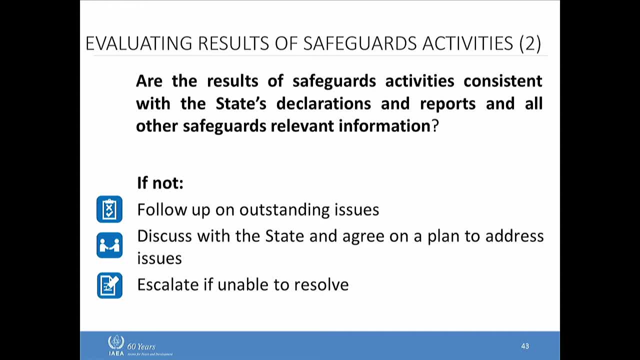 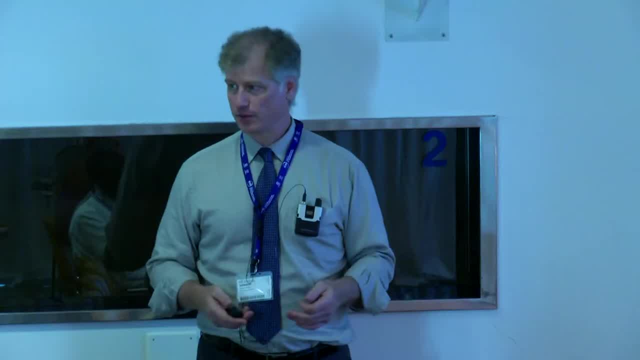 If there's inconsistency, if it's minor, it usually can be worked out at the facility level. If it still can't be resolved, it usually gets elevated and the inspector will usually call back to Vienna and inform the senior inspector. the section head, the director. 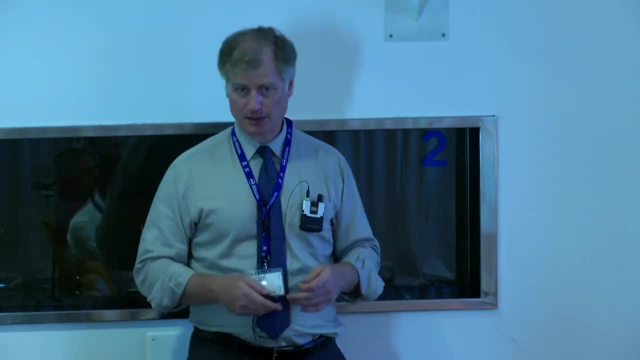 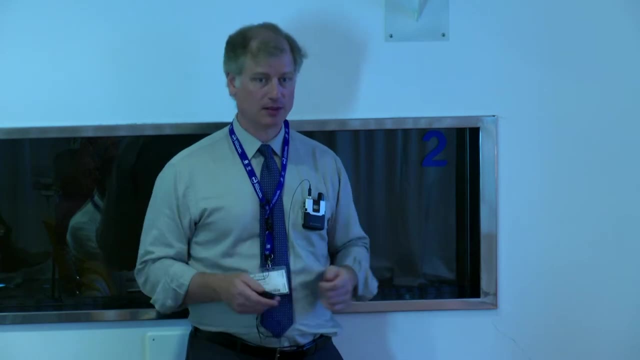 depending on the nature and magnitude of the issue. If it's a very serious issue or a serious anomaly, like if the inspector was denied access, if there's new material that's missing or equipment has been interfered with or tampered with, and other. 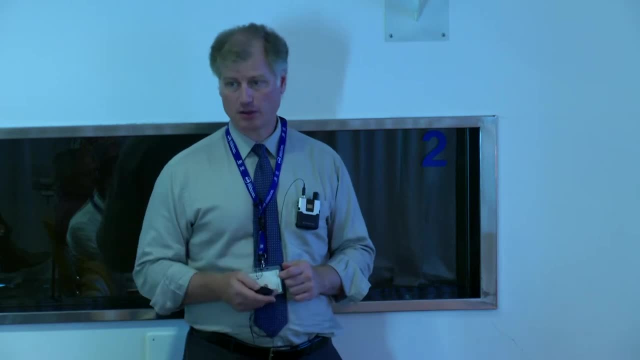 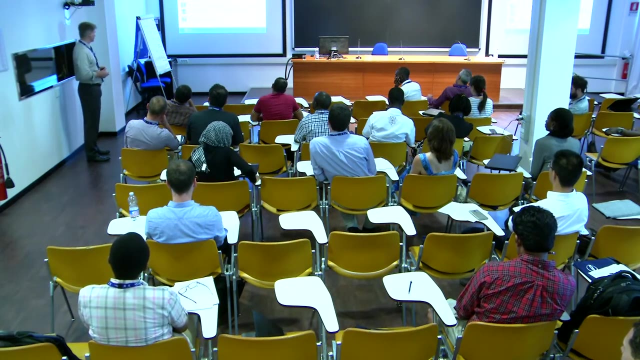 indicators, then it can rise to a much higher level. It could go to what we call the DVG DG and eventually to the Board of Governors, which would have to be a very serious issue. So hopefully these are resolved mostly at a much lower level. 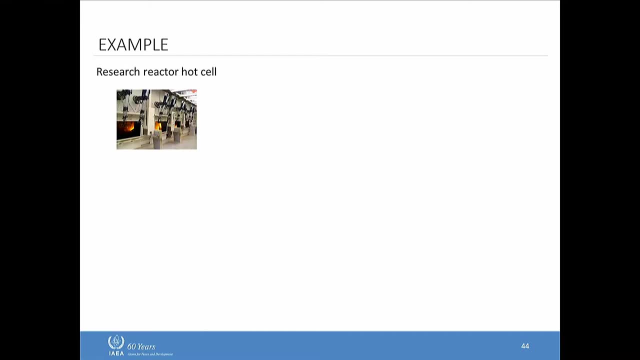 I'll just give you an example of how one might be resolved. So we talked about this. we have this research reactor hot cell and the state declares that they only deal with low enriched geranium in this hot cell. but if you're taking a sample and it goes to 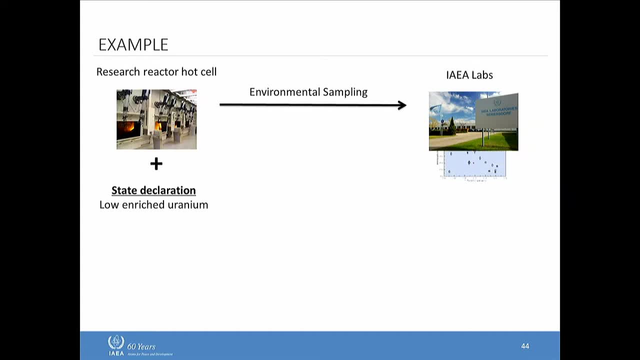 these IEA laboratories and it's analyzed and it indicates HEU particles. so let's say they said 5% but we're seeing 37% or 69%. this would be strange and it would be a red flag and it would be something odd. here we have to get to the 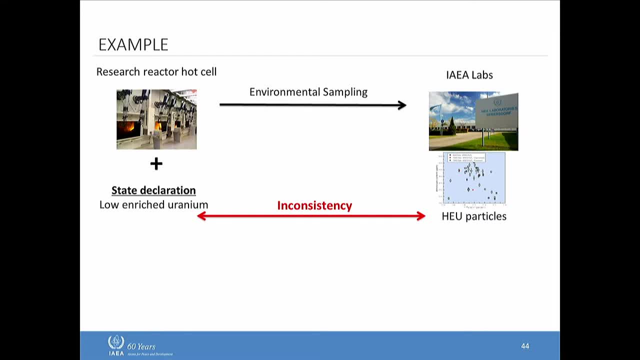 bottom of it Could be. perhaps cross-contamination laboratory's pretty good about things like that could be inspector, cross-contamination brought the contamination from the last inspection, but generally they're pretty good and they do pre-sweep checks to make sure that isn't the case. 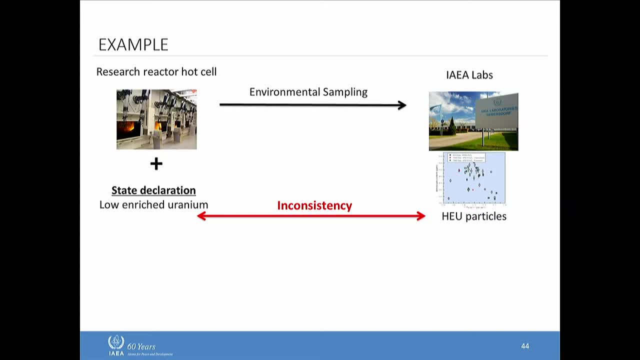 So we just have to investigate and resolve and find out why, because this is a big deal. We've got HEU particles. You said you're dealing with LEU, but we've got looks like HEU. It could be that maybe this is something from the past, a legacy. 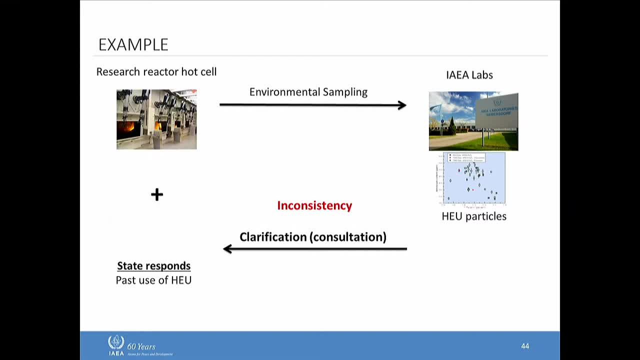 contamination issue from the 60s or something, and the state digs into their archive and says: you know, at one time we did do HEU in this room or in this area and we did have that isotopic composition. we would have to maybe confirm that. 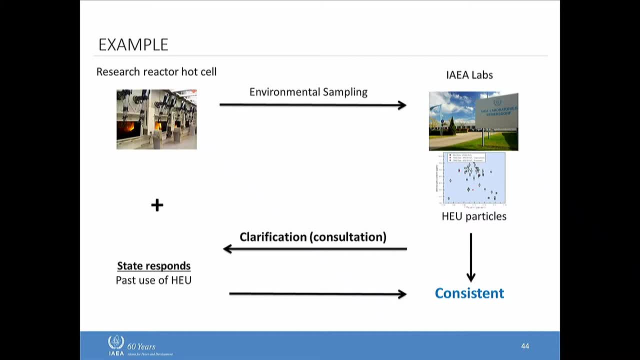 check with other records, things like that, but in the end it could be everything's okay, issues resolved. it's back to being consistent. so a lot of times issues are just resolved like this because a lot of states will have legacy issues, especially states with complicated 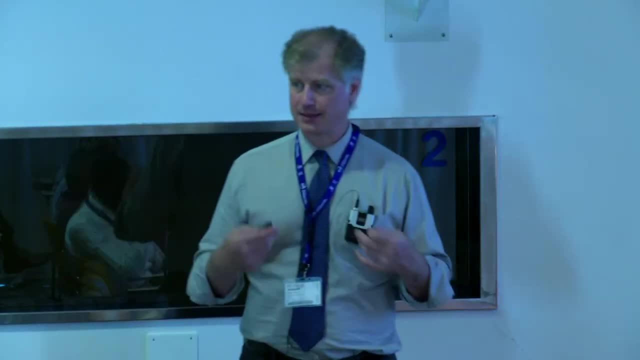 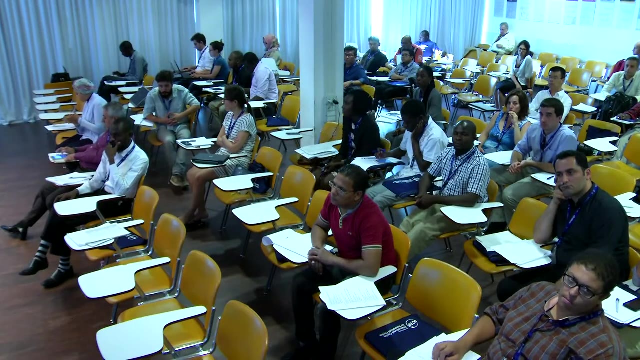 complex nuclear fuel cycles and if those nuclear fuel cycles got underway in the 1960s and 70s, most of these safeguards measures kicked in in the 60s or 70s, but more of the advanced measures like environmental sampling, came later. so our tools are very powerful now. so we detect. 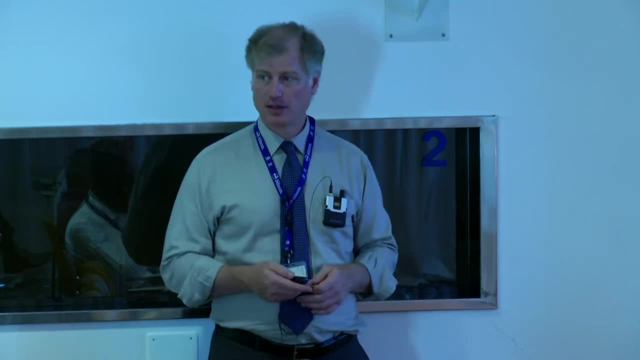 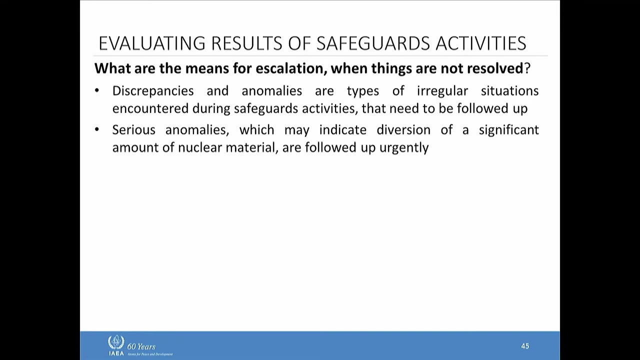 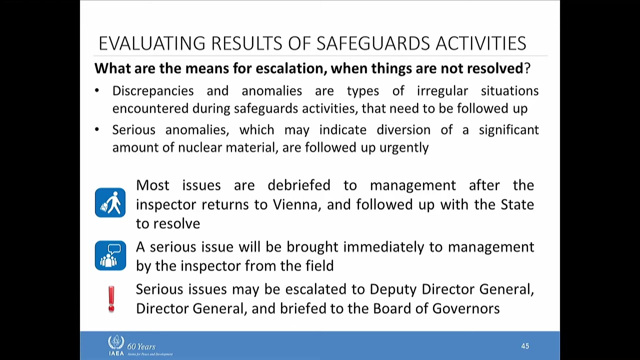 things from the past. I'm just part of the peaceful legacy nuclear fuel cycle. So again, if there's anomalies, these would be raised and they'd be escalated at the appropriate level and followed up, And I think I talked about this. most issues are. 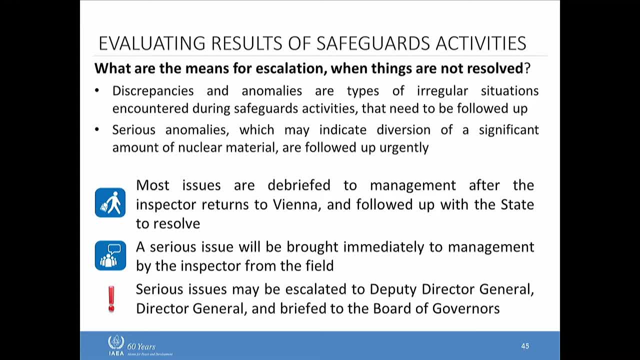 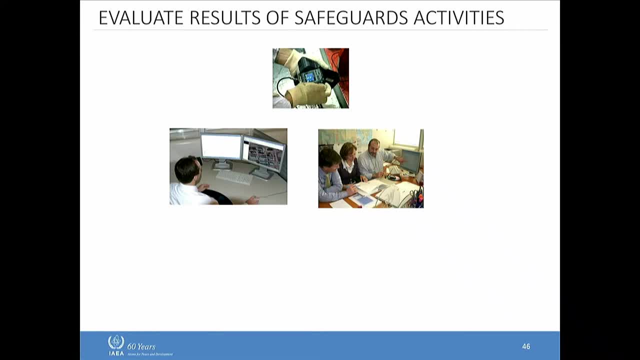 resolved at the state level. if it's serious enough, it could go to the DDG or higher, or maybe to the DG and to the Board of Governors. So I just want to highlight all these different groups: analysts, inspectors in the field, analysts at headquarters. inspectors in the field. 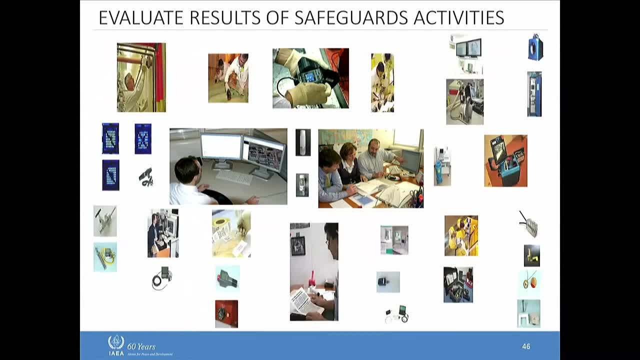 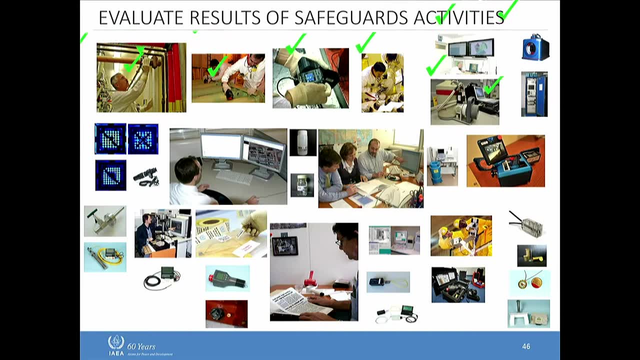 are constantly evaluating all this information that's coming in through verification, consistency analysis, and they're constantly checking everything against the other. Is it all adding up? Does it look like any of these plausible pathways that we pose for the state are materializing? So we're just checking things. 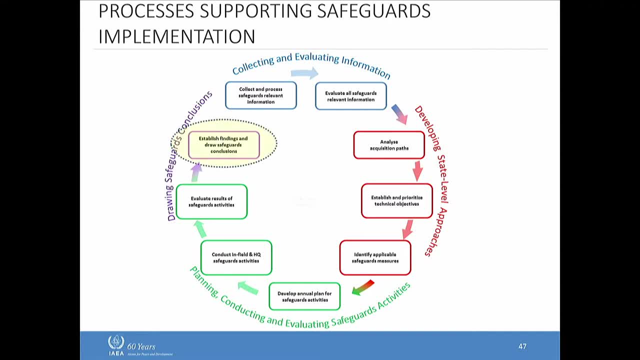 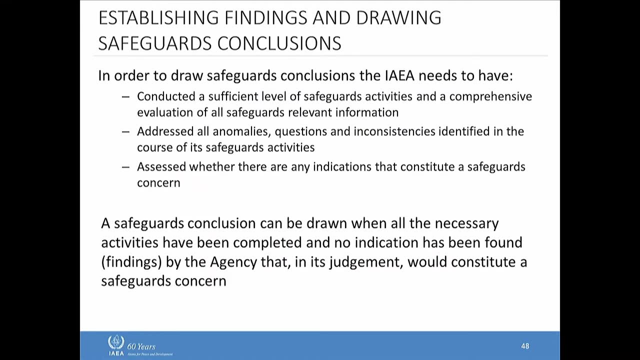 and then finally, after we do that, as we get into these findings and observations, we draw what we call our safeguards conclusions for the state. So in order to do this, we have to make sure there's no anomalies, questions, inconsistencies, Those are resolved satisfactorily. 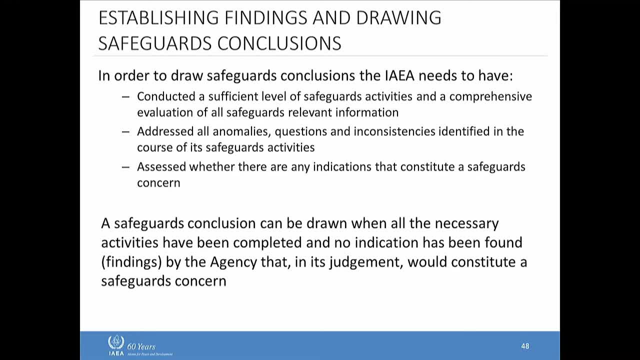 The technical objectives I talked about have been met in a consistent and timely manner and there's no issue that indicates there might be something untoward going on in the state that we would have a safeguards concern If all that's met- and this is usually the case, which is pretty boring. 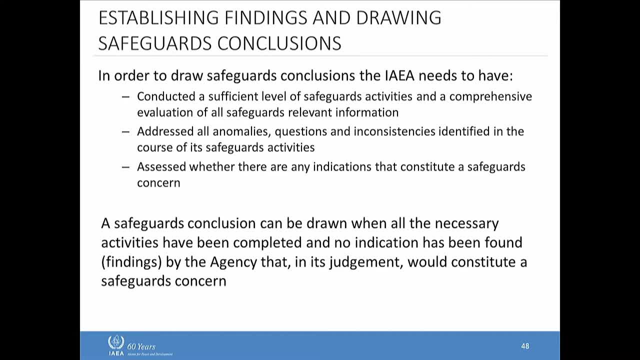 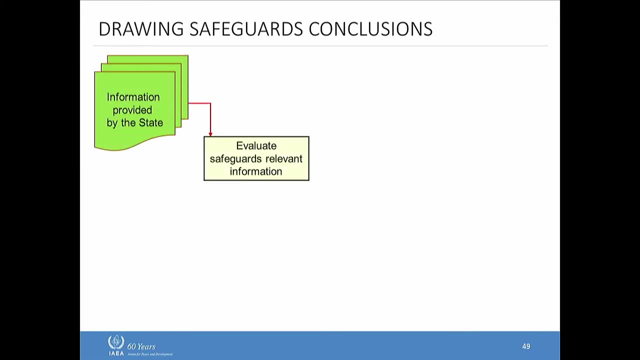 so the conclusion is just fairly straightforward: there's no diversion of declarative material, no indication of no diversion of declarative material and no indication of undeclared material activities. Those are generally the conclusions we make. We would draw these every year. so again, information provided by the state. 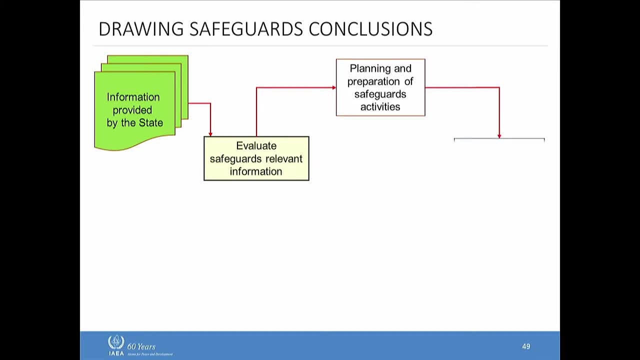 we evaluate it, prepare a plan, state level approach, conduct activities. we get information results from those activities. we compare it to the information the state provided, along with other open source type information. if everything's okay, we draw a credible, sound conclusion for the state that there's been no diversion of the declarative material. 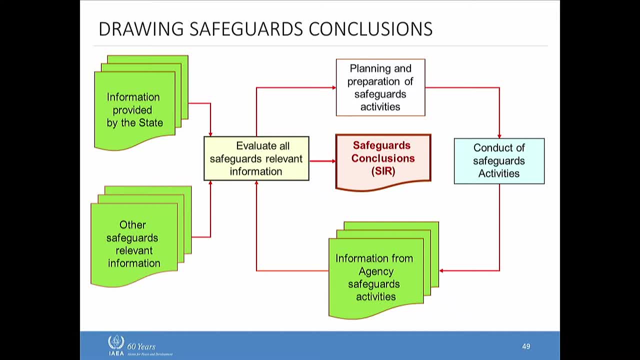 like the spent fuel in the example, and no undeclared material activities like the misuse or the undeclared stuff, And we publish this annually in what's called the Safeguards Implementation Report, or the SAR. usually comes out in the May timeframe and that's where the conclusions are. 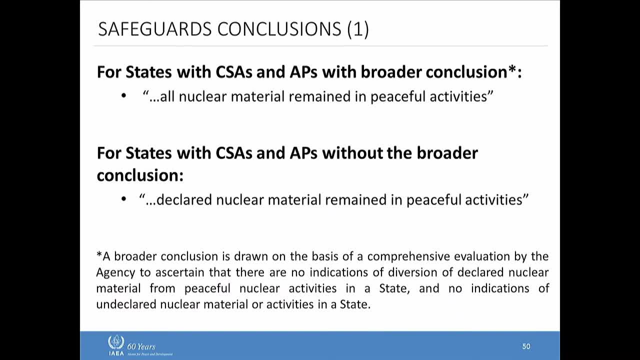 documented for the year And the wording on those conclusions is a bit legal and I think the lawyer will go over these tomorrow in more detail. but for states with this comprehensive safeguards agreement and APs enforce all nuclear material remained in peaceful activities, they don't have this broader conclusion. 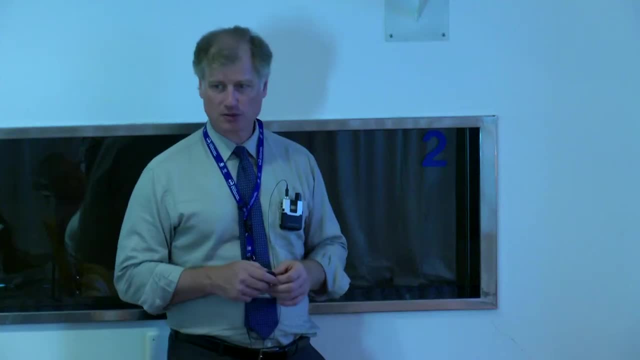 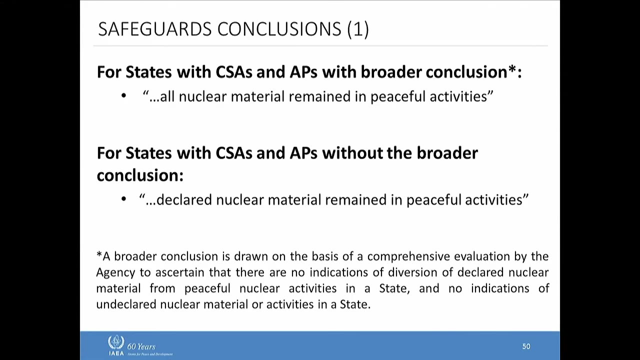 which takes some time- where we have this certain level of understanding about the state that we're certain there's no undeclared nuclear material activity going on. if that's not the case, then instead of just saying all nuclear material, we say declared nuclear material, because there may be some ongoing work. 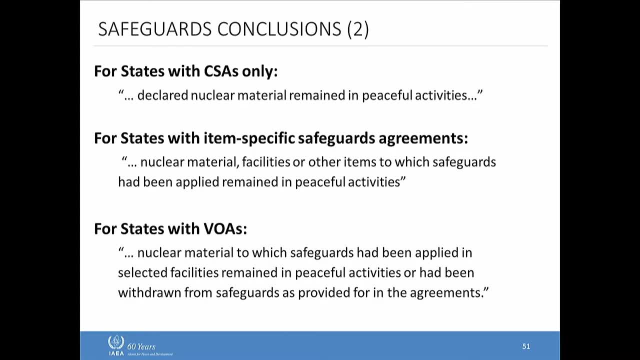 to get from declared to all and if they don't have an additional protocol, if it's just a comprehensive safeguards agreement- remember that first box, that was limited- don't have access to all the information in the state or access to all the locations in the state. again we would just say declared nuclear. 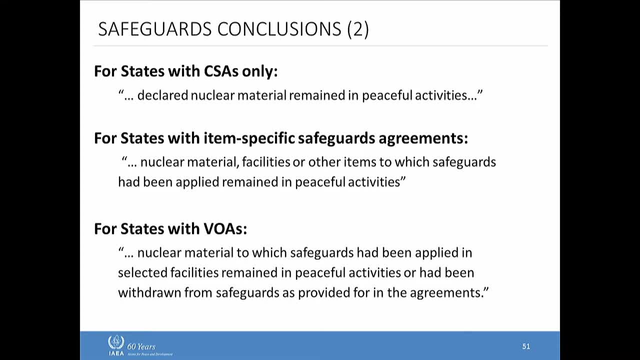 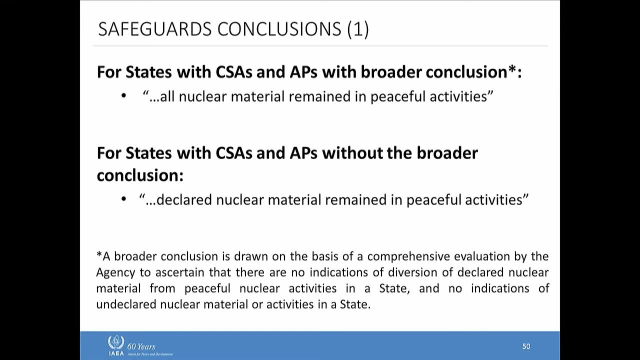 material. So a broader conclusion came up, basically in the late 90s. initially the agency just made a conclusion on the version of declared nuclear material. so if we confirm that the nuclear material is still there, all the material balance evaluations were closed properly. the conclusion was there was no diversion of declared nuclear material. 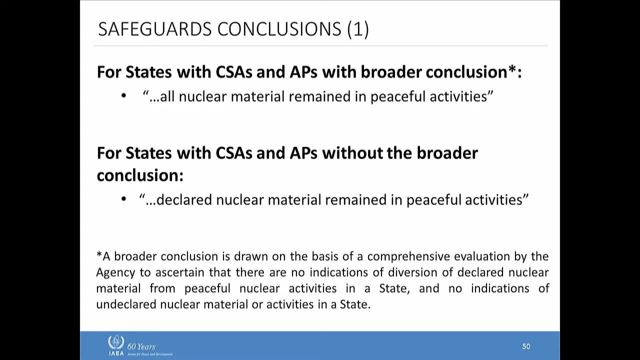 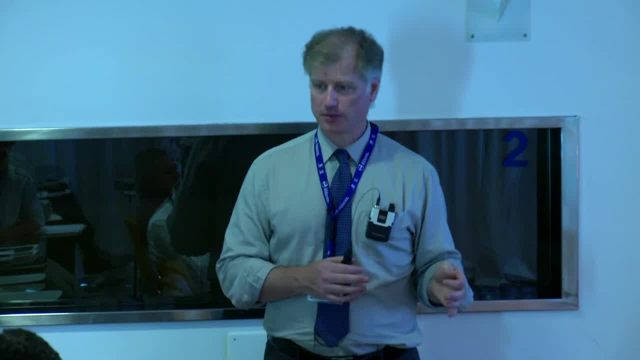 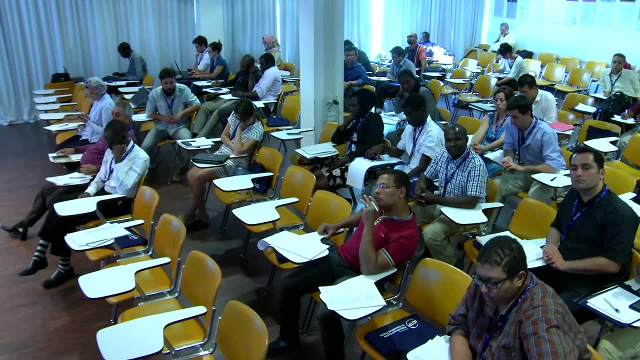 we found this was a weakness in the 90s because there were several case studies, like Iraq and other states, where it wasn't just about diverting declared nuclear material. there was undeclared activity going on at declared sites and in other parts of the state, for the case of Iraq was extensive. 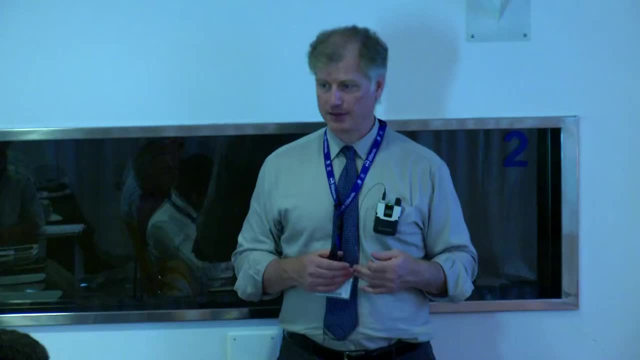 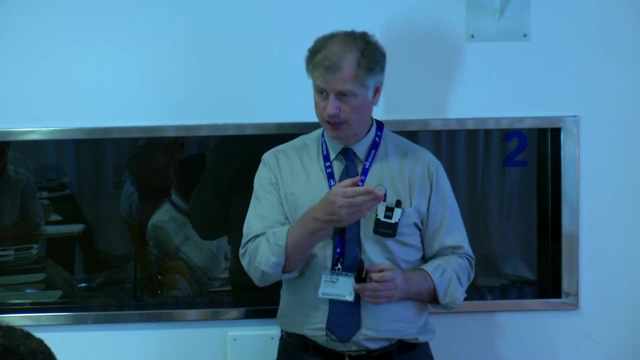 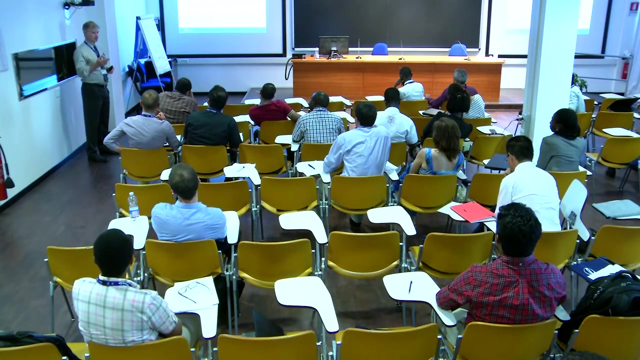 so it indicated to the agency in the early 90s that the current regime wasn't working, just looking at declared nuclear material. so the emphasis shifted. this is when this additional protocol came around, where it gave us more information and access that enabled the agency to confirm what we call. 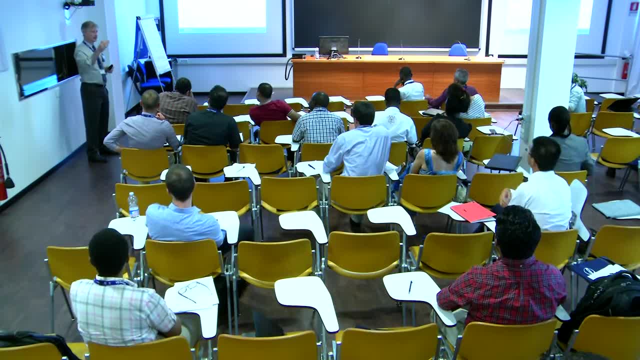 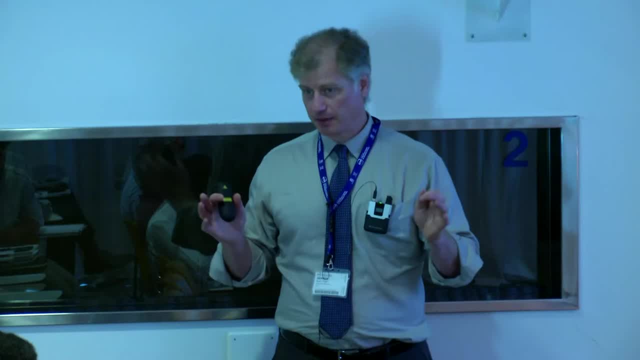 to make a broader conclusion, not just on the diversion, but to broaden that to: there's no indication of undeclared nuclear material. I should just say it's no indication. maybe we just didn't look in the right place, but hopefully we've looked hard enough and this process 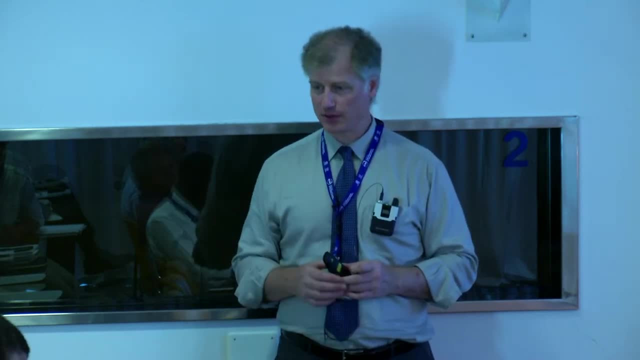 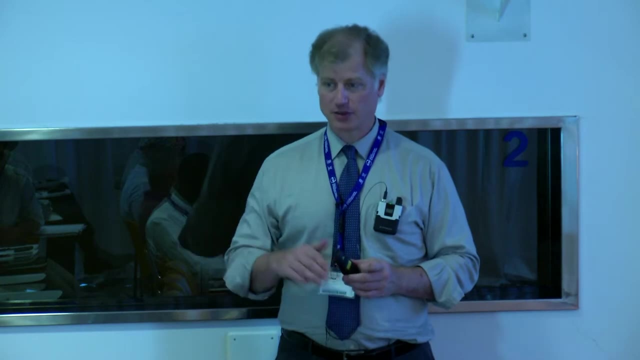 to get to this broader conclusion is pretty exhaustive. we go through all this information and it's very extensive. we do a lot of these complimentary access type visits. the state gets a lot of attention. until this broader conclusion is reached it might drop off a little bit but we still give the state quite a bit of. 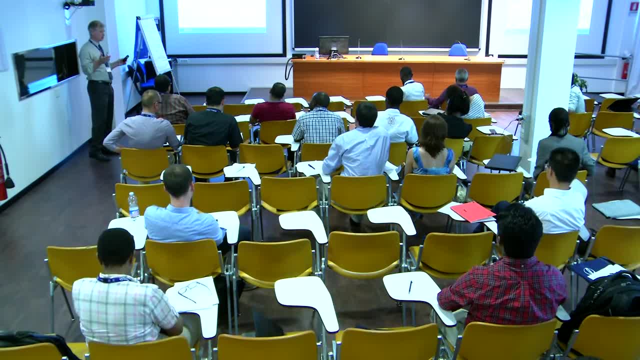 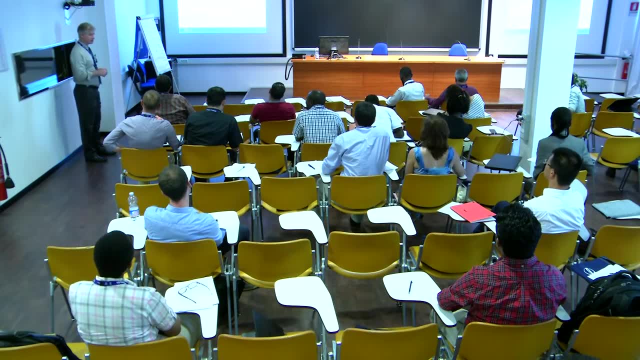 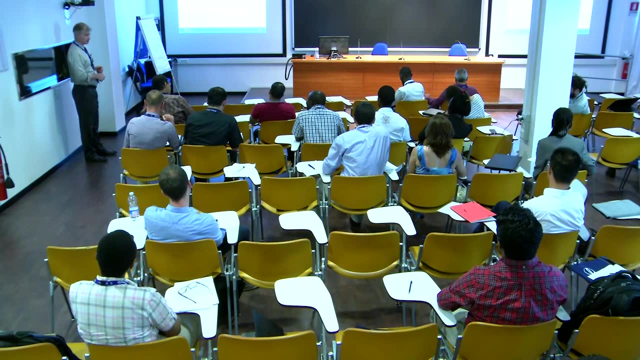 attention on its AP declarations. so that's what we call this broader conclusion. well, it's not really a states, not really a state doesn't have to agree to. what the state has to agree to is to ratifying the additional protocol legally, so it's entered into force. 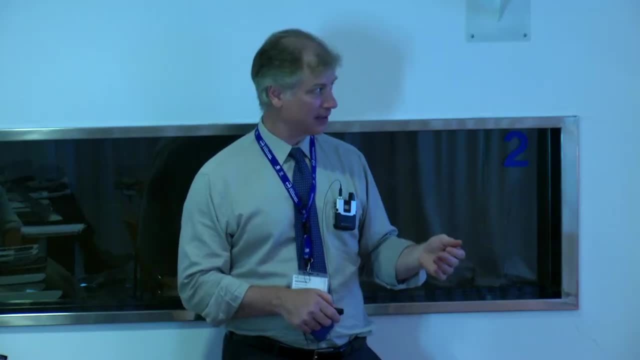 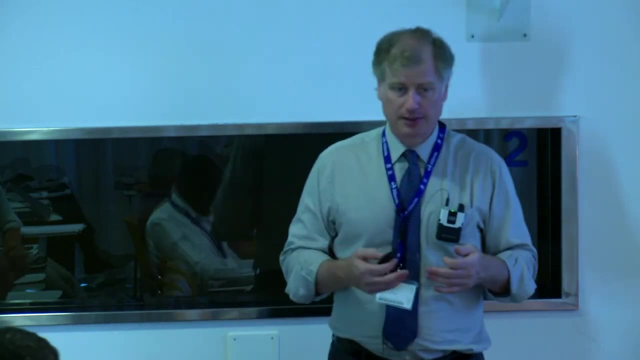 so we have this increased information and access. once we have that, it's just by procedure and by policy, and the agency after depends on the complexity of the state- could take a year, two, three years. sometimes the issues could be very complex, so it could be four, five, six years to resolve an issue. 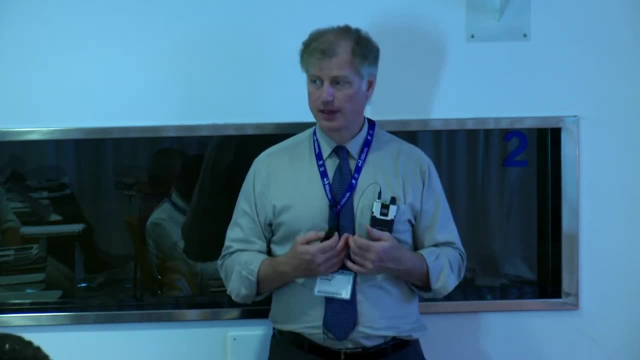 but if that's done, then we could have a higher level of certainty that there's no indication of undeclared material, no indication of undeclared activities going on, nothing untoward. then we could say: there's no indication of this and we give that state, we call it granted, the broader conclusion. 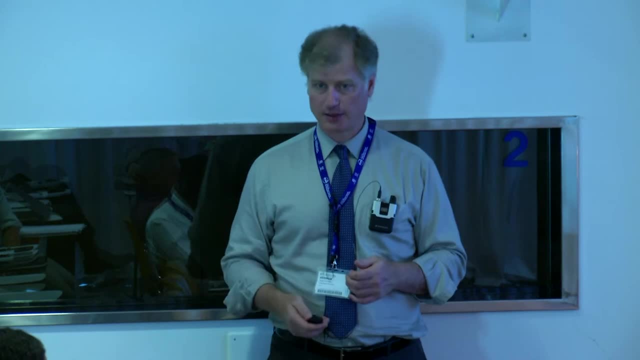 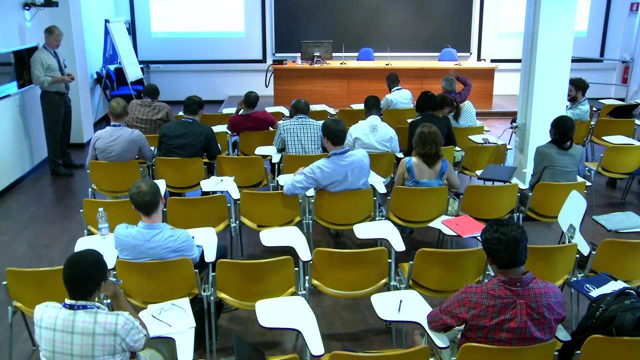 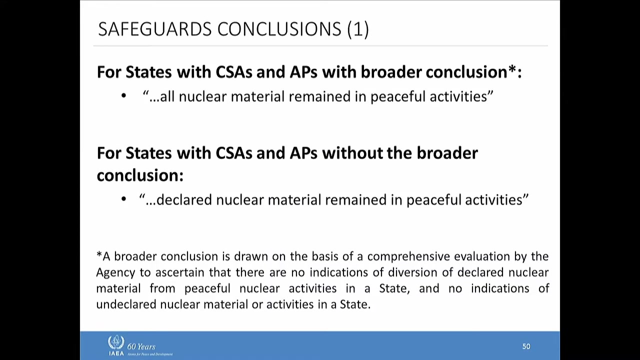 and that's reaffirmed every year. so we have to continue to check that. so there's this diversion, there's the non diversion conclusion. now we call it the broader conclusion and I'd have to check. I think we have about, so every state would get a conclusion. 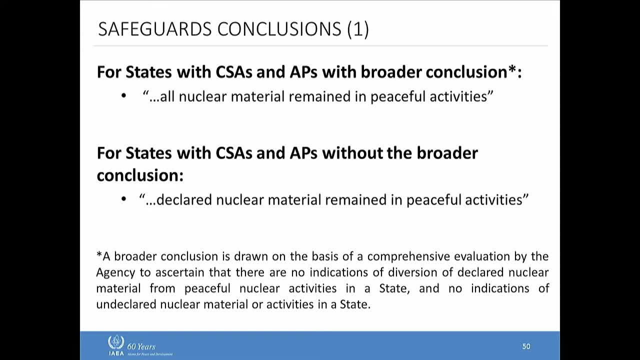 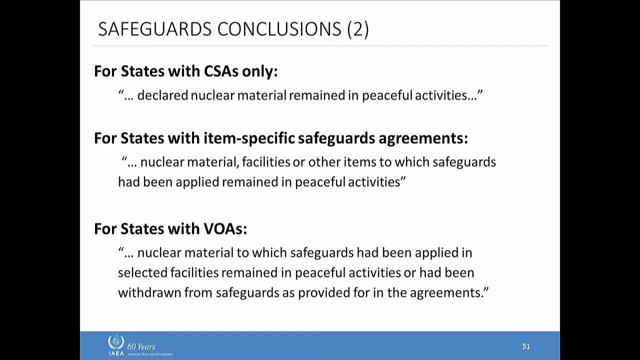 every year, but there's only about. I'd have to check. I think it's around almost 70 states, maybe high 60s, 70 states, that have this broader conclusion, and then I didn't get into this in detail. we also have what we call item specific agreements. 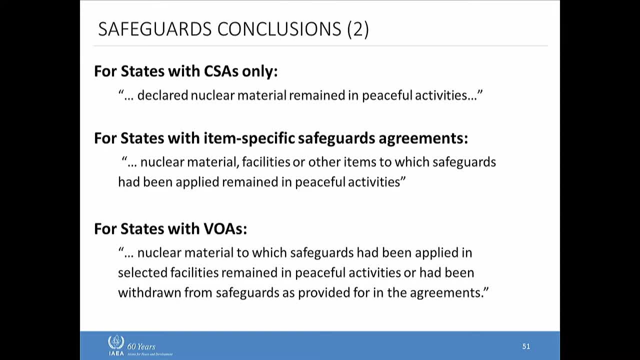 for 66 states. this is basically India, Pakistan, Israel. they get their own type of conclusion because states that didn't sign the NPT could still have access to nuclear material facilities and our conclusion is just focused on the nuclear material facility that was supplied to make sure that wasn't. 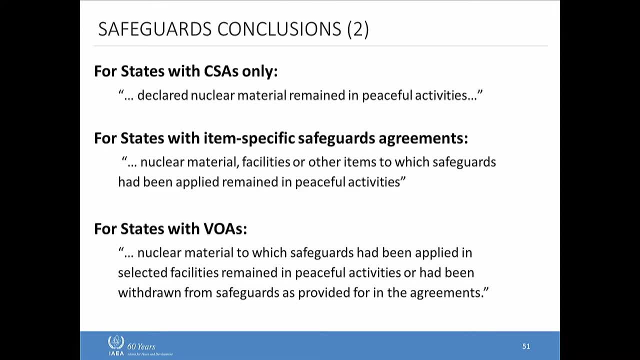 the nuclear material wasn't diverted, that the facility wasn't misused. so it's a very narrow type of conclusion and it's similar for VOAs, voluntary offer agreements. this is another way of saying a nuclear weapon state. so this is the five nuclear weapon states. they could also have the material that they offer. 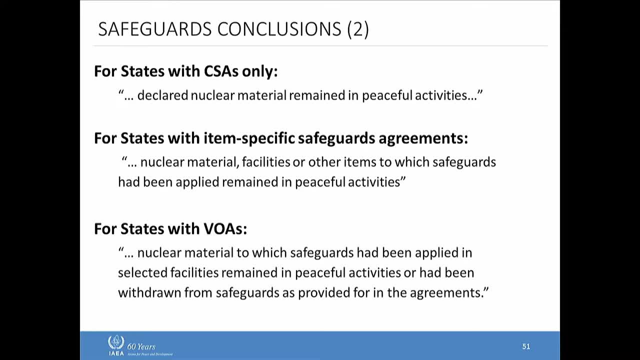 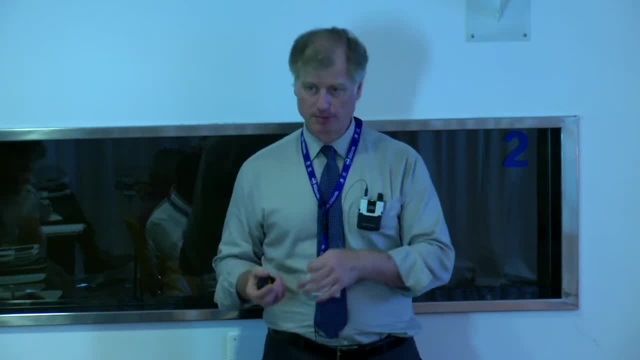 for safeguards. that material that's offered. we check to make sure it hasn't been removed from safeguards. sometimes a state that isn't part of it isn't a nuclear weapon state. they ship material to a nuclear weapon state and they want it safeguarded, so we'll have to apply safeguards to it. 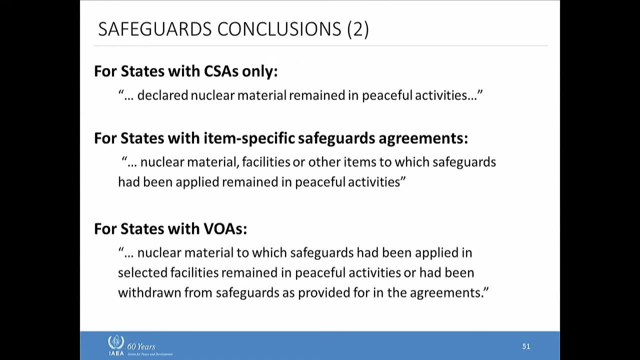 an example might be: Japan had spent fuel. Japan is not a nuclear weapon state under the NPT. they send it to France, let's say, which is a nuclear weapon state under the NPT, and that material will be under safeguards in France. seems a bit strange because it was Japanese material. 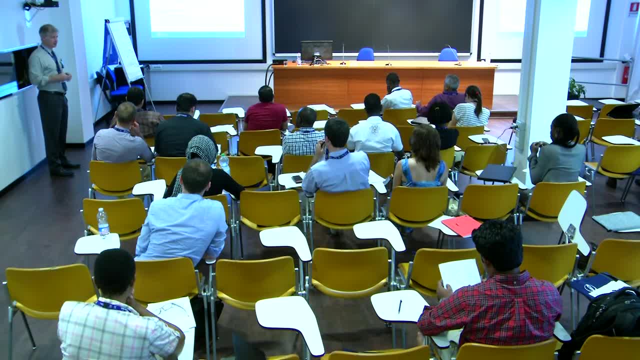 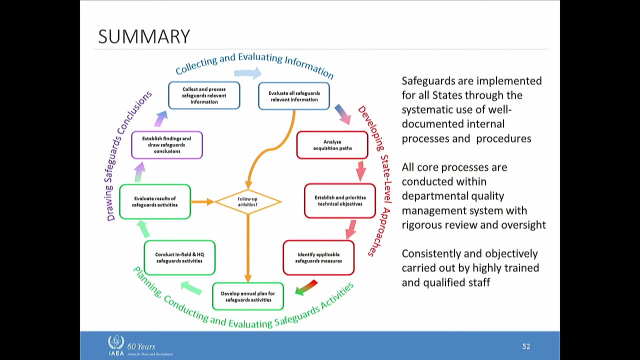 and we're drawing a conclusion for Japan. but Japan wanted us to be there. they put it. they send it to France because France reprocesses it to get the MOX fuel and they send the MOX fuel back to Japan for the reactors. so again, I just want to highlight, this is the 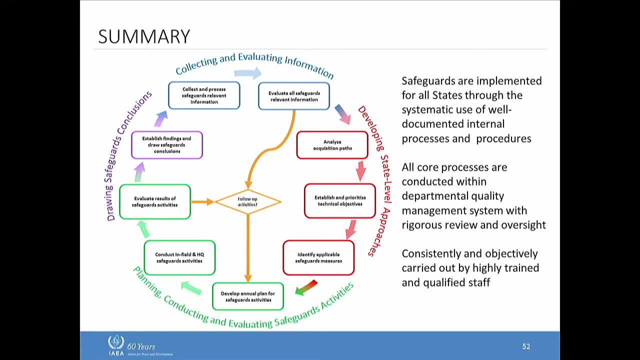 safeguard processes. I went through it kind of quick, but this is a very iterative, dynamic process. it's ongoing. simultaneously there could be parts going on over here, over here. so the state evaluation group is very busy. obviously, if we do anything poorly, we could understand the state capabilities. 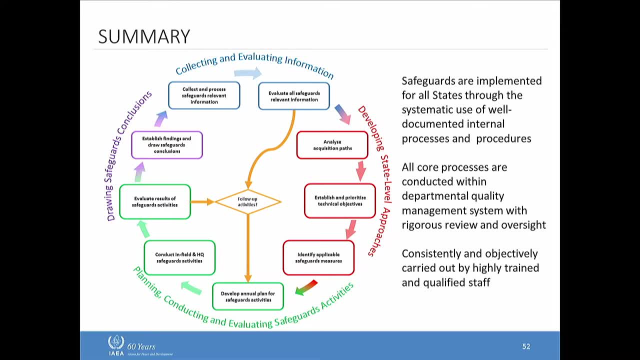 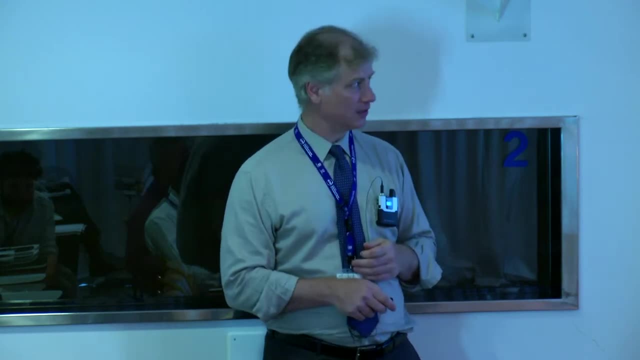 very well. but if we think the research reactor is 5 megawatts and it's actually 25 megawatts, we're going to make a different assessment about the capabilities of that research reactor. so we may not identify the correct, technically plausible acquisition path. so I just want to highlight: 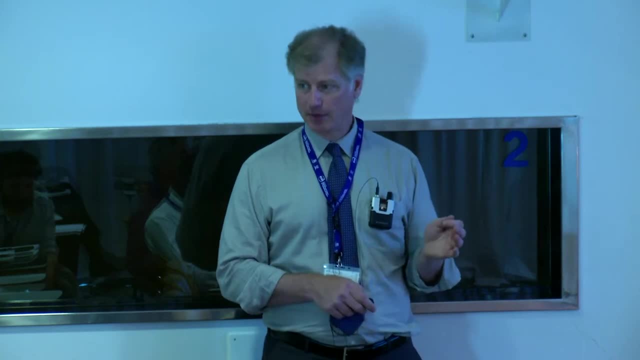 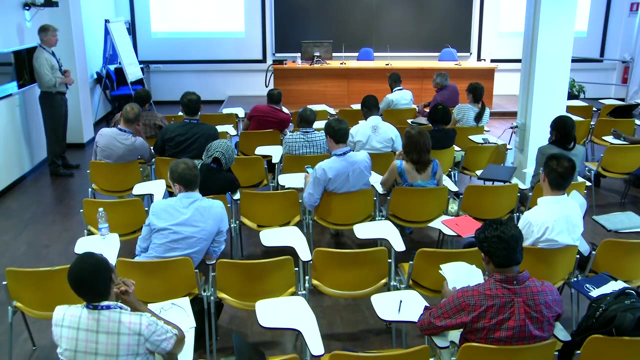 if we don't understand the state well, it doesn't matter. if we do great APA, we're still going to get poor results and it will feed forward into the rest of the process. and likewise we can understand the state real well and if we do shoddy. 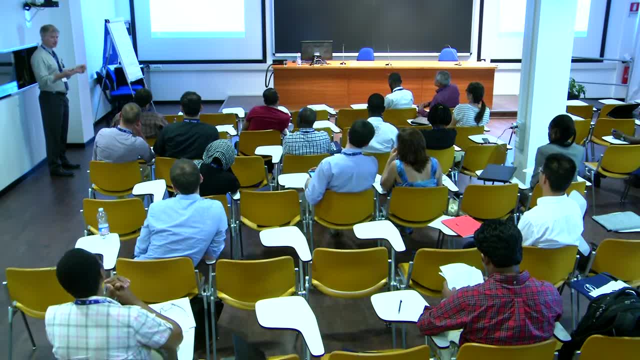 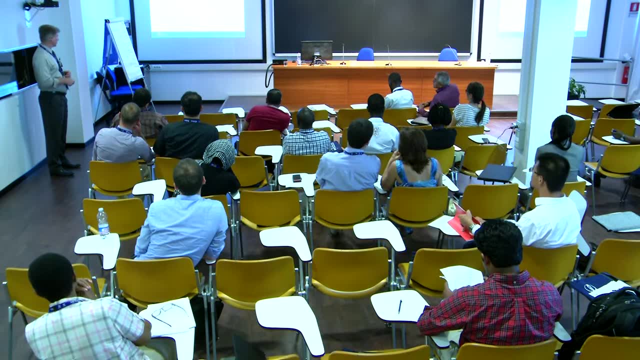 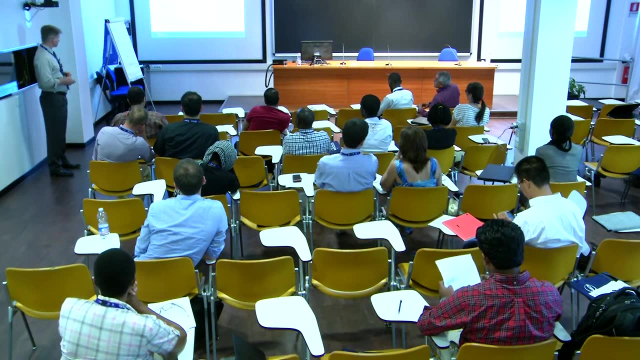 accuracy. path analysis don't take it seriously. we might not fully identify all the technically plausible paths and again it can spiral into poor quality safeguards we also have- I should have mentioned earlier. we have committees that independently check and assure that this kind of erosion isn't occurring. 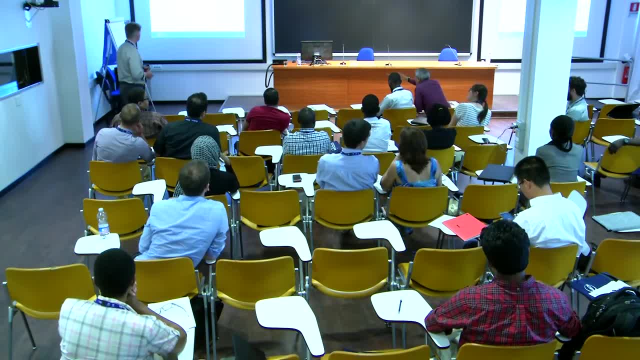 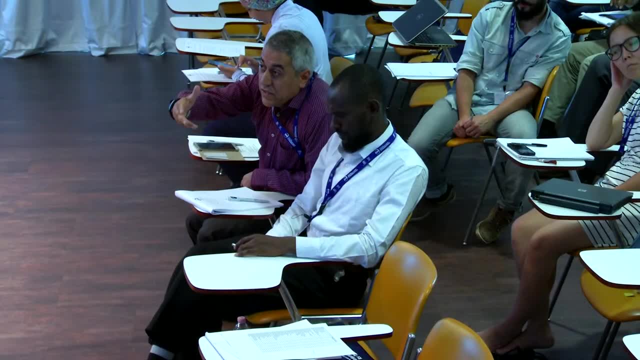 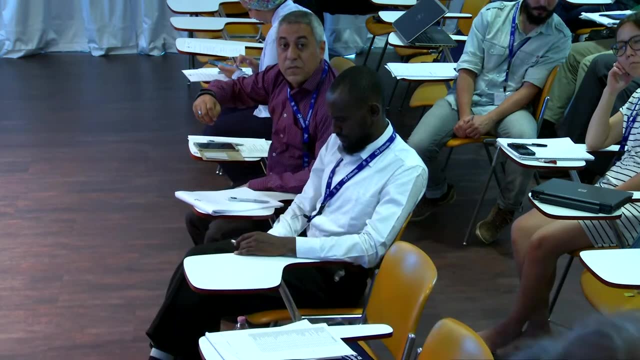 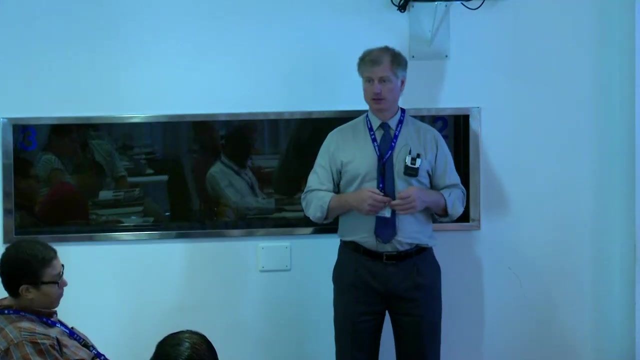 yeah, I can ask for my agency, or yeah, and you won't get it because it's an internal document. so these documents. I probably should have emphasized that at the state evaluation port we put out something called the state evaluation level up here, where we collect and analyze information. 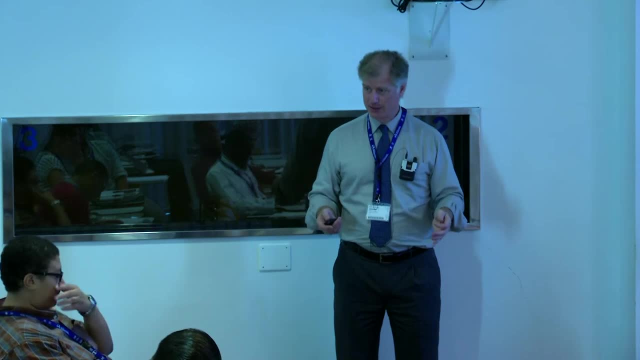 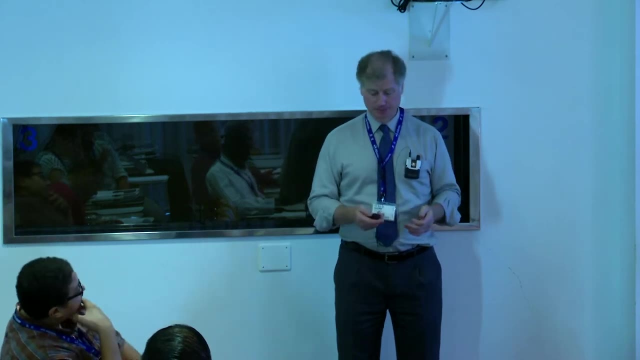 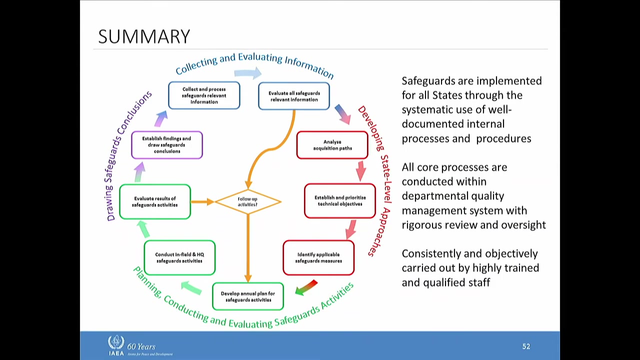 the state evaluation group will periodically document their understanding of the state, what we call state evaluation report or an SER. that is an internal document highly confidential. there's an issue to this state? likewise here, this acquisition path analysis in the state level approach the game plan basically for: 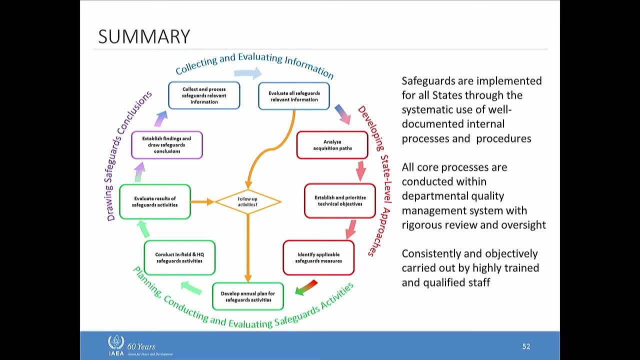 safeguarding the state is an internal document because it gets into the frequency and intensity of how we're going to do activities. we'll get into the selection probability. so if they have ten reactors we may not go to all the reactors. we may randomly select some years and not go to the other ones. 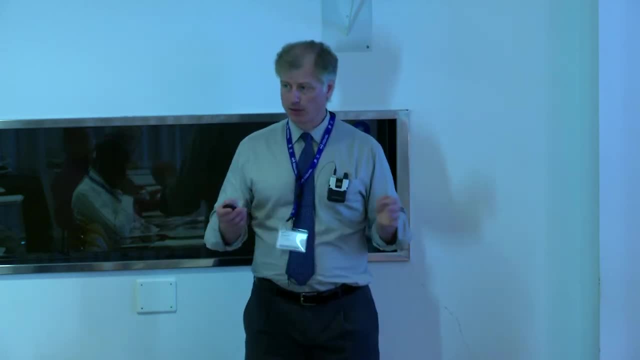 that's statistically supported either 20% or 50%, so it'll be a randomness and unpredictability that's added to it. the state had that document and knew, oh, they're showing up 20% of the time and they would have a leg up on proliferation. 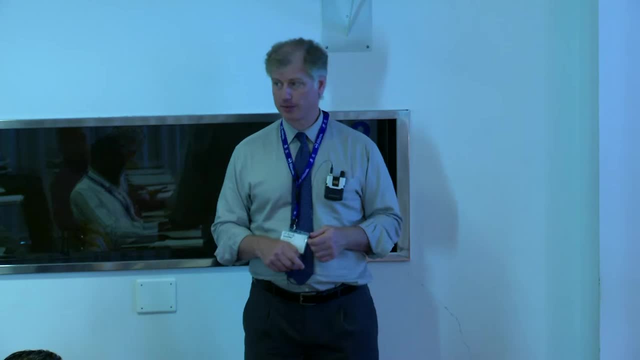 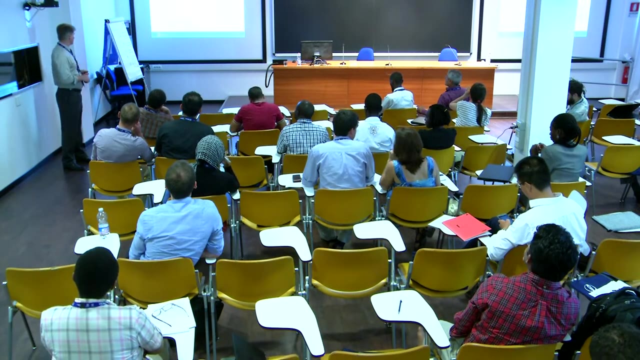 and likewise down here we have this annual implementation plan that comes out. that's a very sensitive document because it again tells exactly where we're going and when we're going, so that can't be released to the state. the state implementation report generally is released, but it's done through the board. 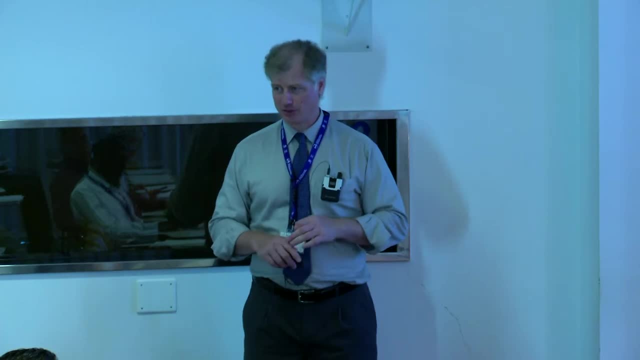 of governors. so the board of governors would get a copy of that and that's the general overarching conclusions I was talking about about all declared material remained in peaceful use, things like that. but generally speaking, to answer your question, no, the state wouldn't get a copy of that. however, 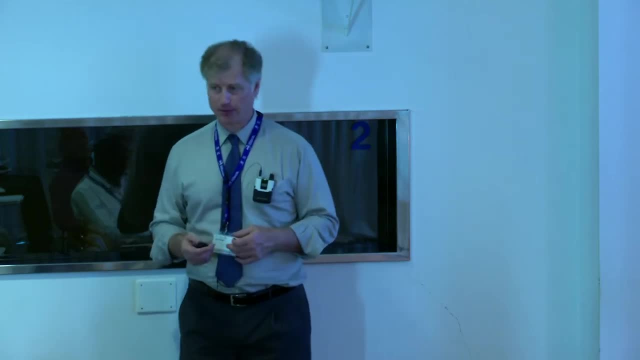 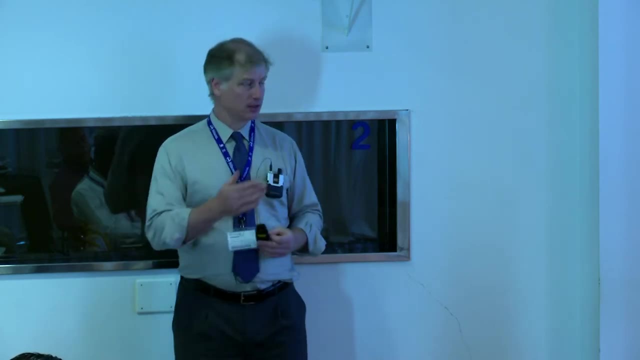 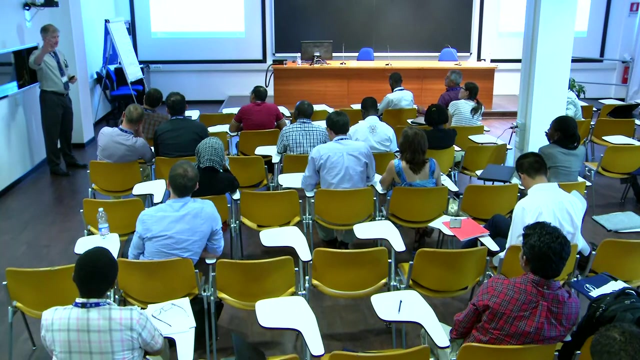 I should add, the agency would consult with the state, because sometimes we have to implement a measure. many of the states cooperation just can't install equipment, so that I mentioned in here one thing the agency has for verification: they have remote monitoring. so I talked about the surveillance systems. 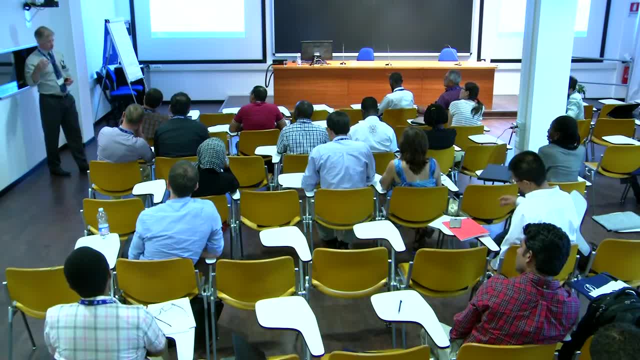 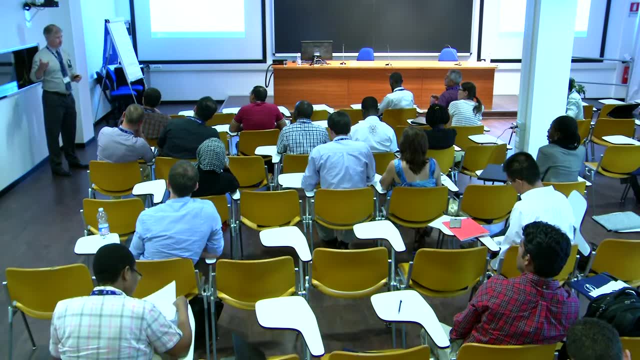 well, in the past the inspector had to go into the field service camera, take out the flash card of the media and bring it back to review it. but it started a while ago. 10, 12 years ago we implemented what we call remote monitoring. the data is transmitted remotely. 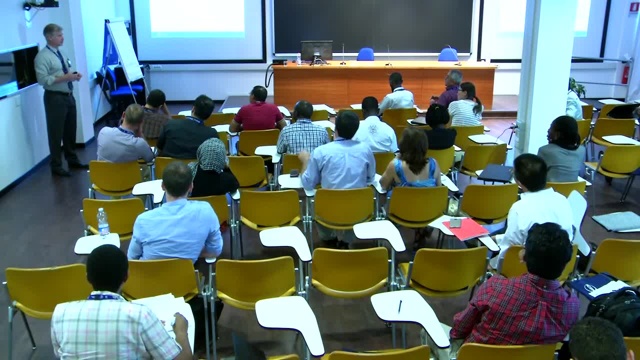 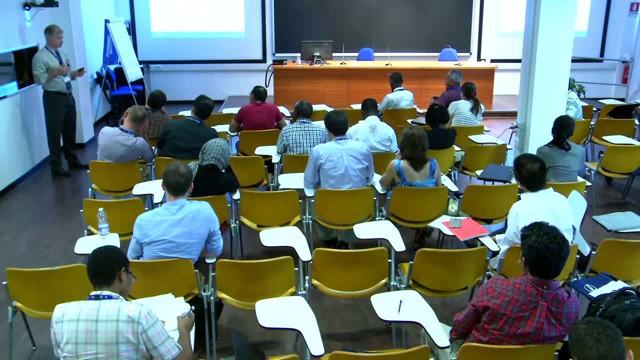 agency headquarters could also be a regional office and the data can be reviewed there. but we just can't do that without the state knowing about it. so the state would have to agree to that. usually it's in their interest because we can find out if there's any issues and if 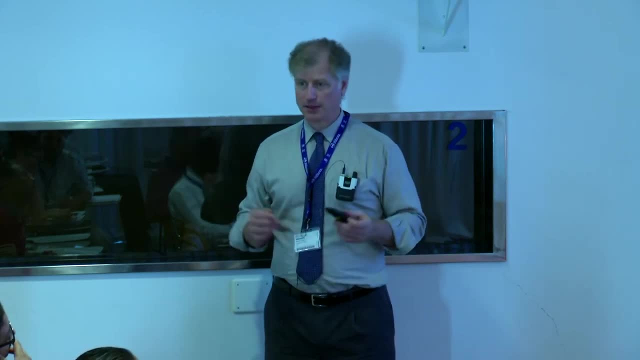 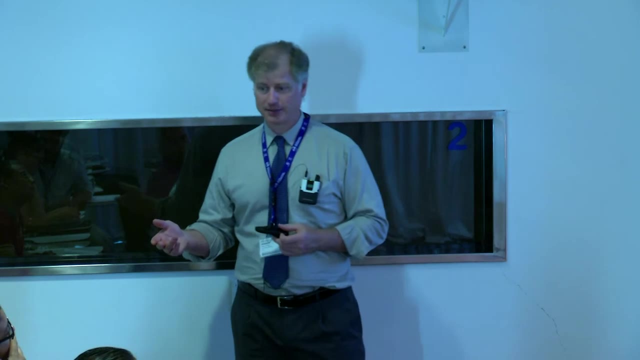 there was something that was accidental, something that was they just forgot to tell us about. it's better that we find out about that sooner, and remote monitoring allows that capability. also, if our equipment breaks, you may not know about it. if we go to visit, we'll just find out how this 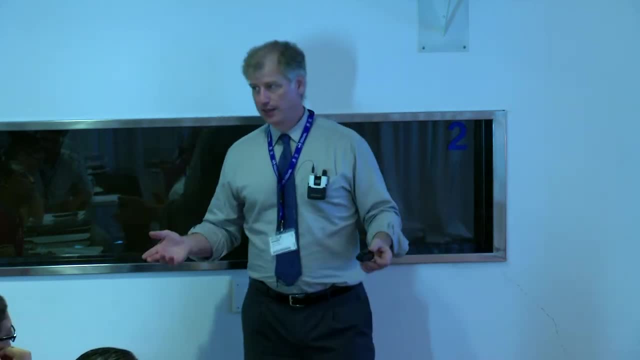 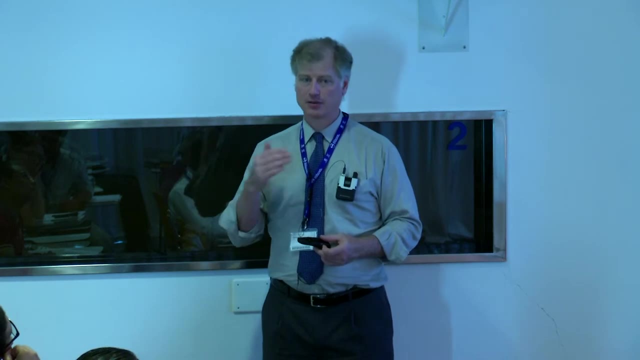 equipment broke and that's a problem for everyone, because now we'll say, well, sorry, our equipment broke, but we can't draw a conclusion, we've got a problem. we still have to verify this new material that was under surveillance. but if we have remote monitoring that could tell us. 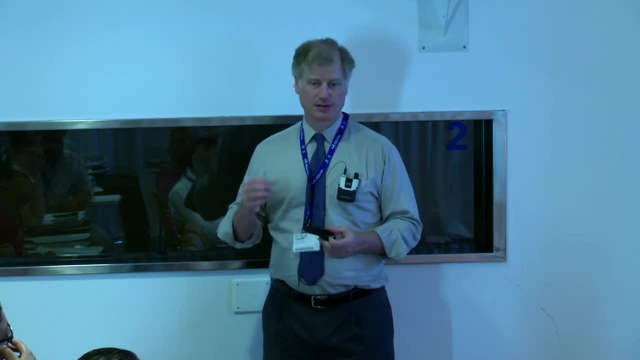 sooner in the process that the equipment is about to break or it's failing and there's a weakness or some problem, and that we call it state of health. information is transmitted to the agency and it can tell us if there's an equipment problem so we can find out. 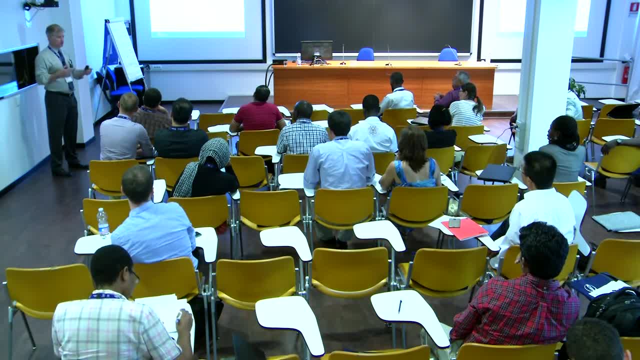 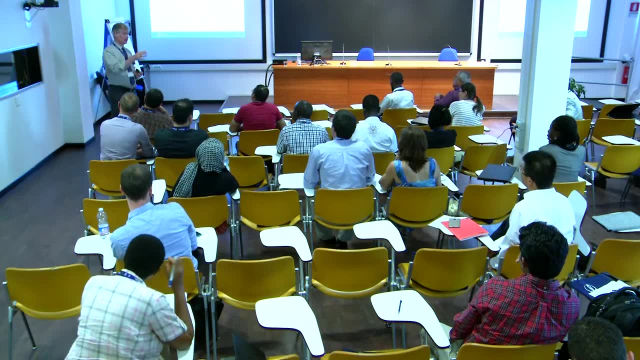 sooner. so that would be an example. we'd have to have the state involved but just can't install equipment. likewise, if we want to do, in some states we do what we call unannounced inspections, so don't give any notification to the state, but we just 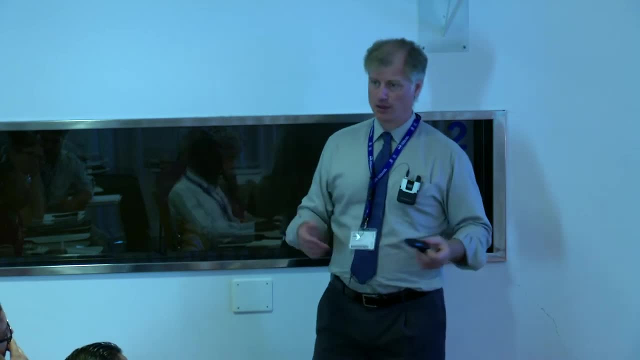 can't do this in a state, they have to at least agree to the principle and the procedures we're going to use. so we're not notifying when we do the unannounced inspection, but they have to be aware that this regime exists, that we can do it. 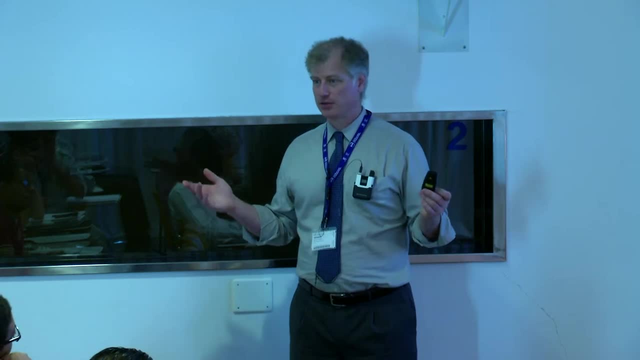 we just show up at the gate and knock and send here for an unannounced inspection, we'll say we don't know what you're talking about if they're used to predictable quarterly or annual inspections. but the state may like that because it may reduce the amount of 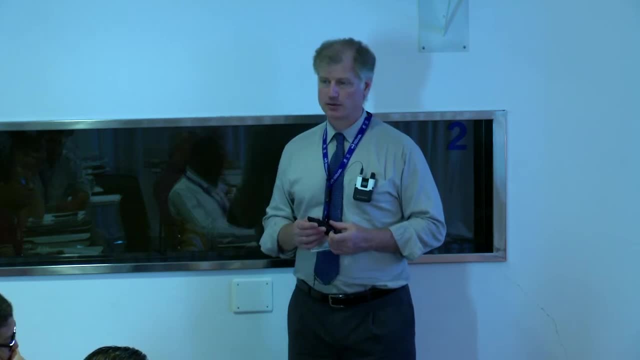 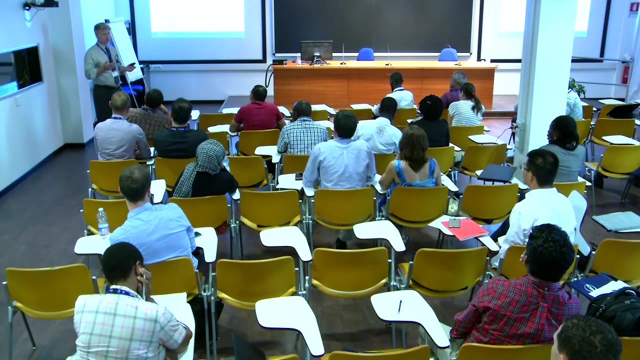 resources they need in terms of accompanying agency safeguards inspectors. so there's certain aspects. i should highlight that they have to cooperate with the state and we need to- we should- to make it smooth to implement certain safeguards measures. i think that's it. thanks for your attention. it's a lot of. 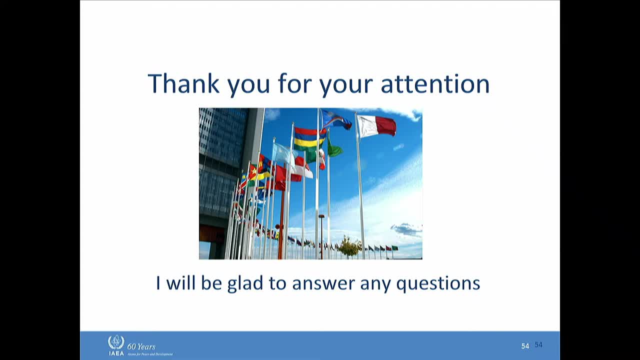 material- you'll get some more tomorrow on the legal aspects- and actually gave you basically for, uh, new inspectors. they get this in about four months, so it condensed and really shrunk down to a lot of information. so if you feel overwhelmed, don't worry about it. the idea is just to 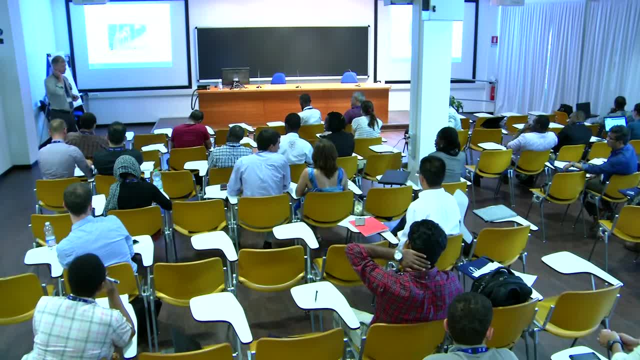 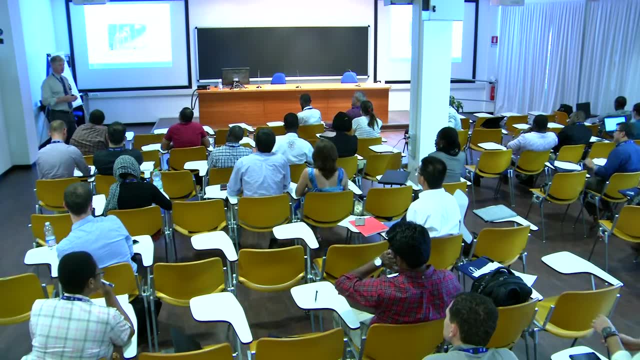 give you a feeling for the safeguards. so if you go back as uh managers in your, in your facilities, in your states, you'll have an appreciation for the appreciation for some of these. you can't absorb it all day, i don't expect it. i don't expect it to, but just there's. 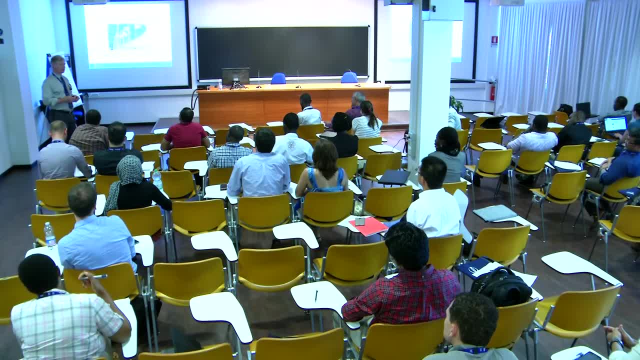 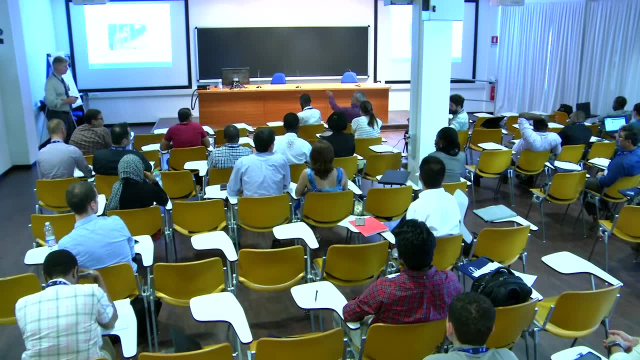 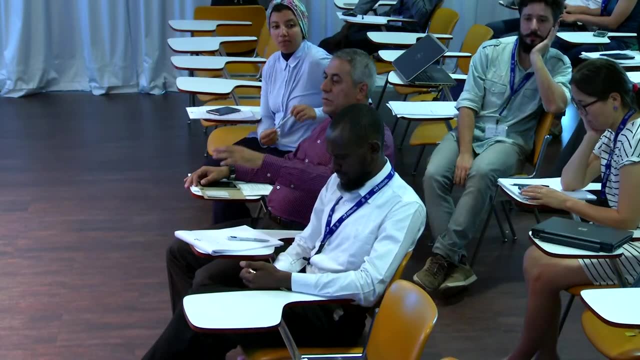 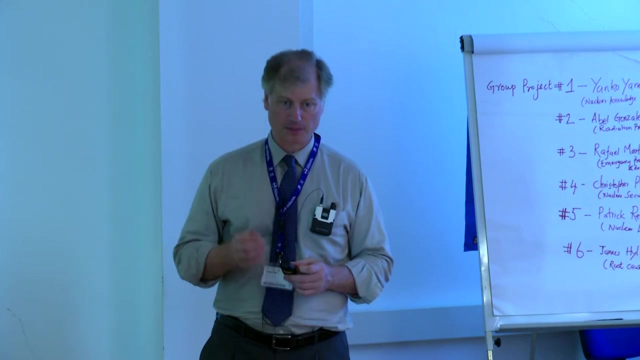 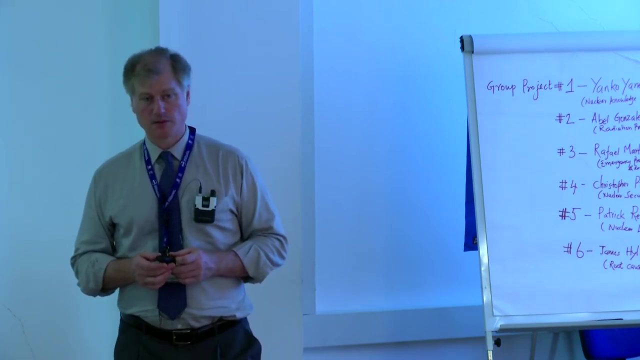 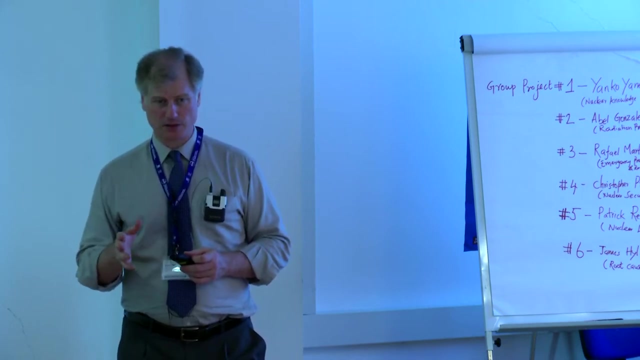 a lot of material and it's also involved, so it's changed over time to make things more effective. any questions on safeguards? yeah, i mean by a political issue just as an example like: uh, i mean generally it shouldn't, if the agency is a technical organization probably is at high very. 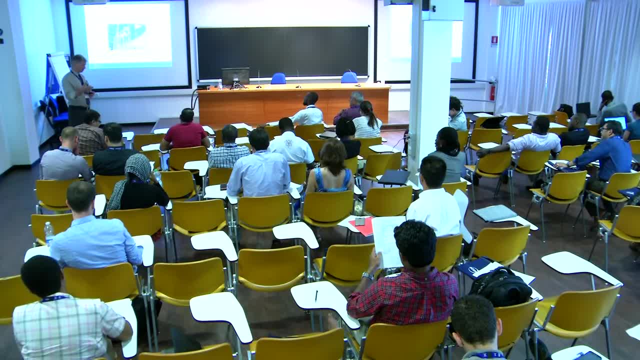 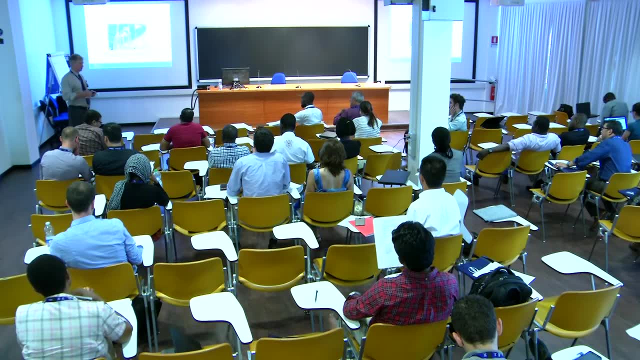 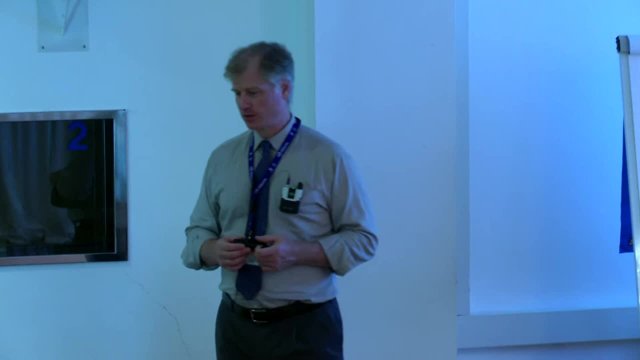 high levels. there's probably political influence, but it's the inspector analyst level that shouldn't come into play. we just have a job to do. we have to verify new material. we're probably going to have to look at the report or information that comes in now sometimes. 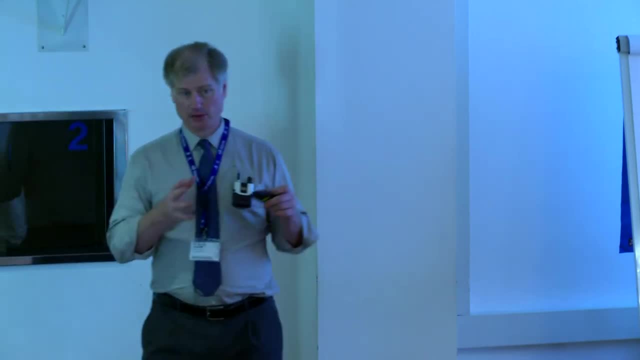 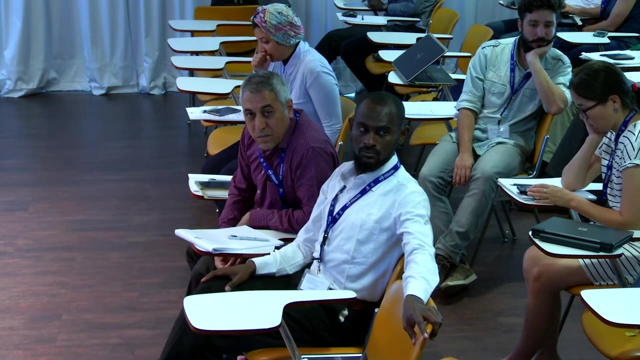 some inspectors, some, some sections may go a bit too deep and maybe there's nothing there and state may not like that and it could be justified. maybe you need to back off a bit, maybe you're doing too much. you can get a little bit out of balance, if one. 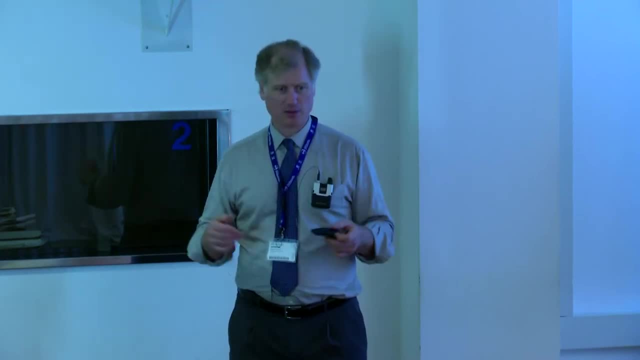 seg is, uh, inspecting to one level and it doesn't make sense to the state. maybe you know we need to look at that and say what. look back at your, your plan sense. are we overdoing it? um, re-evaluate your action paths, things like that, because some states may have 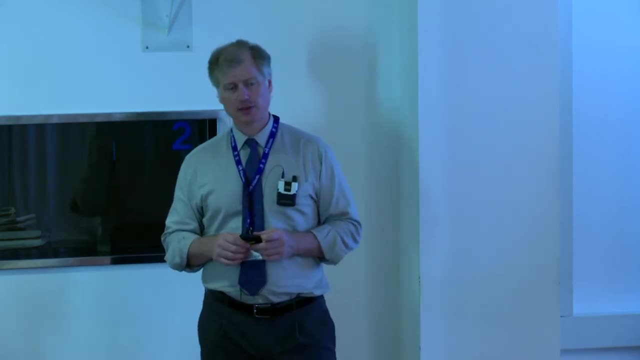 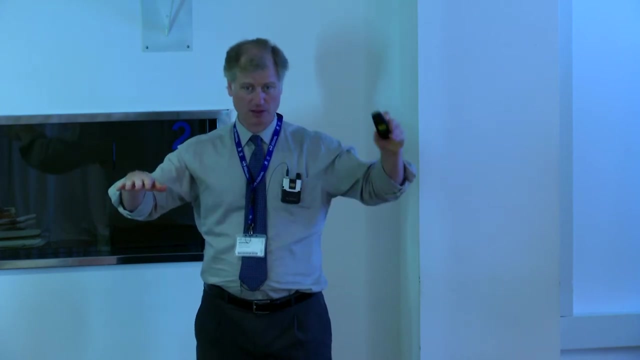 some uh segs and analysts may have analyzed differently than others. however, i mentioned this committee process, the review. hopefully that injects some harmony into this. so there isn't similar fuel cycles and one fuel cycle is getting a lot of bells and whistles, a lot of safeguards measures, and another 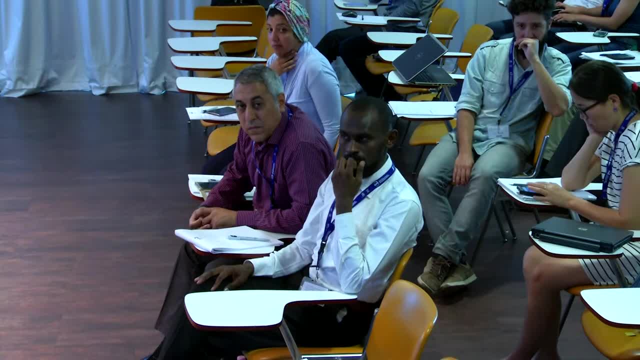 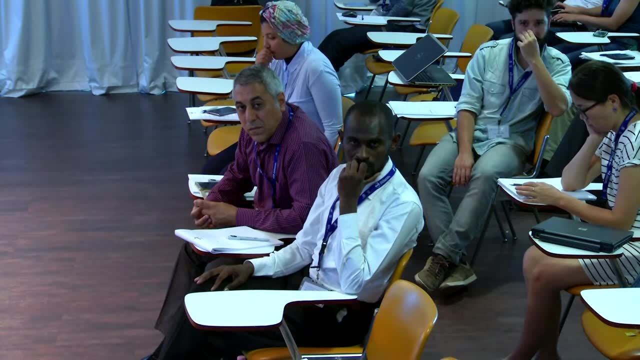 one isn't getting much or a lot less. shouldn't be that kind of imbalance. should be, should be similar. it should be. may not be identical, because no two nuclear fuel cycles are identical. some are similar. but capabilities, know-how, past experience, past capabilities, even if they're decommissioned, could give. 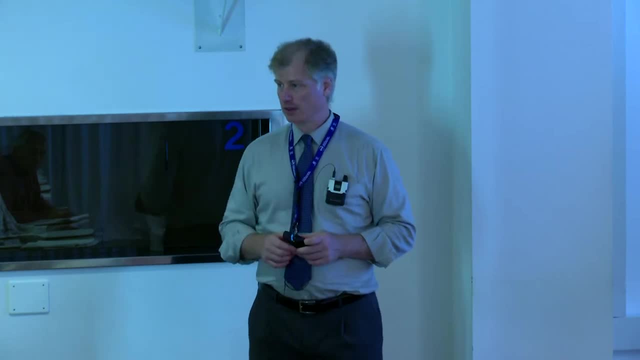 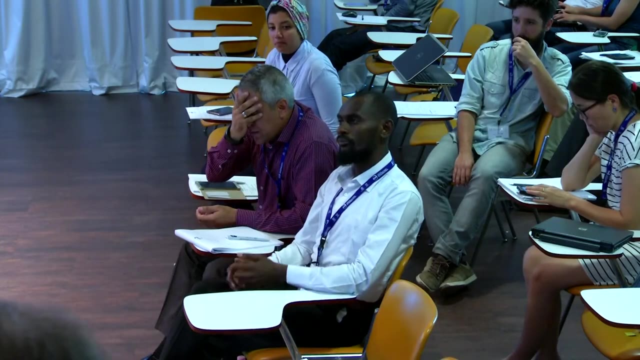 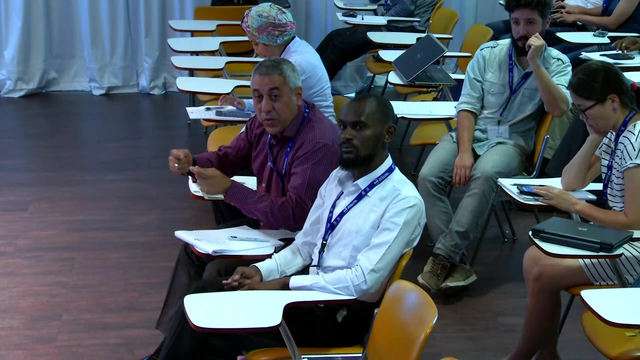 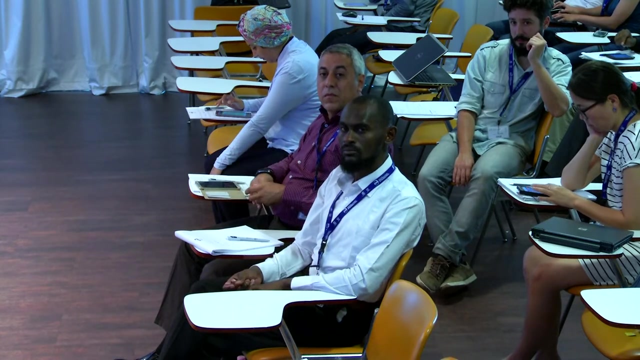 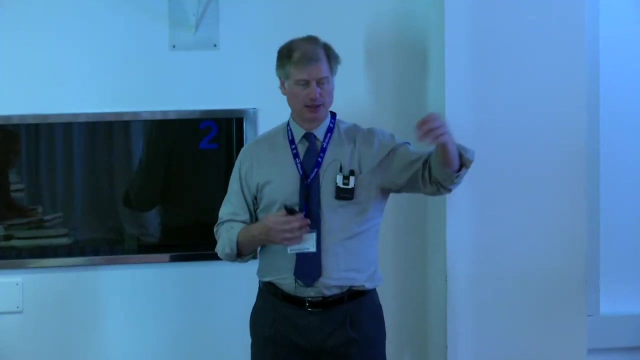 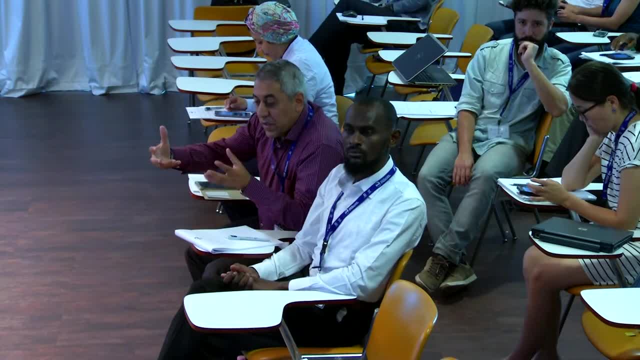 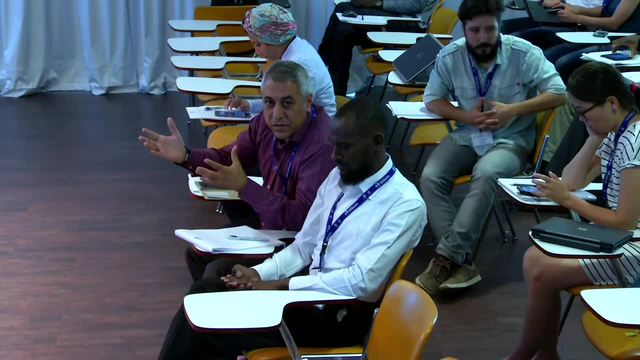 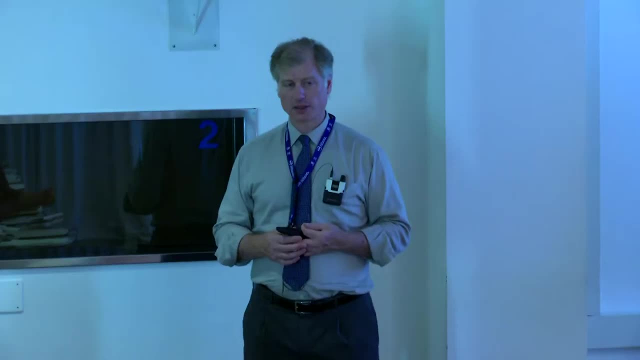 share that information. No, we don't really look at collusion. That's not part of it. As I mentioned earlier, two states are colluding on a field cycle on a clandestine activity. Both SKAGs are trying to make sure that isn't happening in both states. Now 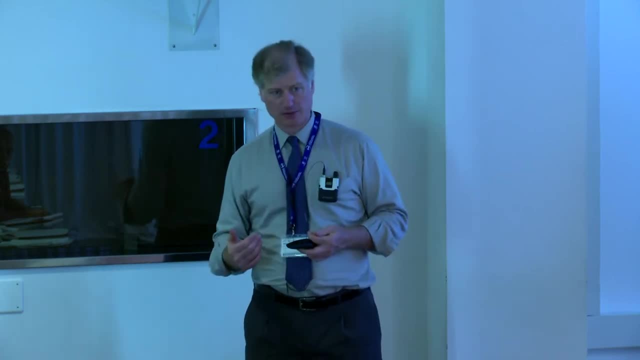 there could be cases. note, this is what you mean: work. one state may have something to do with it, another state may not have, And that's just a way of something that the other state needs. One may have uranium but no capability to enrich it. let's say: 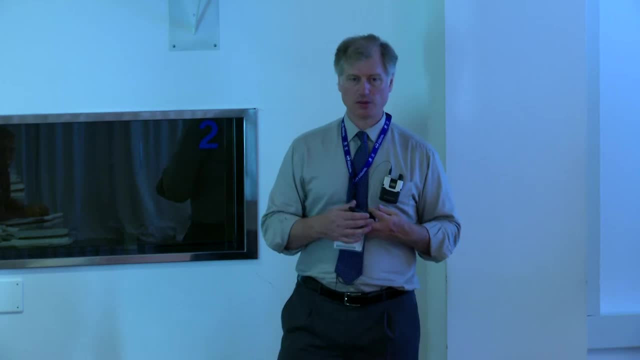 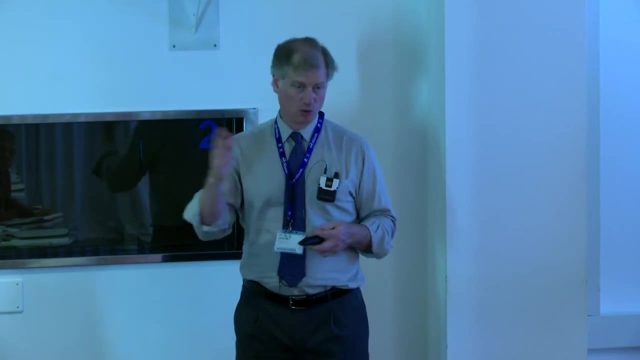 The other state may not have uranium resources but the capability to enrich it. So we would look for that in the state that has enrichment. We're also looking for any misuse of that enrichment facility. that involves domestic uranium or, I guess, uranium from another source, But generally as part of the exosympath analysis. 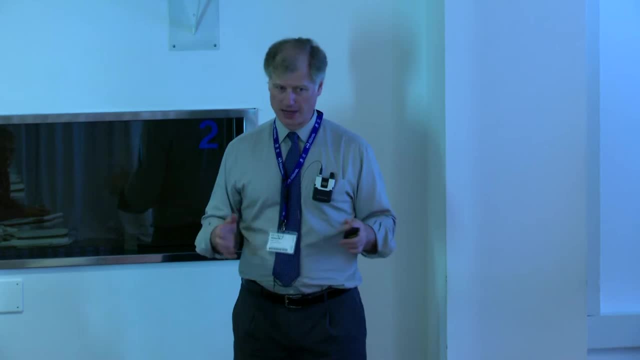 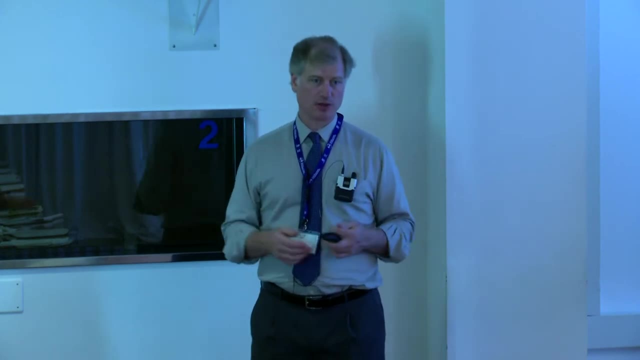 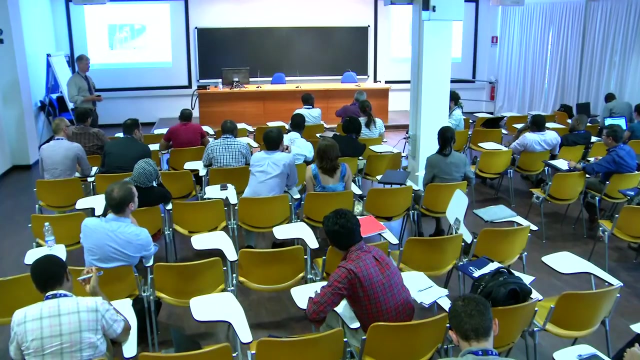 and the state-level approach. it doesn't consider that collusion is going on, But if there was information to indicate that, then those two sites would get together and share that information and assess it and run it to ground. Yeah, Good question. How much will the state-level agreement? 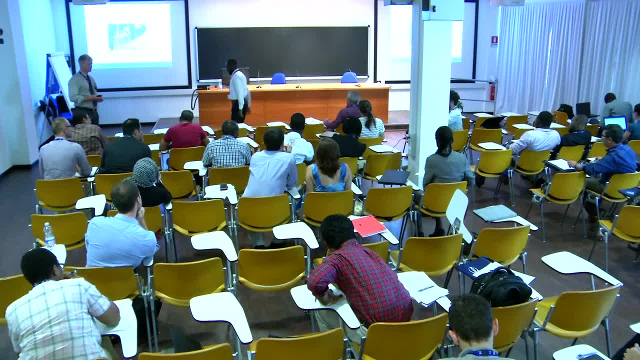 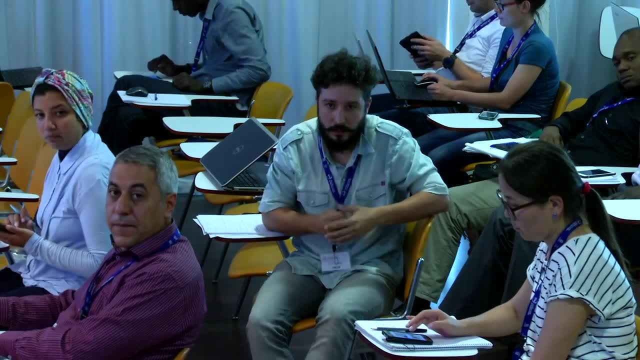 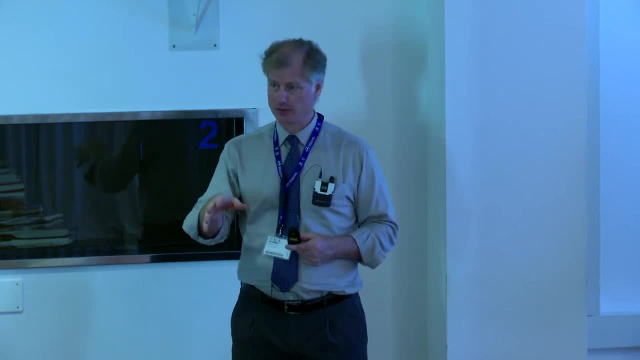 in Argentina, with Brazil. what do they expect? How much will the state-level agreement? That's a good question. I didn't mention it at all. In Argentina and Brazil, for example, there's a group called ABAC and they have their own arrangement. 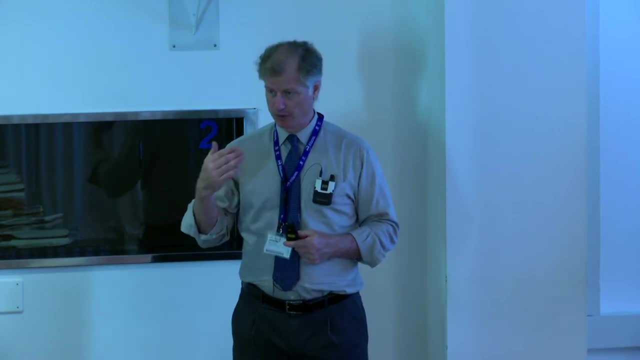 It started in the early 90s, When they both entered into what we call comprehensive safeguards agreements under 153, and they established their own SSAC, their own inspector, their own national inspector, but a little bit independent. So they have their state authorities, and then they have 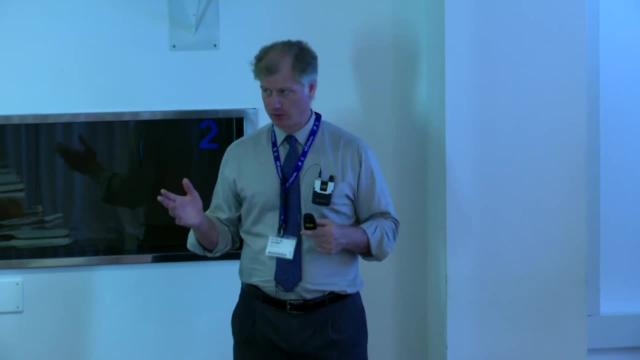 this independent, what they call a regional authority. Uratima is another major one. So over a lot of the European countries they have a European commission as their own inspector. From the agency standpoint, we would consider this and we work with them and they're counterparts. 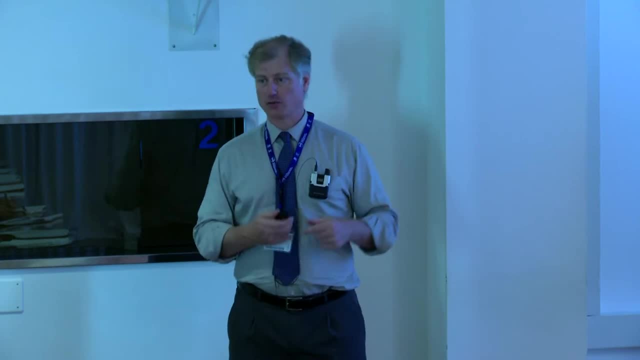 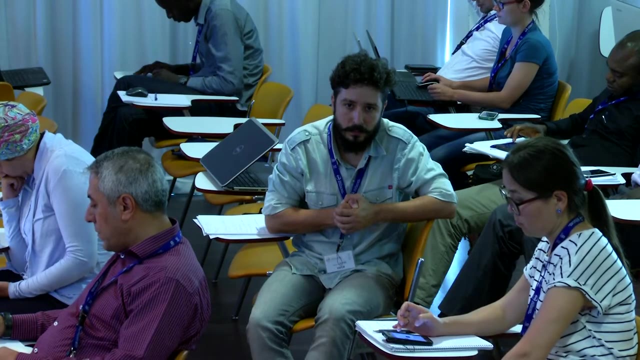 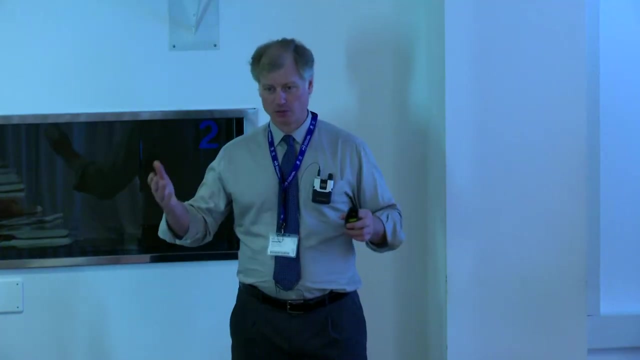 in terms of ensuring that we have a comprehensive safeguards agreement. Sometimes it saves effort because they also have similar measures. They have cameras and seals, and we'll take advantage of that. Generally, the agency has to derive independent findings. So I'd say we use this information and we work together, but we also have to be careful. 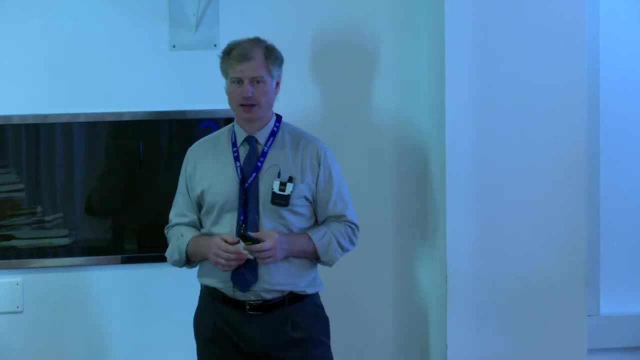 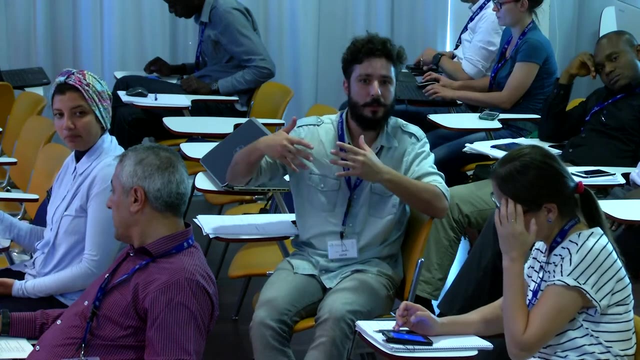 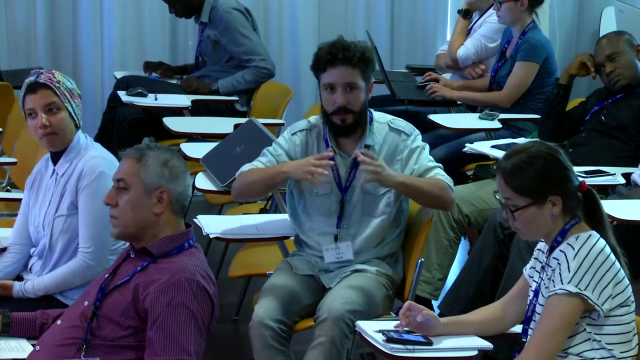 to make sure that our conclusion is independently derived. I have a question: How, from the point of view of the central college, the agency is designed, I think, to a fourth-generation reactor, but the reference would be based on more than 5% of the 20, so how is it working in terms of the new restrictions? Yeah, in general, the nuclear fuel cycle hasn't changed so much. However, I'm not as familiar with this fourth-generation or if we're going with fast-breeder reactors, but there are other ones that are coming down the pike that are going to create some interesting safeguards. 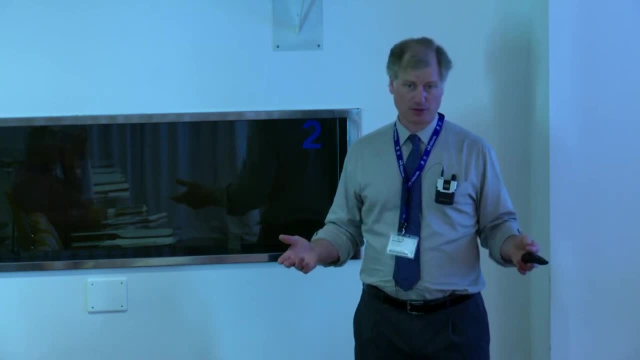 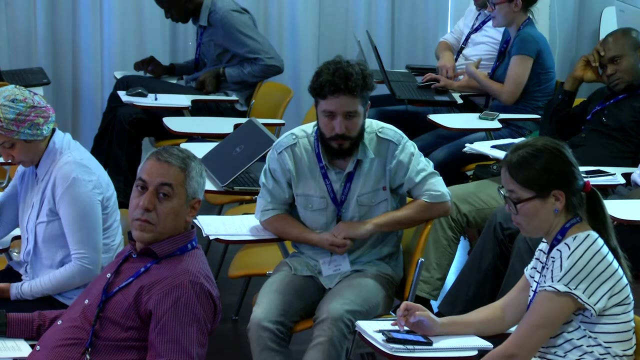 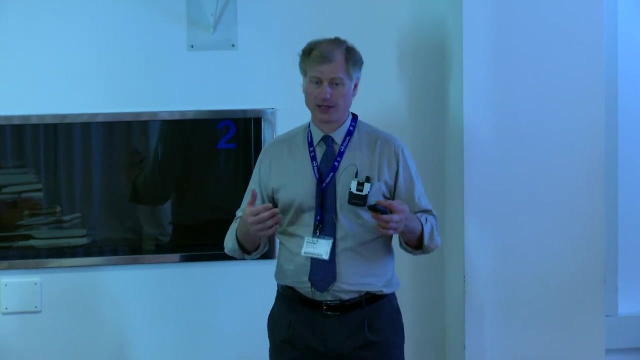 challenges. So we have floating reactors. So there's a few countries now- France, China, Russia- that have designs and actually I think Russia's built and I think France and China are close to commissioning these units. And there tend to be, and right now it's not really an issue for the agency because these are nuclear weapon states And again, the lawyer will go into this tomorrow. Under the NPT- when that was established in late 1969, came into effect 1970, there was five states that were nuclear weapon states And they got out of a lot of safeguards. so this would be one area. 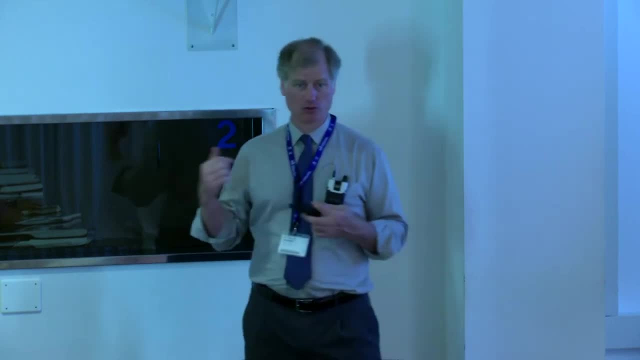 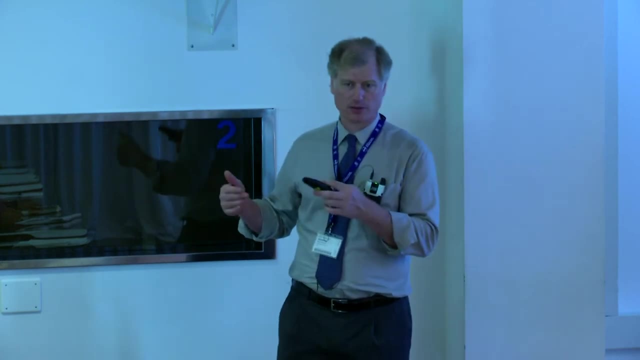 So it's not under safeguards. But if they export that technology, let's say, to a coastal region that wants a floating reactor or floating barge. I don't know what the thermal power is. I think it's on the order of 200 or 300 megawatts. 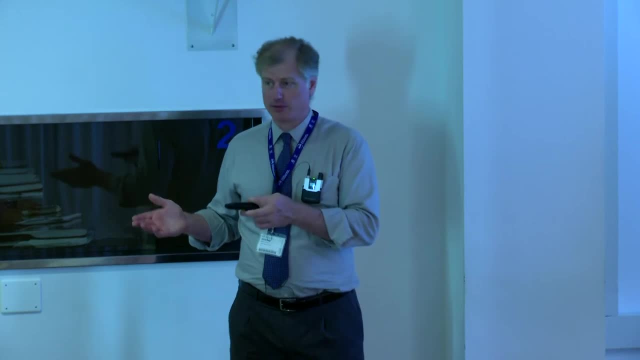 So it might be good for a small-sized city and it could have some advantages. You provide electricity. maybe the state's developing and they don't have the time to develop their own infrastructure, and then, when they no longer need that electricity. 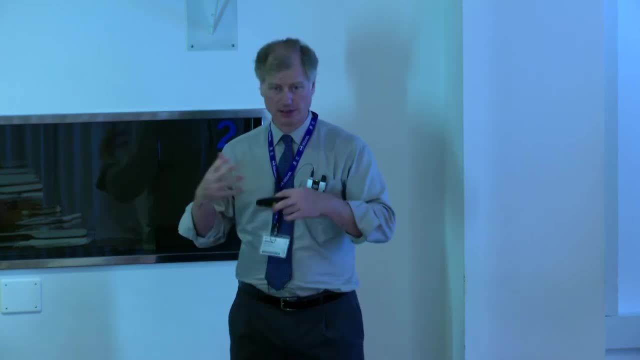 well, the host country just pulls it back. They're their own country, so it's gone. There's no D&D, no installation on your soil, no environmental, long-term D&D. so it has advantages. So these are the types of innovations we'd have to say. 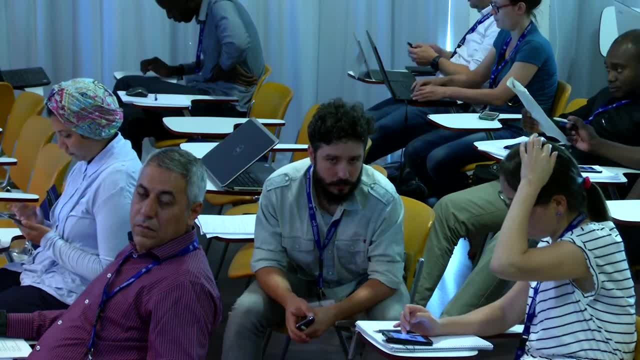 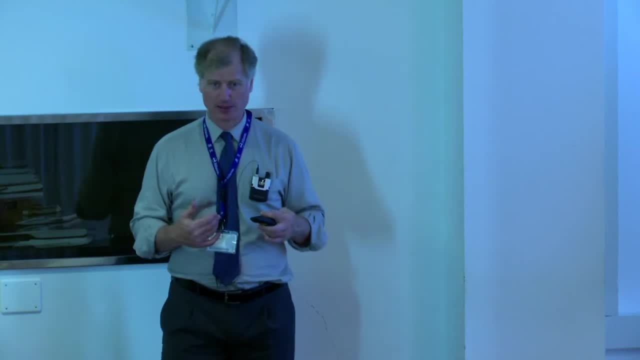 We have to figure out a safeguards approach, not safeguards how to safeguard this, because essentially it could become a step. So we always come back from an analytical standpoint. Again, I'm probably staying up nights, maybe overly suspicious, but I'll say: how could? 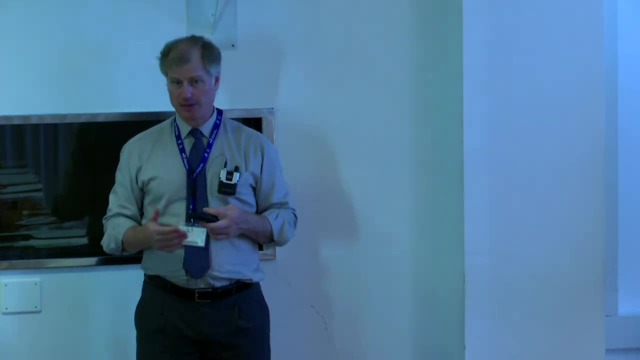 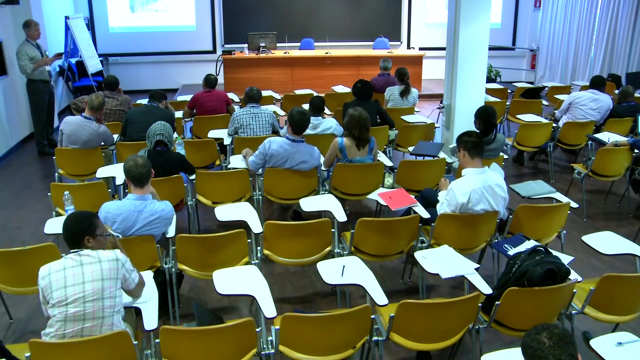 they misuse this floating reactor? The state that gets it. Maybe they can't, Maybe they have no control over the reactor- It's still under the state that provided it. but we would still look at it that way and then apply certain measures. but it's good to get in on the ground floor because we can. 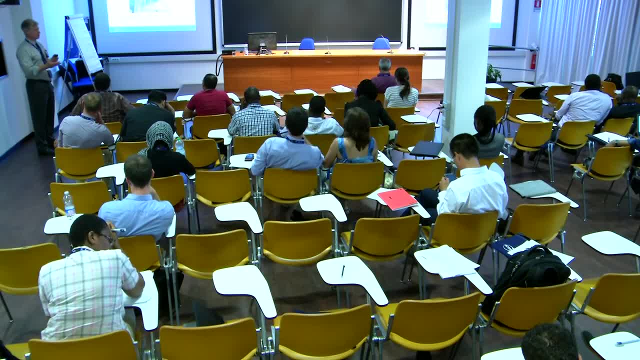 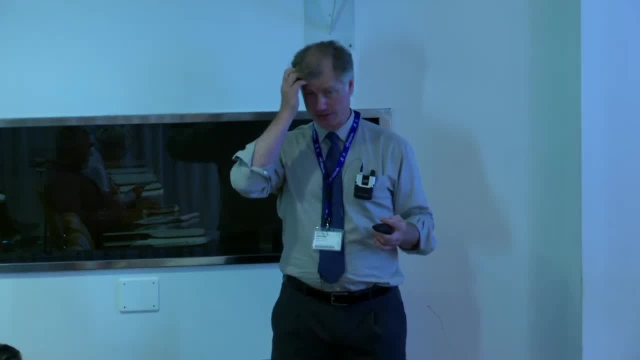 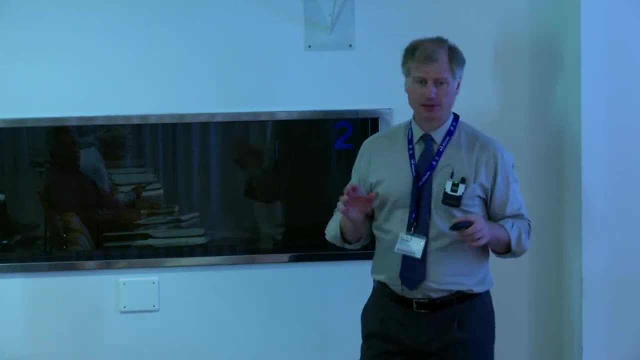 maybe make it so it's very difficult to misuse this or, if it is, we would identify it very quickly. Another example: I was at a presentation on small modular reactors and there's a company in Canada that wants to use these in Canada domestically, mainly for remote areas, and 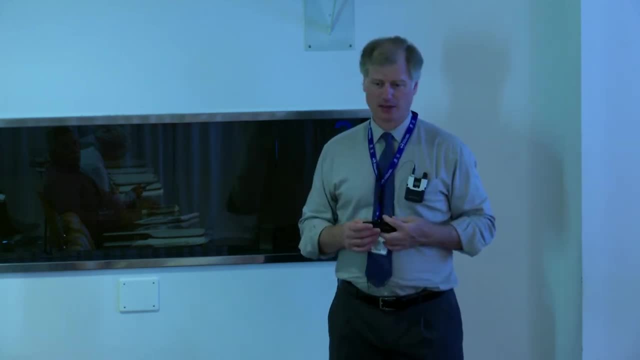 they're generally low. They have thermal power reactors. I mean, they're not. I don't think they're building yet, I think it's still just a design idea, but I think it's been approved, the design, And that's a challenge, because now we start to disperse the power. 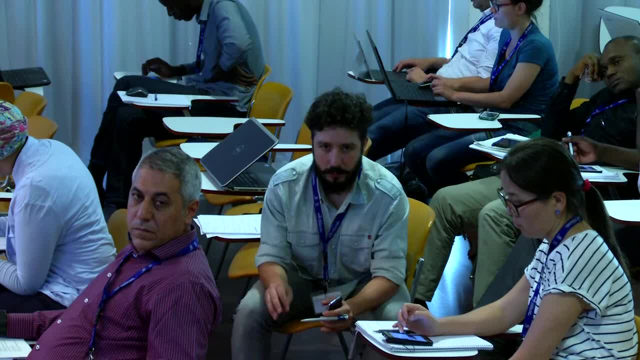 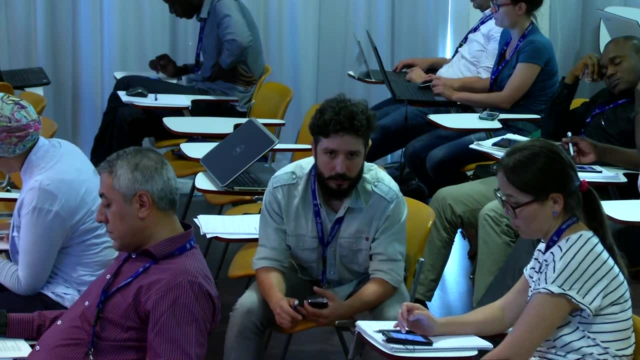 So instead of having a 1000 megawatt plant in one single place, a single address, maybe a couple of units at one site, now you're getting maybe 10, 20, 30 of these dispersed and for candidates to hit remote regions where they have mining: 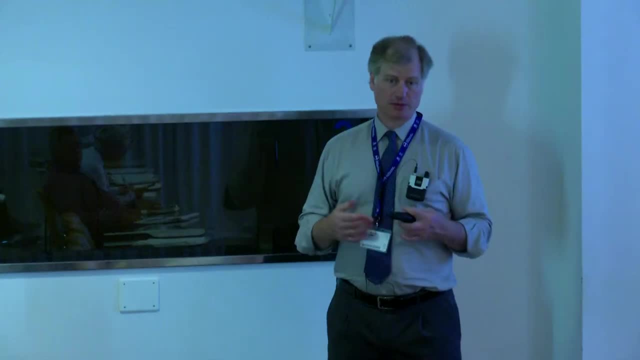 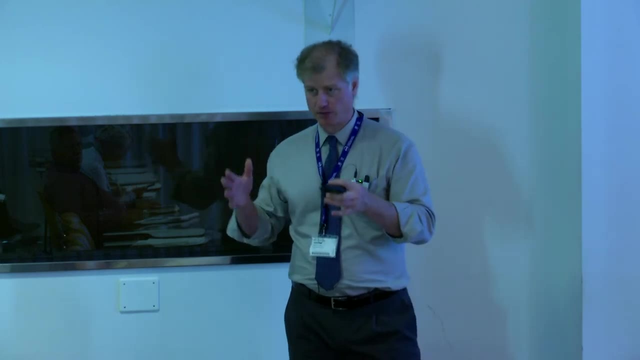 but they need a power source, So they're not going to be able to get out of the reactor, But we still have to safeguard it. But if this can be fairly, you know, kind of like a maintenance-free battery, if it's a maintenance-free type reactor. it just goes in place, is used, so it's spent, let's say, a year or two, three years, whatever it lasts. The company comes and takes the small modular reactor back and replace with another one. Then we just have to safeguard. 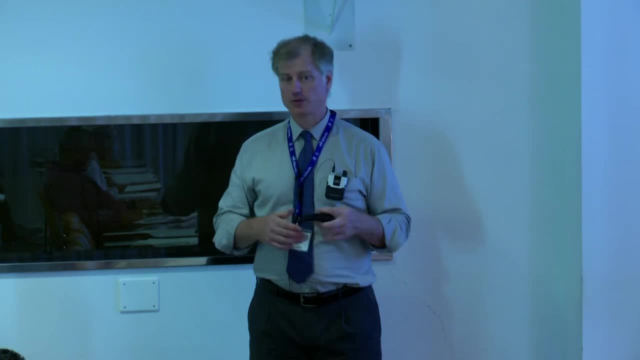 It's basically an item, a unit. It's not so much something that could be misused. Perhaps we use something different, like satellite imagery, some type of global positioning. So we're constantly trying to innovate And I think that's a challenge. 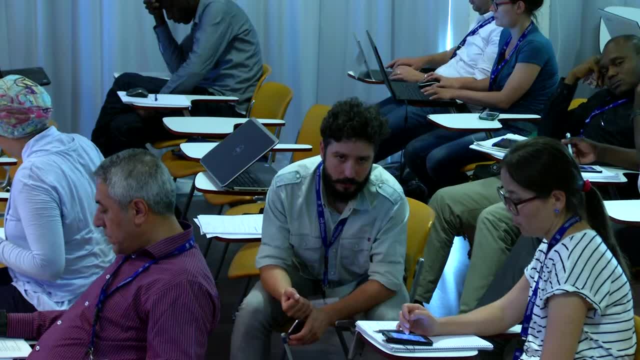 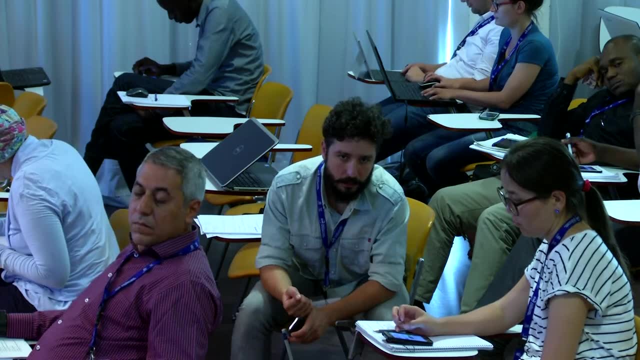 And our technical measures. if there's a new way to safeguard something And if we find out about these next-generation technologies, we can get into it a little bit sooner. Fast-breeder reactors are hard, because I used to inspect at Manju. 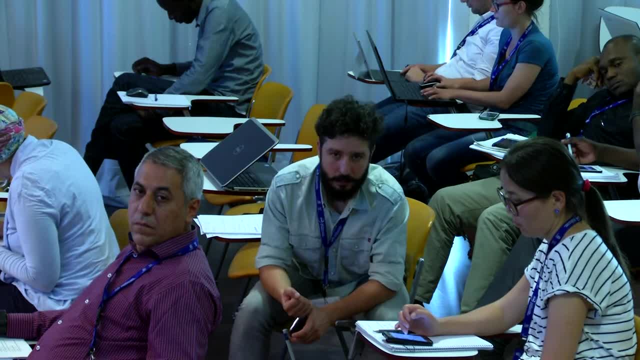 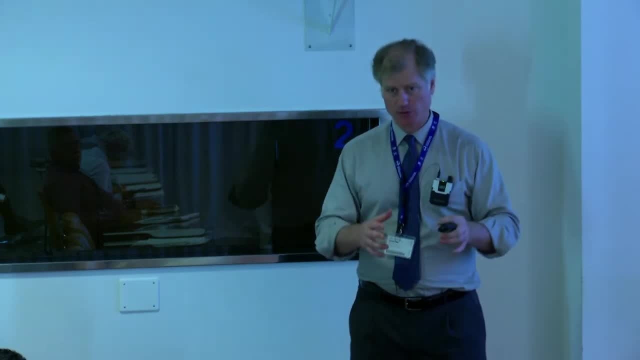 And anything that has liquid metal or anything just becomes a problem because usually it's not transparent. So at normal LWRs we're used to seeing above the water. We see the fuel, We can item count, We can keep an eye on the fresh fuel, the core fuel, the spent fuel, et cetera. 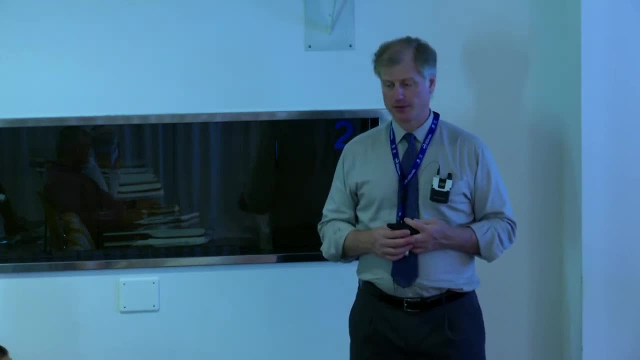 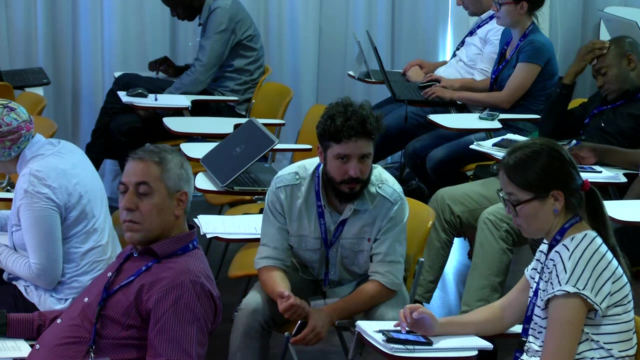 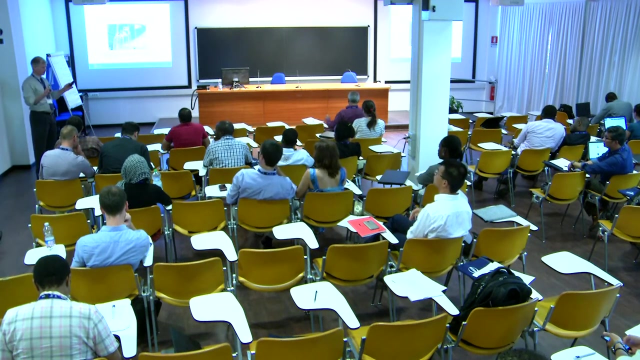 It's key. It's key measurement points, But for a fast-breeder reactor this gets a lot messier quickly. In fact, at Manju there's a lot of installed non-destructive assay-type gate monitors to monitor where the fuel is flowing. 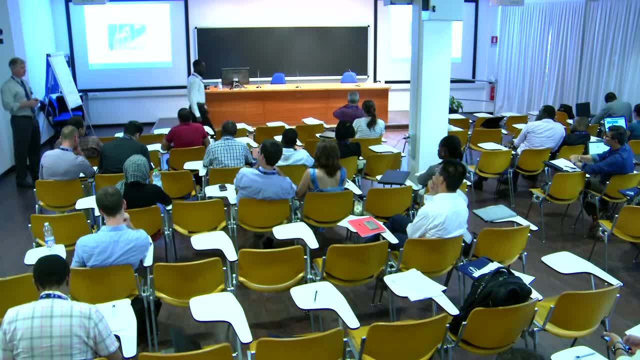 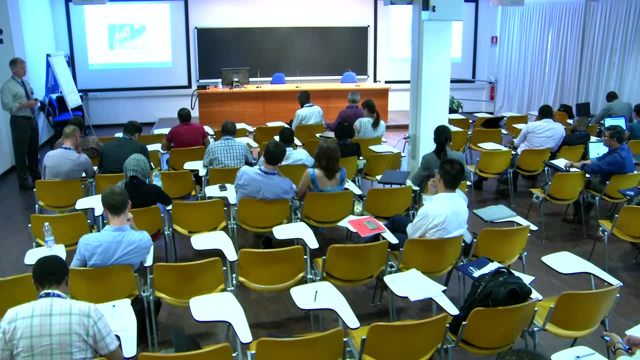 That reactor is actually shut down now. It was going to be brought back online but it never – they had a small incident, but it never came back online after Mishima made it home, But I'm not sure of the latest with that type of one. 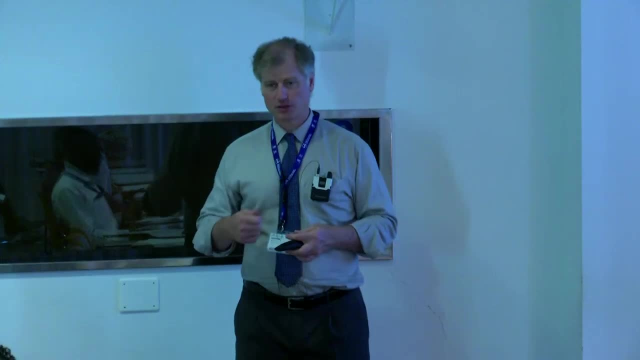 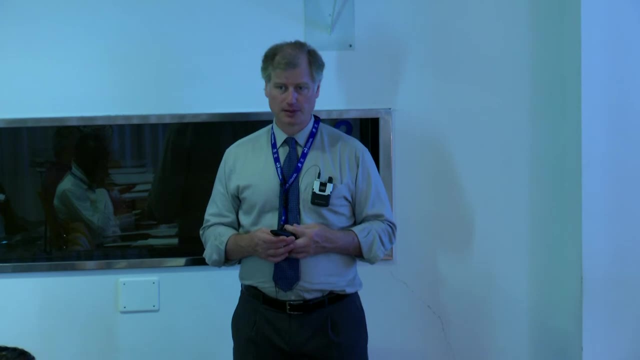 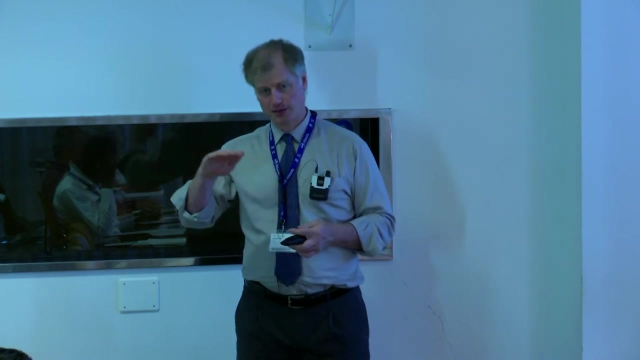 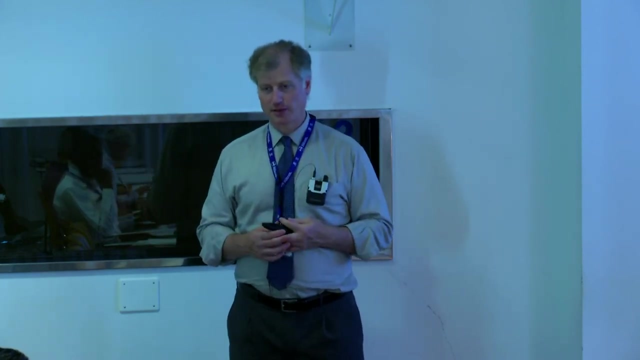 But there aren't too many of these exotic reactors, fairly just the traditional LWRs, PWRs, BWRs in Canbu. So it's a fairly traditional nuclear fuel cycle. My own view is: I think the nuclear fuel cycle after Three Mile Island and then Chernobyl is making a recovery and then Fukushima and some parts of the world- maybe mainly in the West- it's really slowed things up. 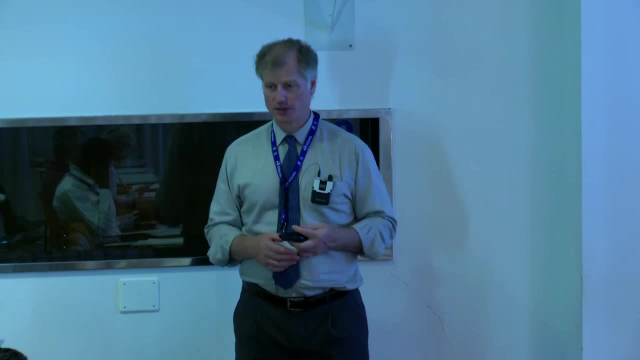 So countries like Germany change course. They started shutting down reactors So their nuclear fuel cycle is kind of in decline. I think a few other states- Switzerland is another one- that might be reconsidering their nuclear fuel cycle plans for the future. The US had a couple of reactors. 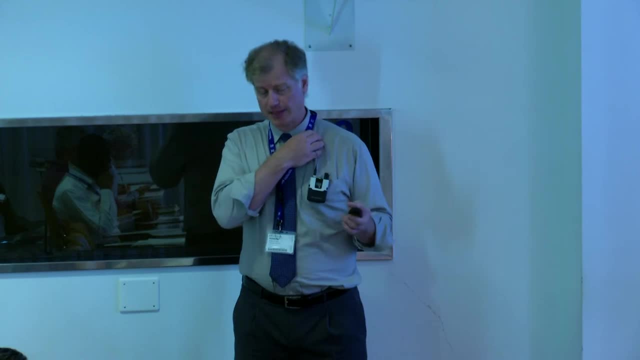 I think it's South Carolina- that were about to come online. I think those are on hold now, Maybe not just entirely because of Fukushima, because that was six or seven years ago, but also because they're finding that something. But they tend to be fairly standard, tried-and-true designs. 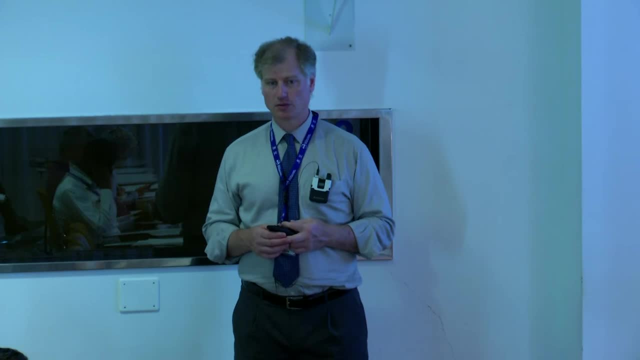 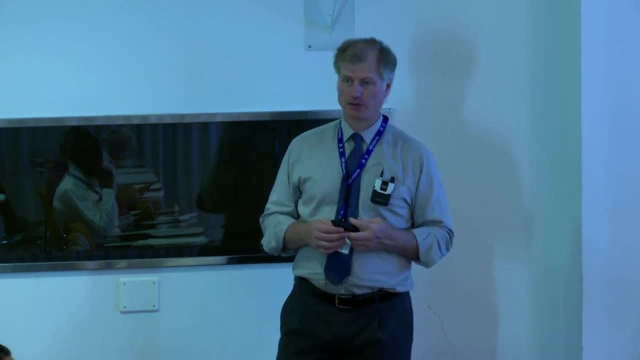 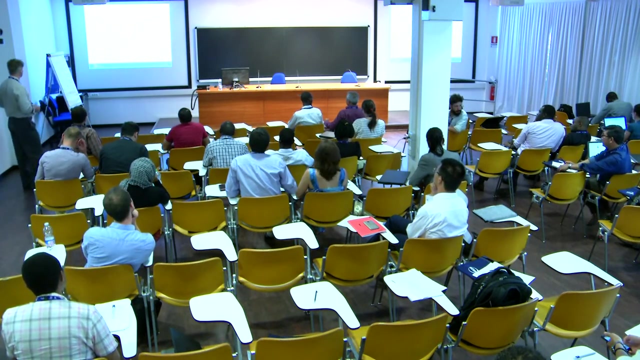 But there may be some breakthroughs And then the safeguards challenges will arise. Any other questions on safeguards, safeguards applications, inspecting analysts, anything like that? This one Or this one? Okay, That's a good question. Most states are, I mean, members of the IEA. 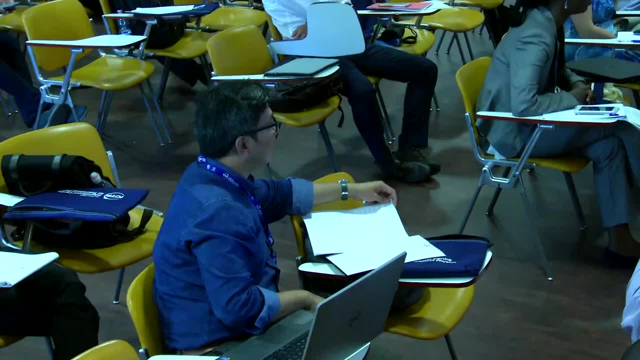 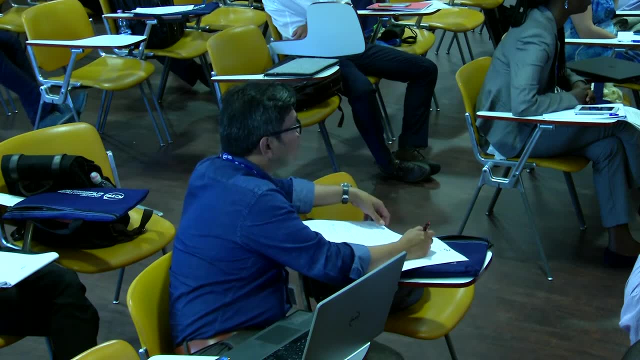 Well, no, they're not members of the IEA, but I mean, you can be a member. It's kind of tricky. It's a good question for the legal guy tomorrow. actually, You can be a member of the IEA. 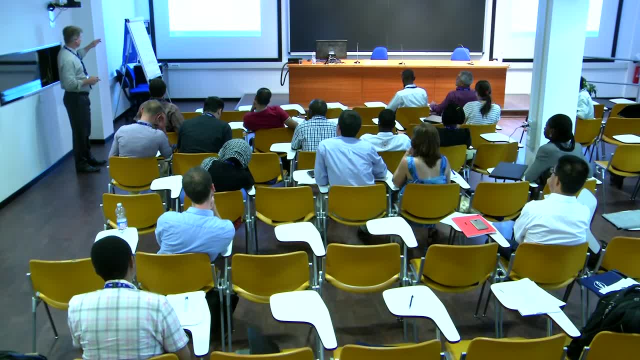 You may not have any nuclear material And you may not get a. basically, if you have a comprehensive safeguards agreement in force, if you have a CSA, you get a conclusion. So there might be a handful of states- I'm trying to think maybe small Pacific Island-type states- that don't have one. Or there could be a new state that comes about, like South Sudan, that's still working out their agreements or something and they're not in effect yet. something like that. I don't know, But generally this would apply to all states. 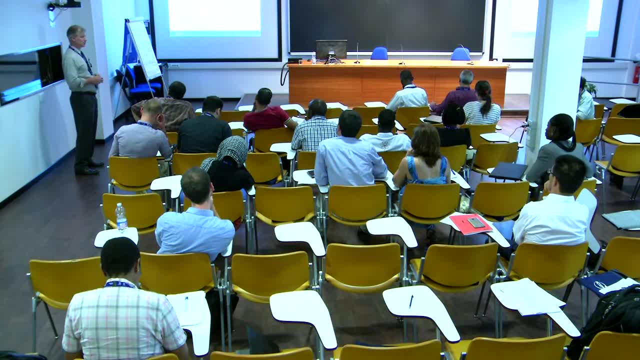 It's about, let's say, like 181, 182 member states. But if you don't have nuclear material, we would still. there's something I think I should highlight: If you have a very small nuclear fuel cycle, we just almost. 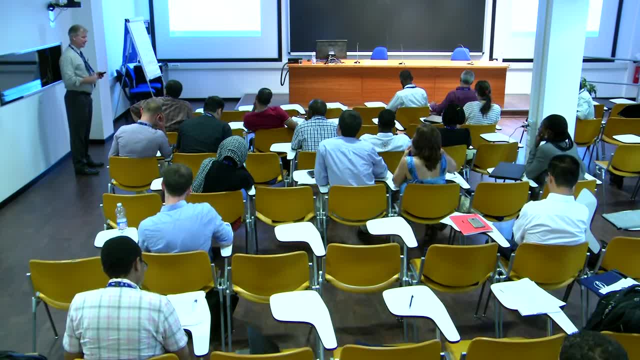 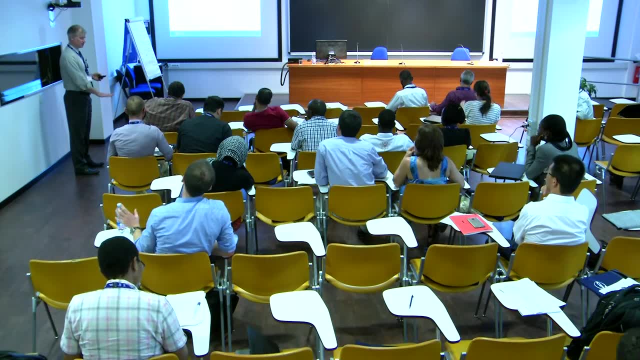 if you have nothing, something called a small quantities protocol where legally you don't have to get all the bells and whistles of a comprehensive safeguards agreement as long as you stay below a certain amount of nuclear material. So it's very low levels. 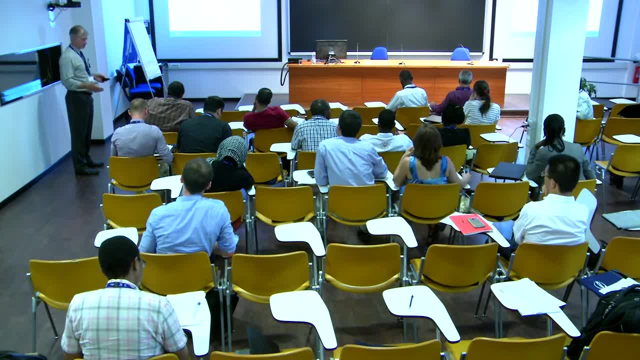 You couldn't. it'd be very difficult to acquire weapons with nuclear material because it's just very limited. So we call that an SQP status. As long as you meet those eligibility limits and the criteria for that, you can have this. 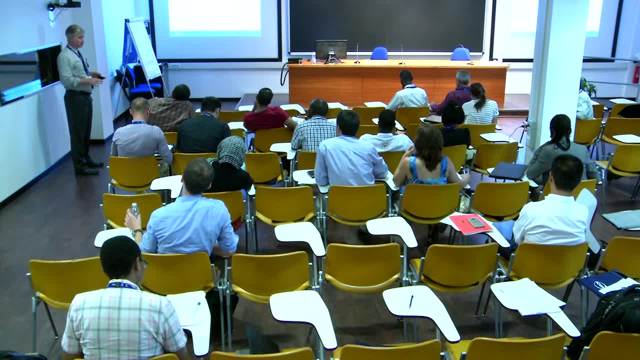 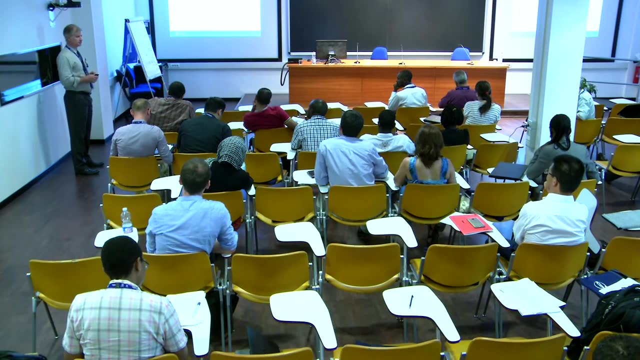 We would still draw a conclusion but we'd do a lot less in that state because there's a lot less nuclear material and the agency would just verify that. Very infrequent It'd be every. it might just have a loft, a location outside of a facility, a small university-type thing that might go there every three, four, five years. 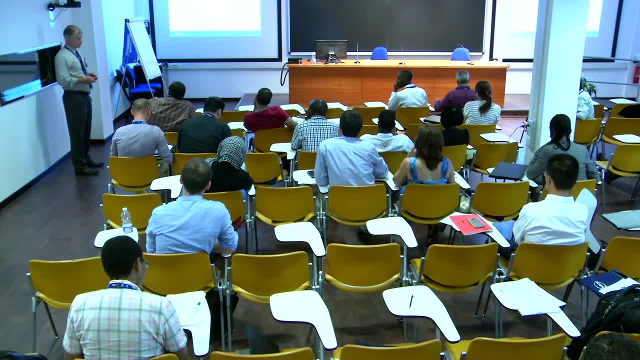 But generally there would still be a conclusion. Sometimes we didn't do much in terms of activities to support that conclusion, but over time we do, which we would, So over a three- or four-year period. So there's something we refer to as in the statistical inference. 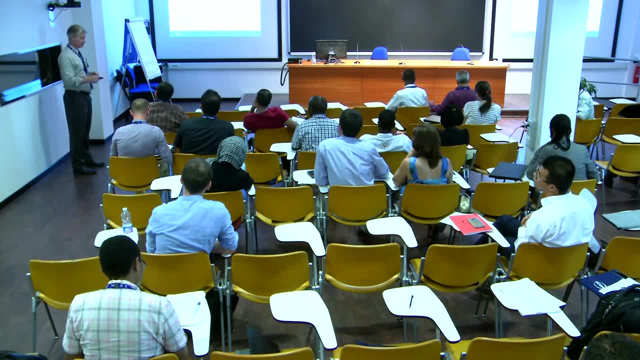 So even if I didn't select that to be verified, that's fine That facility, that nuclear material, I can still broaden that because I could have selected the entire population over certain times And I can still make the case that I could have shown them. 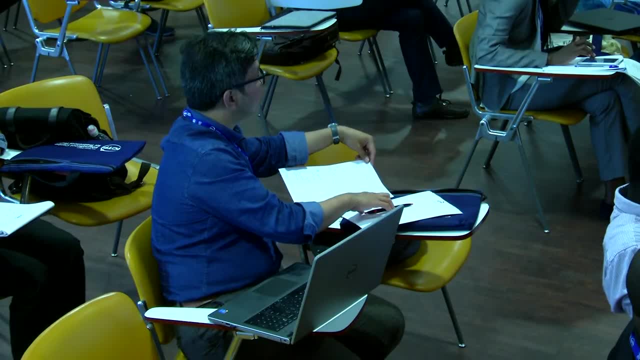 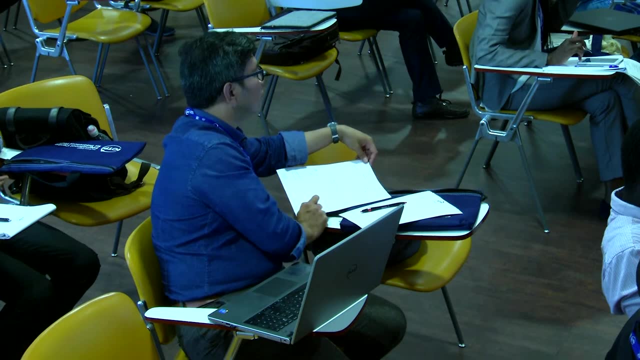 I could have verified them. Now, if it's a very low selection probability, it starts to get a little shaky. It's got to be a certain amount And there's a whole section of statisticians at the agency that confirm these types of selection probabilities and detection probabilities. 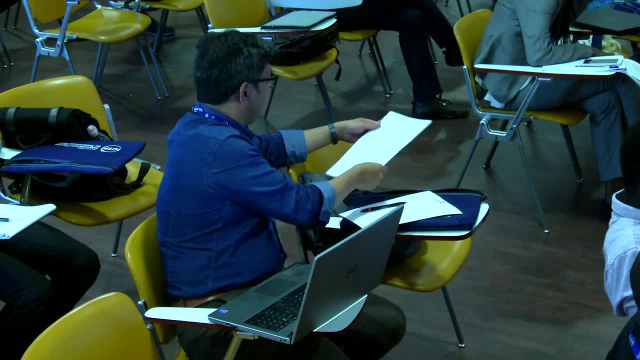 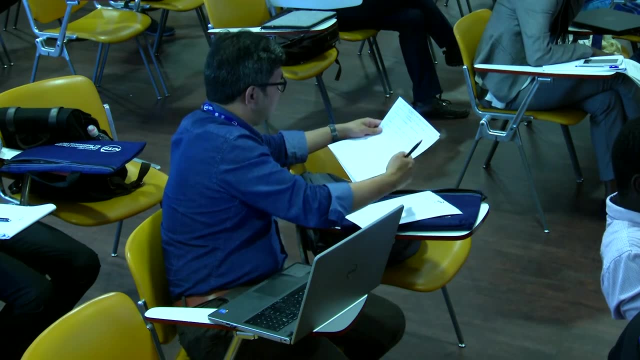 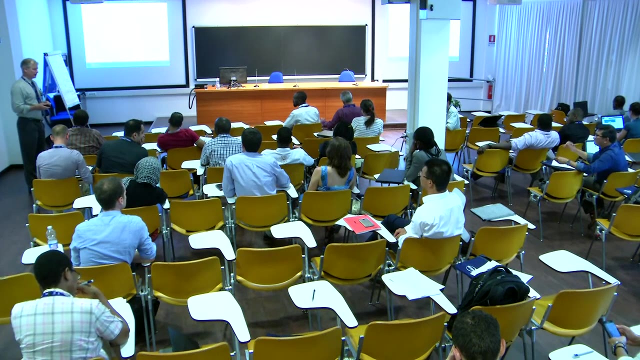 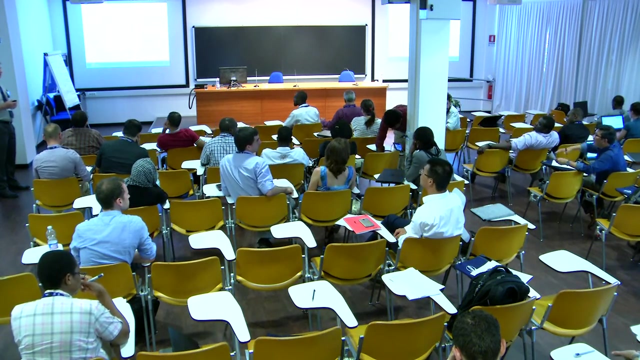 Yeah, It would depend on their agreement, and unless it's, let me say, a nonmember state, I'm not totally understanding. Well, it may not be their call, because if they want to be part of the NPT, if they 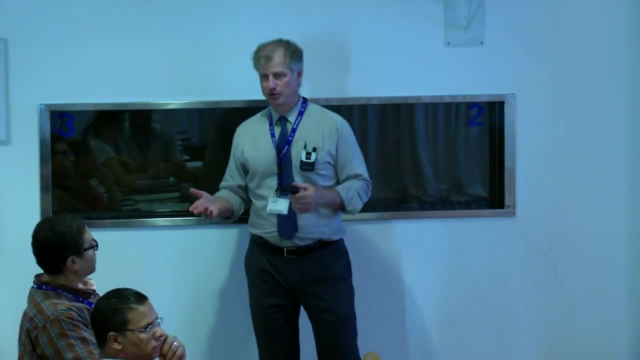 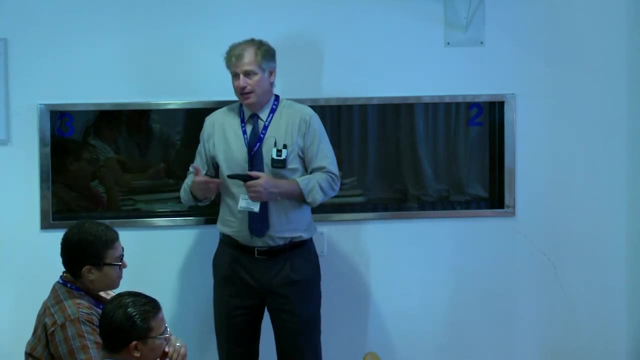 sign on to the NPT, then they have obligations associated with that. One of them is they've got to declare all their material and their facilities and they've got to open them up for inspection. So if they didn't do that, they're not in. 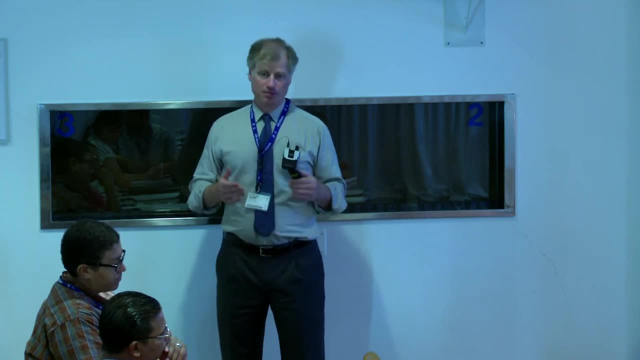 compliance with the NPT. basically We would be a little bit lower in the sense of we're confirming a comprehensive safeguards agreement, but that's coming directly out of the NPT because they they have to put this agreement in place. So they would not be basically wouldn't be meeting their wouldn't be in. 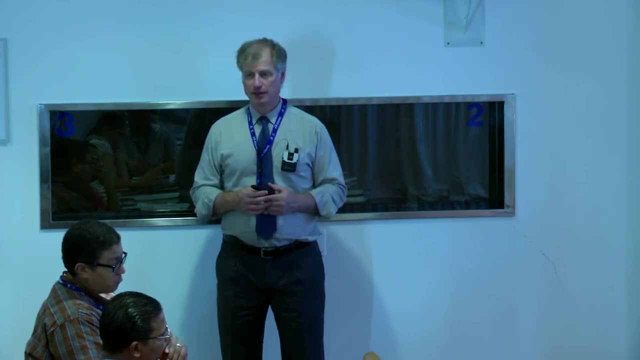 compliance with their agreement And they definitely wouldn't get if they had new material. we have to access that and provide a conclusion And sometimes you know I'm thinking about this and you know the segs will get. the state evaluation group should get caught up and I think you know we're not the 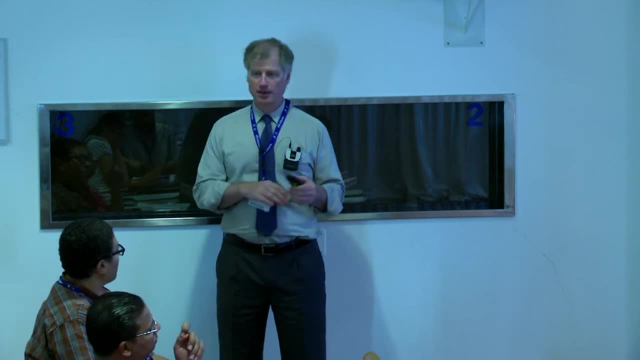 agency. we don't work here at the agency to draw conclusions for ourselves. That's so we can put out a nice document. This is to provide credible assurances to other states that might be concerned about that state Say nothing is going on in that state. So if we can't draw a credible conclusion, we 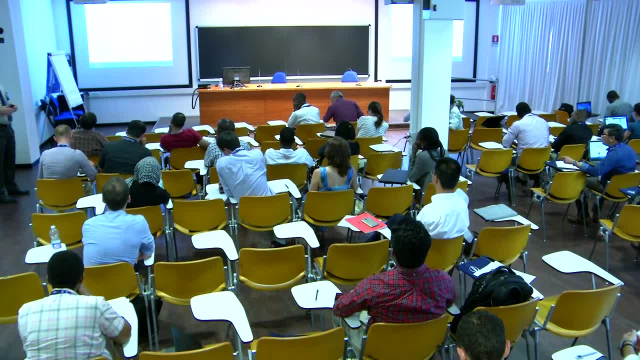 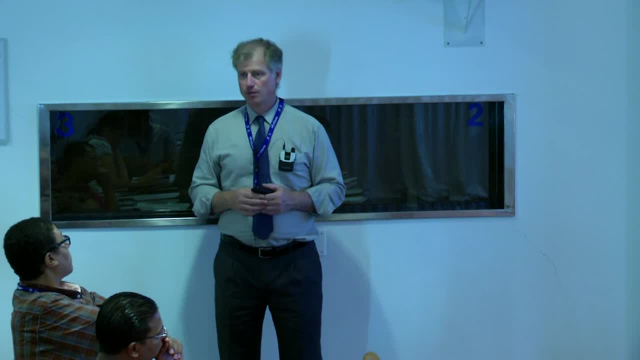 can't, we can't, we'd be misleading, We're giving a false sense of assurance. So we have to make sure it's technically sound and if we've done enough activities and met those technical objectives I was talking about, then we could hopefully meet that sound and credible safeguards conclusion. But people you know states 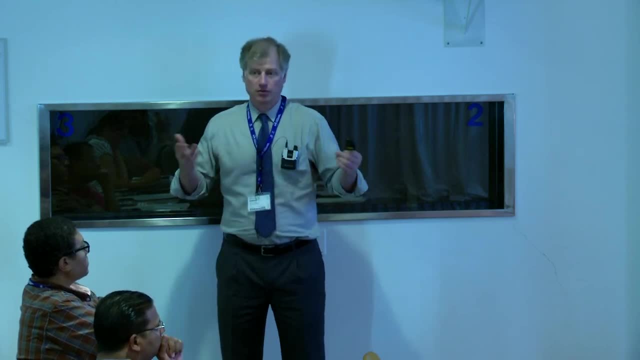 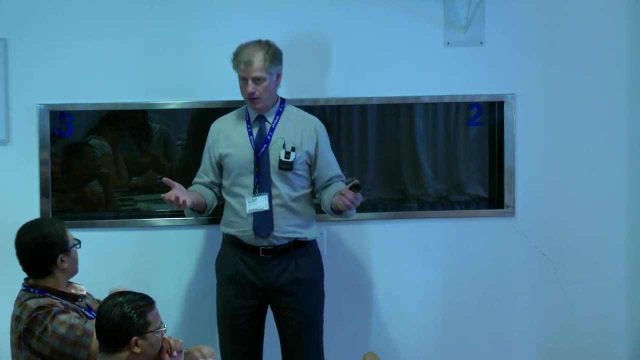 are relying on this because they've committed it, though they've joined this, this group, this treaty- say, okay, we'll join this treaty. We're giving up some of our security sovereignty in a way, because they're also committing that they're not going to pursue nuclear. 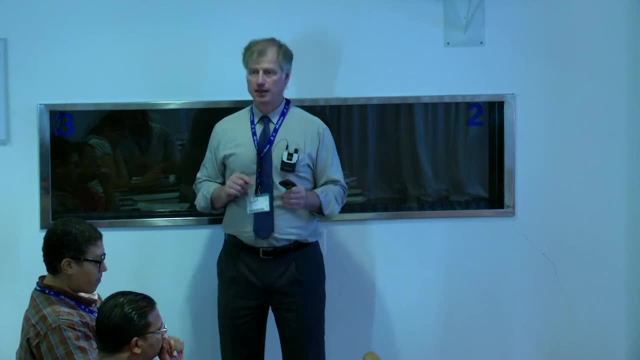 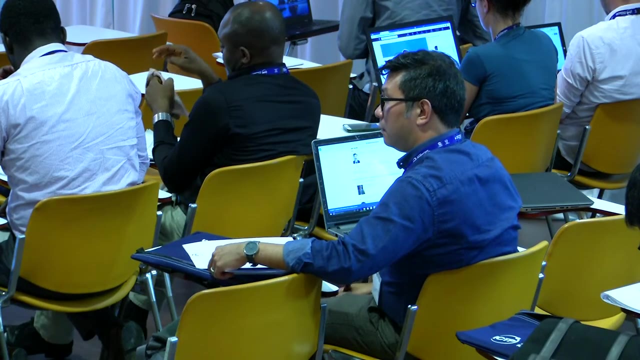 weapons, but they're expecting everyone else to be doing the same thing and they're relying on the agency to make sure everyone is doing that. So if someone is playing a game, it would be obviously incumbent on the agency- if that is the case, and we confirm that- to communicate that to the wider non-proliferation. 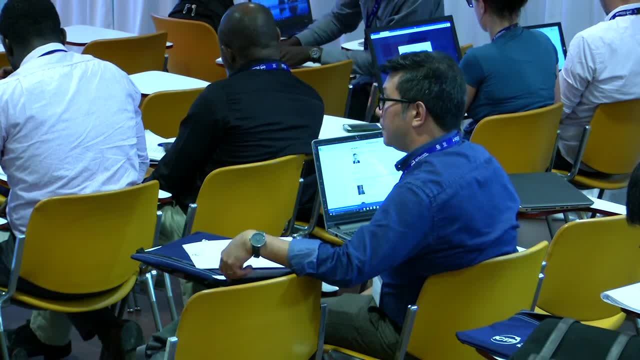 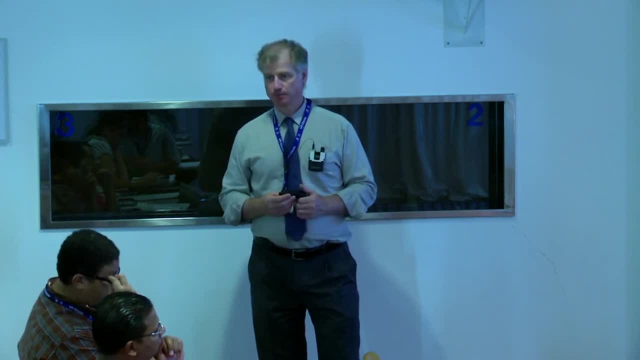 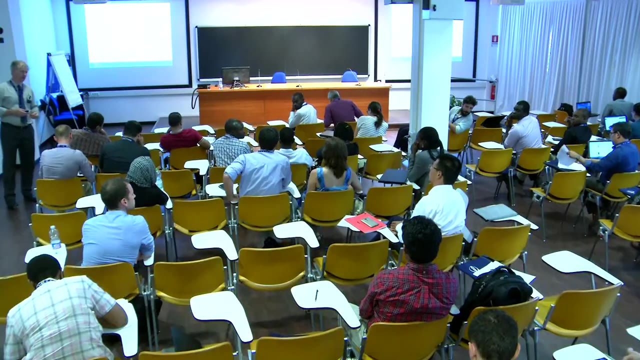 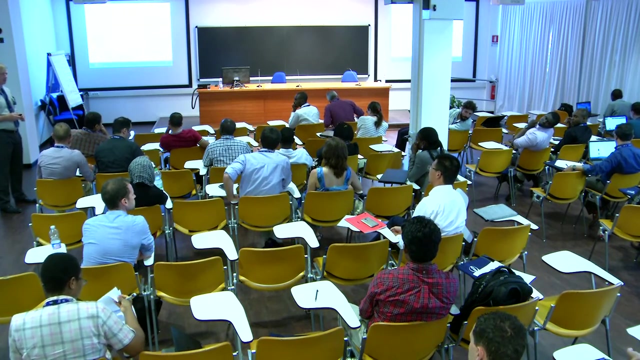 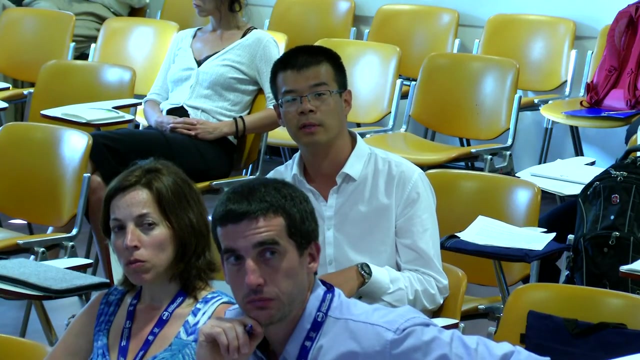 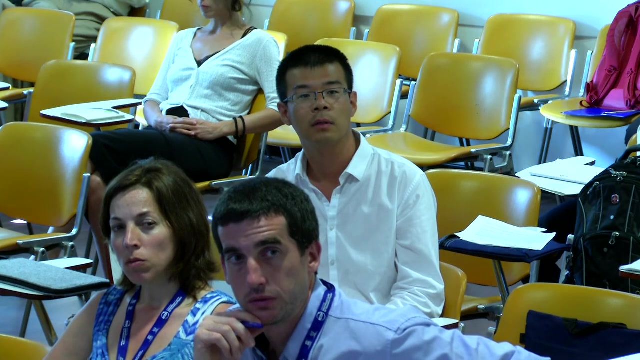 community And that's what happens to this safeguards implementation report. Annually we provide these conclusions. Any other questions on safety: Generally the information wouldn't be directly shared if it came from- that's highly, that's highly confidential information that came from one state. 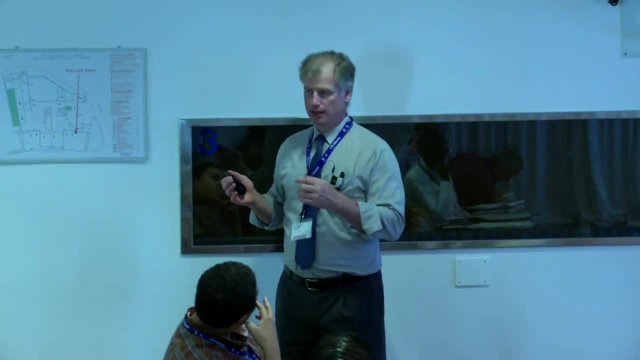 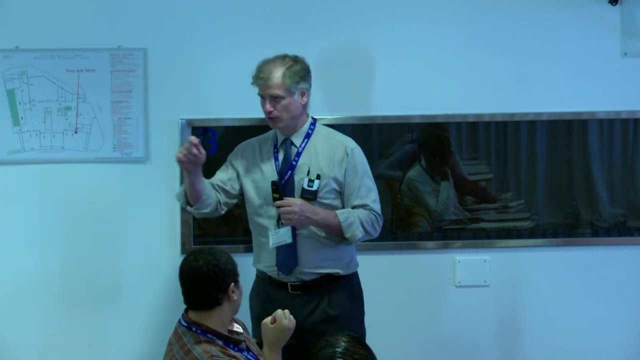 let's say the Nipton County or some sort of declaration, and the agency has to be very careful when they handle that information. but if I understood the question correctly, would we provide that information directly as evidence to another state? No, that wouldn't happen. The fact that something might be 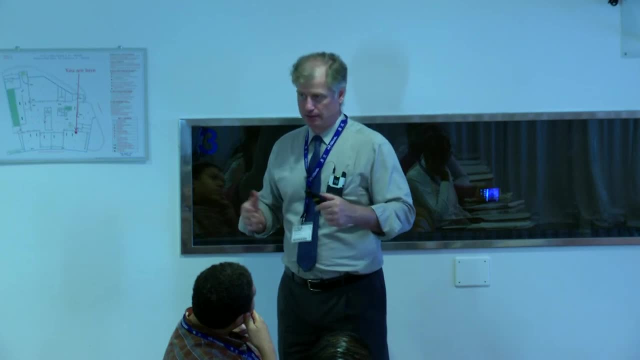 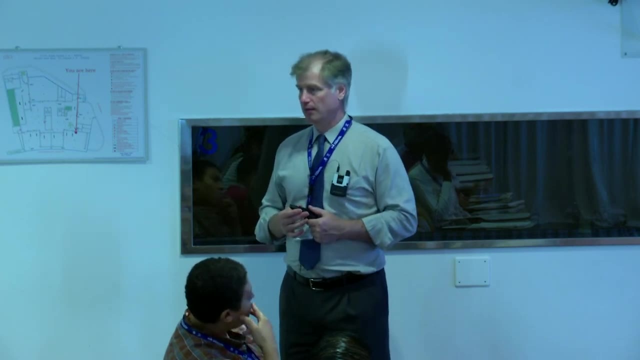 occurring or the allegation that might be communicated, might be communicated to a wider audience. First, that information would have to be corroborated, usually for other sources and other independent means. before the agency just jumped out on some limb, You have to make sure it's sound. I don't know. 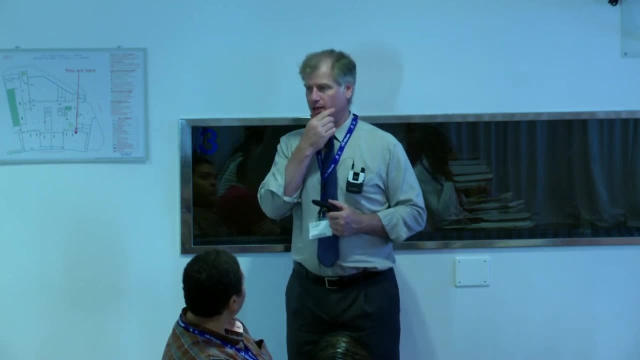 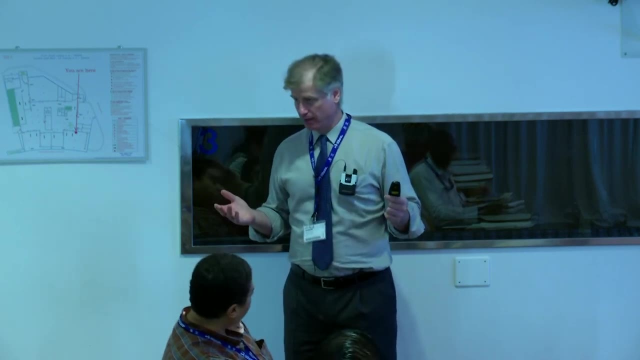 you know, in our safeguards implementation report there was a case in Syria, I think in 2007. they were building something and it was bombed. so the way the agency found out about it, as far as my understanding- I don't work on that state of variation group- was it was in the newspaper- basically because Israel bombed this reactor. this 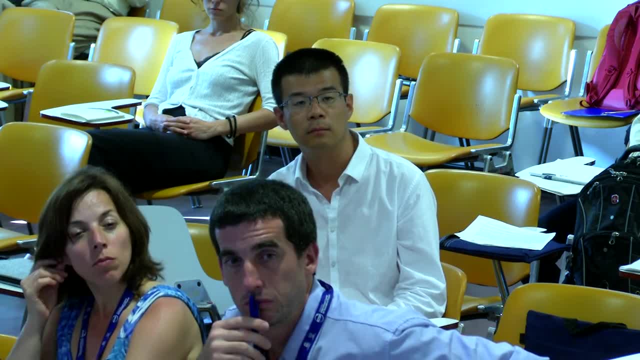 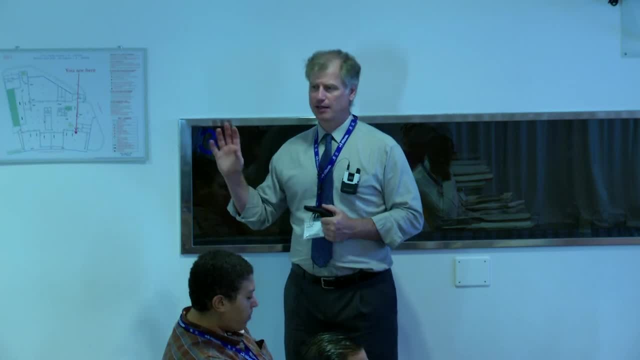 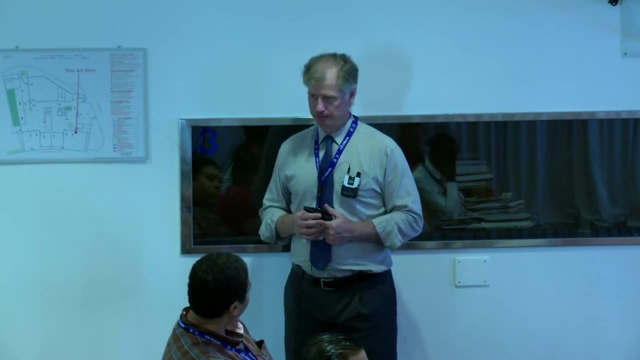 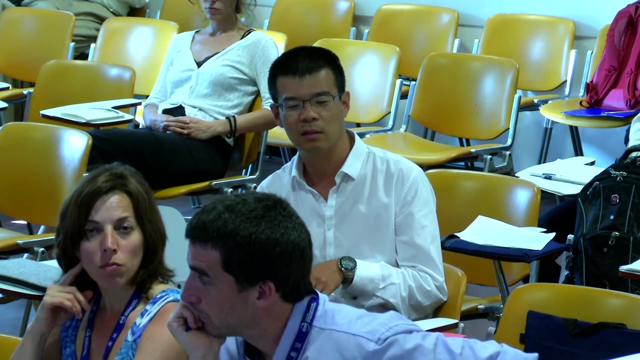 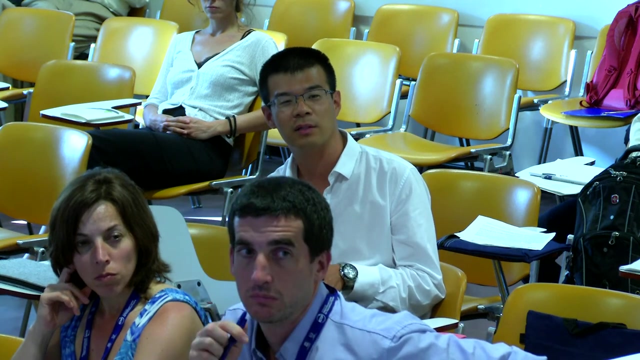 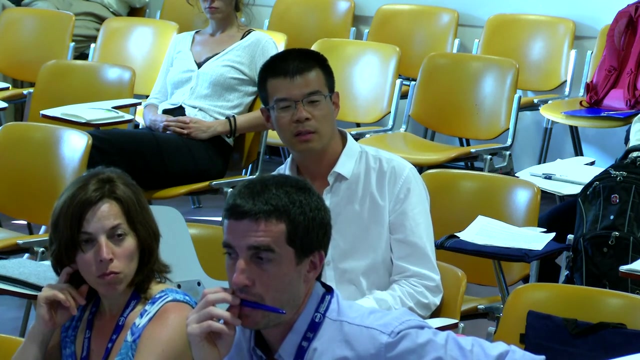 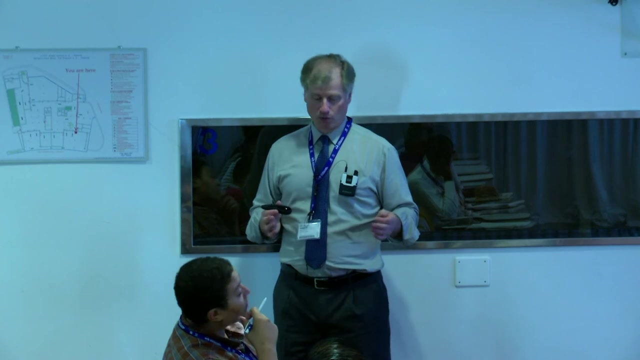 probable reactor. So I think in the early days the wording was it's a possible reactor and the agency official wording and terminology and then later, I think in the 2000- sure exactly 12-13 time frame, it turned into a probable reactor. I don't work on that state, have never expected in the states. I'm just giving you my own personal. 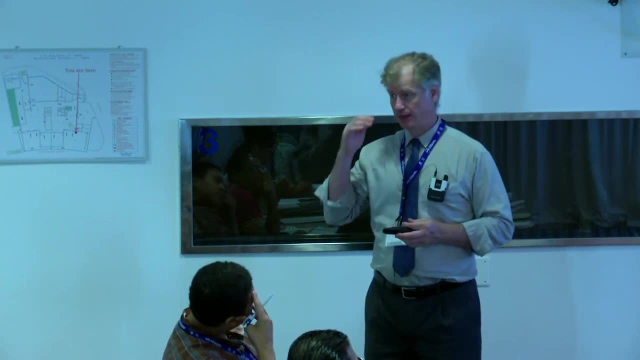 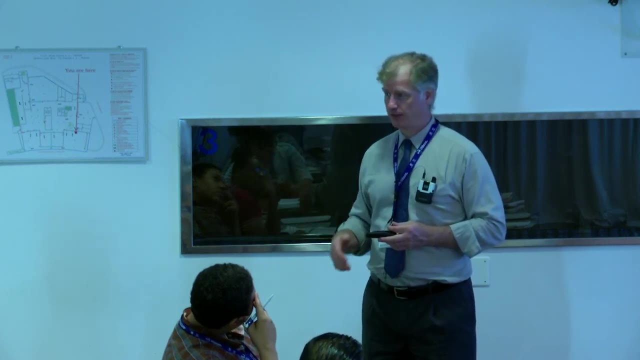 view, your opinion and speculation. I think that's a state that has their own security concerns in isolation and probably going back to the 70s and 80s, obviously is still just an armistice in terms of peace on the Korean Peninsula. 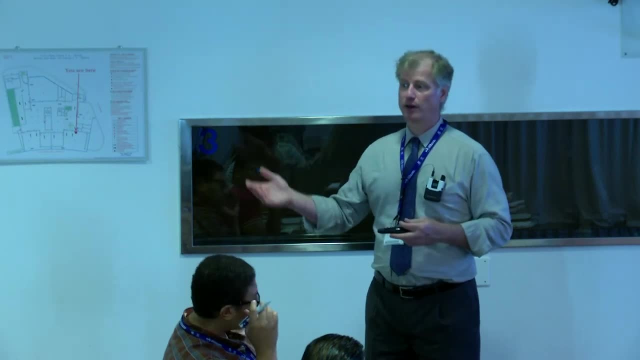 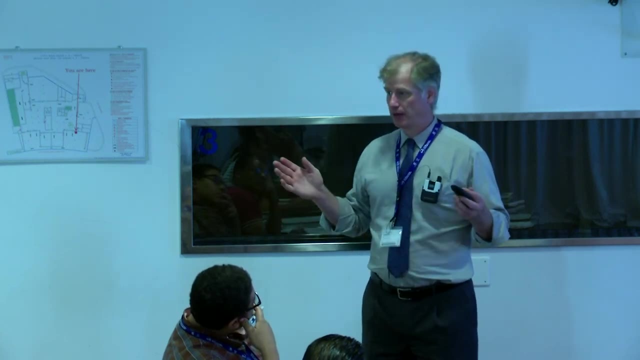 So they probably have their own security concerns and out of that, maybe acquiring nuclear weapon capability was perceived as vital from their standpoint. So maybe that's what they were pursuing all along. I don't know that They could have been acquiring research and other technologies from other states. 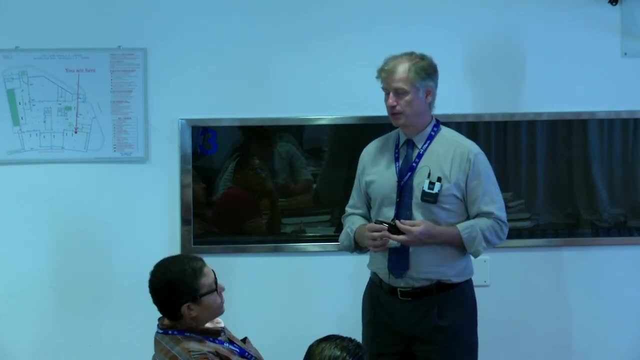 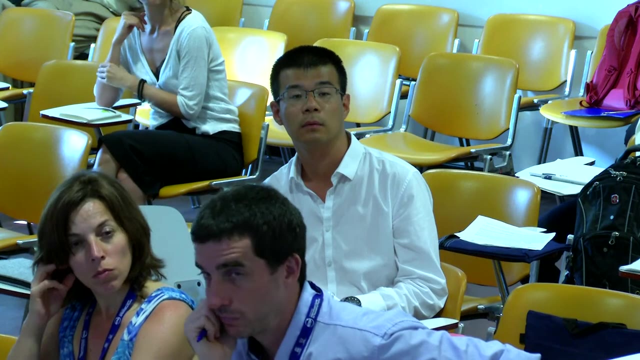 under a peaceful, the auspices of a peaceful program And they weren't a member of the NPT. I'm not sure exactly when they signed, but when they put a comprehensive safeguards agreement in force and they came out with their first initial listing. 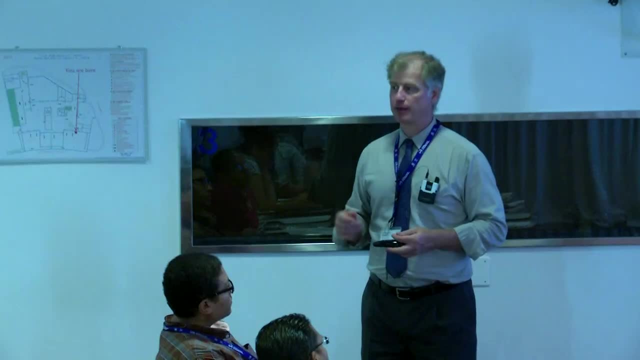 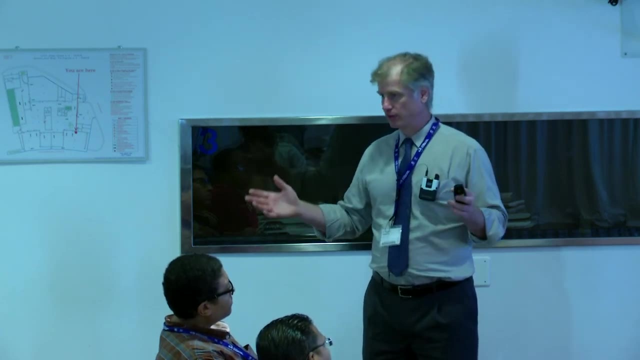 there was some doubt about that, that they list everything every time they've operated their research lab. So there's some doubt initially, and then there's a lot of frameworks and cooperation over the years involving multiple states. I don't know. I think they maybe were playing for time. 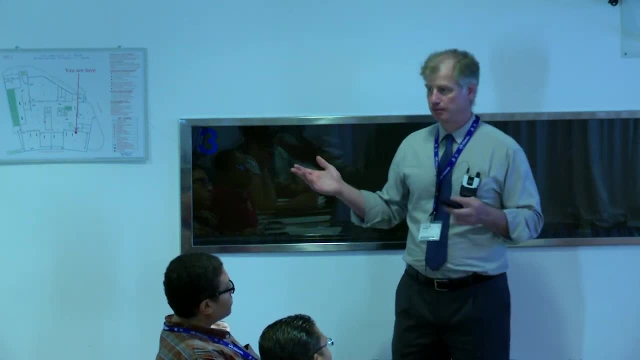 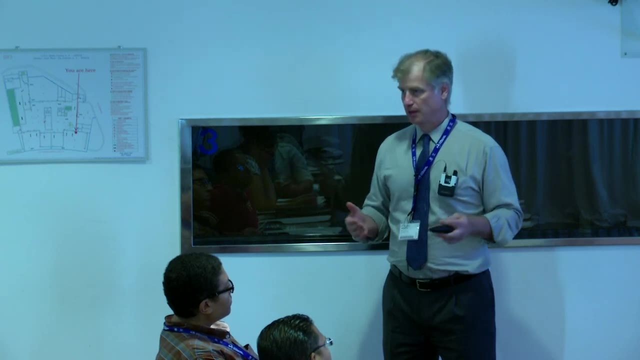 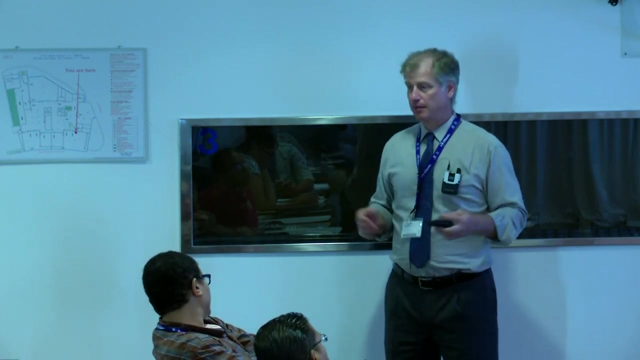 They've been negotiating, a little bit cheating, a little bit Negotiating, but that's just my opinion. So they probably took advantage of a system in order to gain time, to acquire know-how and capability. But from their perspective again, maybe they view it as they have an imminent security concern. 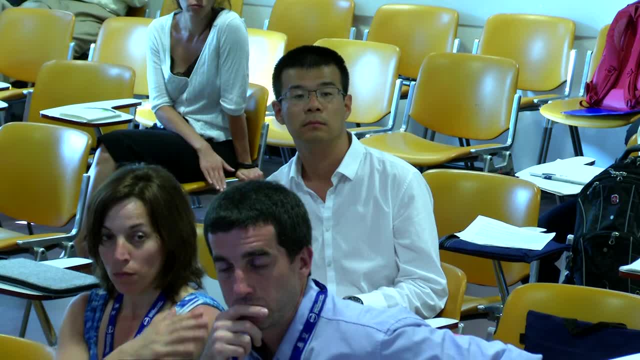 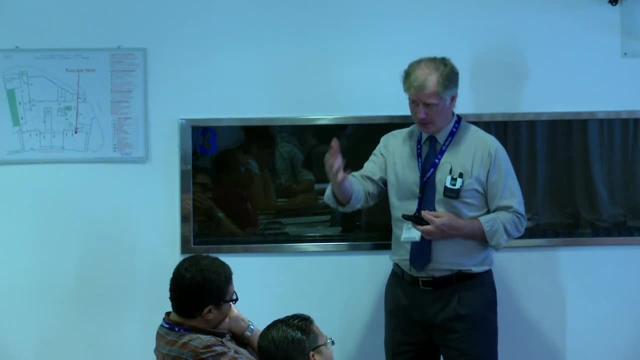 and they decided that overrides their obligations to the NPT or whatever. But they also- I don't know the exact dates, but they basically threatened to leave the NPT because the NPT you can leave, You have to give 90-day notifications. 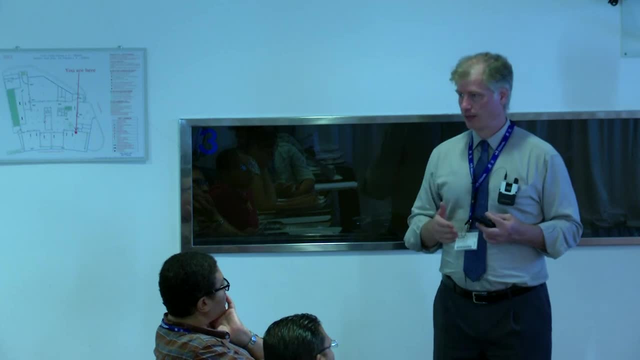 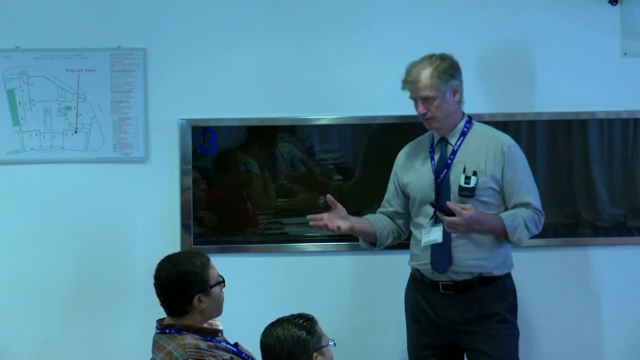 like leaving your apartment, I guess. So they did this and gave this notification and then, I think at the 88th or 89th day, suspended it. Then later, I think several years later, they reactivated it, but only waited a day or two. 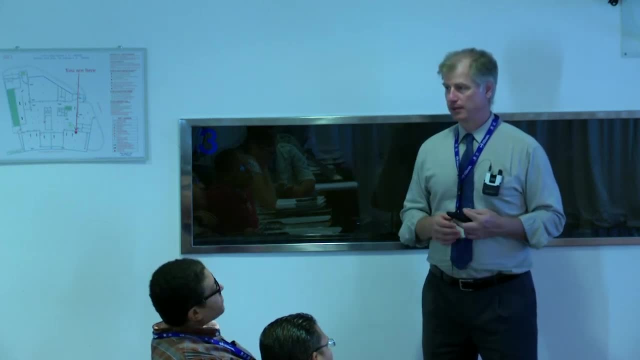 for the full 90 days to expire and they left the NPT And there's been efforts to go back and look at parts of their fuel cycle, But there's, you know they had a, they had a reprocessing facility which was known about and inspected. 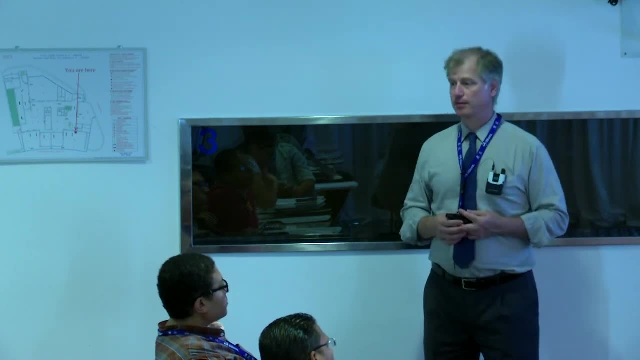 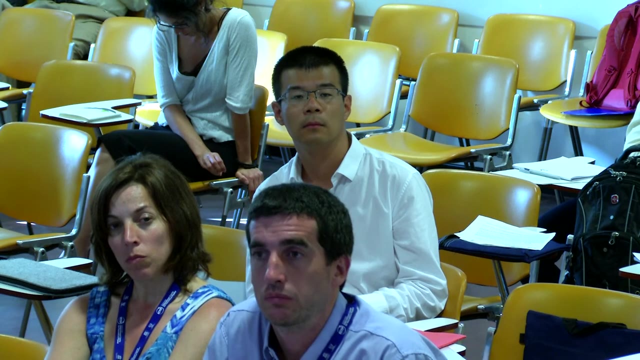 but they apparently also had an enrichment going on which they didn't inform the agency about. Although they didn't, they did invite some foreigners to look at that and they think they confirmed that they saw it look like a gas-centered future enrichment plant. 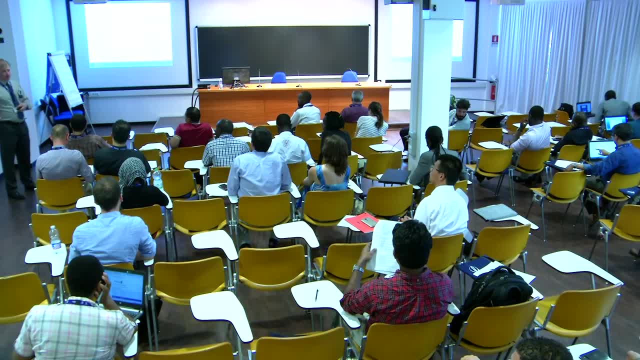 So they basically modified a facility- fuel fabrication- to enrichment, but not under safeguards. But they had also left the NPT. There's other states and I know that this: if you leave the NPT or you never join the NPT. 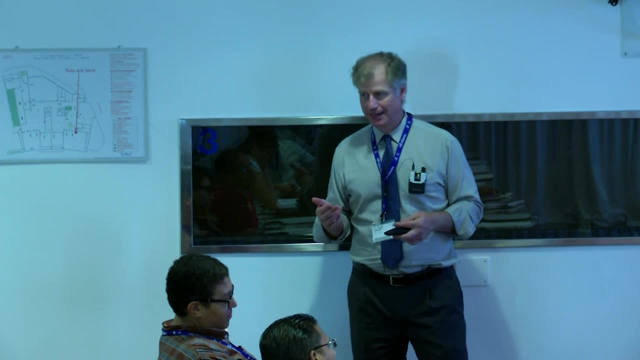 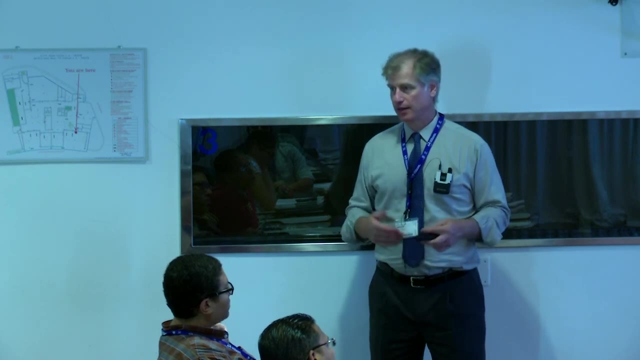 the NPT has been fairly successful. Only one state has left it. The three states with complex nuclear fuel cycles have yet to sign on. sign on to the NPT. So they're not violating the NPT by having nuclear weapons, But it may limit their access in terms of just commercial nuclear trade. 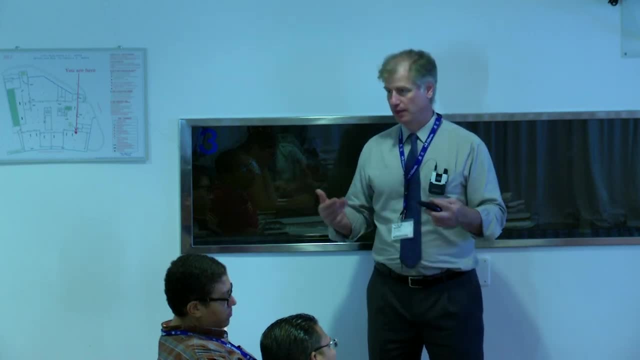 Some states may not trade, The states that haven't signed the NPT. that's one of the benefits of signing the NPT is you get advantages you get. I'm talking about these research reactions. I'm talking about these research reactions really here. 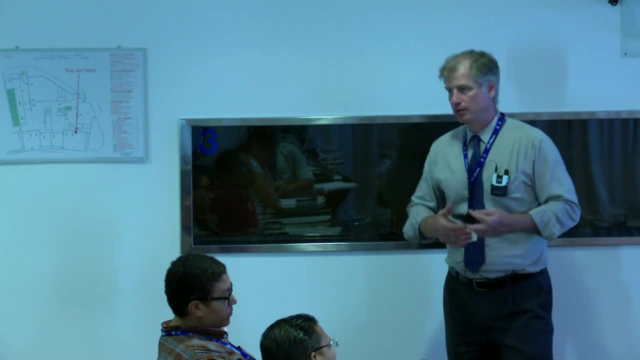 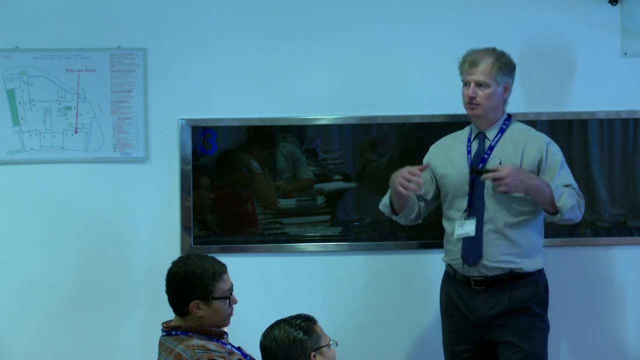 If you get research reactor technology, that might be a starting point to understand for training, for your medical isotopes, industrial isotopes, And usually it starts with a research reactor and then it expands into a power plant. So you get the benefits of nuclear energy, which is actually 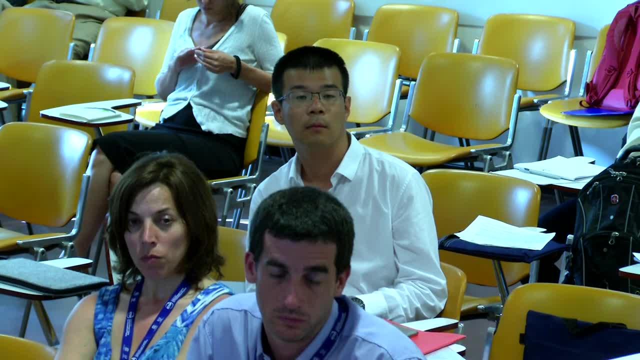 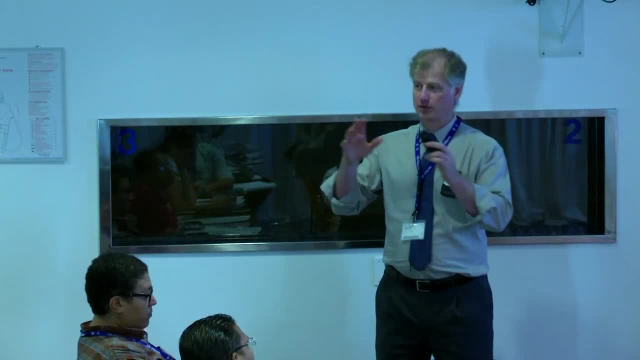 that's. the mission of the IEA is to promote and accelerate the uses of nuclear energy. I just work in the department- that's a little more paranoid- to make sure that when that nuclear material or those facilities are provided, that they come with strings attached. 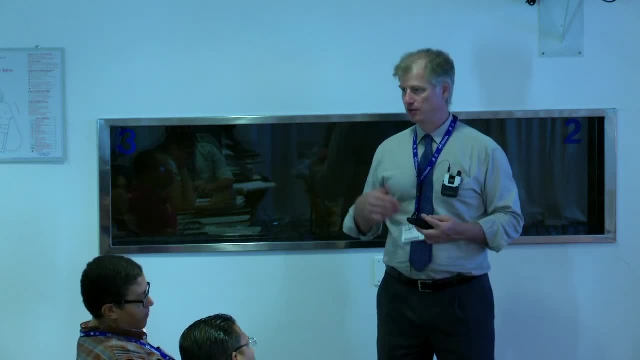 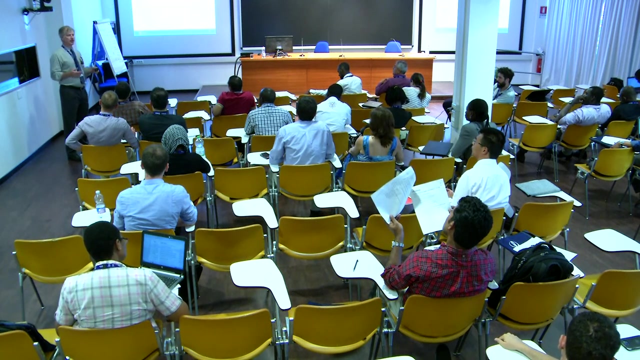 So the strings that are attached to these inspections and these verification and these conclusions, Probably not the best outlook, because instead of like what is it? trust but verify, I guess I'm more the outlook: don't trust and verify. But at the end of the day I can, I just walk, I approach things. 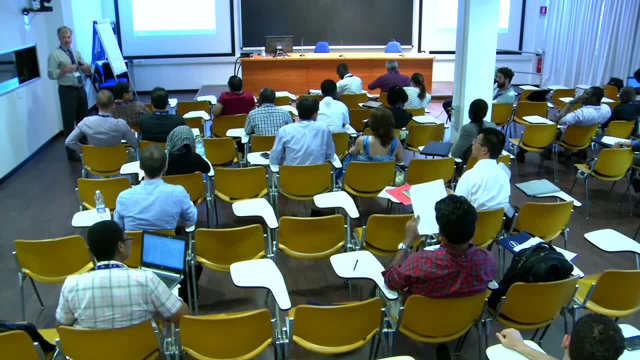 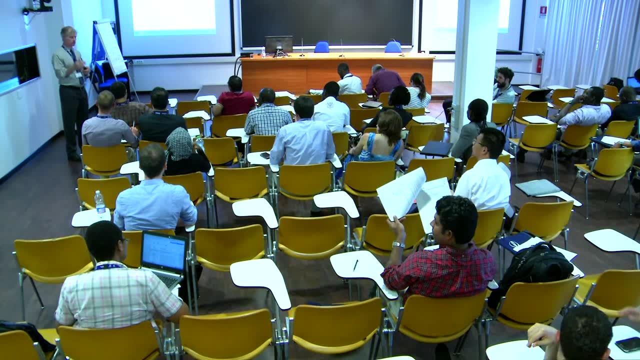 with that, because it's a what if for all states. But I can always step back at the end and say, okay, we took a very conservative outlook and there was nothing going on. Our conclusions are sound: There's been no diversion. There's no indication of undeclared material activities. 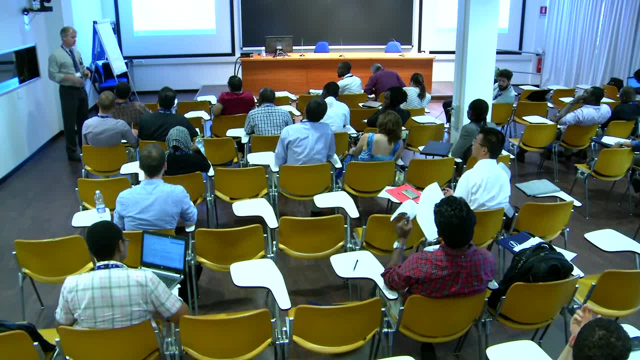 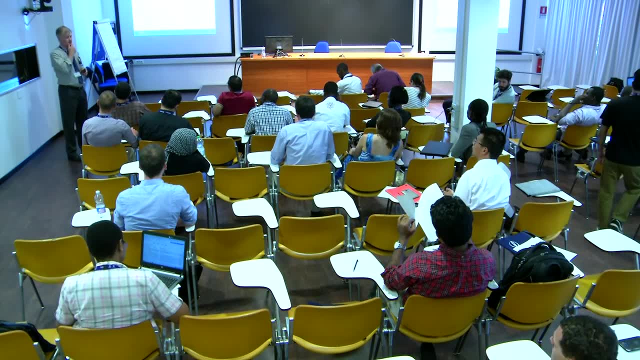 But I think it's good to go in with an outlook that you're looking for it and you don't find it, as opposed to saying, ah, this is the same old state. I've actually had states say that to me. I've had, I've been inspecting in some states and they say, gosh. 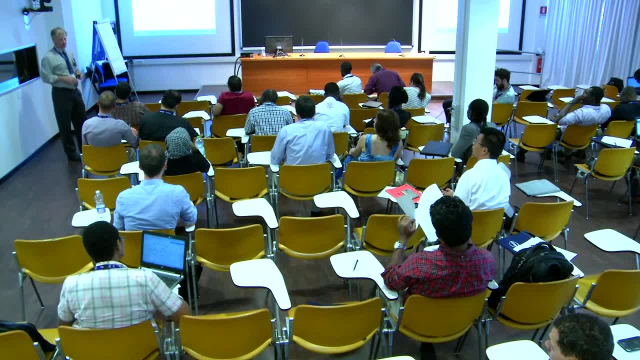 you're treating us like we're around or something And so you know another state. say a non-controversial state To me. I'm thinking: okay, then I'm doing my job, If they think they're getting a lot of intense verification. 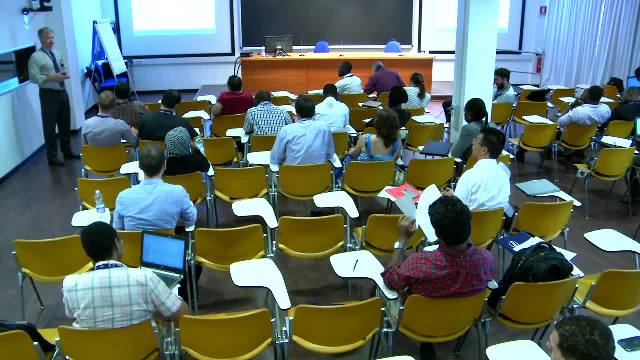 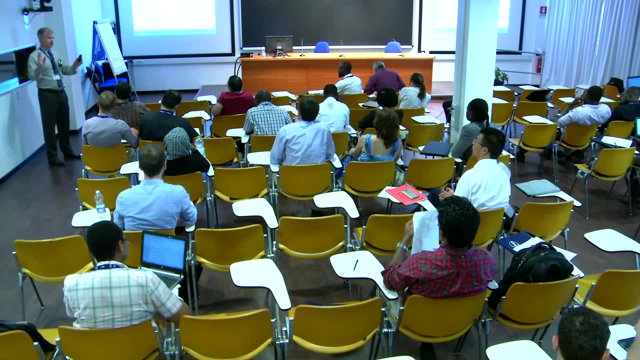 that's within the scope of the inspection, then I'm doing my job because I feel like I've got a. I can't say: oh, this is, you know, whatever Belgium or Bolivia or Germany or Canada, I'm not, you know nothing going on here. 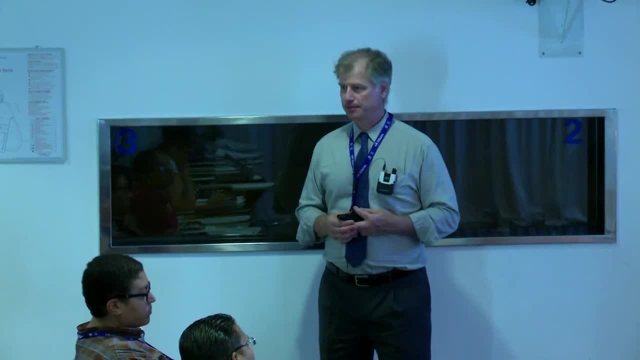 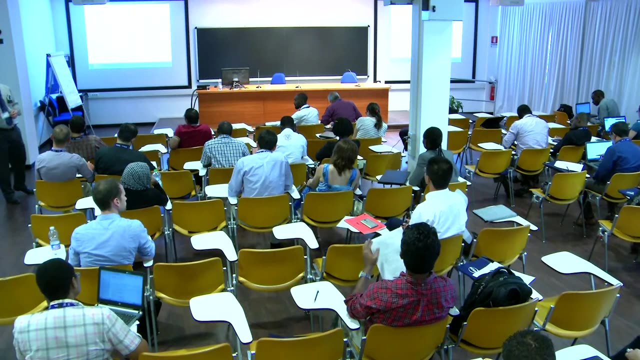 But then things start to fall apart, start to lose credibility. so Any other questions, All right. Thank you, Thank you.